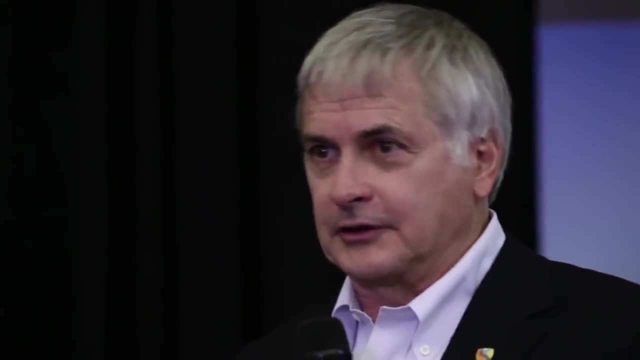 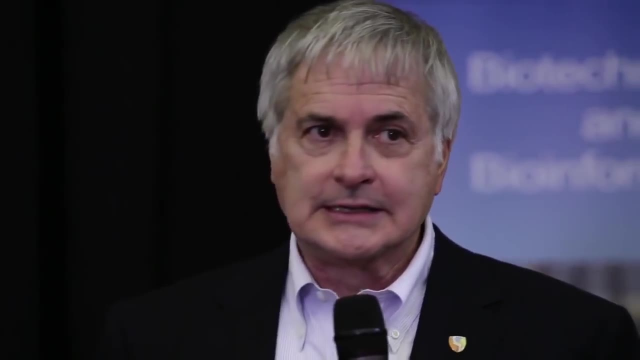 He's been saying that for 20 years. that I know of Jill Tarter says my grandkids may find ET and so forth. so she's a little more conservative in her answer and I was giving an answer as well. I'm going to try and give you what might be a better answer, but probably isn't. 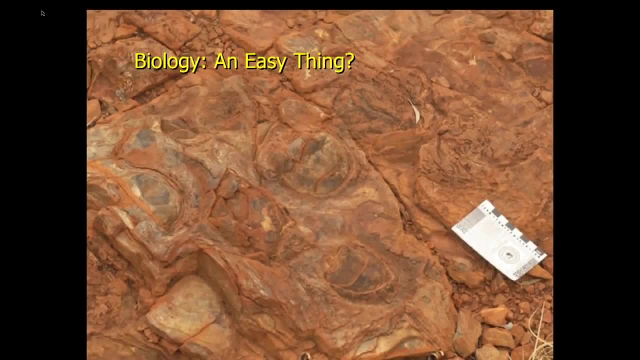 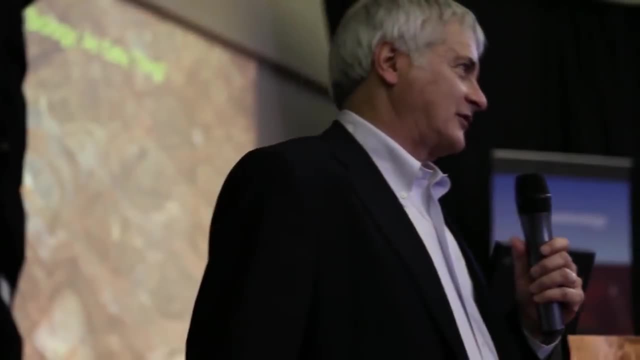 Let me just first say that the reason that we think that the routes are safe is because they're very, very good. Let me just first say that the reason that we think that the routes are safe is because they're very, very good. What's happening out there is partially just a sunny view of the cosmos that suggests that this planet might not be a miracle, that what's happened here may have happened in many places. 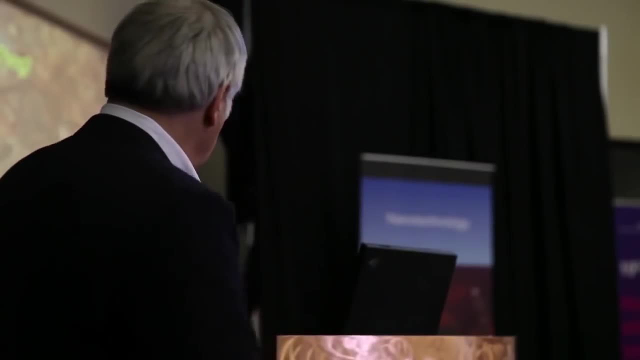 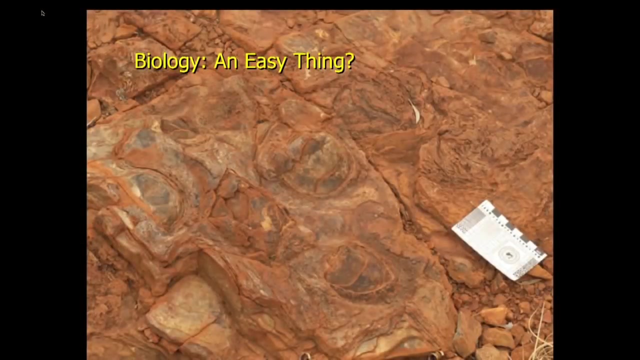 One of the possible bits of evidence for that can be seen in this photo here which I made in northwest Australia a few years ago, up in the Pilbara Hills. Anybody from Australia it's not a place you'd normally go, unless you're a cow or a fly, but you see some rock there. That rock. there's a business card on the bottom right. I put there for scale That rock. there's a business card on the bottom right. I put there for scale. You can see some rock there- That rock. there's a business card on the bottom right. I put there for scale. 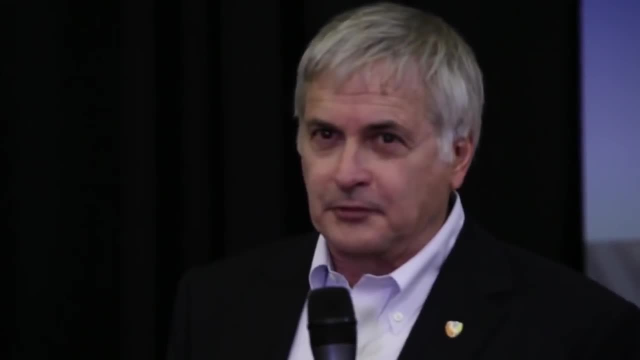 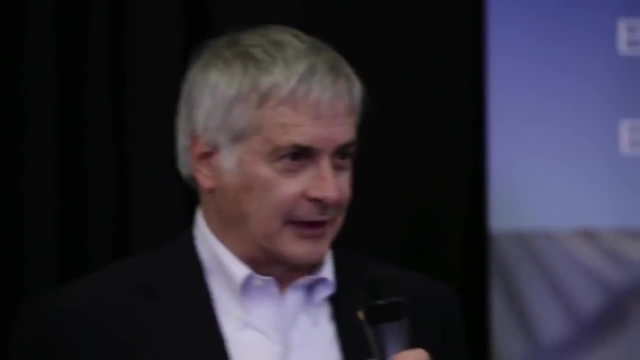 that rock is known to be about three and a half billion years old, plus or minus a few percent. We know that from radioactive dating, which was actually the kind of dating that I did in high school. So we know how old that rock is and you can see. 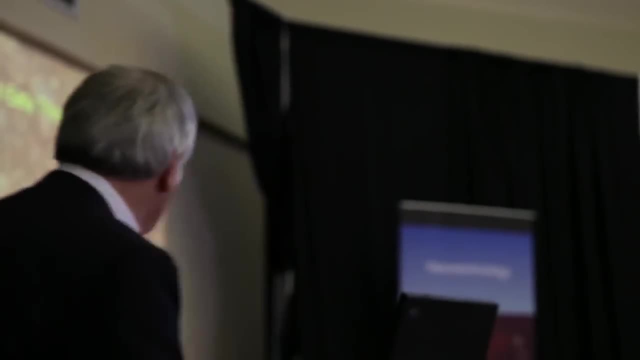 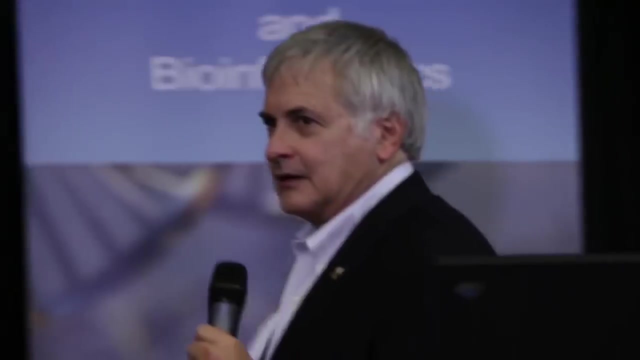 there's some. does this have a laser pointer? It doesn't matter. You see these sort of round shapes here look like cauliflowers in the rock, And the question was: what are those things? Are they just geological formations that happen to get ensconced in the rock there, or are they the remains? 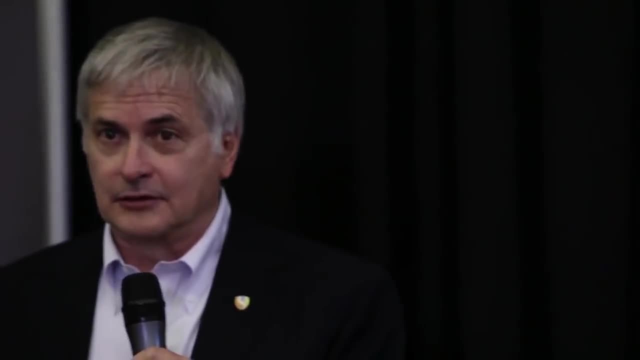 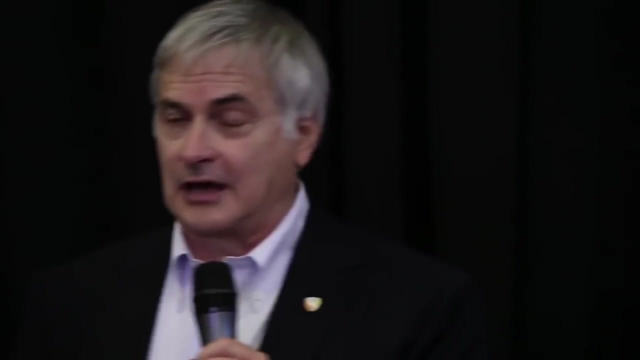 of bacterial colonies, stromatolites, from three and a half billion years ago, And the consensus now is it wasn't when I made the photo, but today the consensus is these are fossilized bacterial colonies, stromatolites. 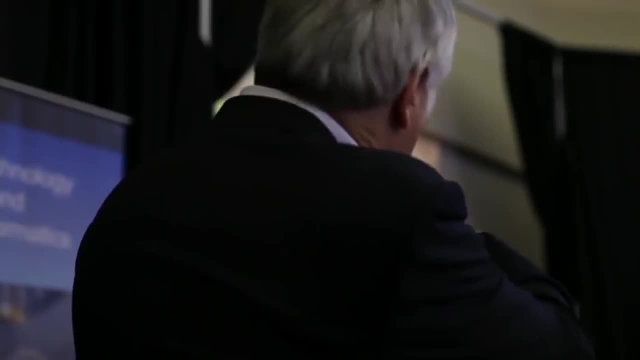 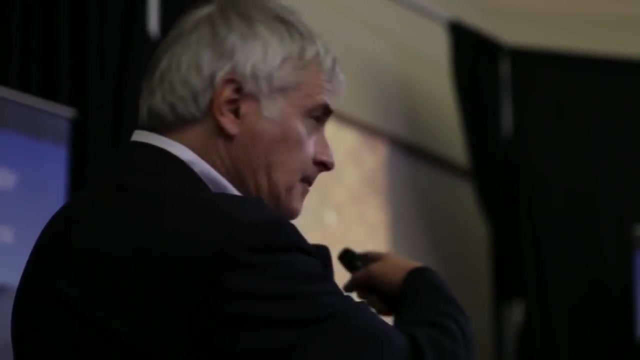 Bacteria themselves don't make such great fossils, although occasionally they may, but the mounds they build, of course, are macroscopic, big enough to be fossilized, and that's what we see here Now. the point is, you all know the Earth. 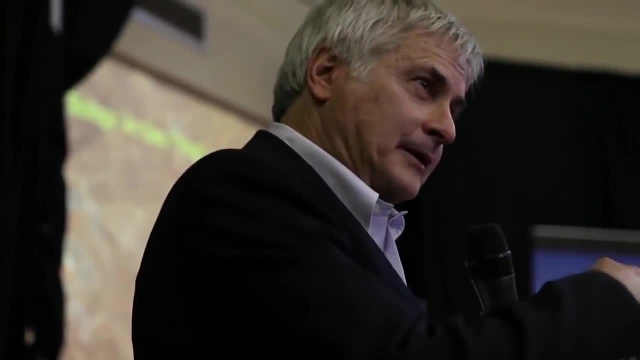 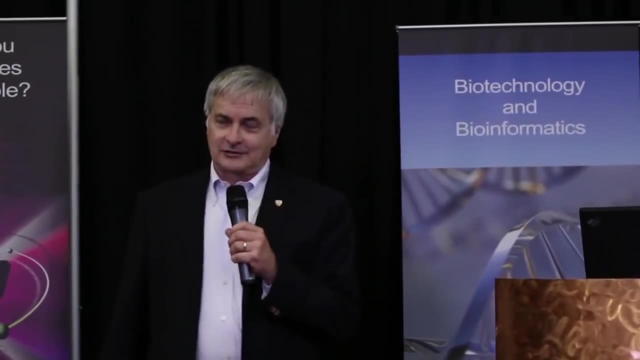 is only four and a half billion years old. So three and a half billion years ago, which is rather young in the Earth's history, there was already life and fairly sophisticated life, And that suggests- doesn't prove, but it certainly suggests- that life is not an improbable event. 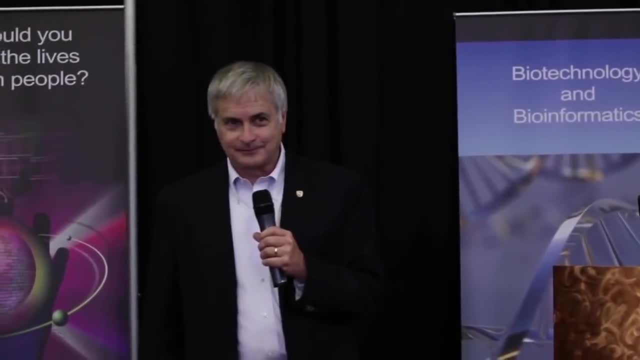 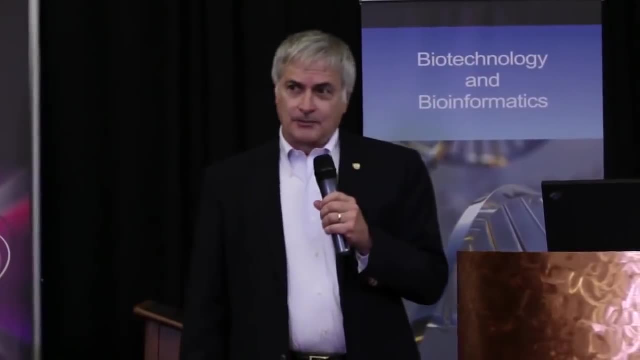 because it didn't take very long to get it started. Sort of like if you go into a casino in Las Vegas and you put a quarter in the slot machine and $10,000 drops out the bottom, you might conclude: well, gosh, that wasn't. 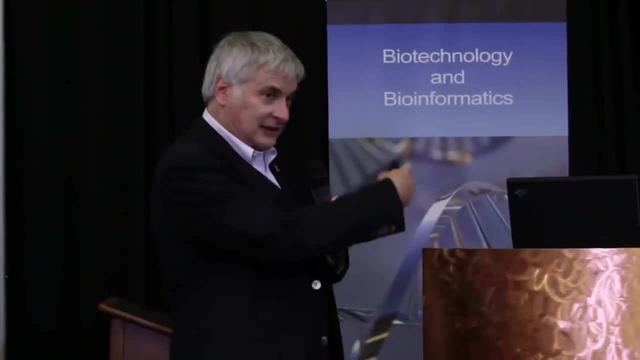 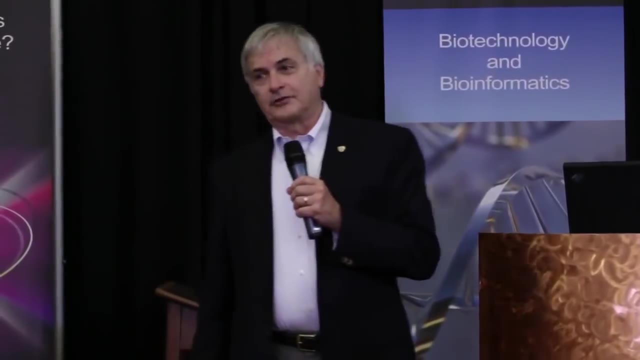 a very improbable bet. Now, it might have been. it might have been that we're just lucky, because otherwise you wouldn't be suffering through this, But on the other hand, this is suggestive. The other thing that's suggestive, of course, is merely the size of the universe. This is just one of the many surveys of galaxies. 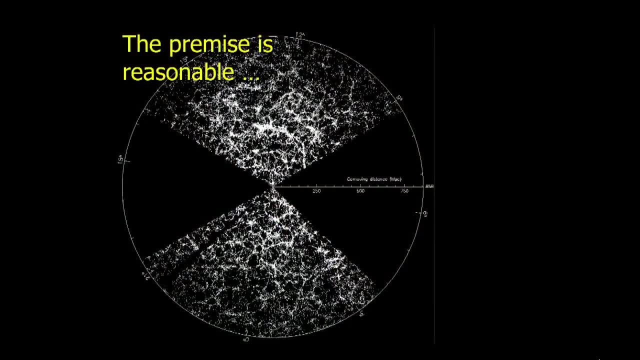 of the universe. I don't know how many of you are interested in astronomy, but every one of the dots here is a galaxy. These areas on the left and right here are just areas that were unavailable to the telescope, so they're dark. 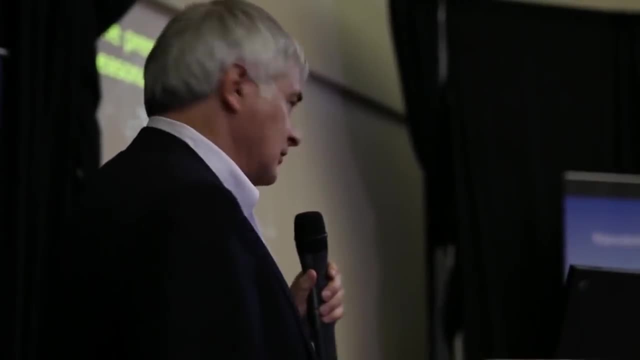 But in fact you can see that the universe is fairly homogeneous in a large sense, but rather inhomogeneous on small scales, because the galaxies are distributed in filaments and sheets, And that's what we're talking about here. And that's what we're talking about here. 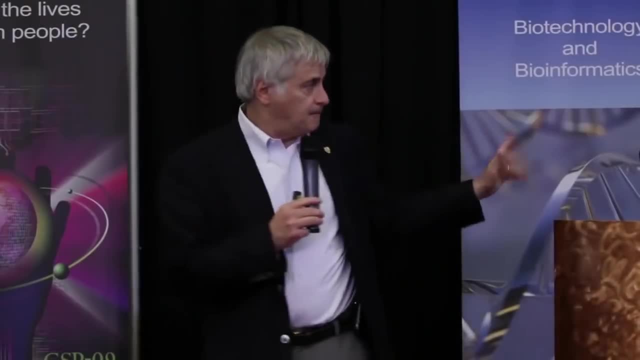 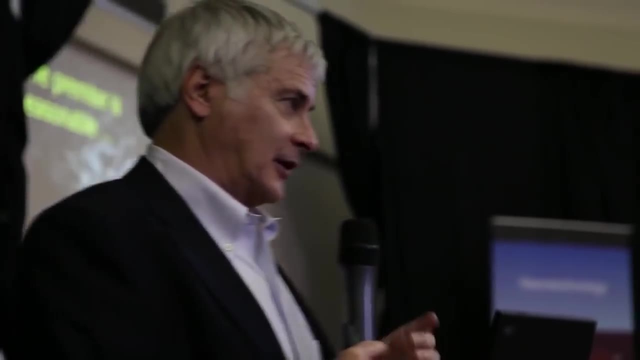 And so forth and so on. That all tells you something about how the universe was born, but the important point is that there's a lot of real estate out there, right? Our own galaxy has a few hundred billion stars, and the number of galaxies we can see is on the. 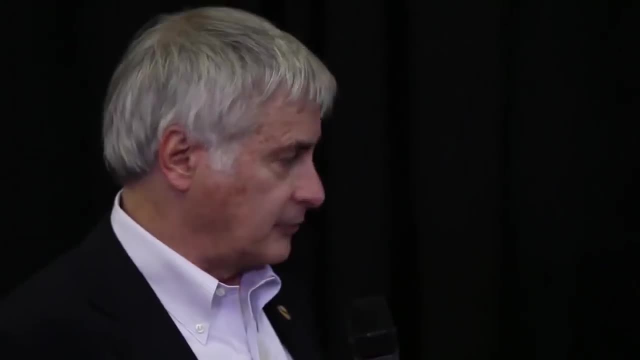 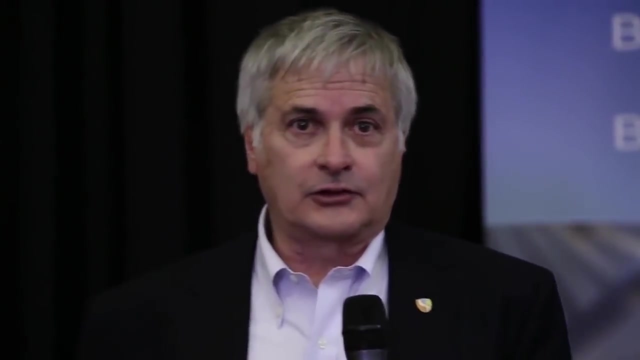 order of a hundred billion as well. So most of you have multiplied those two numbers together in your head or on the back of the shirt of the guy in front of you. That's 10 to the 22 stars in the visible universe. The actual universe is of unknown size. It might be infinite. it might not be infinite. but in any case it doesn't matter. It's just a matter of how many stars we can see, And it doesn't matter. It's still a lot of stuff, just in our own universe. That's just a close-up of one of these things. 10 to the 11th galaxy is visible to our telescopes. 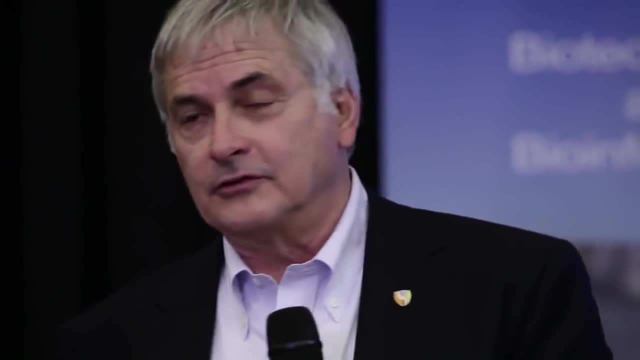 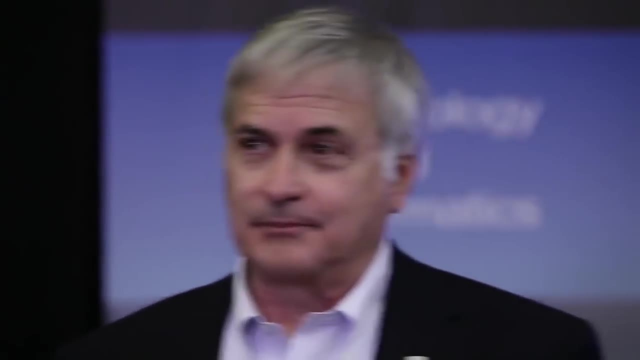 Now, the other thing that's kind of new in this business and wasn't known when the first SETI experiment was done back in 1960, is how many of these stars have planets, because you're not likely to cook up life on stars When I was a kid, which was sometime before the 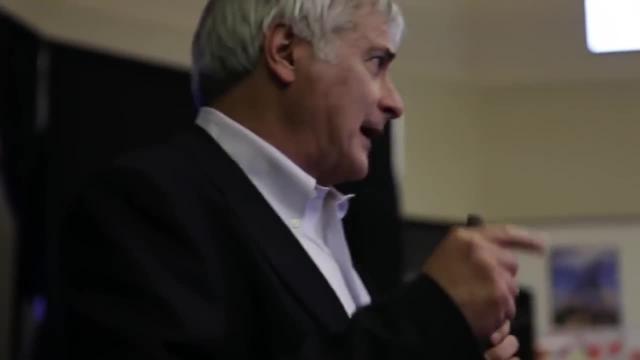 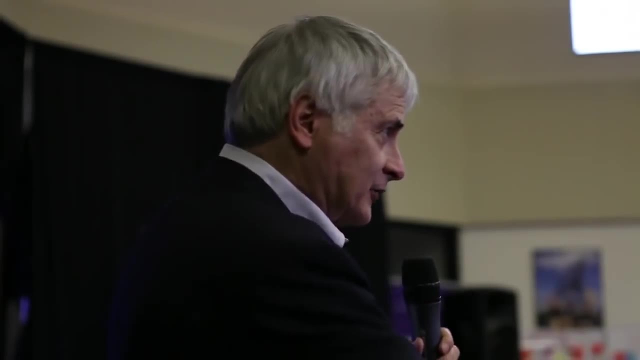 Crimean War. we were told that the way you made planets was to rip stuff out of the sun. but there was another star that had sort of a fender bender where the sun didn't actually hit it, but it got close, pulled out gas and that formed the planets. That was a theory. 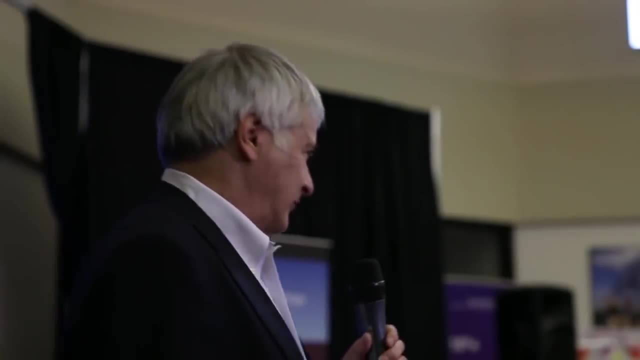 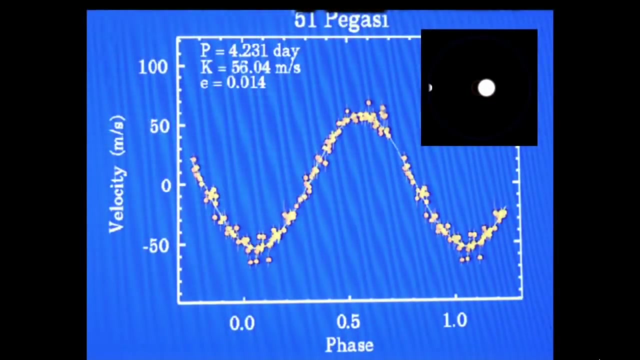 that had a long run, even though it turns out that it doesn't work, which kind of ended the run. But if that were the way planets were made, then this is the only solar system in the galaxy, because it's very unlikely that two stars get close enough together to 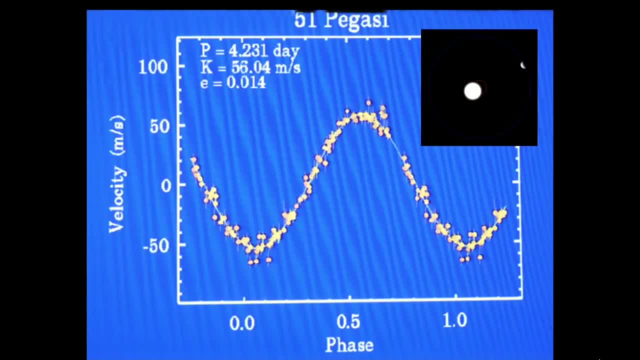 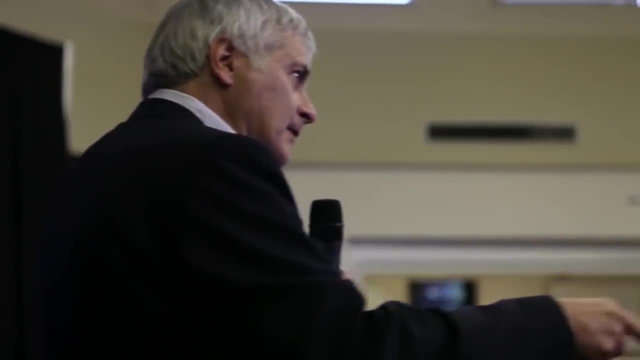 have this happen. You can work it out yourself, right? You all know the scale of the universe. If you reduce the sun to the size of a ping-pong ball- which that's a project we leave to the students, we leave to the students here for the weekend- if you do that, then the nearest other star 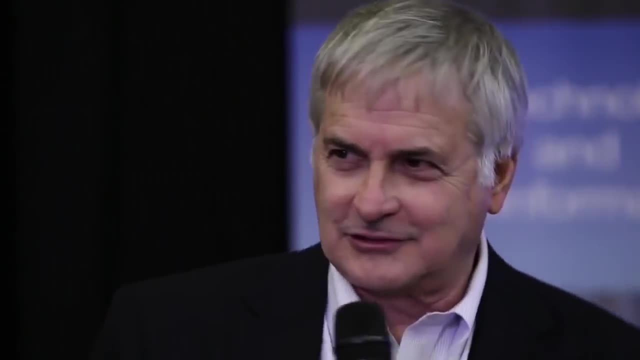 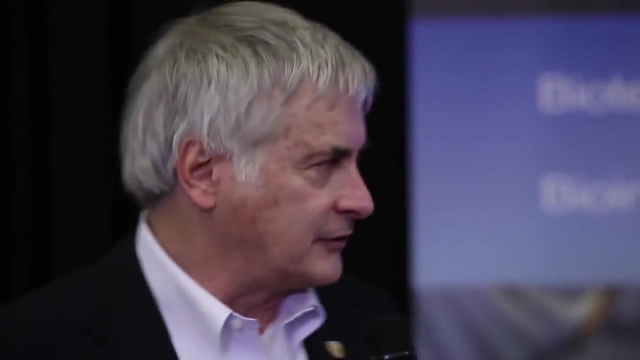 is another ping-pong ball, but it's in Salt Lake City. So what are the chances that those two ping-pong balls are going to get within an inch or two of one another just by the random motions as they move very slowly through space? Obviously, it doesn't happen very often. 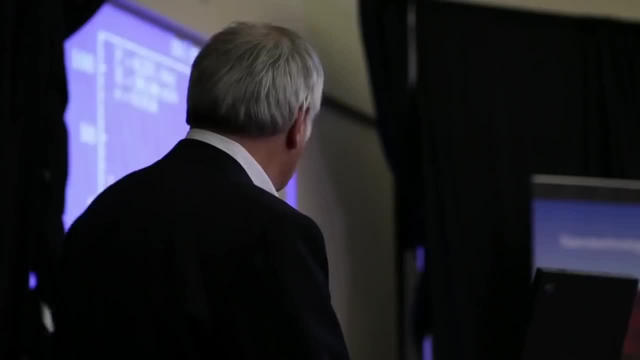 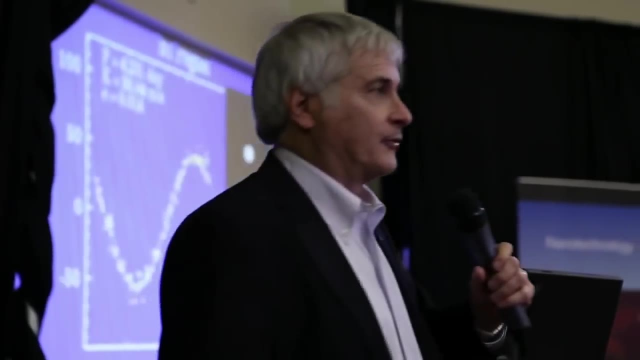 In the entire history of the galaxy. you might get a collision like that in this neighborhood. So this was suggesting that planets were rare. Well, we know that's not true, thanks to the work of astronomers since 1995, who have found more than 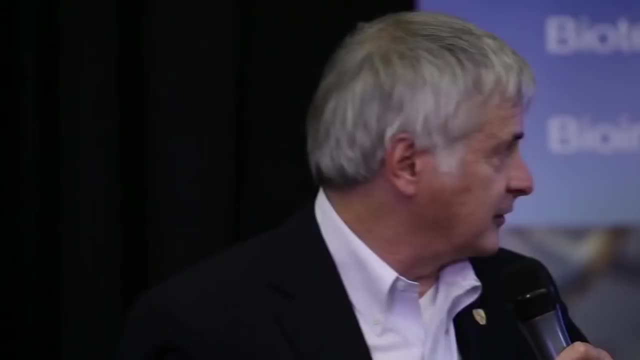 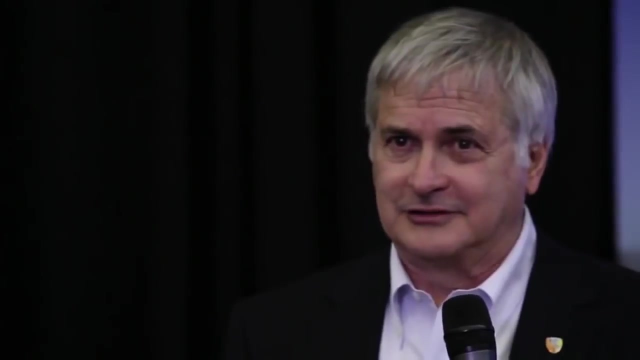 400 planets around other stars, and they mostly have found them via this technique here. That little cartoon shows you that well, finding the starsorry, the planet itself, is very difficult, because planets are dim, right, And they're right next to a very bright star. The problem for the telescopes is not so much that the planets are so dim, it's that they're near such a bright star, so the dynamic range is enormously great. It's billions to one, and it's very hard to find that planet. There are instruments being designed that can do. 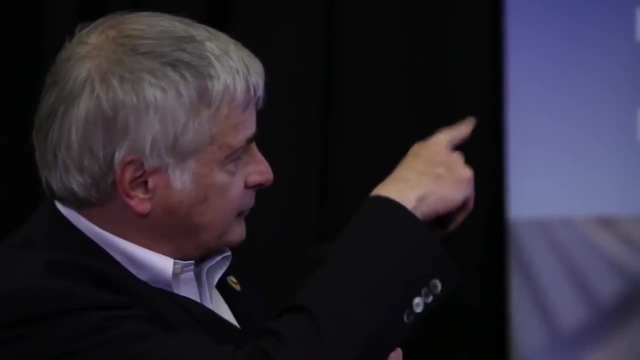 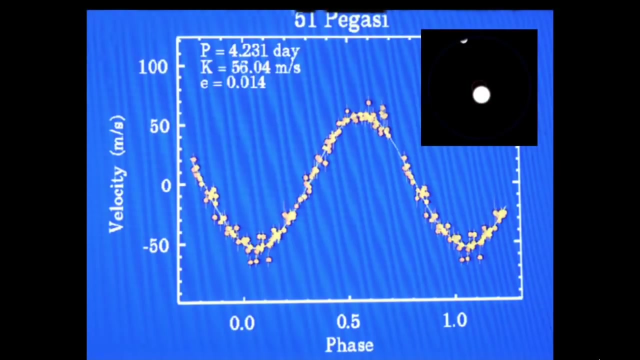 that, but anyhow, That's not the way it's done so far. Instead of looking for the planet directly, you just look for the slow wobble of the star. I think most of you know how this works, And that graph there shows you, in fact, the first planet around a normal star. data for that. 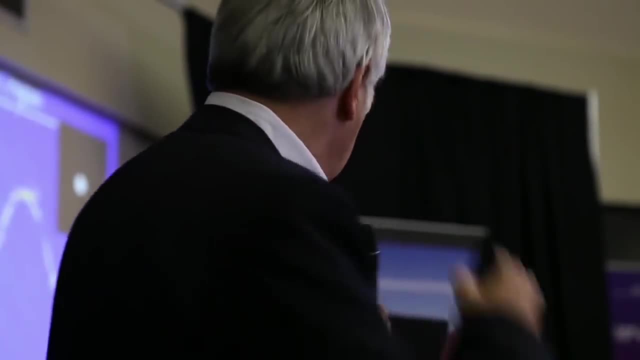 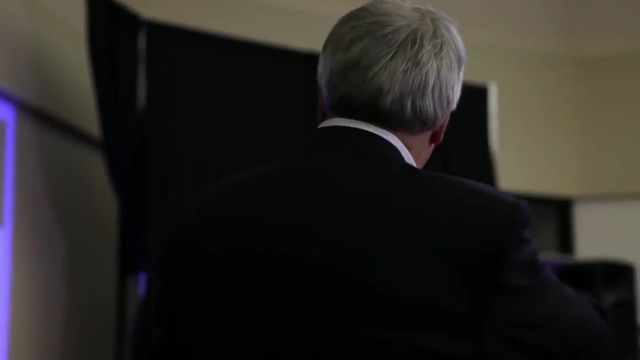 taken up here at the Lick Observatory on Mount Hamilton, not very far from where you're sitting, And you can see that. you know, for a couple of hours the star was moving toward you at about the speed at which your bicycle goes, and then it was moving away at about the same. 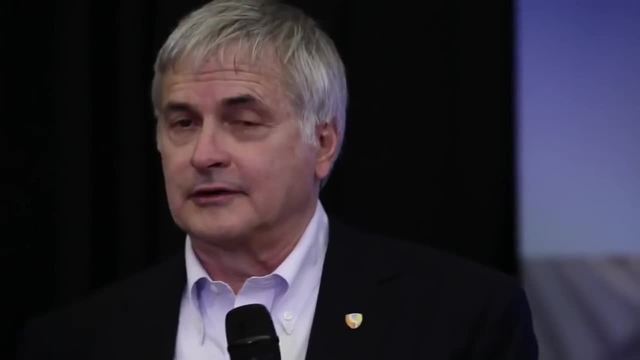 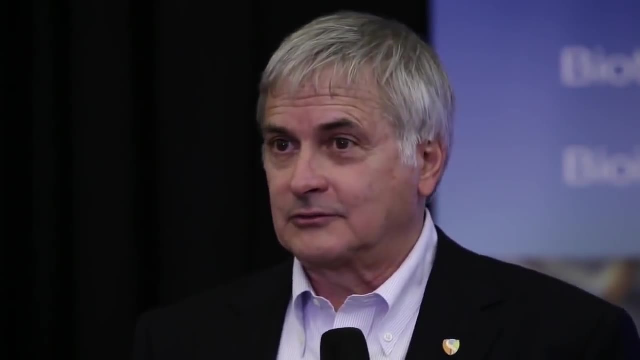 speed and then coming close and so forth. So they found these planets. We found more than 400 of these things, But that number isn't really so interesting. What's interesting is to know what fraction of stars have planets, not how many we found. That number just goes up every two weeks. 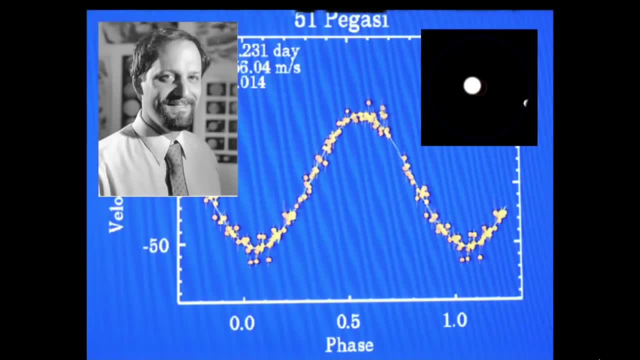 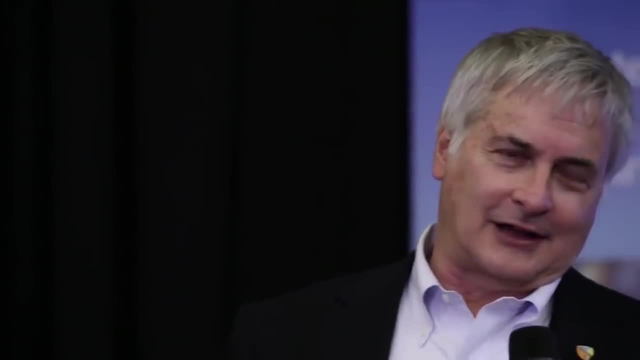 If you talk to guys like Jeff Marcy- I think it's a picture, Here's Jeff. You talk to guys like this who make a modest living finding these planets and say, look, Jeff, if you had perfect telescopes, right, so you know infinite signal to noise whatever, what fraction. 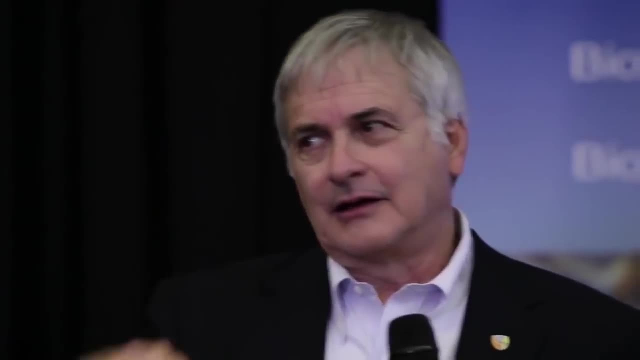 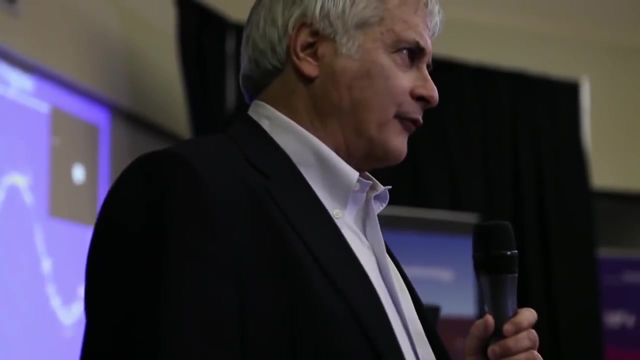 of stars do you think would show planets? And he can make an estimate of that on the basis of the statistics he has so far. And his answer to me, at least a few months ago, was: well, maybe half, maybe three-quarters. Well, to an astronomer, half is the same as 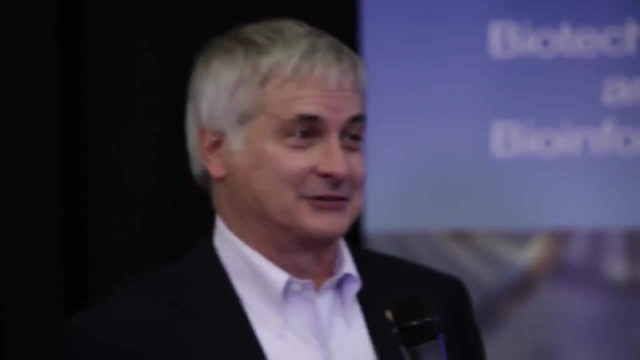 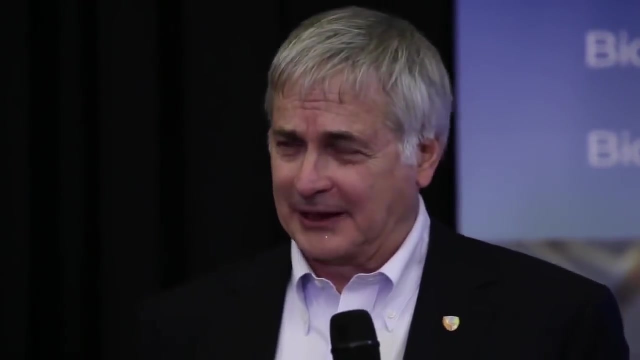 all right. I mean, there's no difference. So if you can get something within a factor of two, that's really good in astronomy. So that means all these stars have planets, right? So the only question that remains is: well, how many of these are good planets? Because 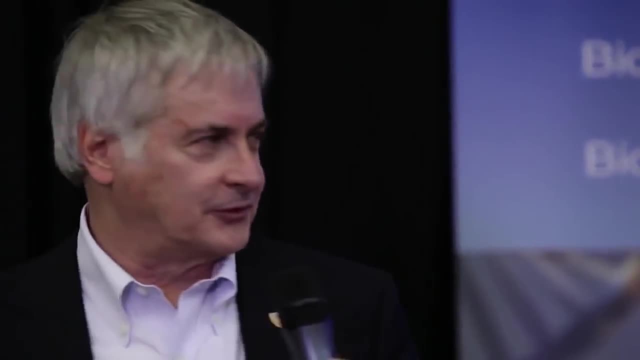 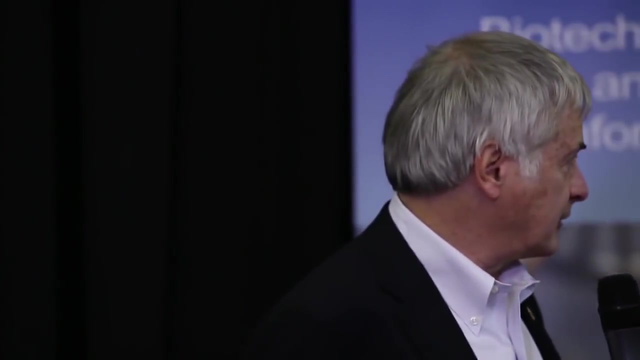 there's a lot of worthless planets around. I mean, look at Neptune. I'm sure Neptune's not big in your life And it's probably not you know a whole lot of life on Neptune. for that matter, Pluto's probably, if you consider it a planet, probably not very interesting either. So 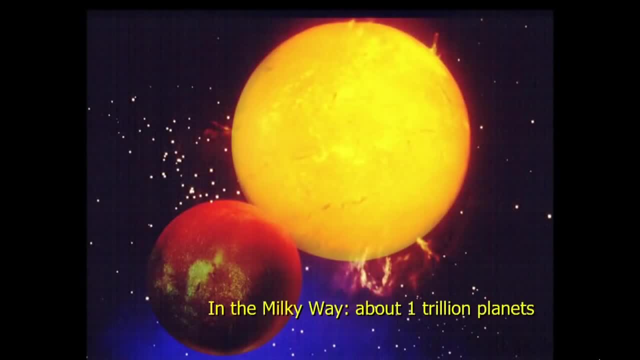 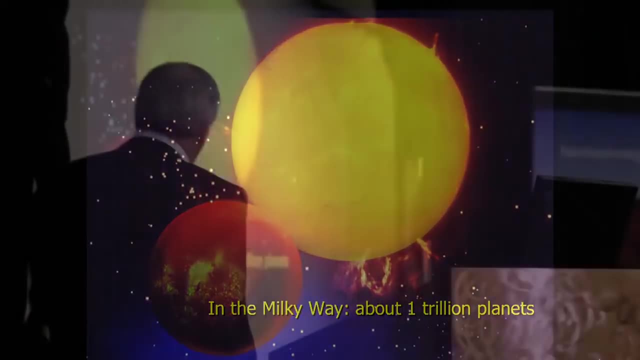 a lot of these planets are going to be like this one. This is a rendition of the planet found around that star that I just showed you the data for, 51 peg. This is actually a photo I made in my garage with the tennis balls and things like that, But never mind. 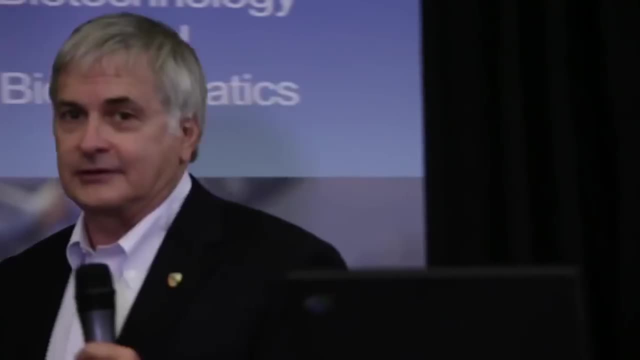 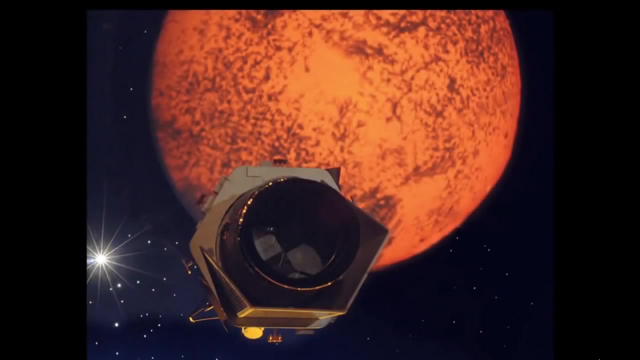 This shows you what it would look like. There are on the order of a trillion planets in our galaxy. That's the consequence of what Jeff Marcy had said. How many of them are like the Earth? Well, we don't know. We've never found a twin of the Earth. We've never. 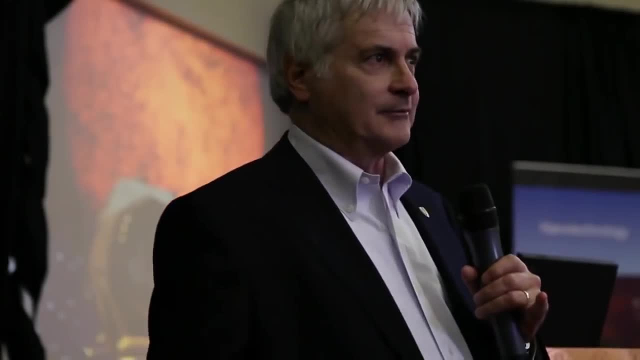 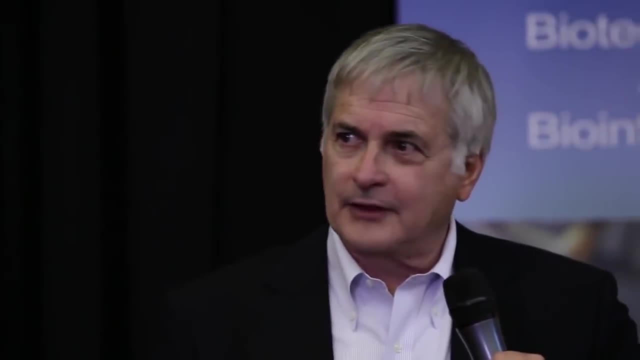 like the Earth, One that you could say: yeah, you know, this might have liquid oceans, thick atmospheres and, who knows, Klingons. We just haven't found them because they're very hard to find. They don't make enough of a wobble to find them using that technique, not with. 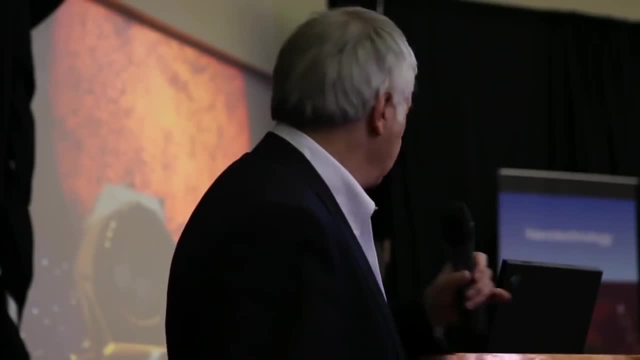 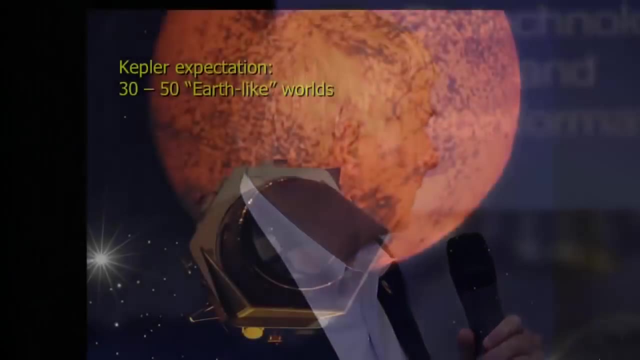 the kind of instruments we have today. It's just getting very close to being able to do that. The instrument that will find them is being run right out of NASA Ames here, and that's the Kepler Space Telescope. And Kepler is finding planets by looking for many eclipses as a planet gets in front of its star. 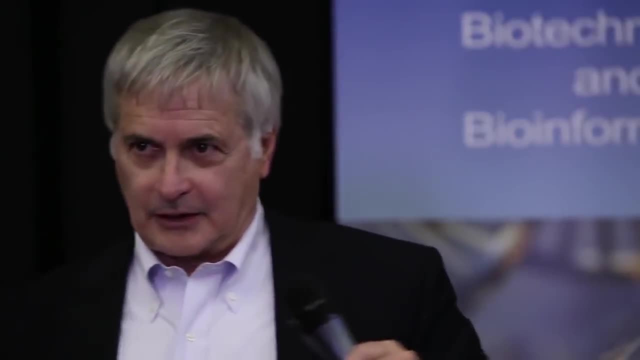 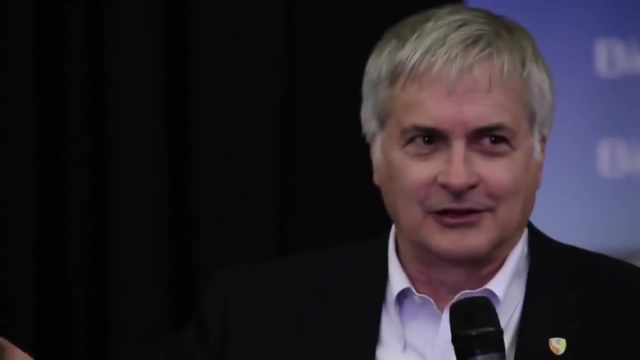 It's the ultimate staring contest. Kepler is looking at about 150,000 stars. This is a really boring job. It does look at 150,000 stars and every 30 seconds it downloads the brightness of that star. It just measures the brightness of these stars. Some of them, by chance, may have. 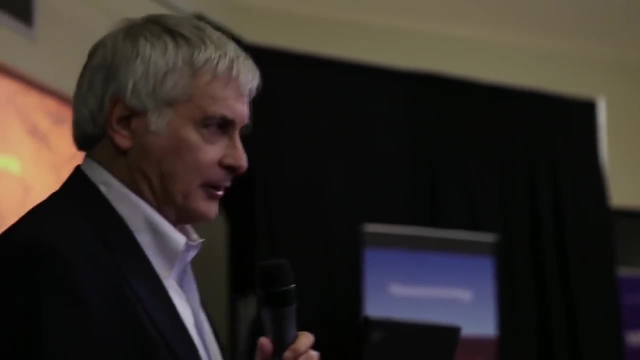 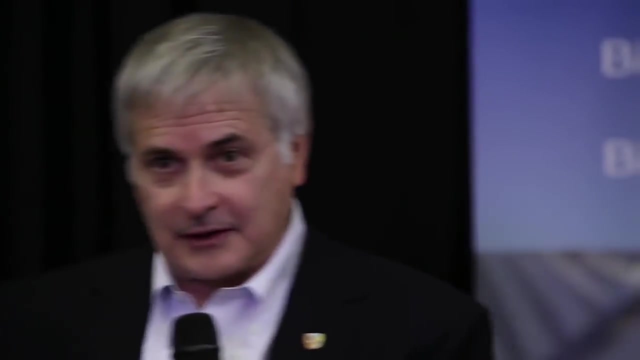 planets that cross in front of them and that reduces the brightness by maybe one part in 10,000 if it's an Earth-like planet, And if they see that and then they see it again, and then they see it a third time, now they can compare the intervals and make sure. 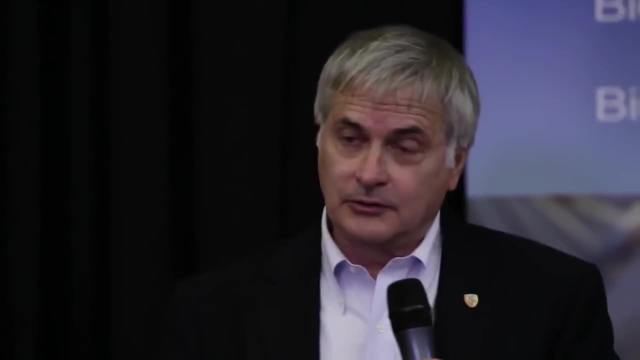 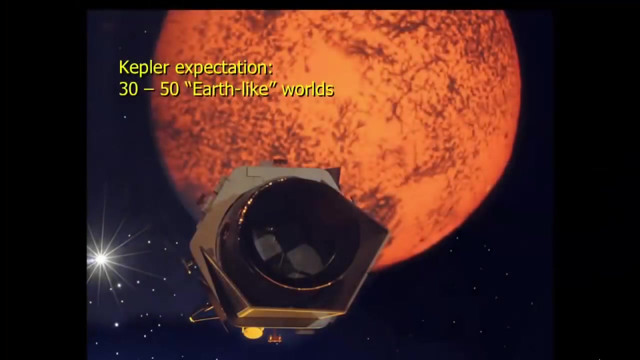 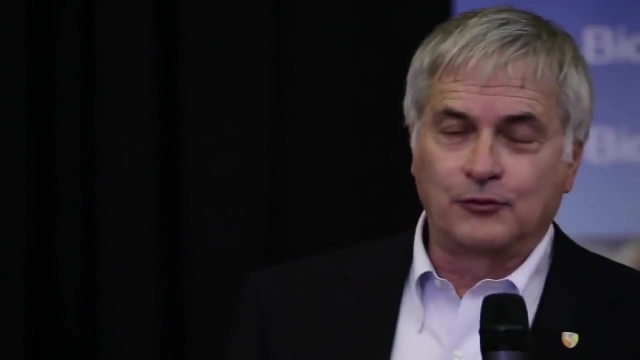 that it's really an orbiting planet and all that, And that will tell you the mass and the orbit of that planet, In other words, bottom line. this instrument will do something that no other instrument could ever have done, And that is to tell you what fraction of stars have worlds. 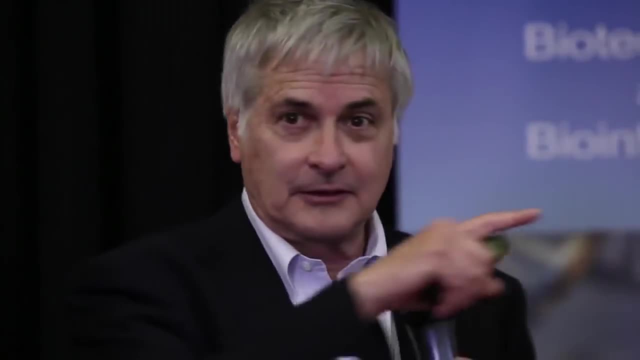 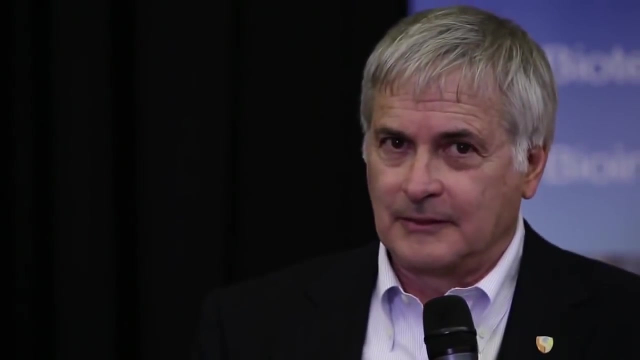 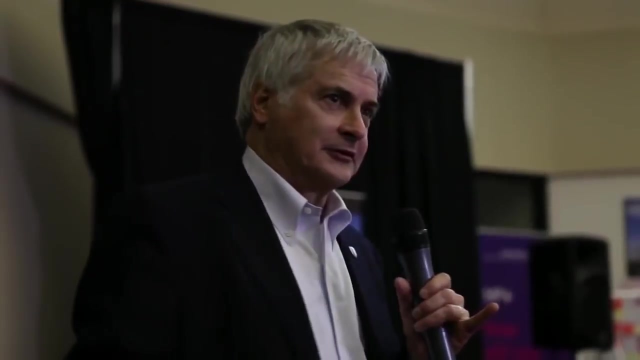 sort of like the Earth. It's a very interesting experiment, not only because it can tell you that, but because this is like completely analogous to what happened after 1492.. After 1492, within 30 years, Europeans had mapped the globe. You could have drawn a globe in 1492,, but most of it 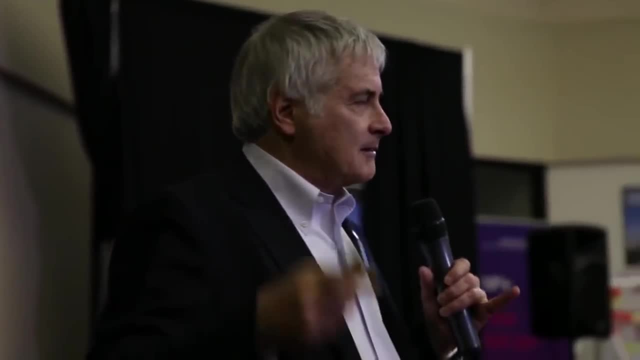 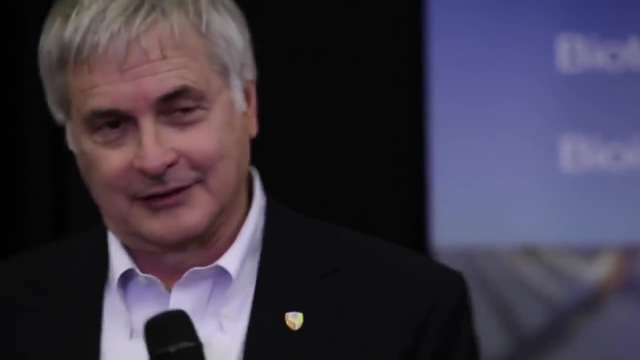 was blank. You had Europe, a bit of Africa and some of Asia, but most of the globe was blank. Thirty years later, most of the globe was filled in. There are a few things missing, like Antarctica and some islands here and there, but fundamentally it was done. One: 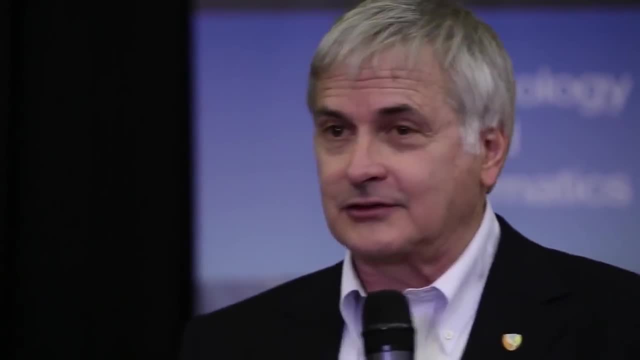 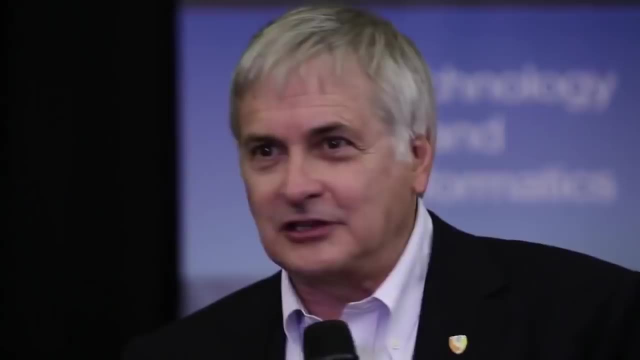 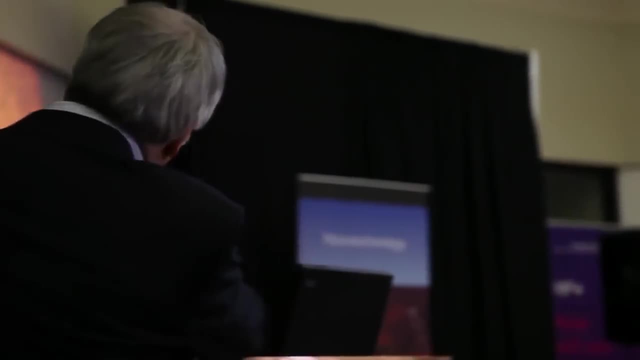 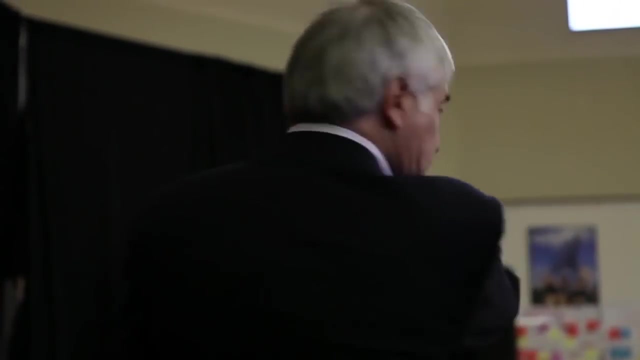 need to do this once and it'll say, okay, you know, if it really does find 30 or 50 Earth-like worlds, you can work this out. that means that a few percent of all stars have planets like the Earth. That's the smart money is saying, that's what it's going to. 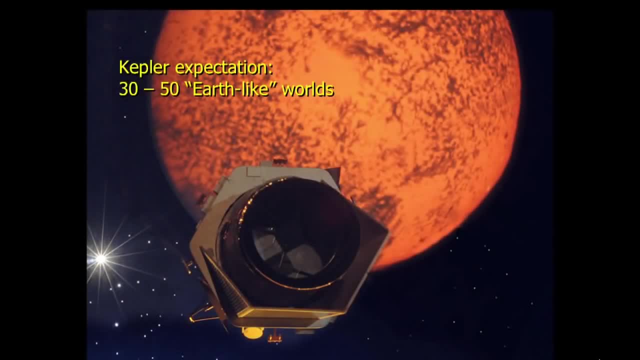 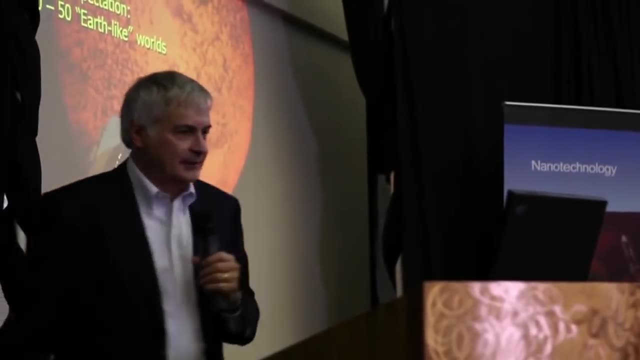 find The smart money, being those who you know successfully competed for the project. Okay, they're all here at Ames. Well, we don't know if they're right, but if they are right, that's what it'll do, And that'll be, of course, rather intriguing. That means, of course, 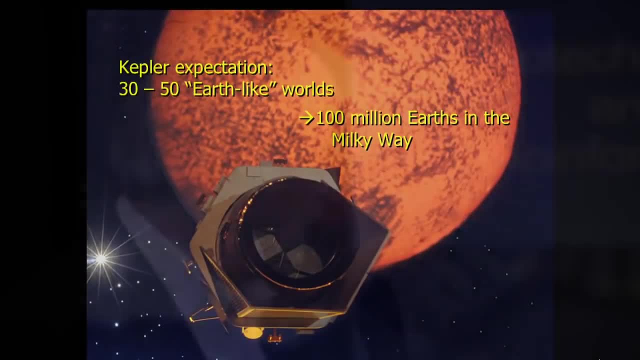 if that's the right answer, then they're on the order of you know four to five. That's the right answer. Then they're on the order of you know hundreds of millions of Earths. That number's wrong. actually It's on the order of billions of Earths in the Milky Way. 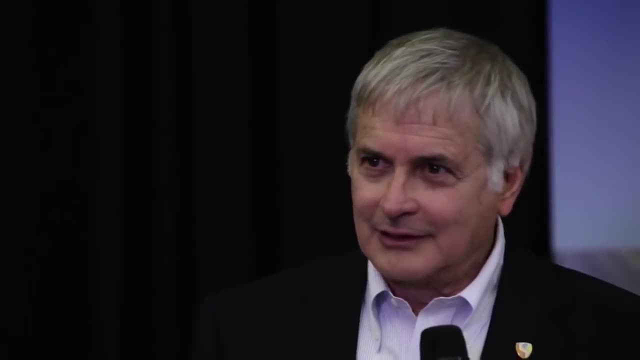 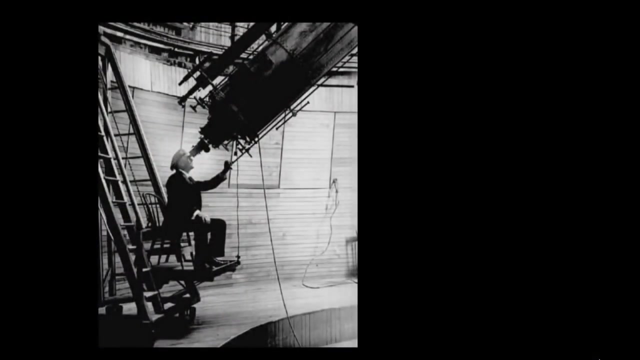 So maybe most of them are just sterile, but it would be remarkable if they were all sterile. I don't know if I convinced you. Now I want to make the argument here that it actually matters. There's a question that I think matters in this search for ET. I've tried to motivate. 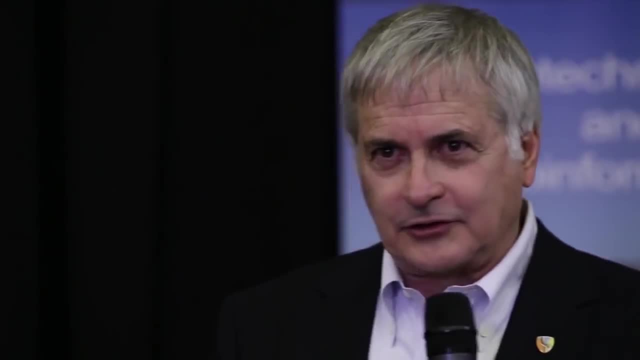 why we think they're out there. I'm sort of switching gears here, because another question you get all the time is well, particularly from the media- is well, what's the answer to this question? What's the answer to this question? What's the answer to this question? 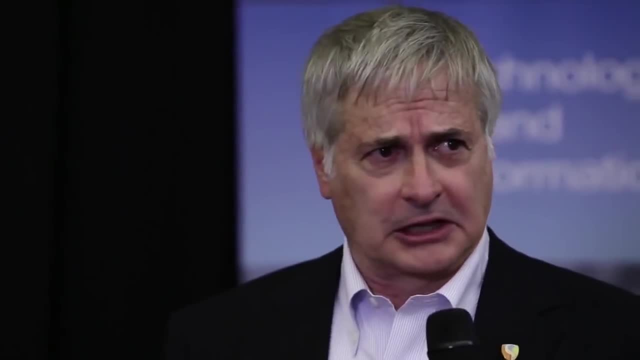 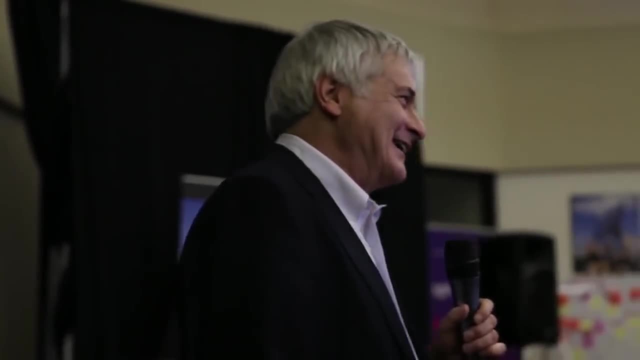 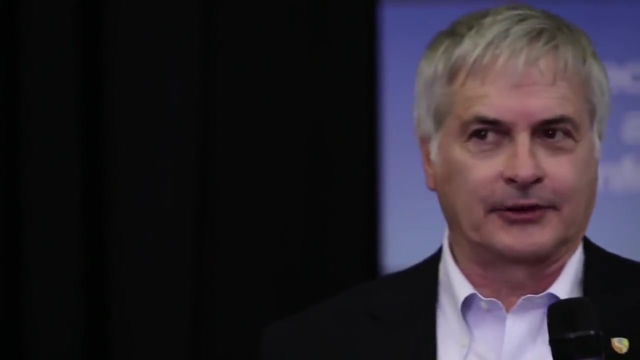 I just went down to LA about three days ago, whatever it was- to some production house down there to be taped for Animal Planet, And I don't know anything about animals except the ones I eat. but they want me on this thing because they want to ask me about the reptilians. 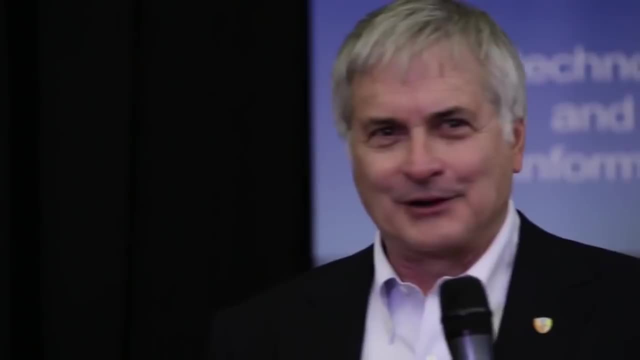 right. A lot of people believe the aliens are reptilians. I don't know why I said you know. if the aliens really are reptilians, why don't you just put them in a tank in the corner of the room and feed them lettuce? Reptiles in general are fairly placid because 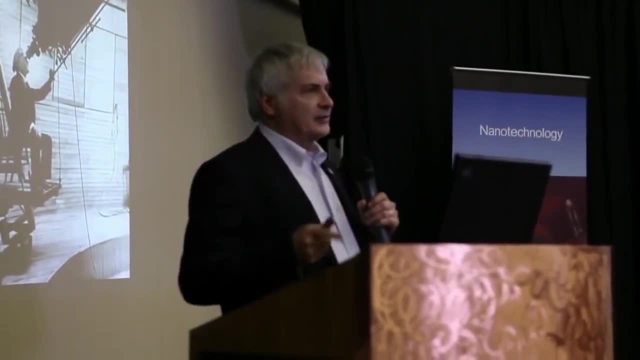 they're kind of cold-blooded and all I said why not? But they do ask. they say so what would the real ET be like? And the answer to that question is: we don't know the answer to that question. 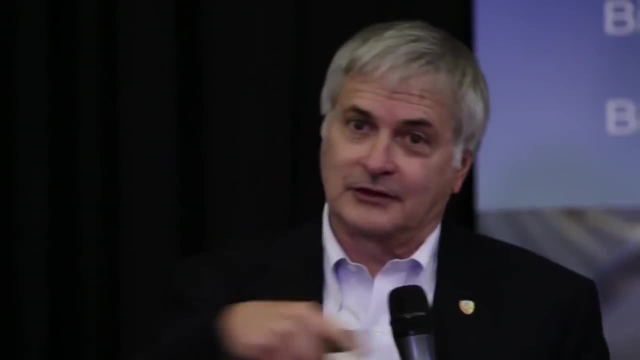 I mean, obviously we don't know the answer to that question, But I think it matters to think about this, And in fact this may be more germane to Singularity University than you're probably thinking at the moment. I'll get back to that. 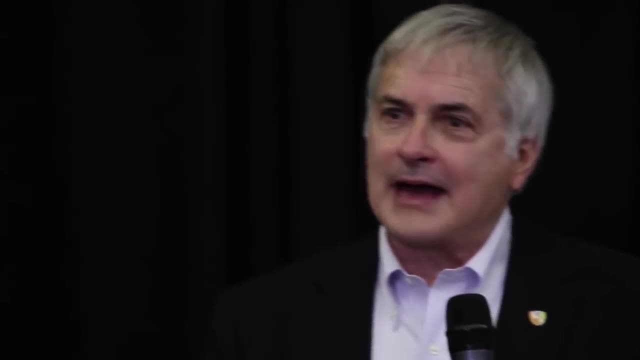 I think it matters. Here's an historical example about why it may matter what ET looks like. You can say: I don't care what he looks like, as long as he sends a signal that we can pick up. So what if he's green gray, has four eyes, six legs. 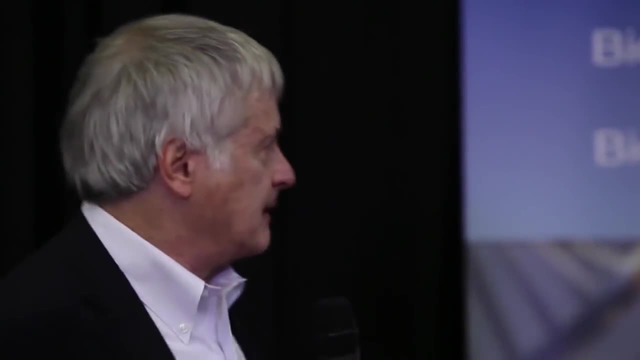 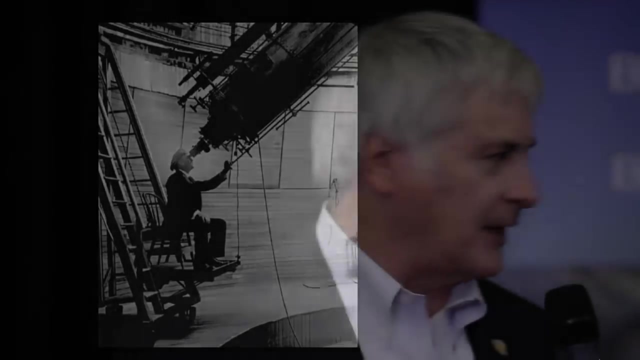 It doesn't matter. It might be interesting to know, but who cares? Here you see Percival Lowell in about 1900. Now, Percival Lowell was a Boston Brahmin or came out of a Boston Brahmin family. In any case, he went to Harvard. 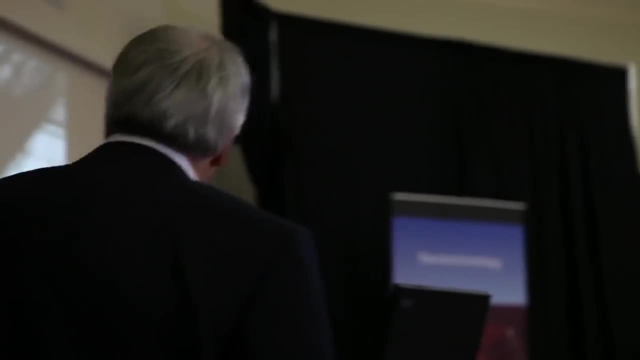 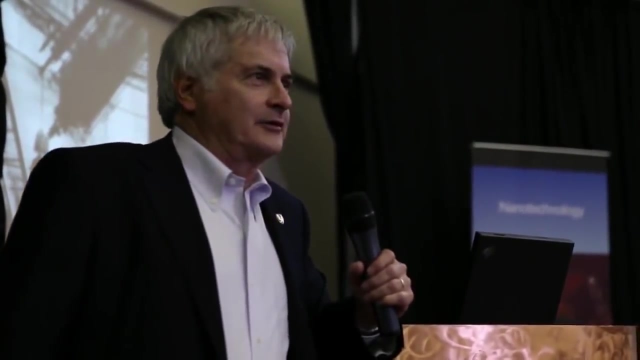 He was one of the best students Harvard ever had, But on the other hand, it was only Harvard, So in any case, he was interested. He studied mathematics, But he was interested in astronomy And rather than taking a job at a fourth-rate university trying to get tenure, he just said to heck with that. 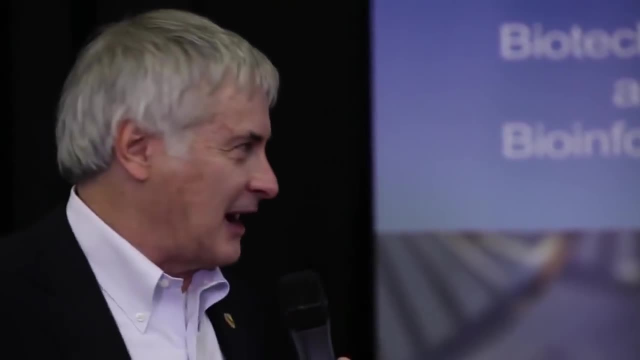 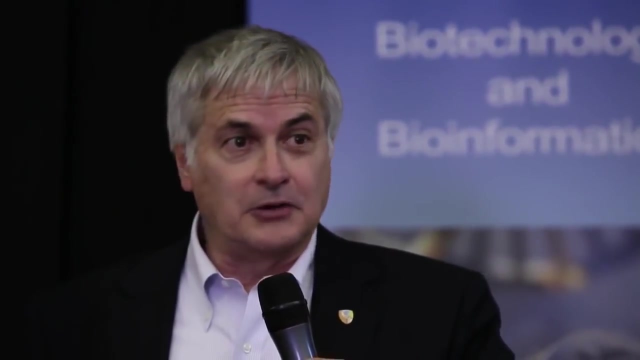 I got money And he just built his own observatory. He could hire him. He did. He actually sent people out to find out the best place to build an observatory, something that was, in fact, a new idea. Observatories previous to this were just built in the center of town, right where the university was, at least in Europe. 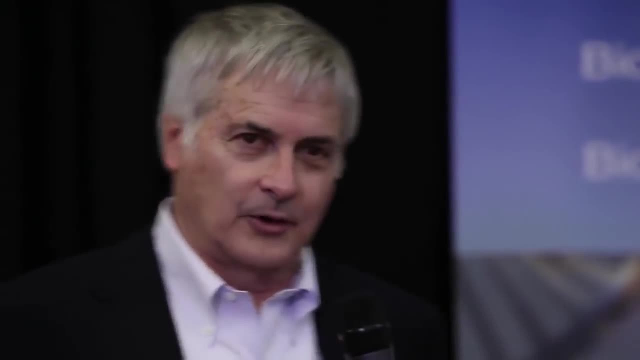 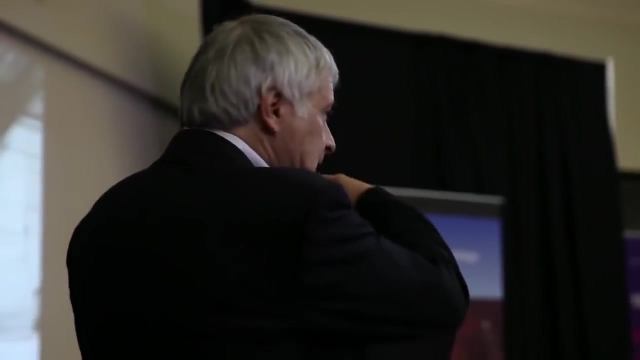 And that would work back then. But of course, you know, in 1888 or whatever it was, Edison, you know, invented a practical electric light bulb And that kind of downtown area is not so good for astronomy. He was told that the best place was somewhere in South America. 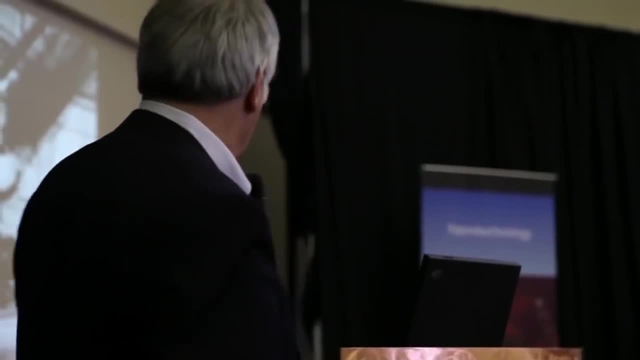 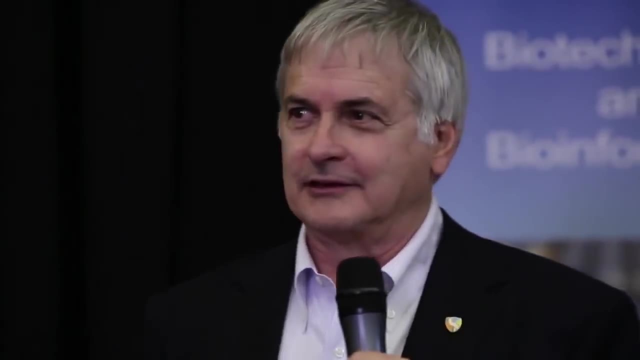 And he said: think again. I guess you know he was worried about the cuisine, I'm not sure. But in any case, thinking again turned up Flagstaff, So that's where he built his thing. He modestly named the observatory the Lowell Observatory. 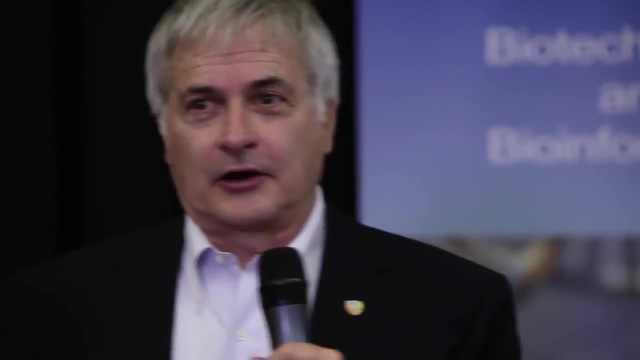 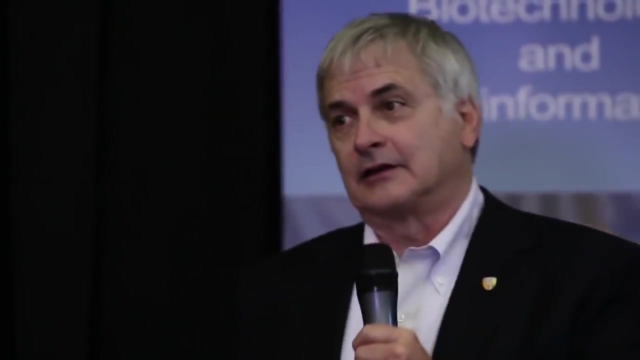 So here he is, dressed in a suit and a tie, sitting in a dark dome all night watching Mars, Because that's what you would do in 1900.. Okay, He was convinced by Italian astronomers who claim they saw straight lines criss-crossing the surface of our little ruddy buddy. 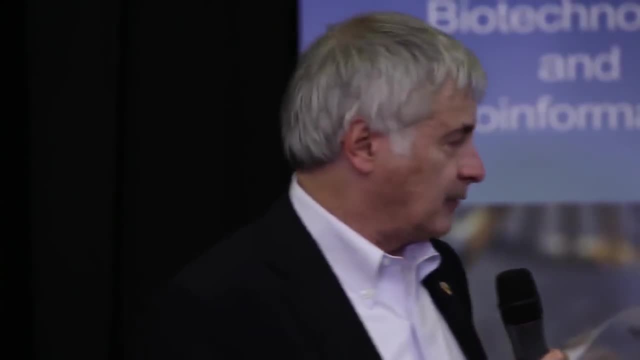 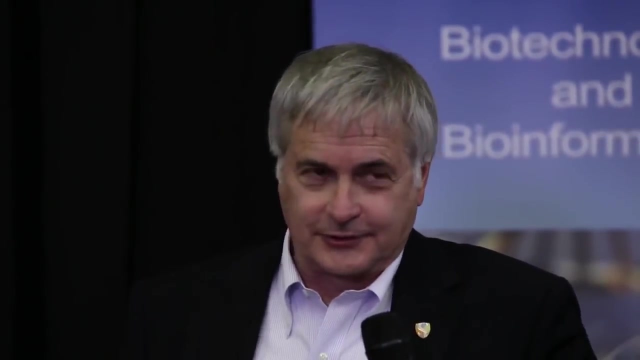 They called them canali, but that's because many of them spoke Italian And it was unclear whether they meant canali to be canals or whether they meant canali to be just grooves or geological features. The Italians themselves were very cagey in explaining what they meant. 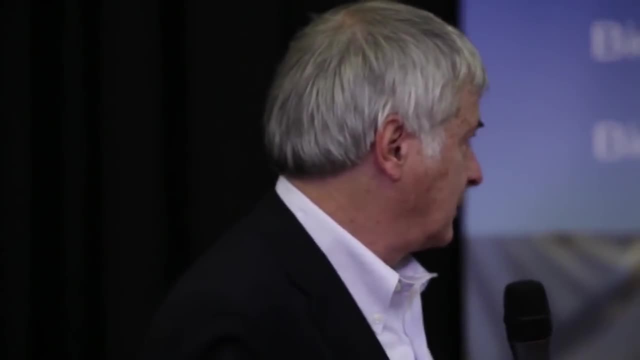 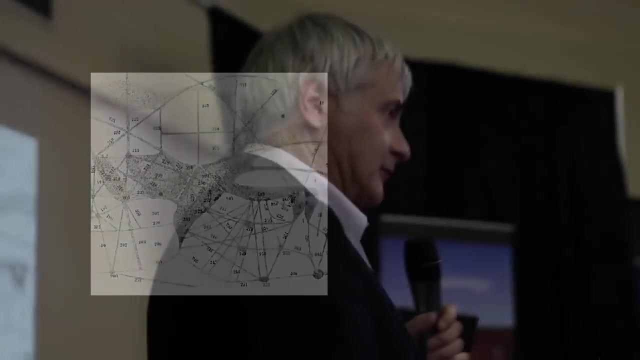 But Lowell was very sure that these were in fact canals constructed by thinking beings. And in fact here's some of his handiwork Now. he mapped hundreds of these canals. he gave them nice Latin names, just in case the Martians hadn't bothered. 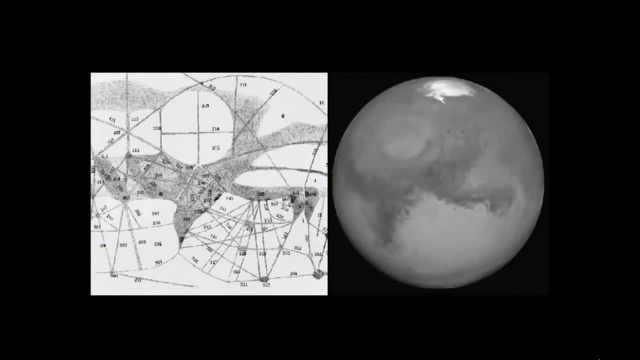 Just to show you what the real Mars looks like, here's a photo of Mars from a contemporary probe, actually of the same hemisphere, And you can see that the dark areas, the big dark areas, correlate fairly well. What don't correlate terribly well are all those straight lines. 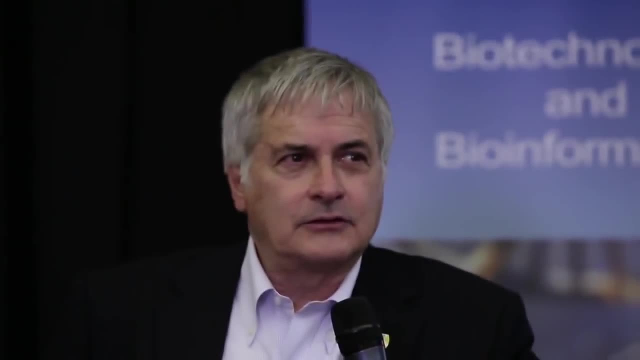 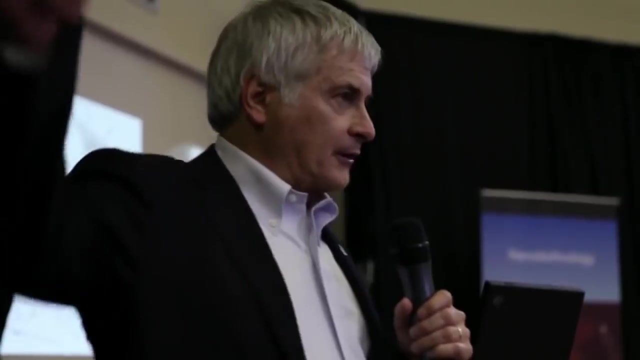 And the question was: well, what was happening here? And nobody's absolutely sure, but there seems to be a good explanation of what was going wrong with Lowell, Because Lowell was confronted with the fact that the people up here on Mount Hamilton, at Lick Observatory, they had a bigger telescope and they did not see these canals. 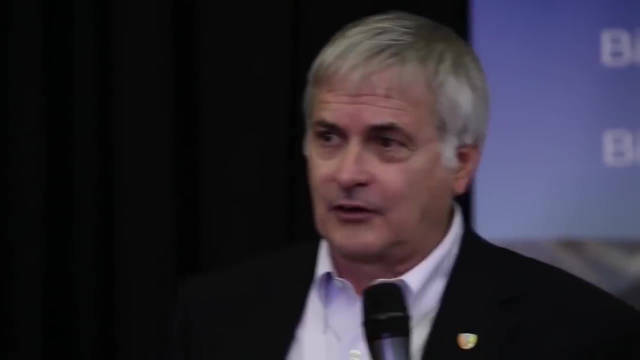 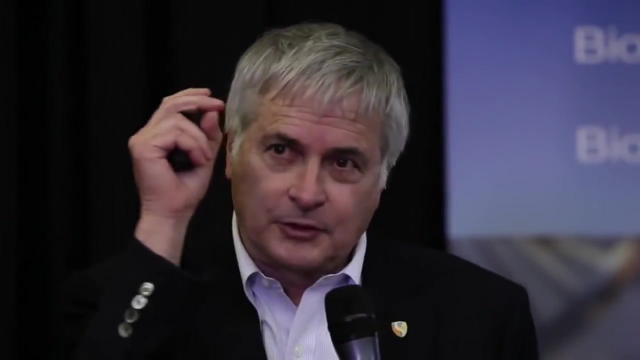 You might think, why didn't they just make photographs? and then you could settle the whole matter. But photography and astronomy was a very primitive art at that time And these were things you could only see when the atmosphere would clear for a fraction of a second, would stabilize, and then you could see fine detail. 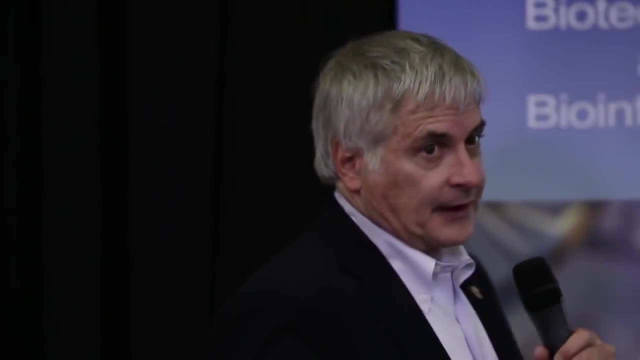 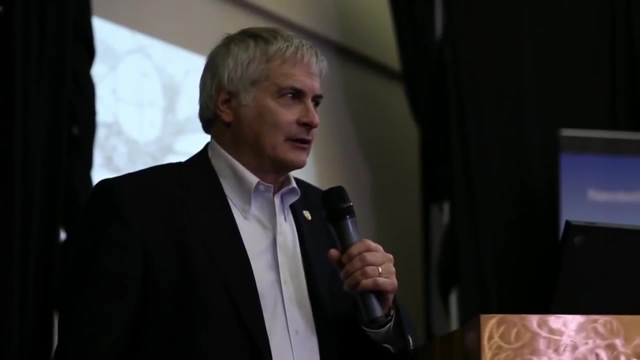 Your eye was better than photographs at this point, So they couldn't verify it that way. But the people at Lick Observatory said, look, we got a bigger scope than yours and we don't see these gosh darn canals And Lowell's retort. 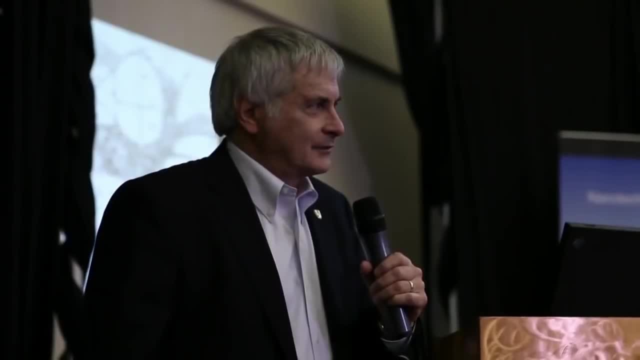 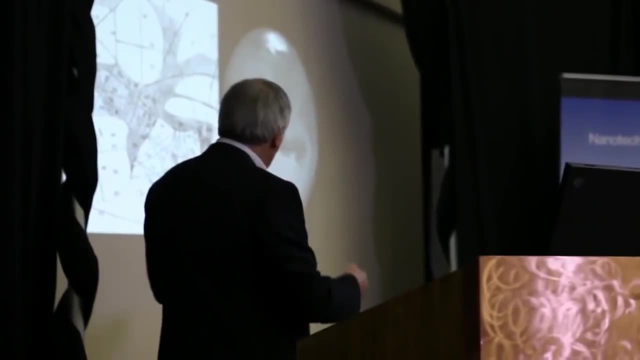 The retort to that was: you guys are not in Flagstaff, The atmosphere is better here. I don't know if anybody from Arizona they can tell me, But actually what was going on here? I mean here Contemporary Astronomy book there's. 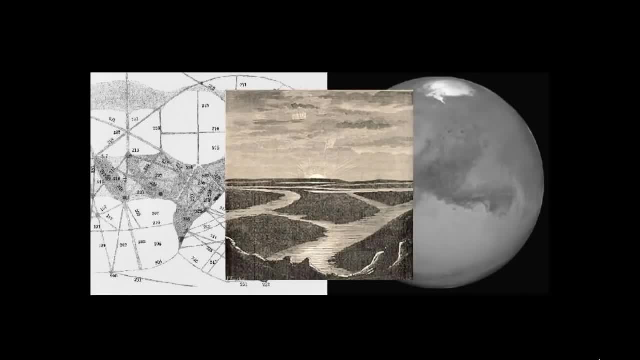 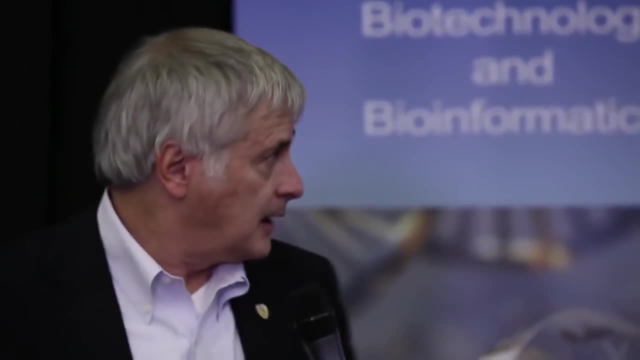 the surface of Mars as it was known to be a hundred years ago, or thought to be in any case, and it kind of looks like Venice, California. Lowell died in 1916 still believing that the canals were real, And indeed, not only did he believe it, but he wrote books about this, and he was a good 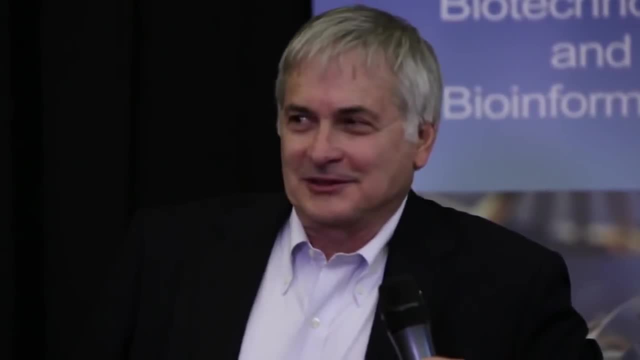 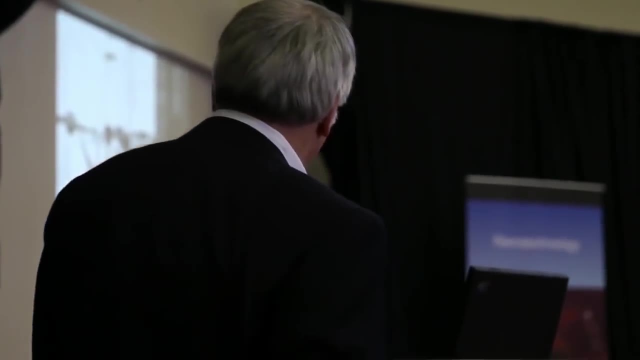 writer. He wrote everything else. He was, as they say, claimed to be the brightest student Harvard ever had. But this is an illustration from a book in 1908, and you used to see the Martians here at a cocktail party. You can tell the females because they wear bows and have long eyelashes, which is of 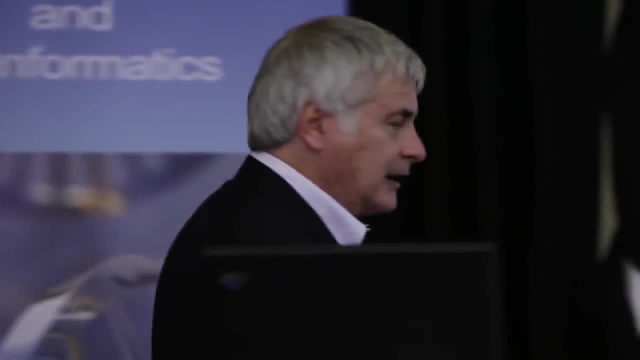 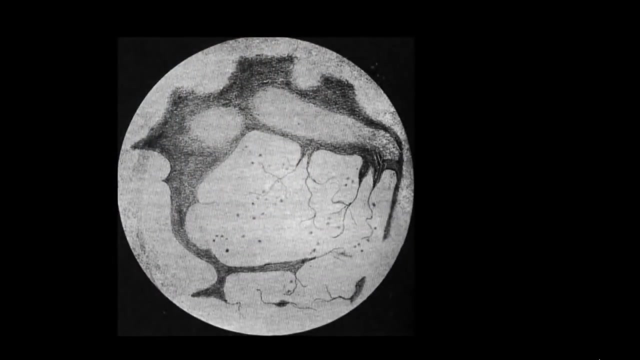 course, true for every species. Any case, here is the explanation, best they could tell, Because, as I say, by the time Lowell died in 1916, while he believed in this, almost nobody else did- There was a guy by the name of Edward Maunder. 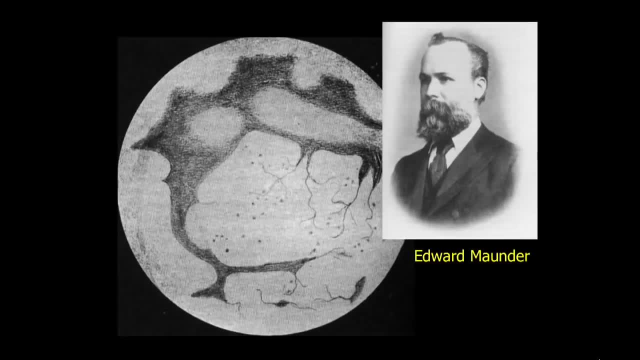 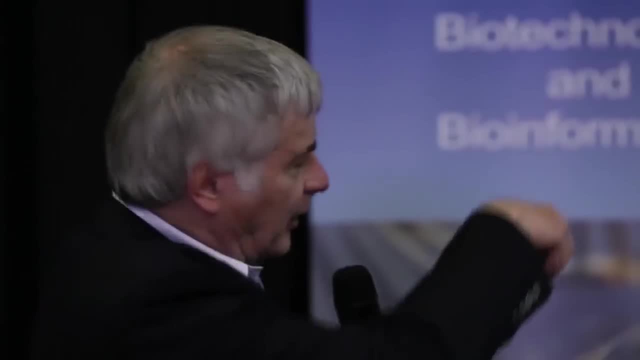 Here he is, Edward Maunder. He was- you may have heard of the Maunder Minimum in connection with ice ages and so forth. He was a clever sort of guy, But he did an experiment in which he made drawings of you know, sort of a hypothetical 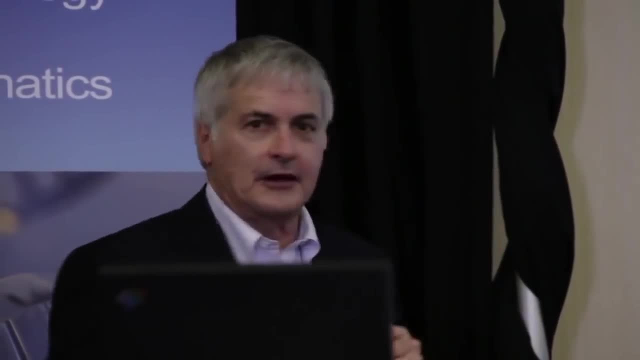 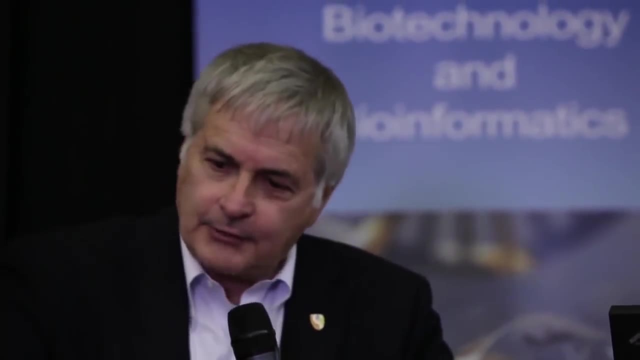 Mars- That's what you see here on the left- And he just put those in the front of a room full of school kids, school boys. Okay, These were. I think they were 11 years old, whatever, And of course they were at various distances depending on where they were sitting in the. 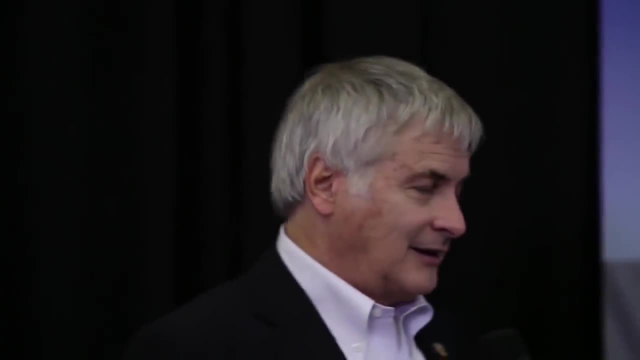 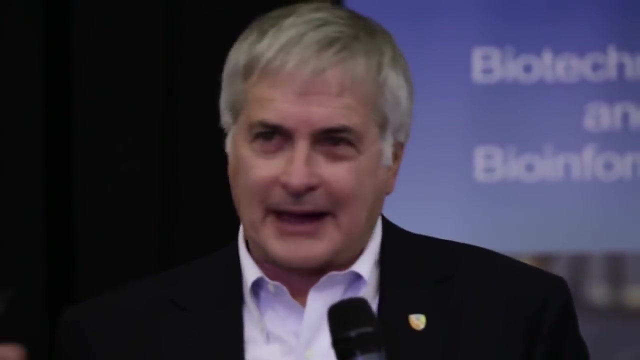 room And he just had them draw on a sheet of paper what they could see And the kids in the front of the classroom, The front of the class, would draw something very similar to you know what you see there. The kids in the back it was kind of you know. obviously they couldn't see all the 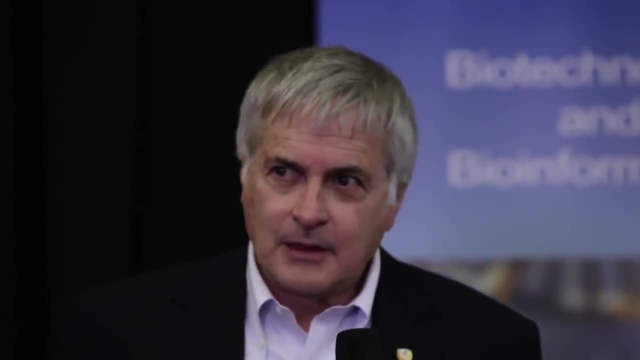 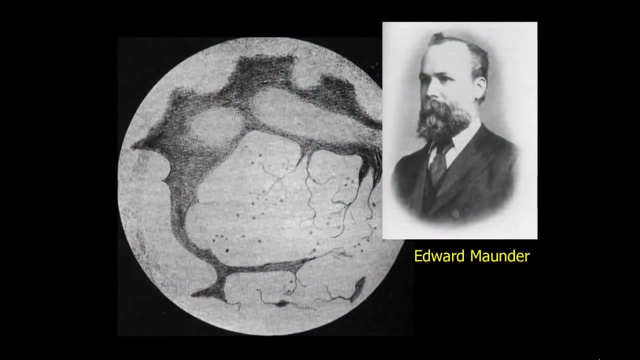 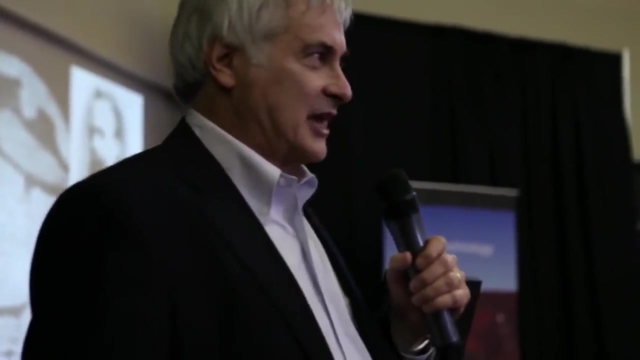 fine detail, But there was a certain distance somewhere in the middle where the boys would connect the dots Right. So that's telling you something about your retina and your brain, which likes to connect the dots. That helps you to find edges of images and you know that may help you. you know catch. 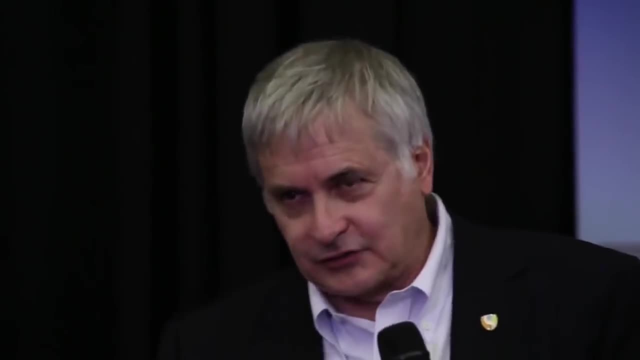 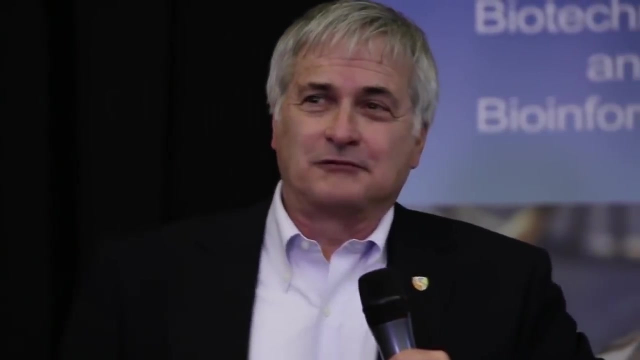 dinner Right. That's a survival value to see edges. So that's what was happening And that's what Maunder maintains was happening to Lowell. By the way, they did try this in Flagstaff. They got a beach ball, essentially drew some canals on it and put it, you know, down a. 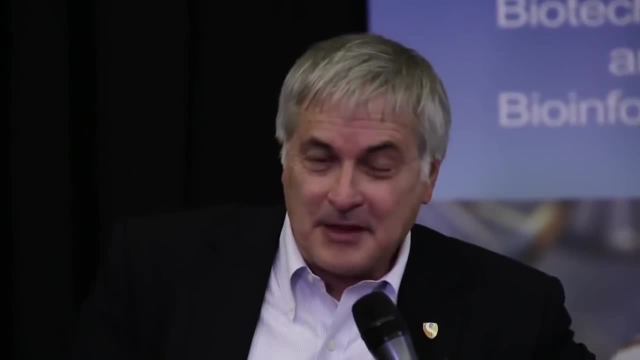 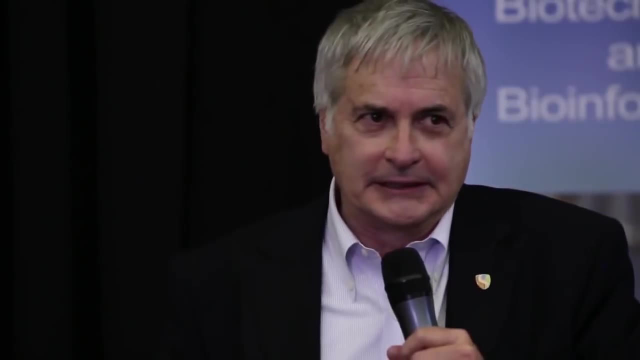 field. and then they set up a small terrestrial telescope right And they mimicked the optical situation of actually looking at Mars And they had Lowell look through that and try and map those canals, which he did, And he got them all wrong. 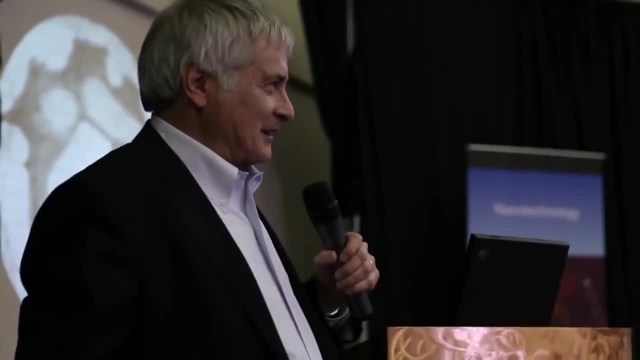 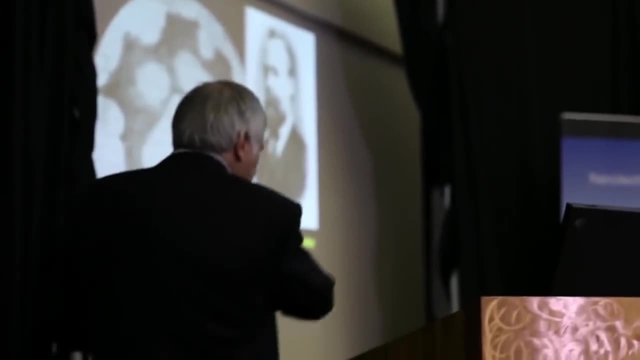 But you know, it was once more the, An illustration of the adage. An illustration of the adage that the boss may not always be right, but he is the boss, And he told them to stop those experiments Anyhow. so Maunder did it rather independently. 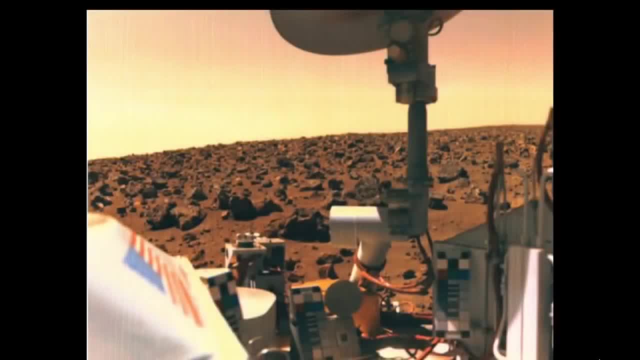 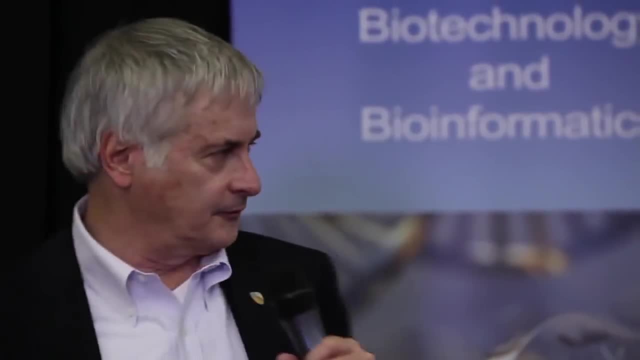 Now my point here is that when we finally went to Mars- of course these are the Viking lander photos- in the mid-1970s, and you have to remember the excitement when these guys plopped down onto the surface of, you know, the rusty, dusty surface of Mars, and they 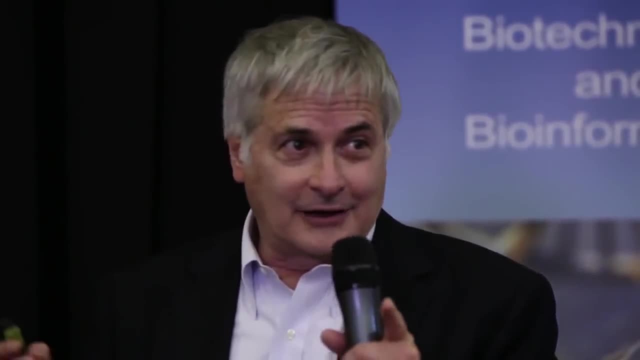 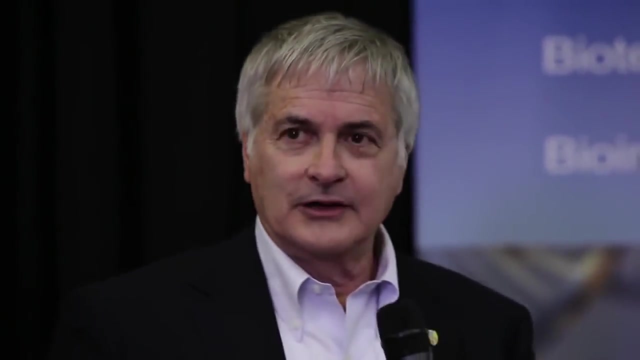 opened up their shutters. Many of you were not around for that, but it was a very exciting time because nobody knew what they were going to see. There might be little green guys waving you know, welcome to Mars. It could have been lichen. 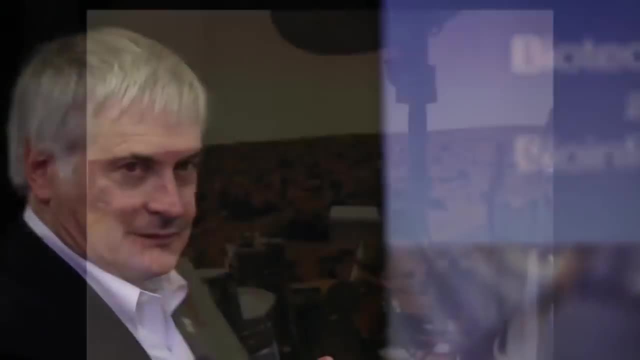 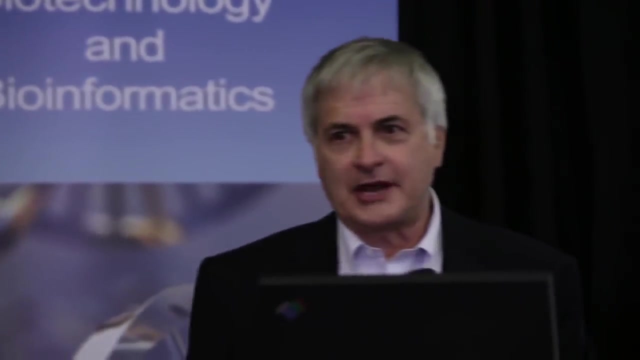 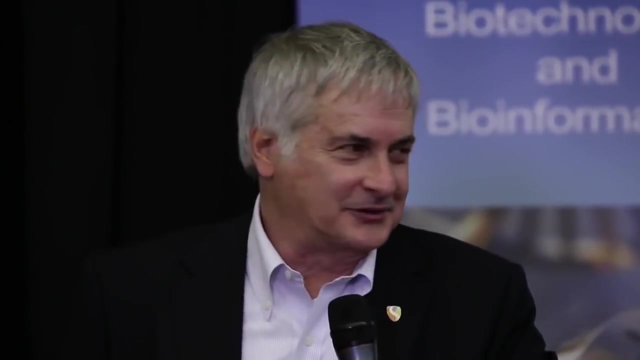 It could have been something And it was that okay, which, as it turns out, is dead, Jim. right Now Norm Horowitz down at JPL at the time, who was part of the Viking biology team, said that well, he realized the public and everybody else was kind of disappointed. 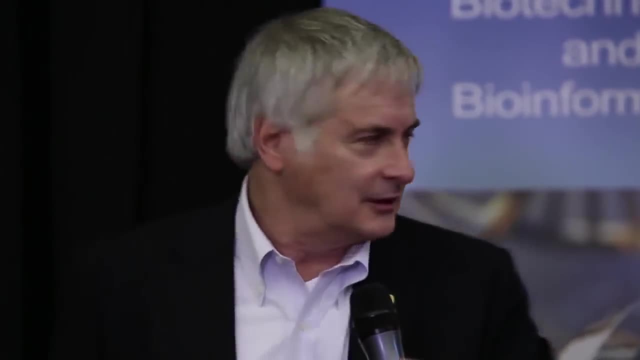 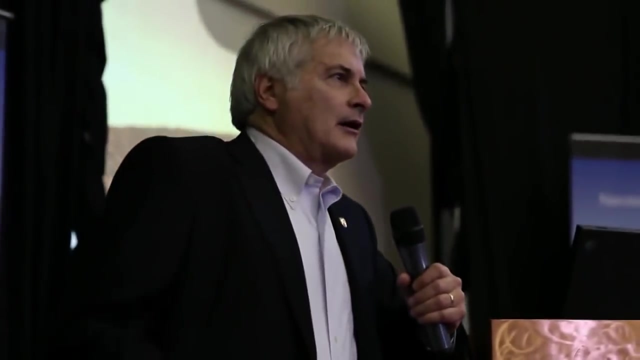 And he said: well, it could be that there's life on Mars that looks like rocks, but more likely, what this is is rocks. We know they're rocks. Okay, So now the point is that that sounds bad, but of course, today we're you know, sanguine. 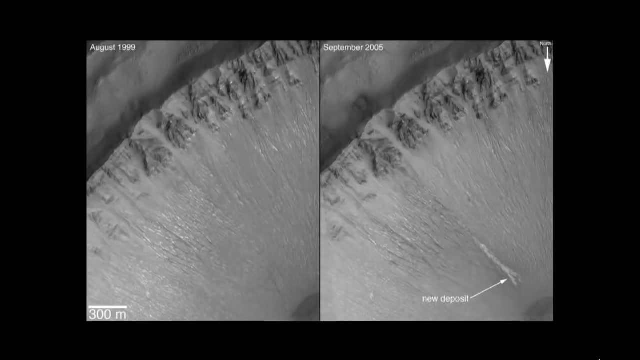 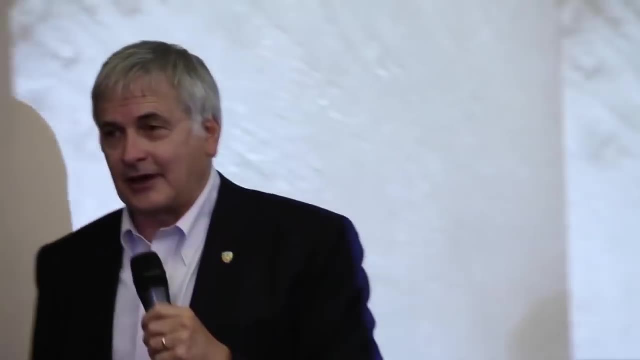 again about the possibility of Martians, mostly from results like this, where you see an orbiter photo of a crater here and here you see it a couple of years later and you see that streak there. Something is obviously leached out of the side of the crater wall. run down the side. 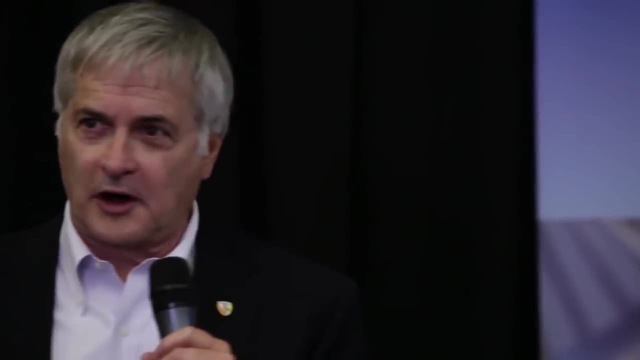 of that crater and it could be Brylcreem, could be talcum powder. Most likely it's just water. Okay, And that suggests that if you really want to find life on Mars, you're going to have to do something. 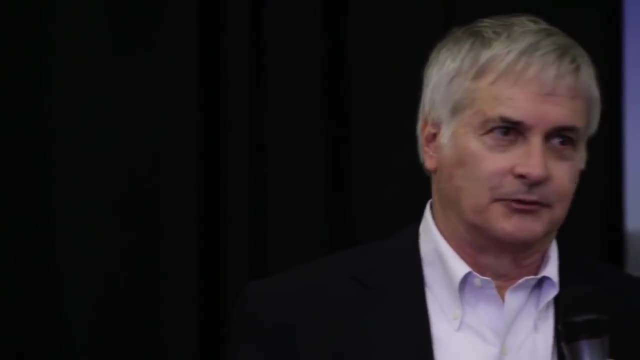 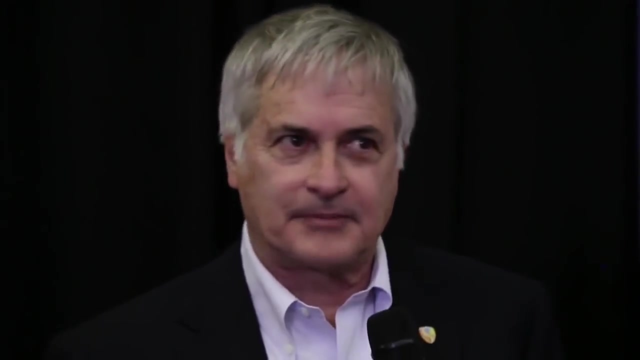 If you really want to find life on Mars, the thing to do is send Bruce Willis to Mars with a bunch of roughnecks and have them drill down a couple of hundred feet until they find the liquid aquifers that we think may exist down there, and pull up that muck and look. 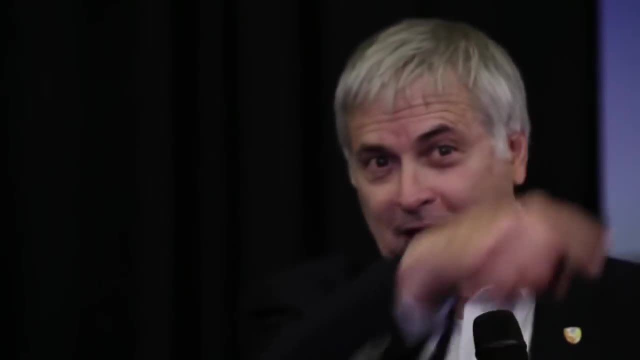 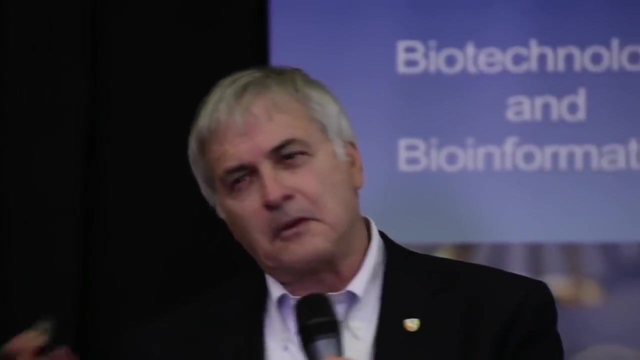 at it under a microscope. Because if you do that outside here, if you do a whole two miles deep and pull up that muck, you'll find microscopic life as well. So that's the thing Now. my point in all this is only that it makes a difference how you picture the Martians. 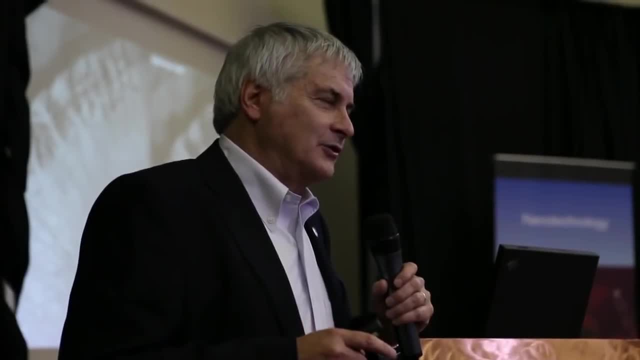 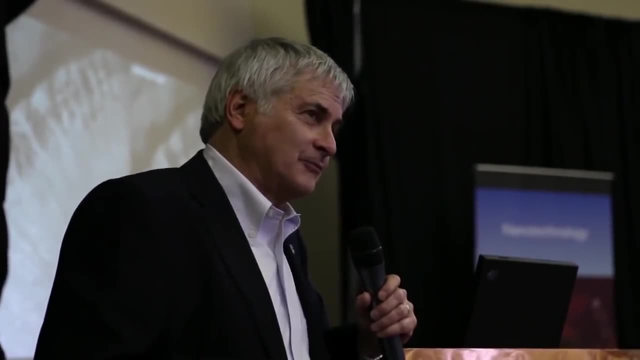 right, Because in 1900, the way to find Martians- Okay, It was to use a nine inch refracting telescope in Flagstaff, Arizona. Today, the way you hope to find Martians is send some sort of robotic drilling rig to. 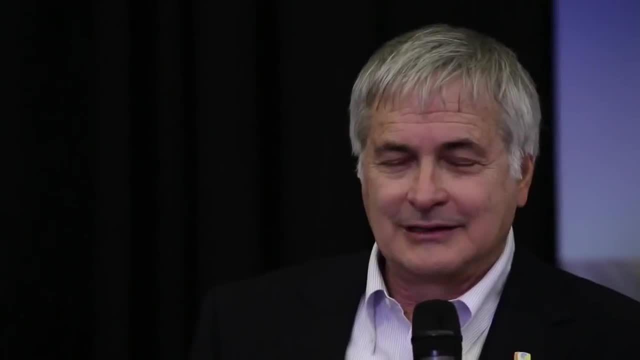 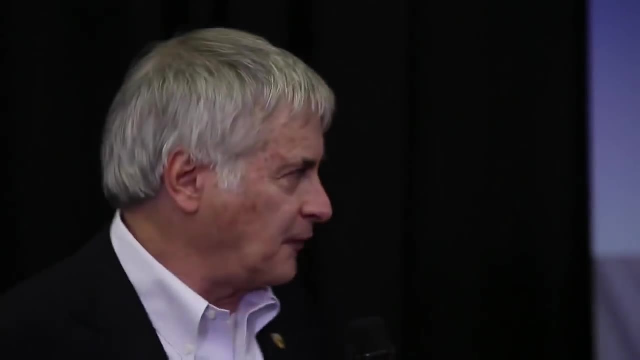 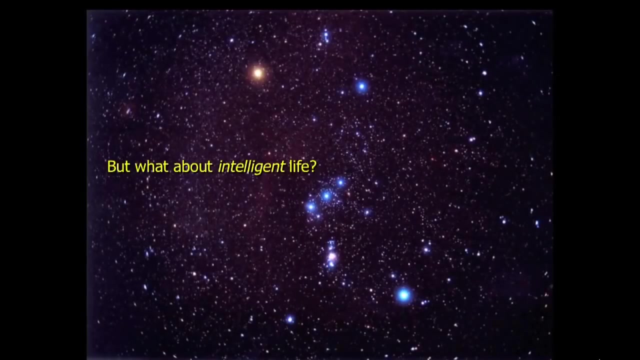 Mars and go down a couple of hundred feet and have a microscope on board. So your image of what the aliens might be like will affect your strategy for finding them. So I'll get back to that Now. intelligent life. If you were to grab the next, you know 10 scientists off the streets here. I don't recommend. 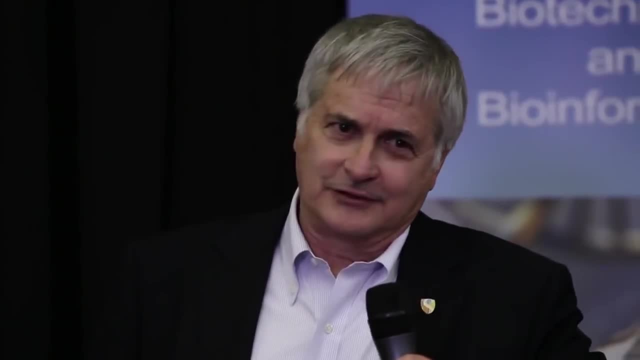 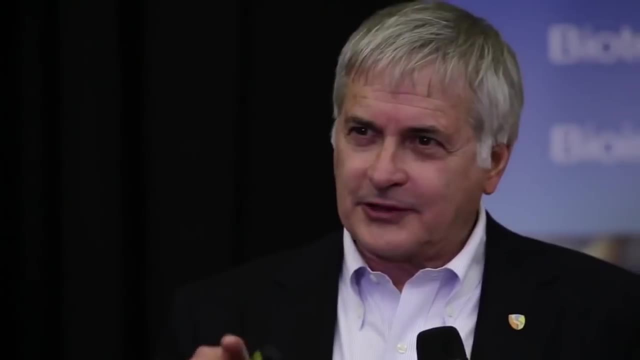 it. If you were to do it and ask them: do you think there's life in space? I suspect nine out of 10 of them would say yeah. well, that sounds reasonable to me, right? But if you ask about intelligent life, the percentage drops a little bit. 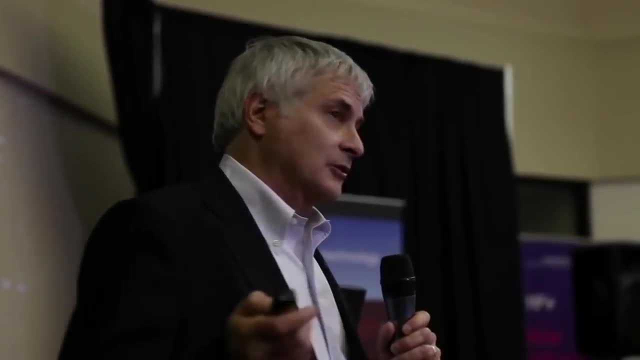 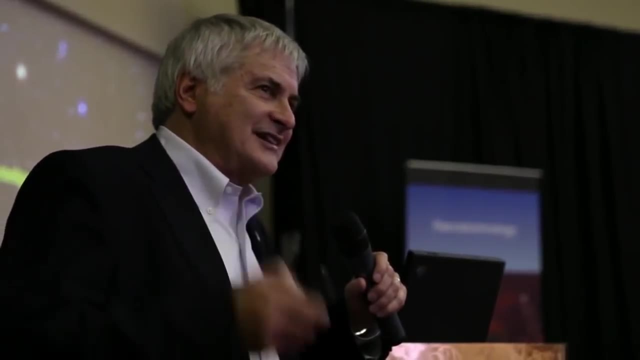 A lot of biologists. evolutionary biologists- and this includes Steven Jay Gould, you know he would occasionally write about this- were of the opinion that you know, all you had to do was change a little bit of our evolutionary history and you wouldn't be sitting here. 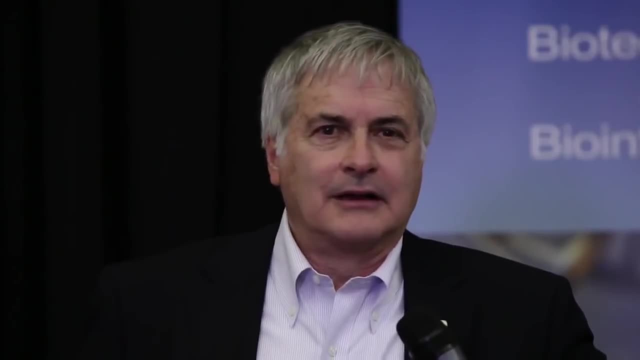 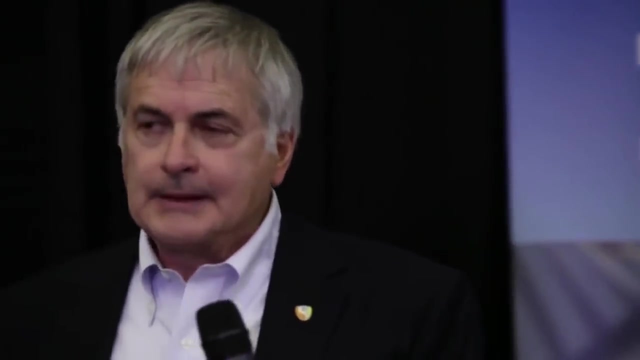 right. For example, a very obvious example: 65 million years ago, a rock slams into the Yucatan, wipes out the dinos and two-thirds, three-quarters of everything else walking around the land. Now, if that rocket arrived 10 hours earlier, it would have missed the earth and there'd. 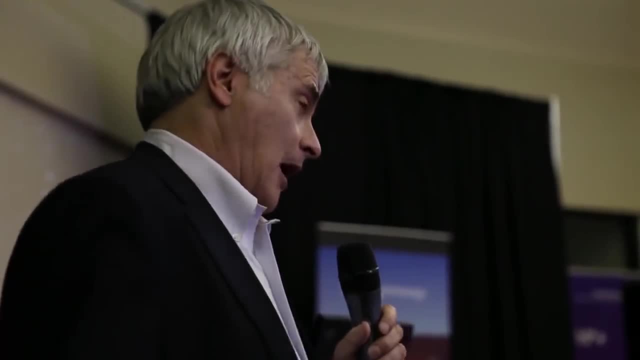 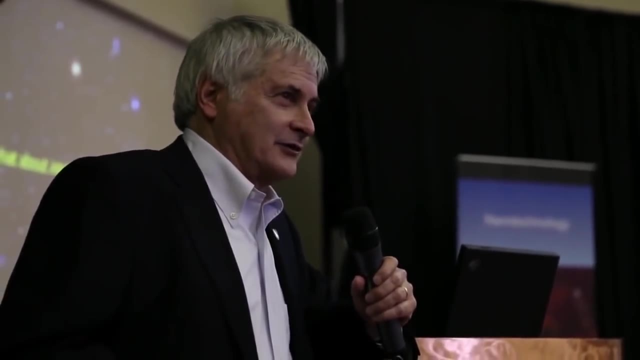 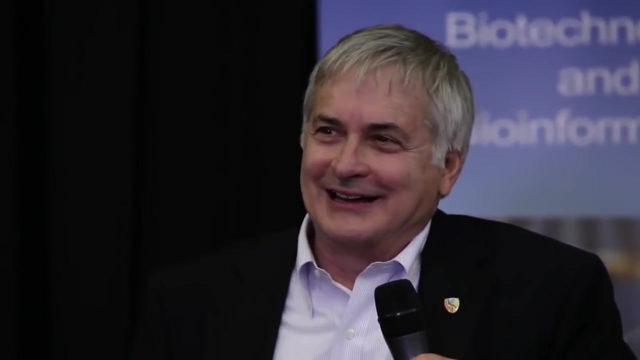 be dinosaurs in Mountain View and you could say, well, yeah, but the dinosaurs would have gotten smart. And there are people who think that that might have happened. I mean evolutionary biologists, not just advocates for dinosaur intelligence, And maybe it would, but I did ask once Niles Eldridge, who's an evolutionary biologist. 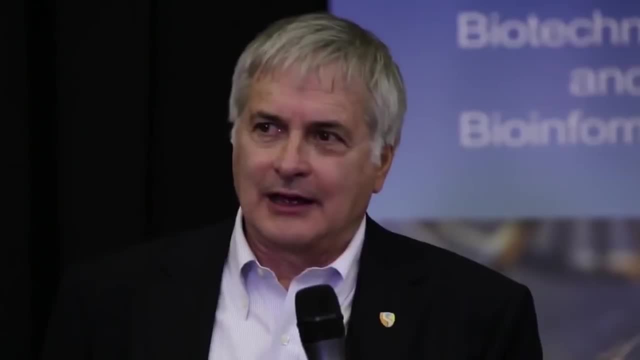 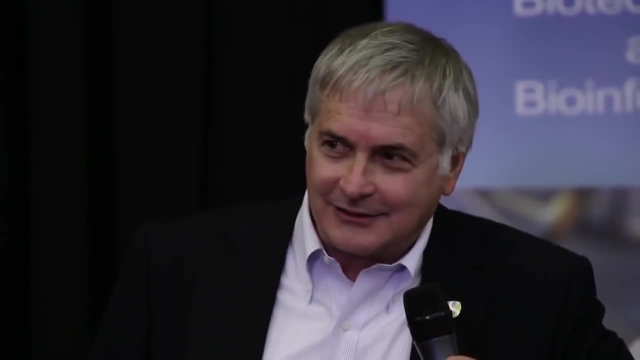 at the American Museum of Natural History. I asked him that question: would the dinos have gotten smart? And he said: well, he said, look, the dinos had 150 million years to get smart and didn't. What would another 65 million years have done for them? right? 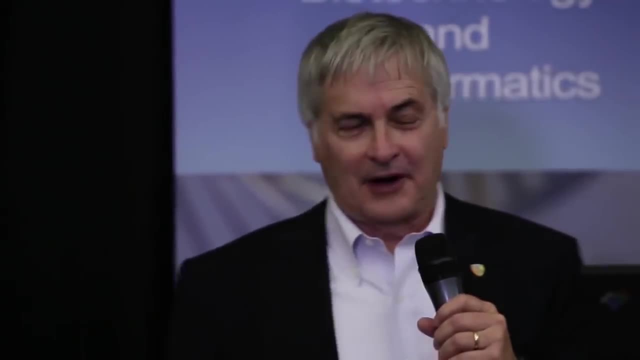 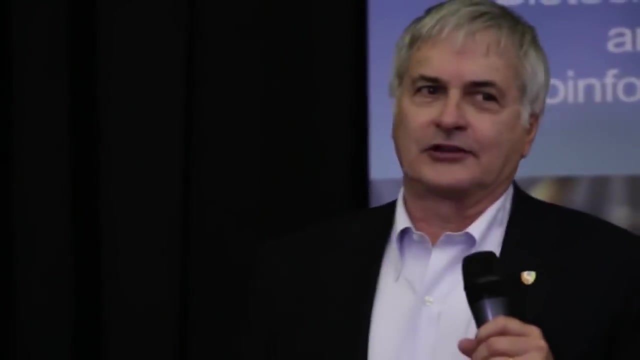 Now you know that argument only goes so far. He could have said the same thing about, you know, primates, and they did get smart eventually, but any case. So this is a very controversial thing. This is highly contentious. Just because I give you a million worlds with life, will any of them have anything as clever? 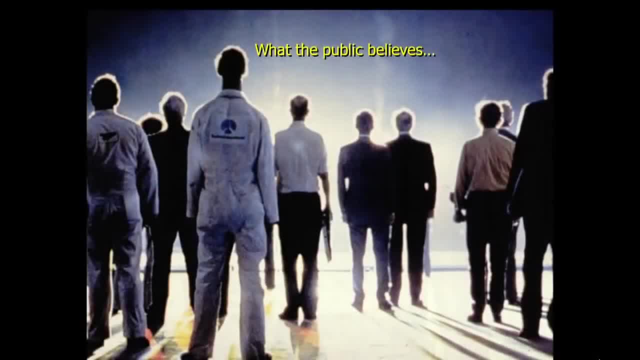 as the average resident of Sunnyvale And we don't know the answer. now The public believes that yeah, it's happening. I'm not going to. yeah, never mind all this. Maybe I won't, Maybe I'll say something about this. 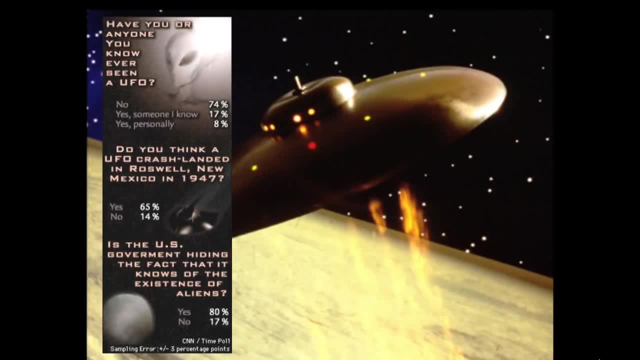 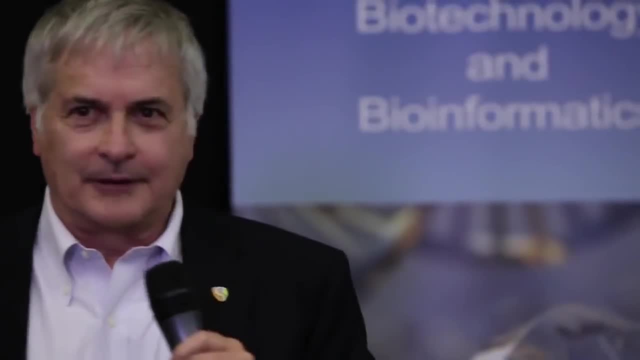 I should point this out, because I don't know how many of you think that the aliens are not only out there, but they're here. right That they're. what are they? 19 species of greys or something like that, right. 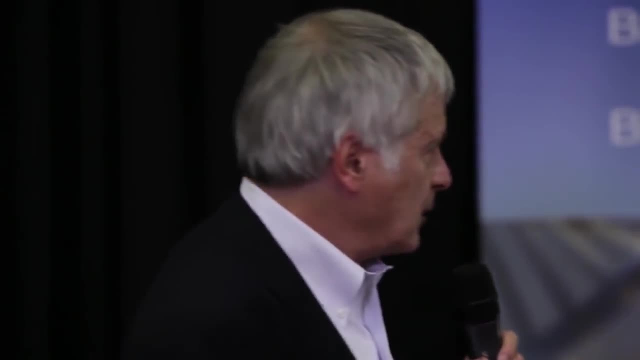 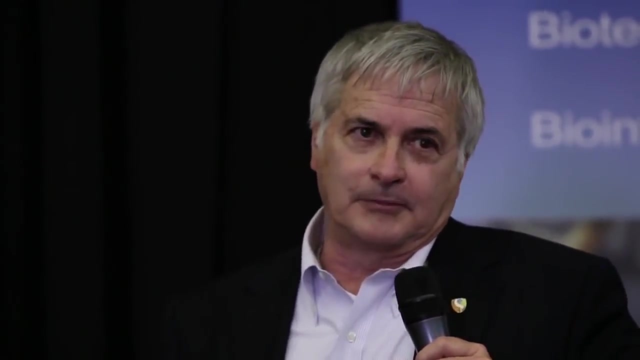 Buzzing the countryside, occasionally abducting you for experiments your mom wouldn't approve of. Well, that's not a fringe belief, right? One third of the American public believes that's true And, by the way, one third of the public of Australia, Japan and Europe does as well. 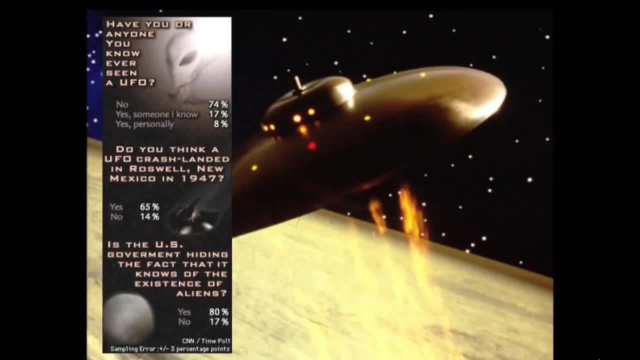 In fact, here's the results of a CNN Time poll made in 2002.. Do you think a UFO crash landed in Roswell, New Mexico, in 1947?? Sixty-five percent of Americans say yes, Right, The aliens. the aliens have come hundreds of light years to enjoy some Tex-Mex cuisine. 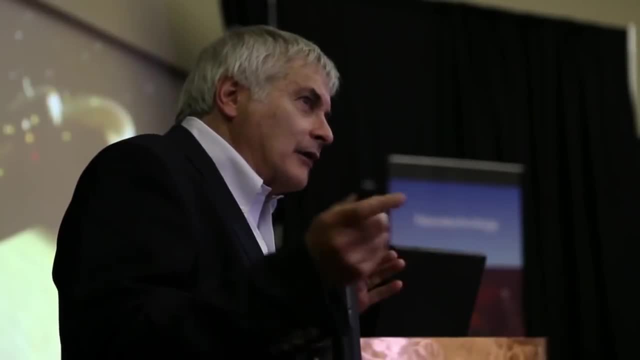 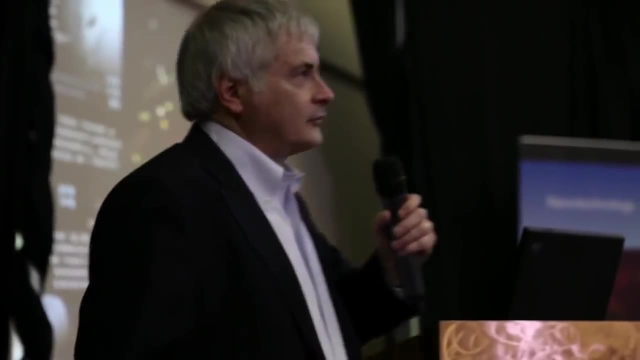 I mean, I don't know why they're visiting New Mexico, but anyhow, And hundreds of light years, and then the last 50 feet, they make a navigation error and crash into the dirt. Now- Certainly could happen. but I mean that's analogous to you driving across the country. 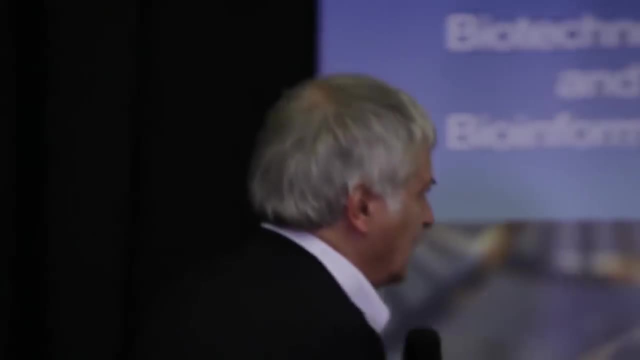 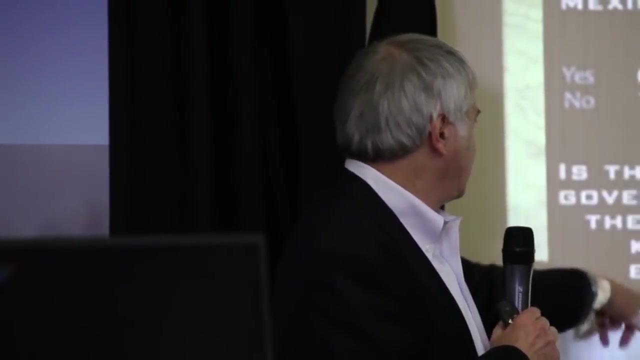 and then tolling your car on the driveway garage door. actually, All right, all right, good to happen, But 65 percent. see that's not .65, but that's 65 percent. Is the US government hiding the fact that it knows of the existence of aliens? 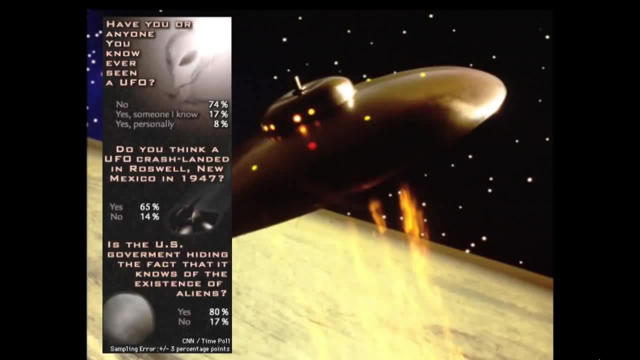 Eighty percent of Americans say yes. The same government that runs the IRS but nonetheless is able to keep this quiet. Now, even if you like to think that the feds are keeping the aliens, they're freeze-drying, strapping them. They're stacked up at Area 51 or wherever you like. Every other country has to be doing this too, unless you think that the aliens only want to visit America, right? So I deal with this every day. Every day, I get phone calls and emails from people who are having difficulties with aliens. 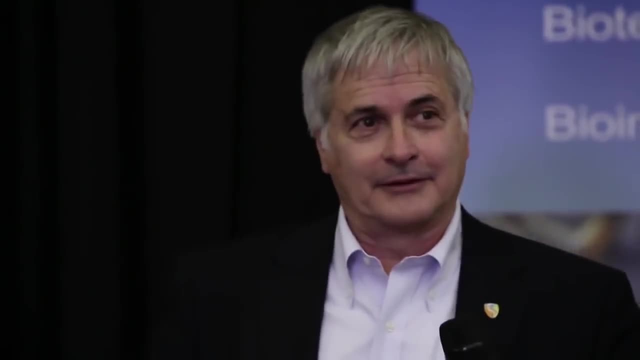 in their personal lives And I can assure you that the people who call me up, I mean they're not. Some are not cases. It was a guy yesterday who called from North Miami to say he's in touch with the Lord of the Rings. 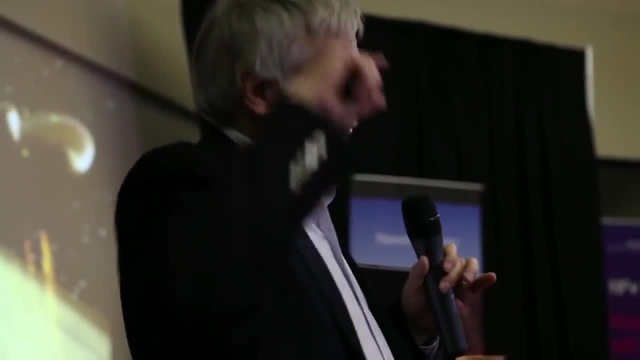 But- He sent a stranger on the phone that he didn't email. I mean they're not. Some are not cases. It was a guy yesterday who called from North Miami to say he's in touch with the Lord of the Rings. But most of the people that call me up I mean they've seen something. 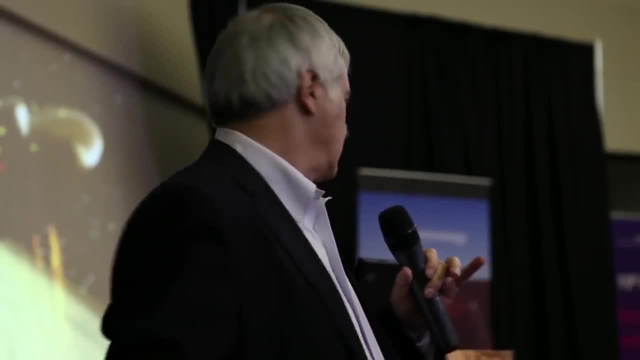 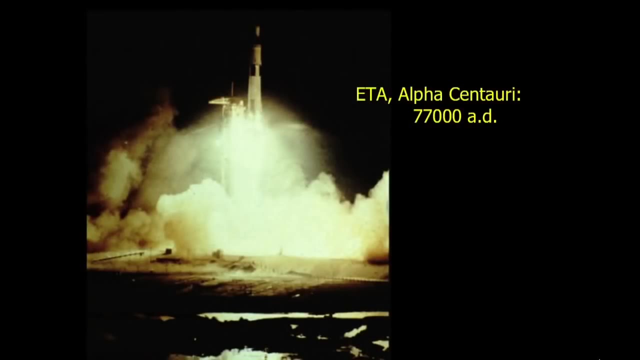 And they're just not very good at figuring out what that something might be Okay. Part of the reason why I don't think they're here is Interstellar travel's rather difficult. Our rockets go seven, eight miles a second. So if you want to go to Alpha Centauri and visit the Navi, for example, to buy some unobtainium, That number's slightly wrong. I think I worked that out again. It's like 110,000 years one-way trip. Okay, So that's a long time to sit there. You know You're eating bad food off your lap. But you can build faster rockets, of course. But the problem with faster rockets is they take a lot of energy. If you want to go half the speed of light, so you get there in 10 years, you can work it out. Just use high school physics. Forget relativity. Just use high school physics. Figure out the amount of energy required, And it's a really big pile of coal. I mean, it's the amount of energy that the United States burns up in a couple hundred years at the current rate. So it's very energetically intensive. You say, well, we'll just use matter-antimatter drive like they do in Star Trek. And well, if you can figure out how to store the ammortizer Or the antimatter. 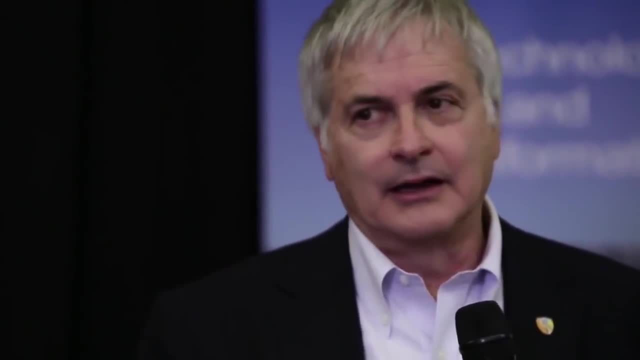 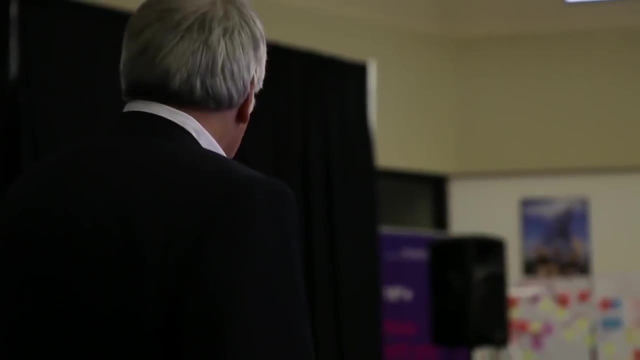 Not to mention making it. I mean, I guess you could, Because that works. But there are other problems. You know, when you're going at half the speed of light through the galaxy on your way to visit the Navi, you know all the interstellar dust and gas is slamming into the front of. your rocket producing high, you know, very hard radiation that zips through the rocket and you know, essentially kills you right away. But hey, You know these are all technical problems, So maybe you can solve them, But it's not easy. 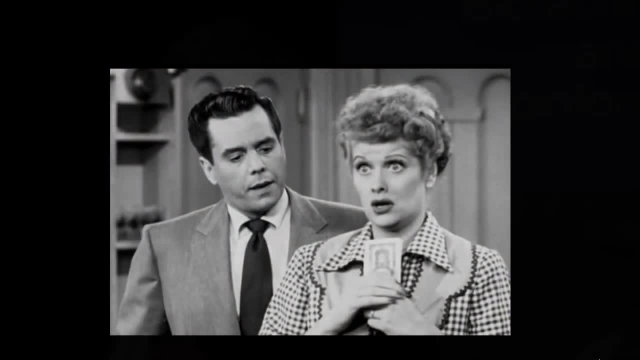 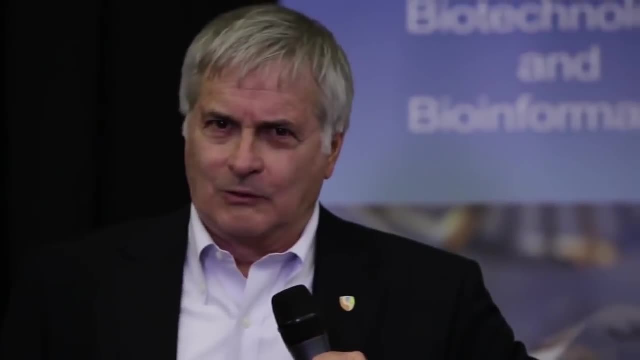 Now here's another reason. I just mentioned this For the heck of it. This is like this whole talk. There's another reason why I don't think we're being visited. The question I always ask people who think we're being visited is: why? now? 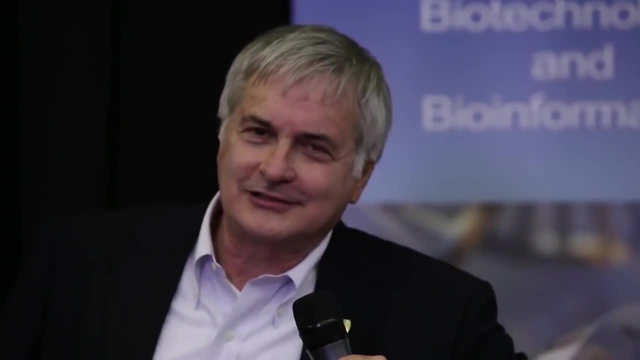 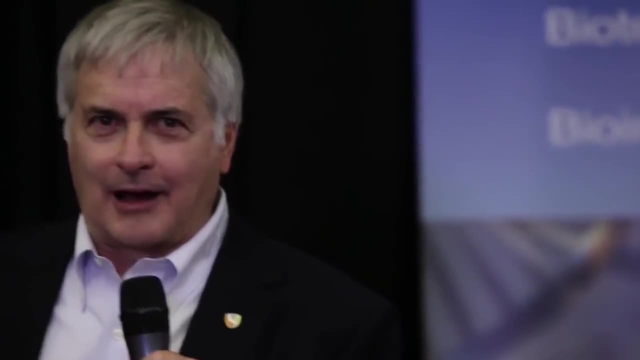 Right, Why now? Why are the aliens here just in time to improve your social life by abducting you for these salacious experiments? Right, Why is that happening now? I mean, you know the Earth's been here for four and a half billion years. 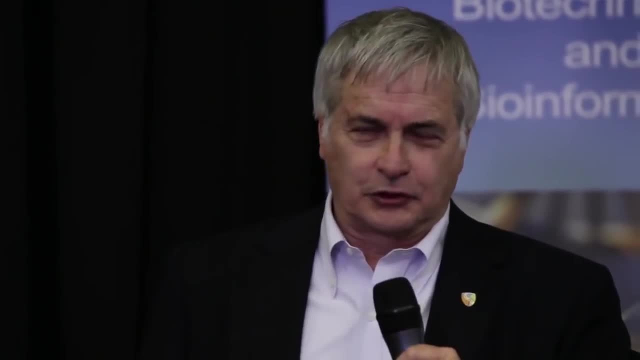 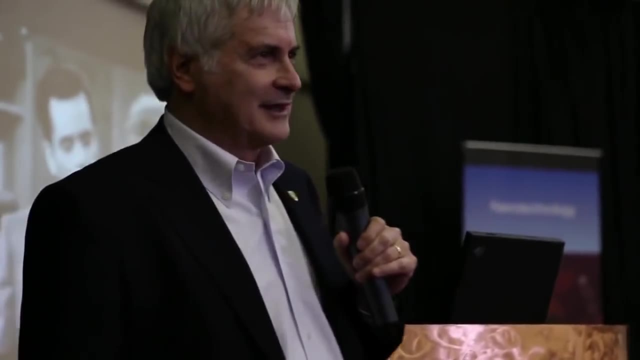 And the usual answer you get is: well, look, The aliens are disturbed by our messing up the environment, Or they're unhappy about the fact that we've got nuclear weapons and stuff like that, That they have some moral interest in us. Now that's alien sociology. 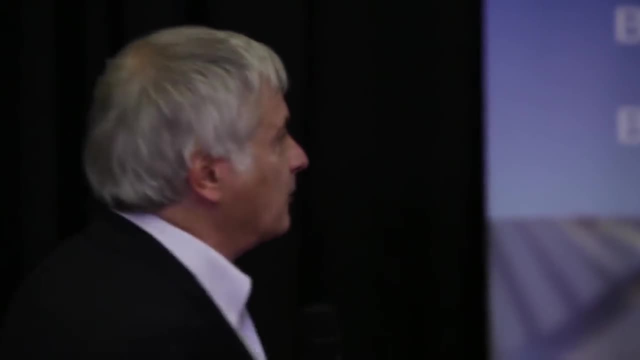 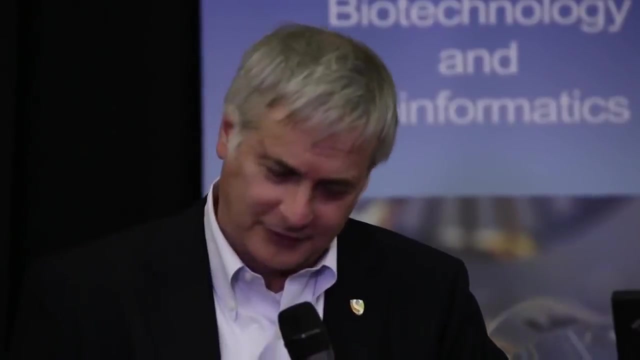 And the data set for alien sociology is very sparse, So we don't really know that, And it's you know. I say I don't go in the backyard and separate the ants. You guys have been warring for years And I just don't like it. 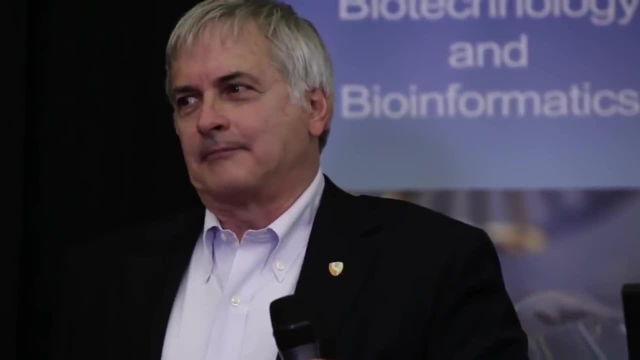 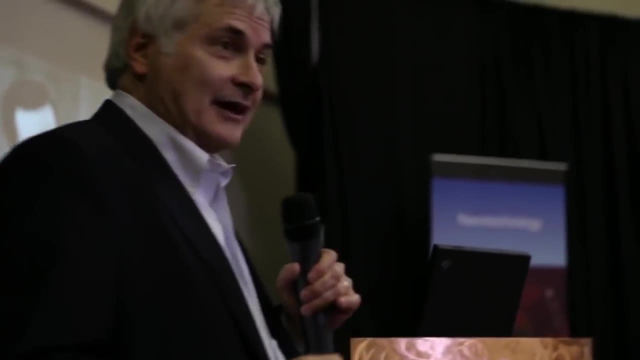 I don't bother with that, So I don't know. I mean, but that's all you know. supposition: One doesn't really know if the extraterrestrials would have any interest in that, But the point is that that argument doesn't matter because they don't know about it. 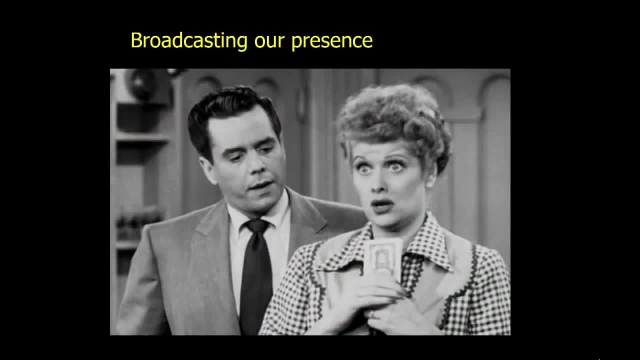 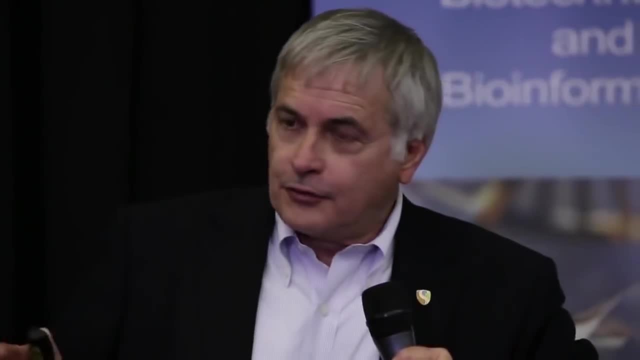 Here's I Love Lucy. First episode was the early 1950s, So that signals like 60 light years out into space. So any aliens that are coming here now because they don't like Fred Mertz's jokes or something, those guys can't be more than 30 light years away because they can't get here faster than the speed of light. 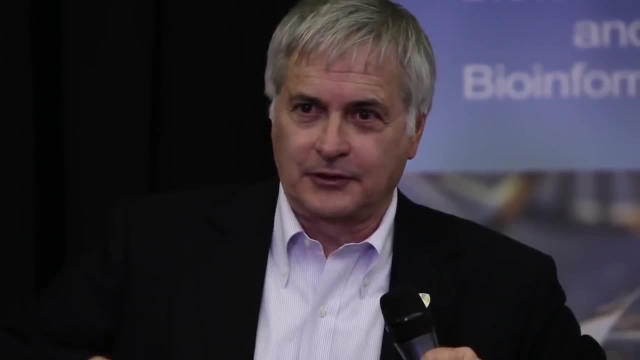 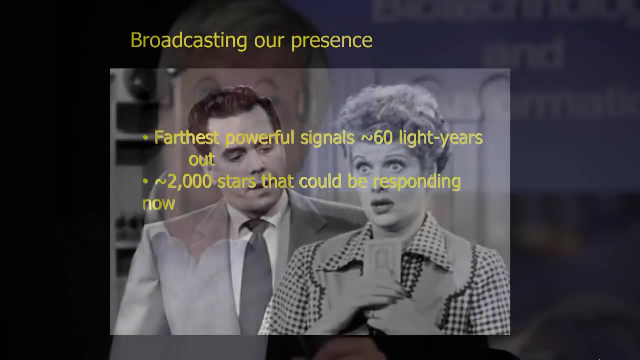 Right. So it takes 30 years for the signal to get there, Another 30 years for them to respond. come back here. That means that they're only 2,000 years away, But there are only 2,000 star systems that have been exposed to our radar, to our television, to our FM radio. 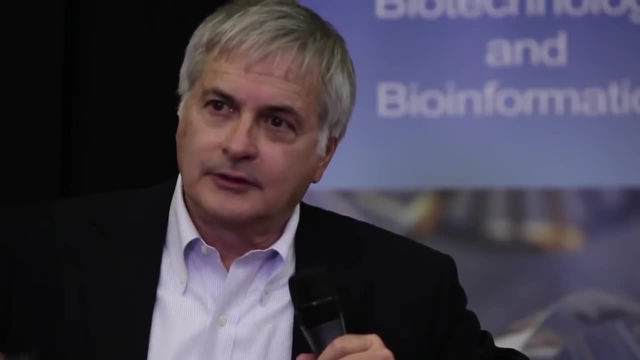 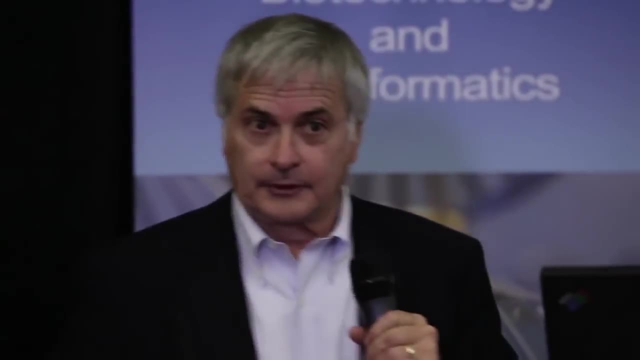 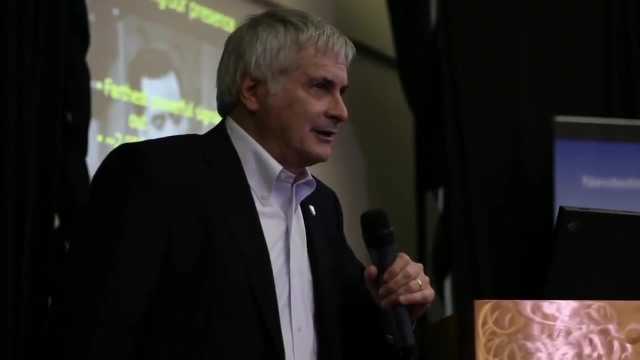 all of which leak off the Earth. Only a couple of thousand stars that are, you know, only half that distance out, so that they've had time to come here and haul you out of your bedroom. That's a very small number. The chances that there's any alien civilization in the nearest couple of thousand stars strikes me as very small. 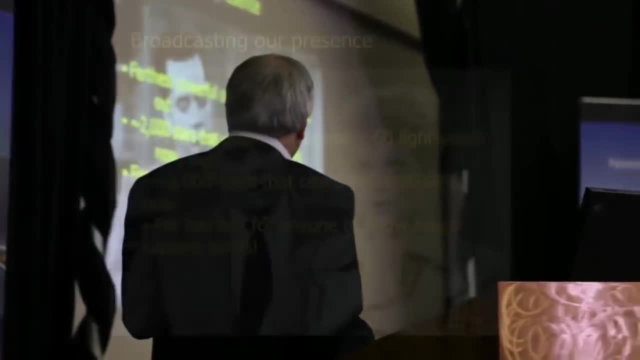 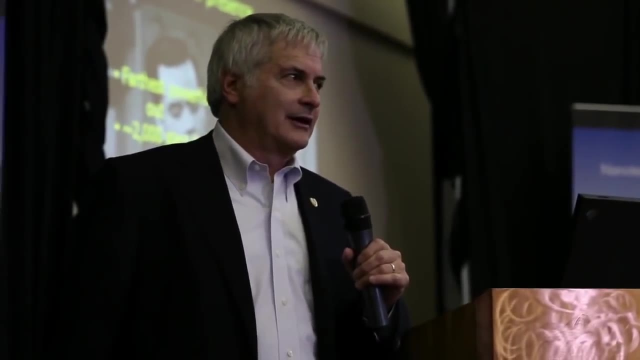 So this doesn't work for me. I think it's safe to say that nobody knows. Nobody knows that Homo sapiens exists, Except residents of this planet. Nobody knows that. They know the Earth has life because they could find the oxygen in our atmosphere. 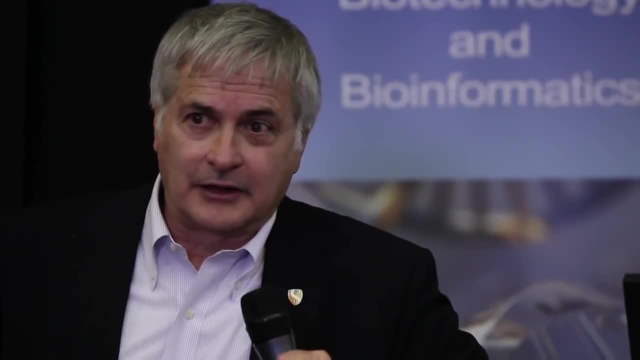 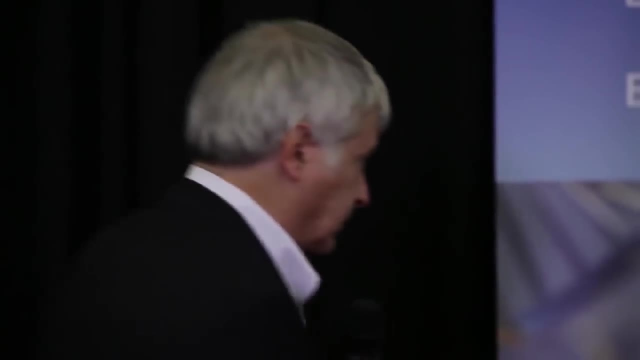 That's not much of a trick. They could have done that, And they could have done that a billion years ago and found it. But I don't know that they would send their rockets just to abduct the trilobites or breeding experiments. that wouldn't work. 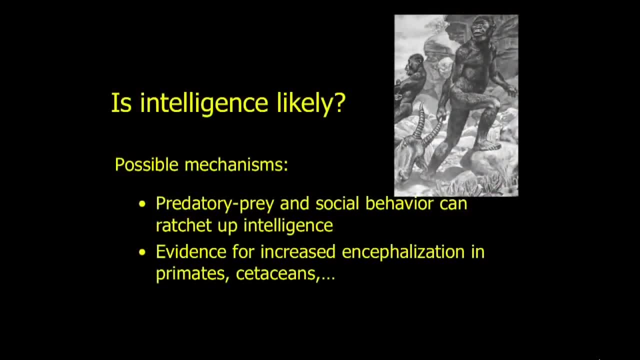 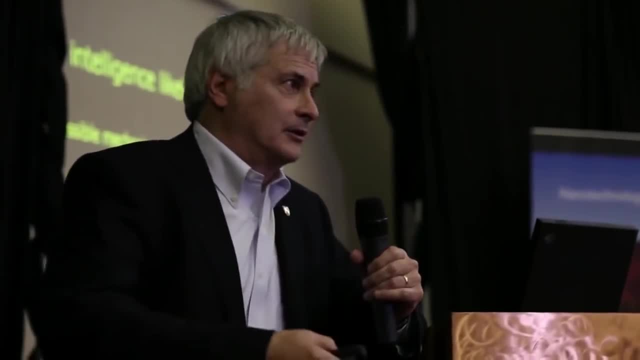 Then again, I don't know the aliens- Maybe they would This very controversial thing about whether intelligence is likely, And we don't know The only way to answer that, whether intelligence is sort of an inevitable evolutionary development or just something that happened here but probably not anywhere else. 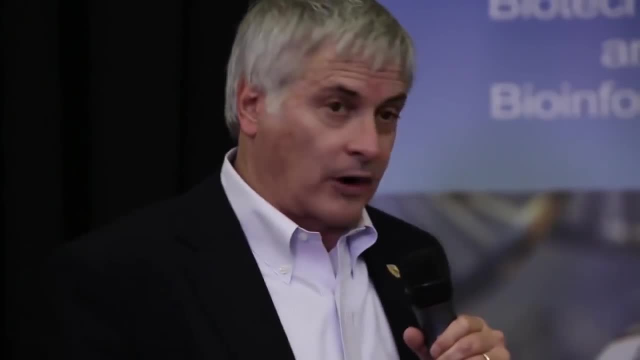 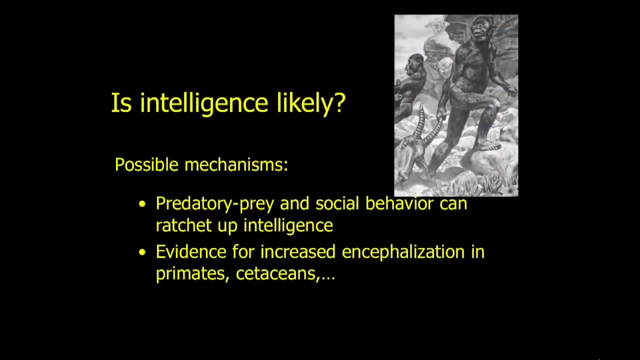 is either to find it somewhere else- that answers the question- or to figure out how it happened here. Why did we get smart? And there are various. I mean, there are people who study this. Not a lot of them, but there are some. 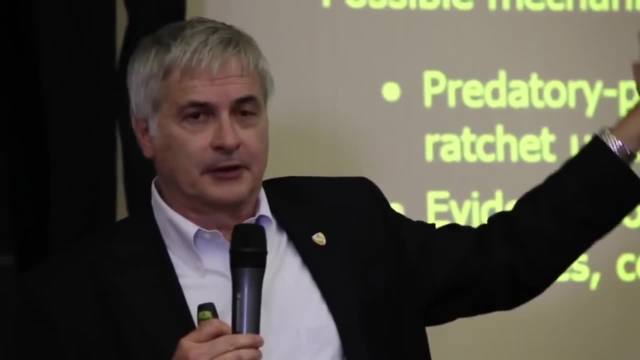 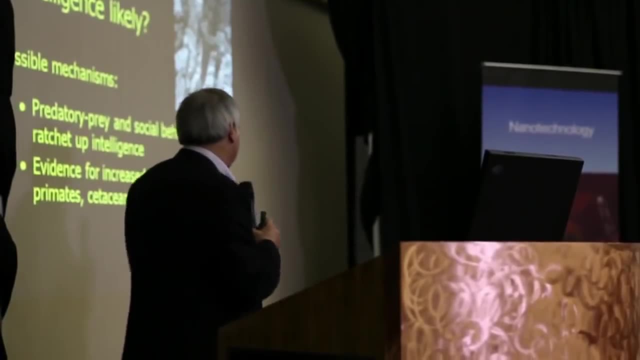 Now, first off, our definition of intelligence is very simple, straightforward. If you can build a radio transmitter, you're intelligent. So you should probably ask the person sitting next to you how well they can do at that. So here's a guy, 30,000 years after this photo is made. 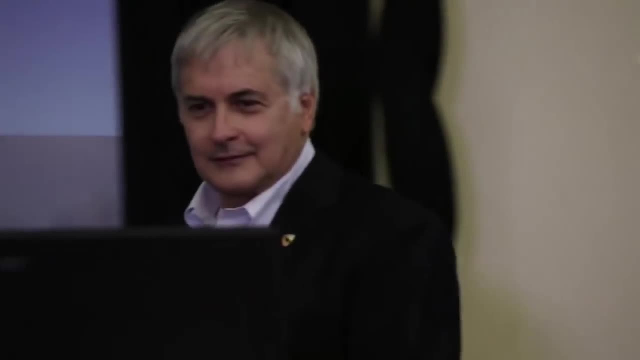 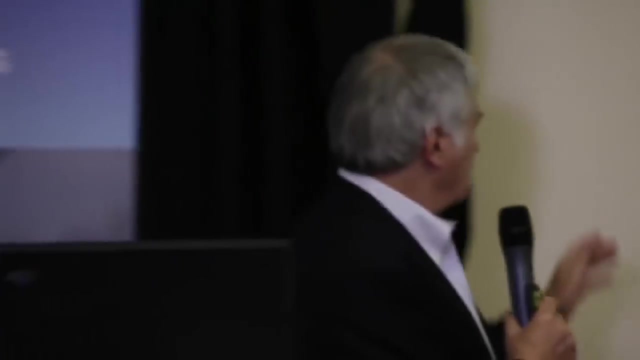 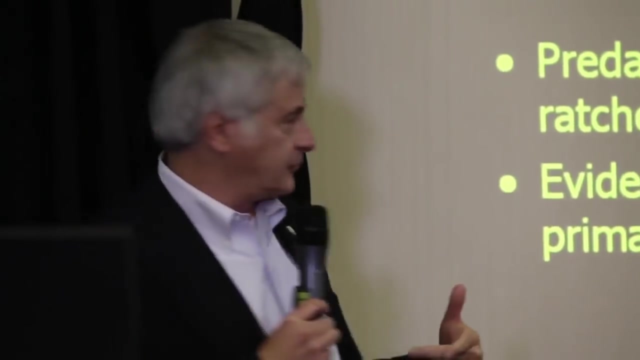 He's building a radio transmitter, so he's intelligent. And I never hesitate to say- although I've said it many times- that you can tell he's intelligent because he's adding some RAM to his computer there. Okay, Now there are various mechanisms in evolution that seem to suggest that the development of intelligence is not a very hard thing to do. 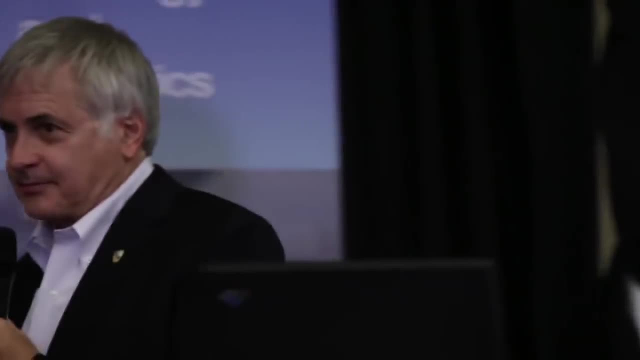 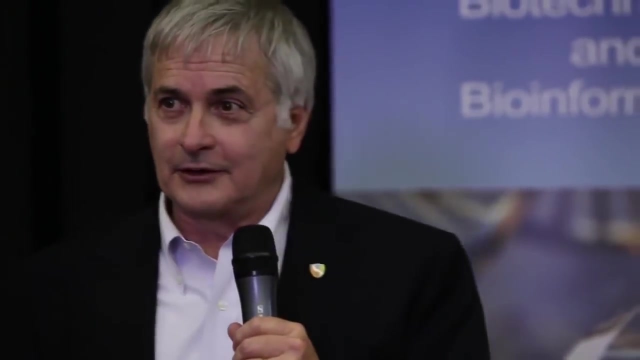 Predator-prey relations. you know They ratchet up the intelligence. They ratchet up the intelligence of both the predator and the prey, because the stupider prey tend to get caught more often and the stupider predators tend to go hungry every night. that kind of thing. 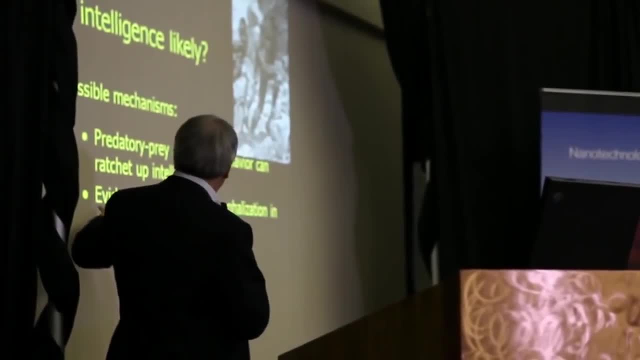 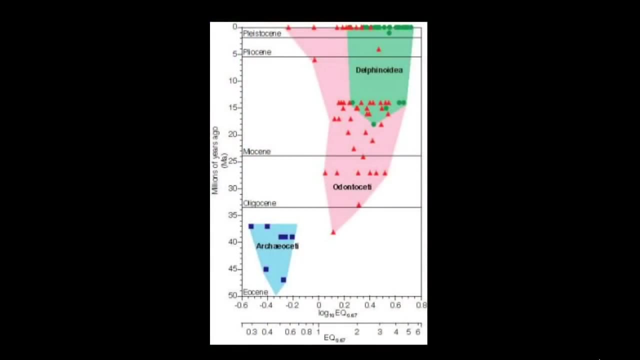 So you know, gazelles and lions are getting smarter. together There's increased encephalization. This is a plot from Laurie Marino, who's a biologist down at Emory University in Atlanta, And what she's plotted here is the IQ of toothed whales and dolphins. 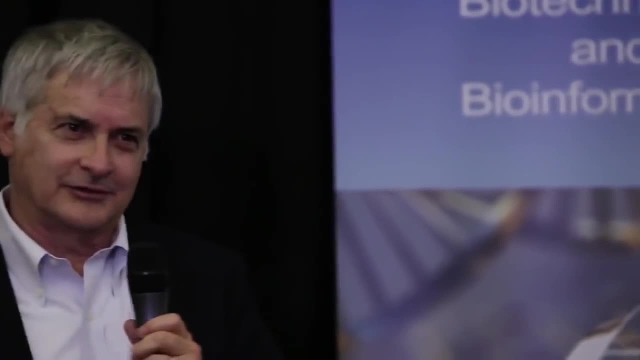 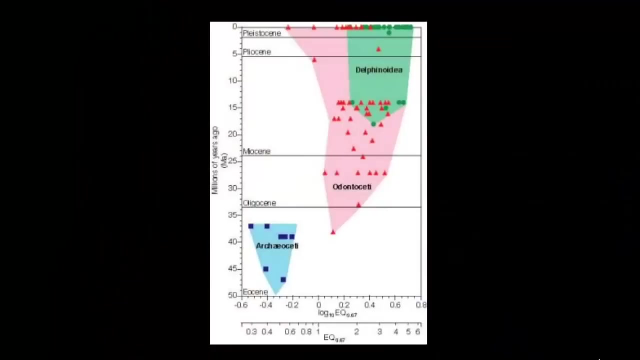 everybody's favorite intelligent species, the dolphins. I think that people like them because they just smile on their face all the time. Now she's got their IQs on the basis of either measuring their cranial capacity versus their body weight, or maybe she's found some fossilized SAT scores. 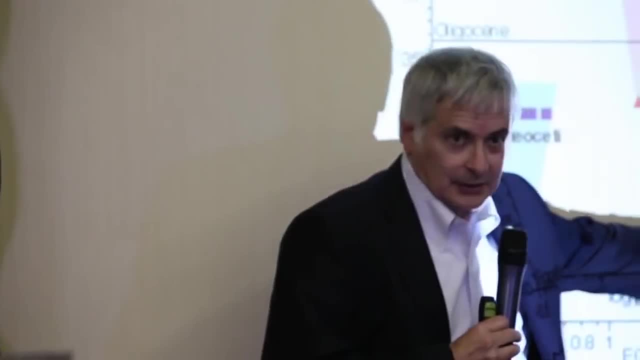 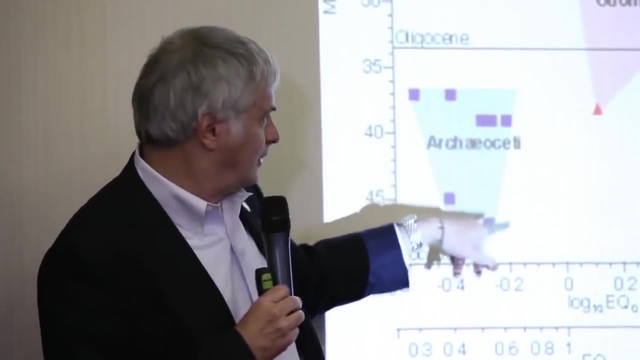 But in any case, you can see this is stupid here and that's smart there, And this is 50 million years ago and that's today up there. So 50 million years ago the dolphins were pretty dumb right. Then they developed echolocation. 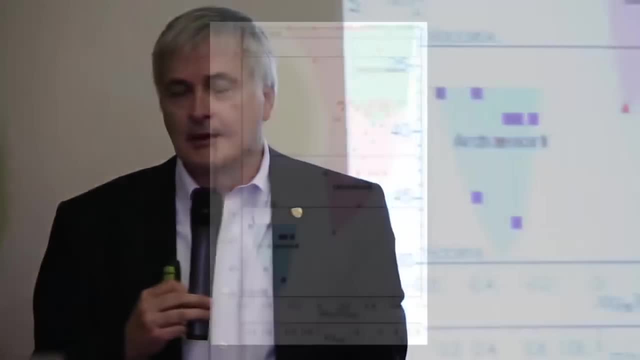 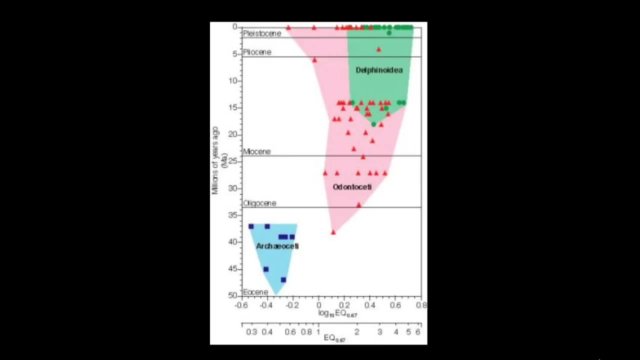 Their brains get bigger, They get smarter, And then you know they do various things. But you notice that some of them continue to get smarter, But still not all of them. Some of them got stupider again, But 2 million years ago the smartest thing on this planet was a white flank dolphin. 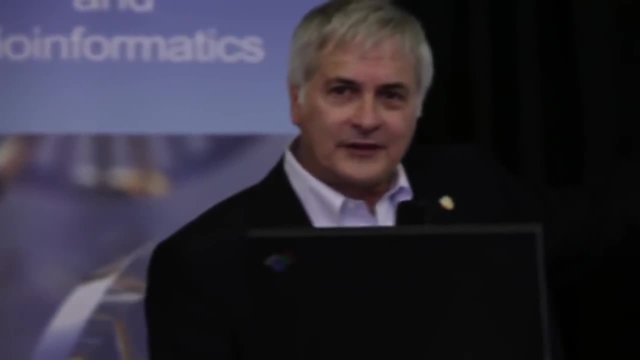 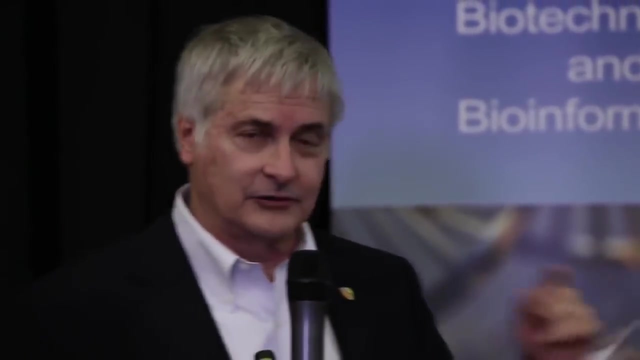 Probably not true today, but I don't know. So what this is saying is that look, here's another species from which we, you know, our common ancestor with this species goes back quite a ways. We're not that closely related to them anymore. 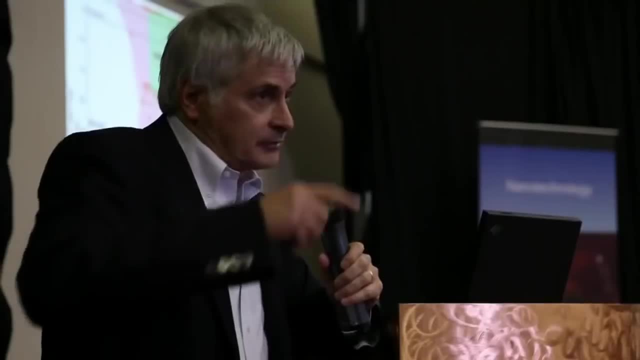 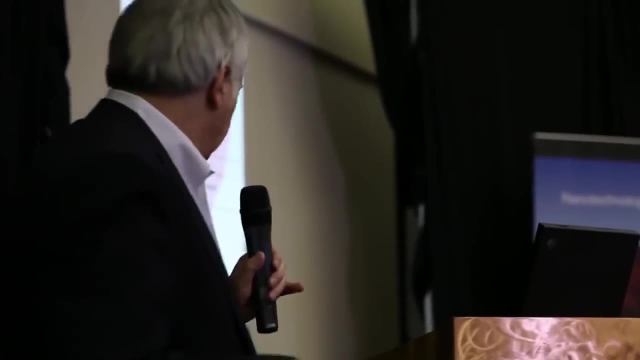 And yet it was developing more intelligent species, or more intelligent, you know, subspecies. Obviously, other primates have gotten smarter: Dogs and cats are probably smarter than all the dinosaurs. Birds- some birds are pretty clever. They say octopuses are clever, although I've never, you know, seen any great literature from octopuses. 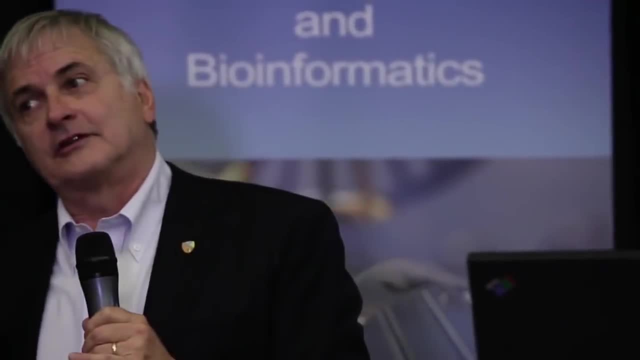 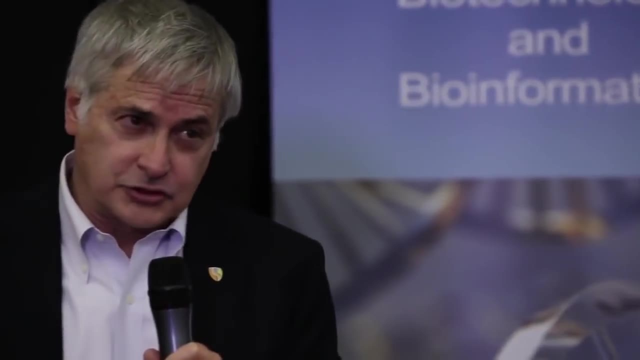 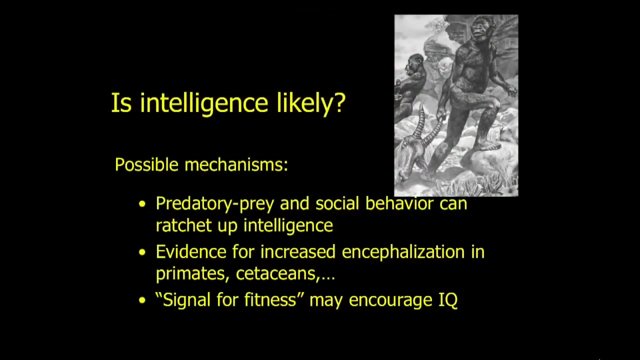 But still, the point is that not only our species got smarter, Lots of them did, And that suggests that there is an evolutionary push for at least some species to develop intelligence. Okay, Another idea, and I show this only because it's of interest to young people. 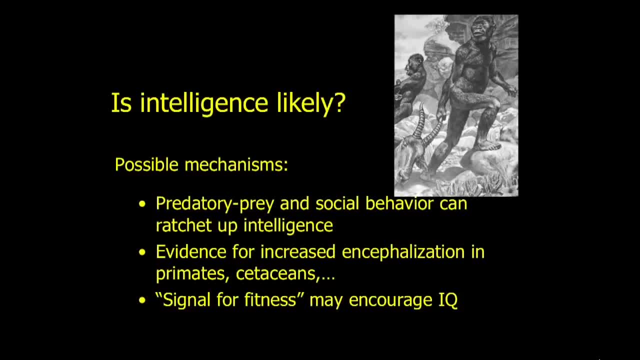 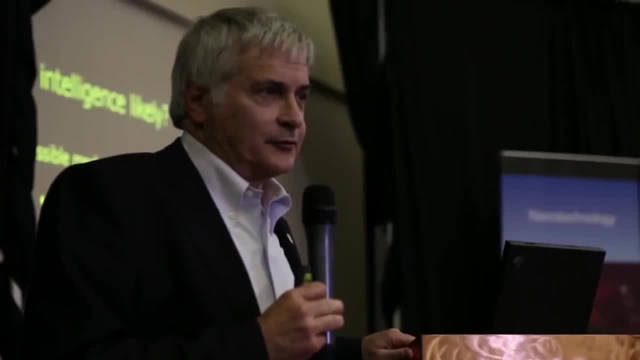 is the idea of Jeffrey Miller Here, A very clever idea, in which he says: look, the reason we got smart was because of the dating behavior of our ancestors, which was to signal for fitness. The canonical example here are the peacocks right. 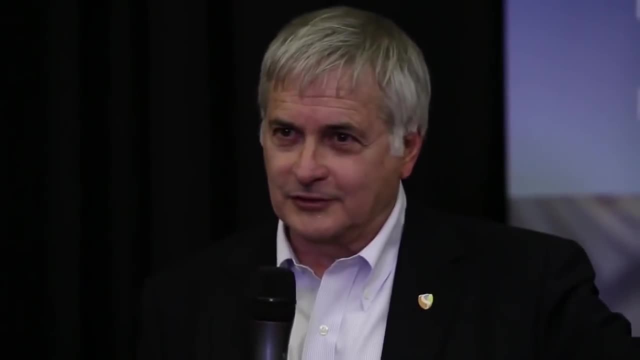 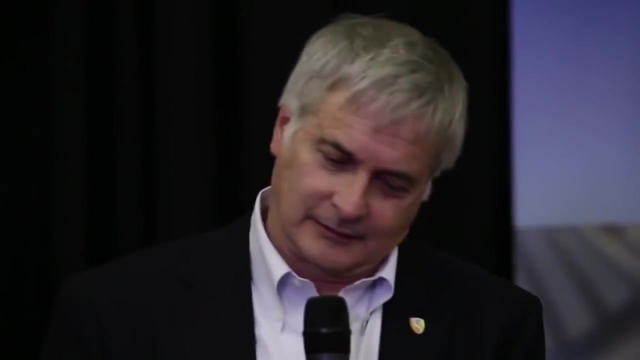 You know, the males display, the females decide. That's the same for us, right? But it's also true for the peacocks. So the peahens are sitting around, you know, looking at these peacocks, these male guys. 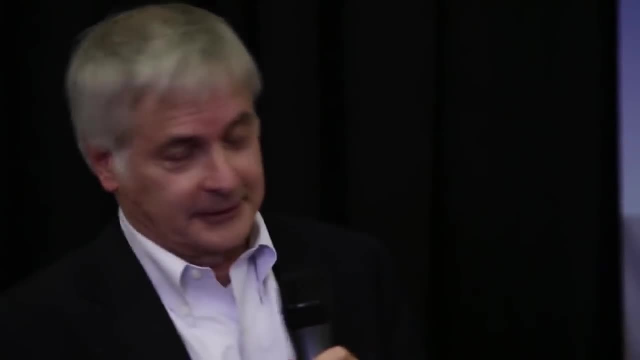 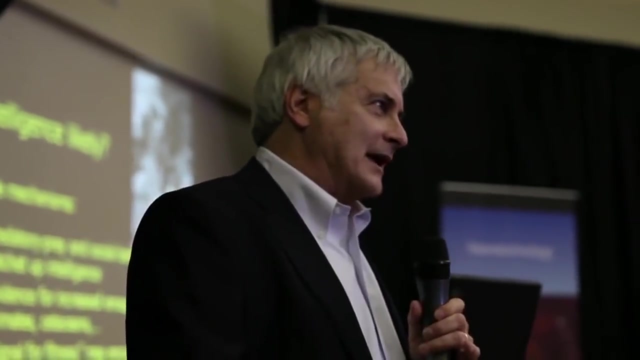 and they're walking around and they're showing their big blue feathers. Well, that guy's blue feathers are pretty good, but this guy's blue feathers are better, Right. So that one gets taken home to mom And the question is: what's in it for the peahen to have a peacock with those big blue feathers? 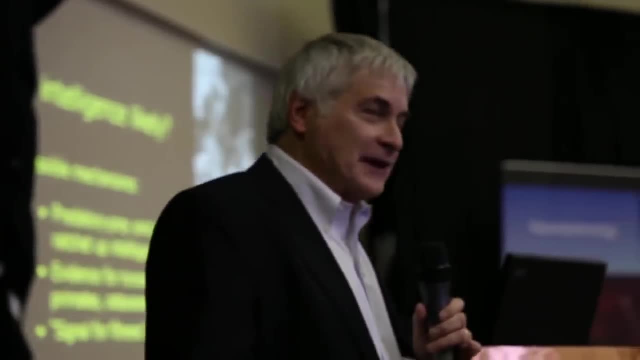 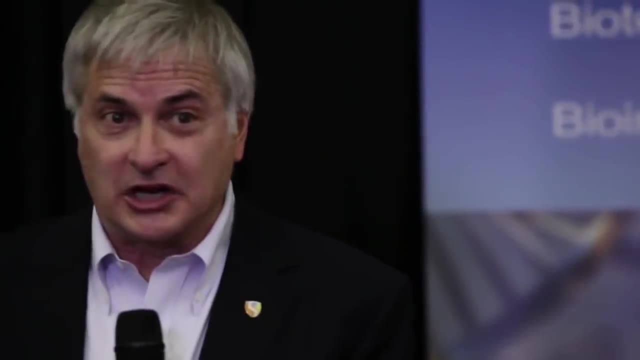 Because, after all, he only attracts predators, Right, And that's probably not a good thing. But on the other hand, he's here, He's made it, He's made it this far. His genes must be good, Because that's what she's really interested in. 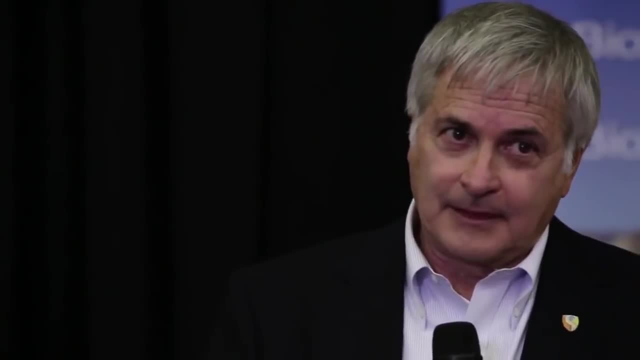 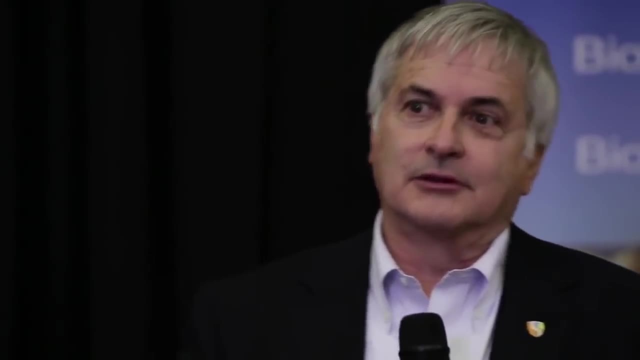 She wants some index into his genetic makeup so that the chicks will be healthy. Right, And it turns out. you know, growing those blue feathers is rather metabolically demanding, And if the genes had a lot of mutations we wouldn't be able to do it. 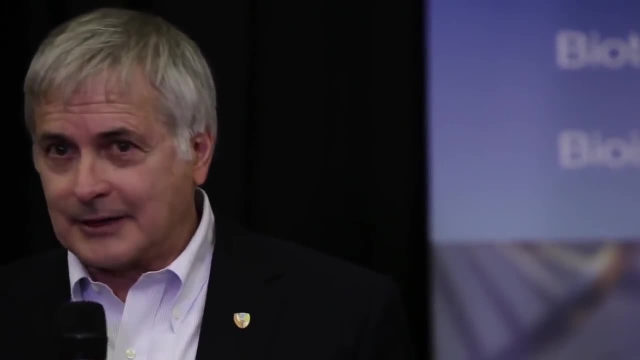 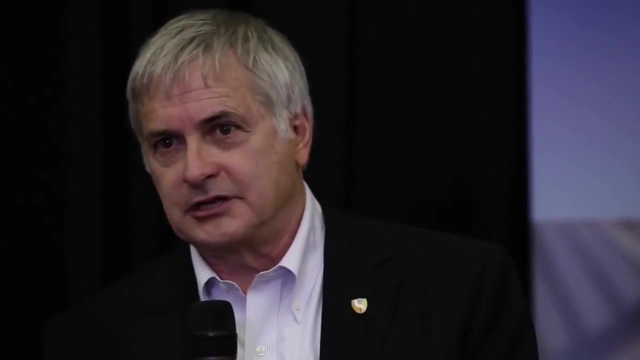 Right. So that's the deal Now. in hominids we don't have blue feathers, But our brains are rather intimately, you know, dependent on how many mutations are in our genome. So if your genome is messed up with a lot of mutations, your brain isn't wired up so well. 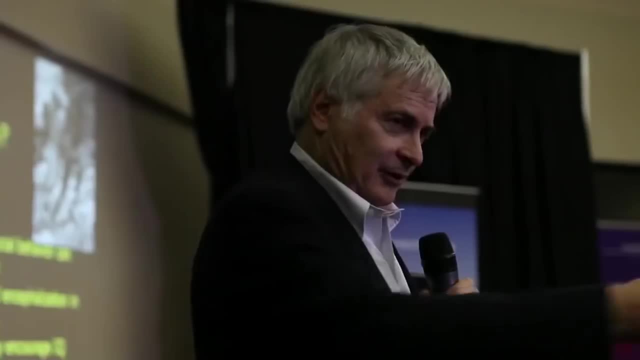 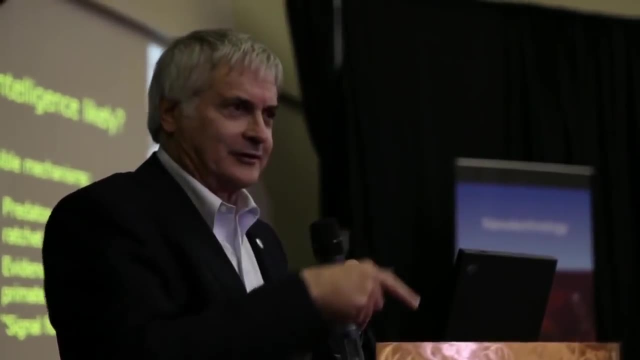 So the women are sitting around. I mean the guys are passing their brains around to all the women- Hey, check it out. And the women are saying, well, you know, Bob over here he's kind of interesting, Fred over there, he's more interesting. 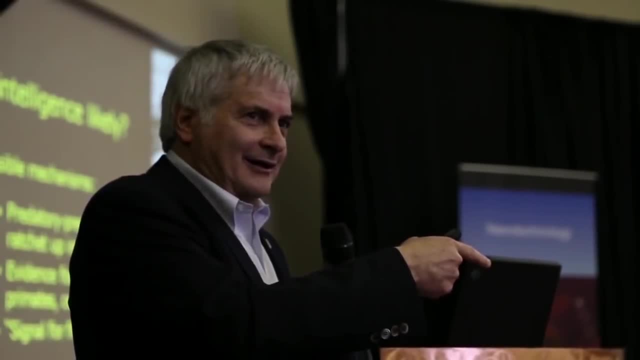 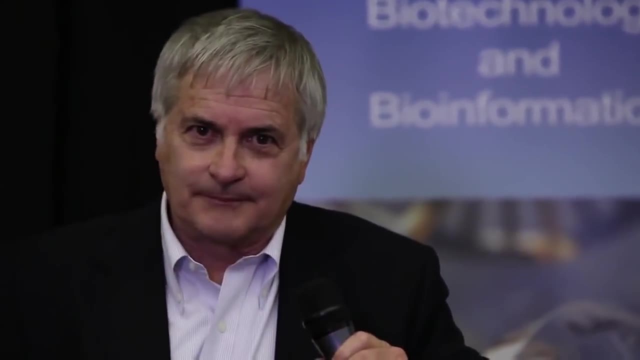 They're listening with their ears. It's not that they want smart guys like Fred. Women aren't really interested in intelligence, as far as I can tell. But the deal is that you know fewer mutations. And then there's the other factor, the fact that he's just walking around. 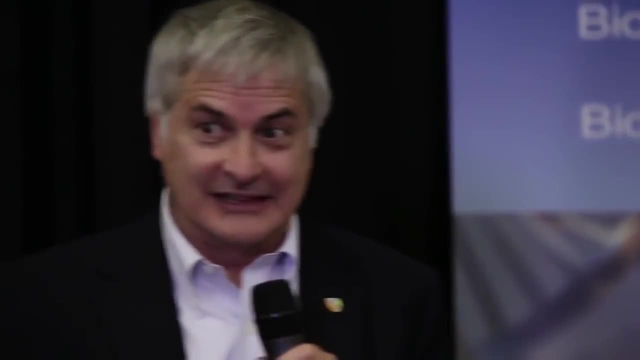 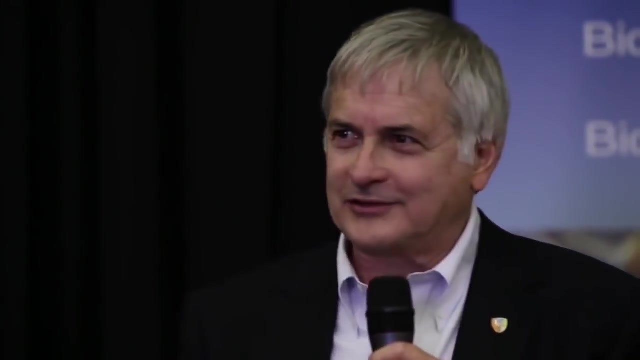 Right, I mean, this is like you know, this guy tracks predators, but he's still here. Remember all those Clint Eastwood films where Clint Eastwood rides into some godforsaken western town on a horse And the women all turn out. 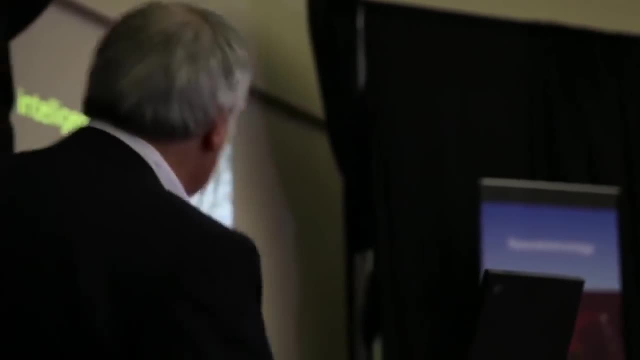 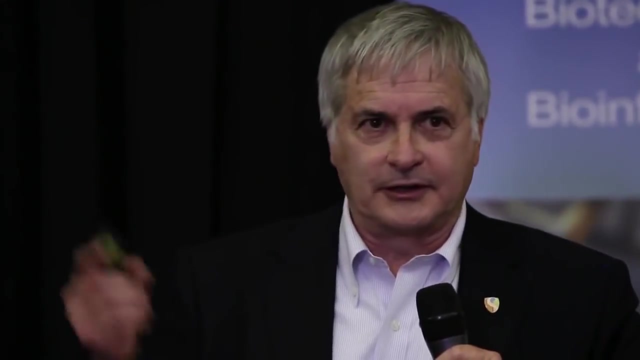 And you sort of wonder why This guy probably hasn't had a shower in three months. But they do it The same thing with Captain Cook. He had syphilitic sailors on board his ships And he would keep them on board the ship so they didn't infect the local population. 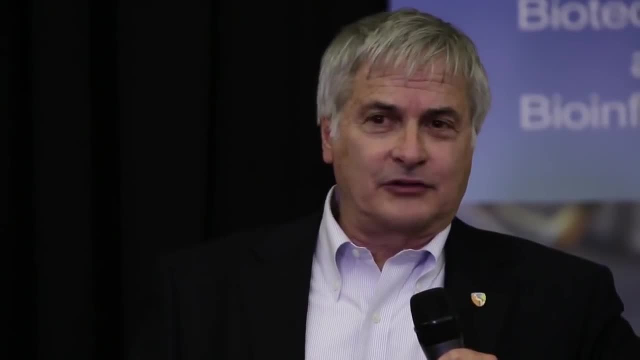 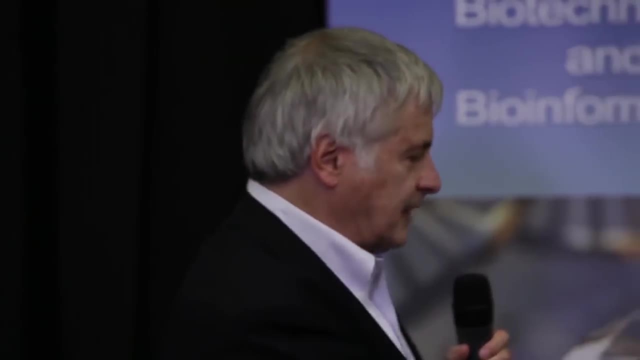 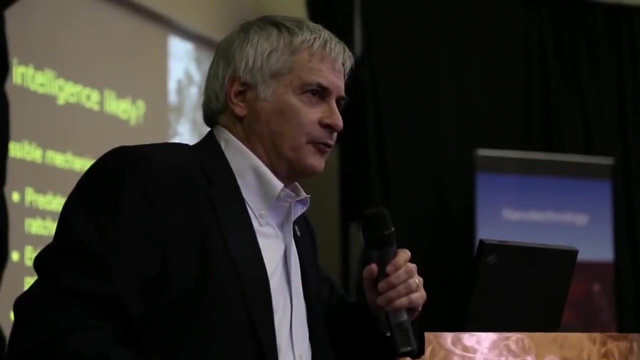 But the women swam out to the ship And I asked an evolutionary biologist, why would they do that? And she said: look, they've made it this far, They must be good. So that's Miller's idea that you know. the male's IQ got ratcheted up by women who were looking for fewer genes. 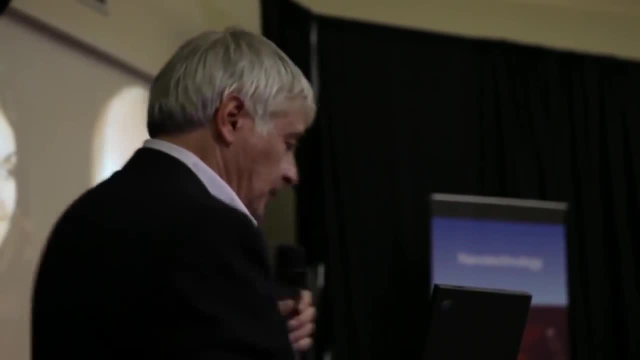 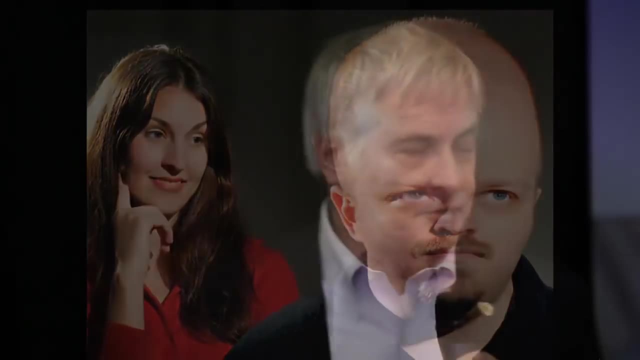 More genetic mutations, Of course, and that means this guy's very popular. But the question, of course, was: why did the women get smart? And his answer to that is: well, they were under a lot of pressure- evolutionary pressure as well- to be charismatic and interesting, to keep the guy from wandering off. 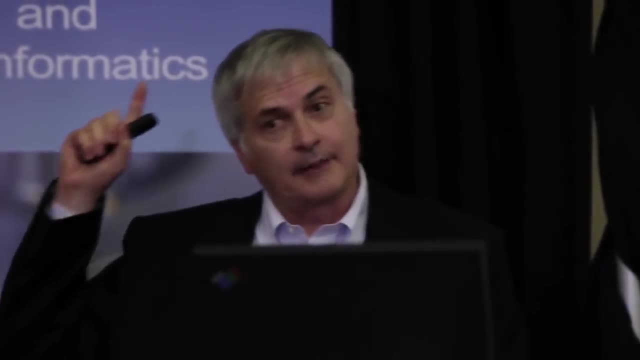 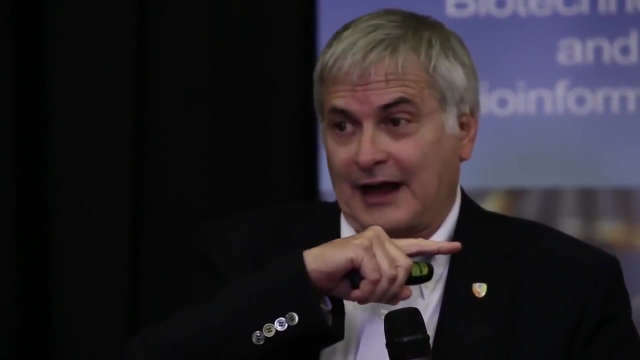 So there you go. All right. Now the point of all this story, which may or may not be the actual story. Miller thinks it is And he makes a compelling case. But if this, or anything like it, is correct, then intelligence should be pretty common in space. 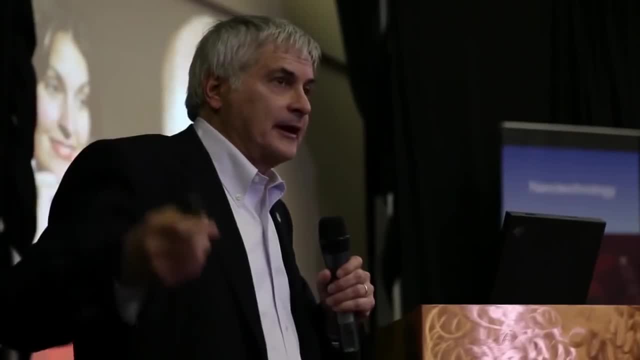 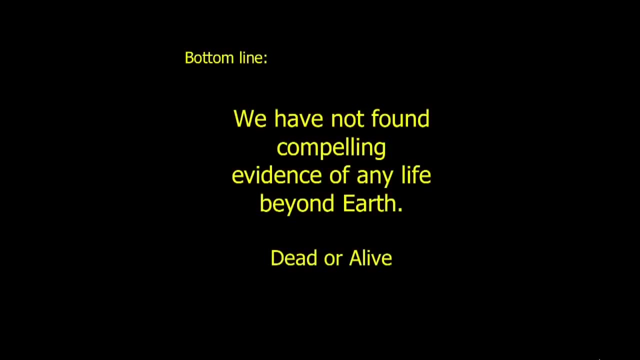 Because this is just a very simple Darwinian mechanism that could obtain on a lot of planets. Okay, The bottom line: we haven't found any compelling evidence of any life beyond Earth, not even pond scum, not even dead pond scum. 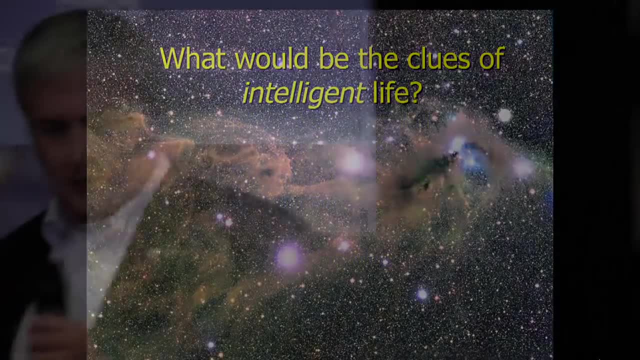 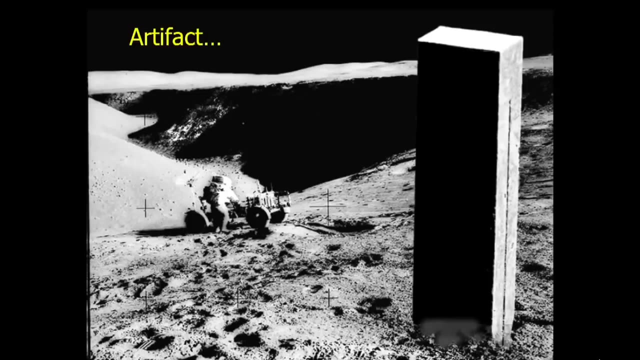 But we're looking, So how do we look? Well, I'll go through this fairly quickly. I mean, one thing you could do is just look for artifacts. This is one of the Apollo photos that wasn't released to the public because obviously I did this in Photoshop. 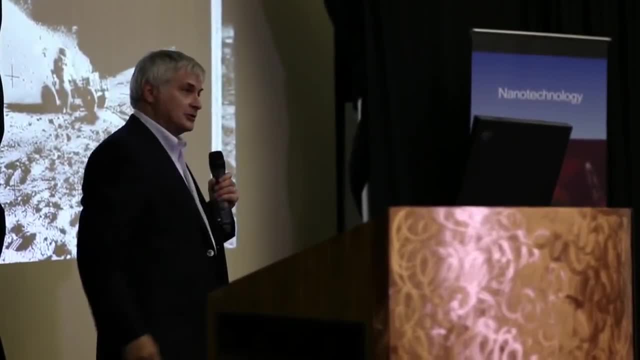 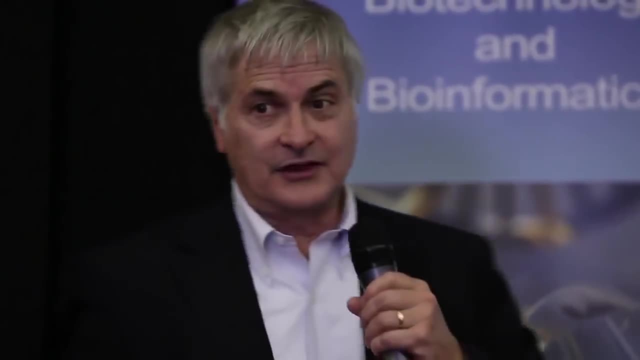 But clearly this is not a you know. there's nothing wrong with this kind of an approach. You just look for things in space, right, that were left by aliens, And one of the big advantages of communicating this way- leaving a time capsule- is that, unlike a radio signal, a time capsule could be there for a very, very long period of time. 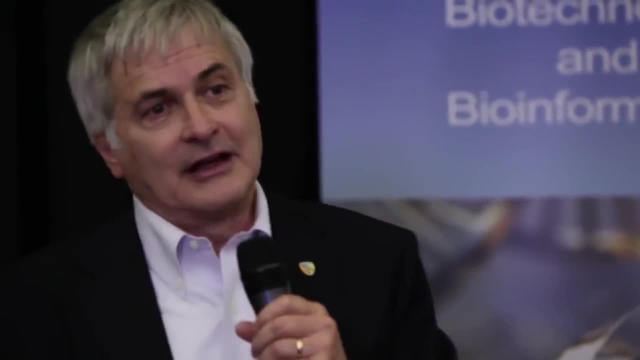 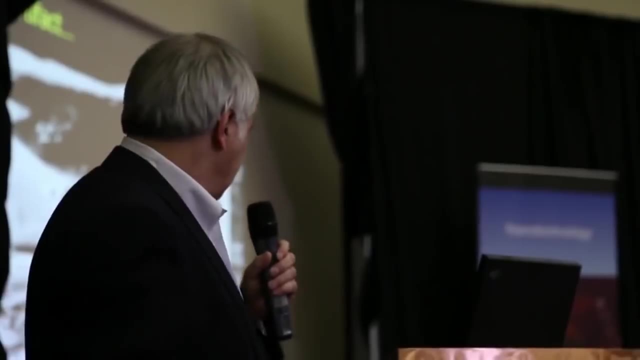 You don't have to have synchronicity, You don't have to be broadcasting a signal at the right time that somebody with an antenna will pick it up at the other end. This just sits there until they find it. Okay, We've not dug up the moon looking for these things. 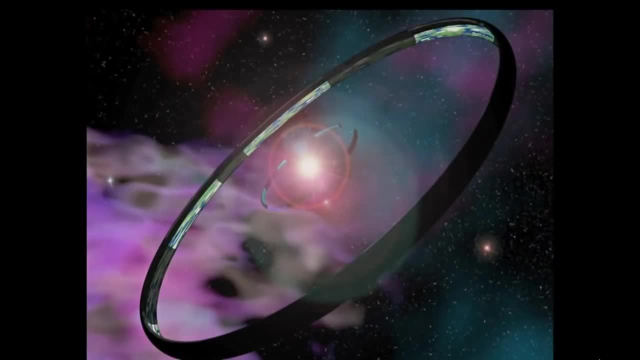 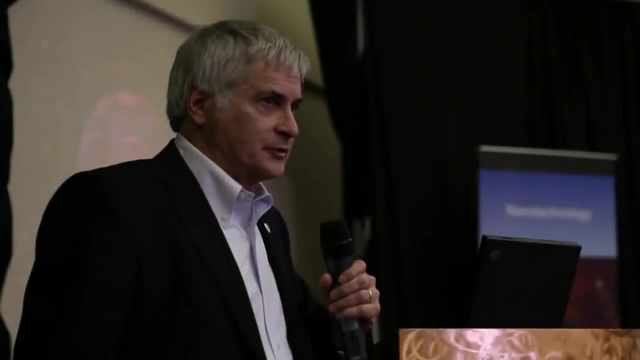 But it's something to do. We could look for, you know, ring worlds or Dyson swarms or stuff like that. Okay, All of these things make sense And there's a little bit of an effort to find these things. not much of one. 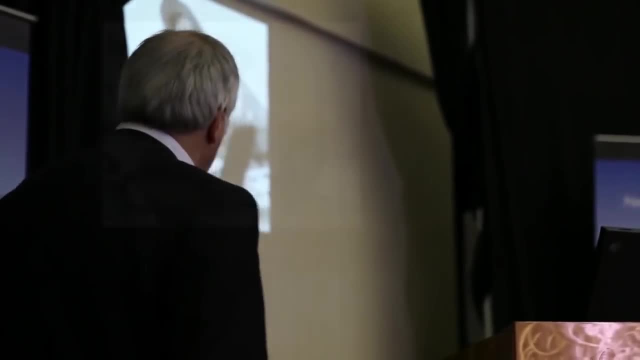 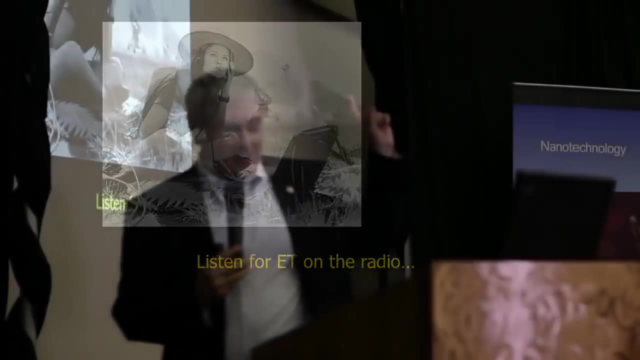 One could use a better effort. And then, of course, there's the Jodie Foster approach, And this is kind of my day job. We told Warner Brothers this is wrong, because we were listening to 56 million channels simultaneously at the time. 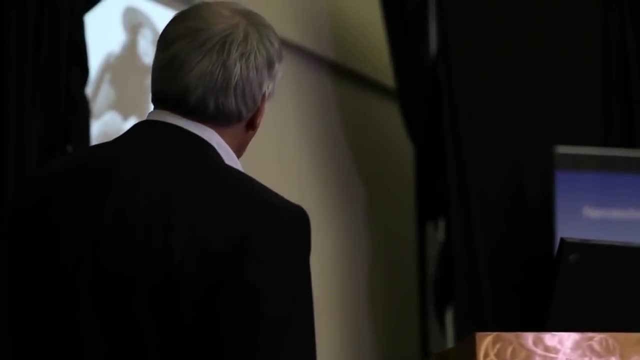 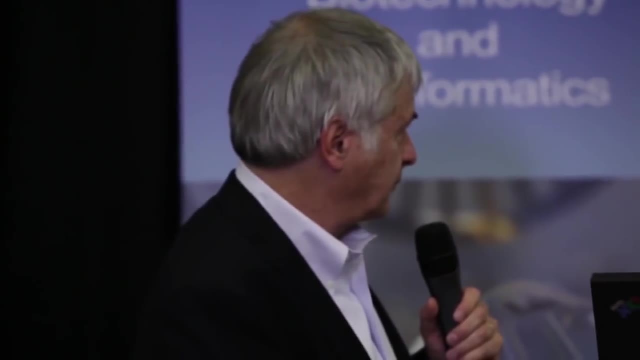 We said you have to put 28 million pairs of earphones on Jodie. They didn't do. There she is again. She's got the VLA, which has never been used for SETI but is very photogenic, And the idea here is that we'll just pick up the signals. 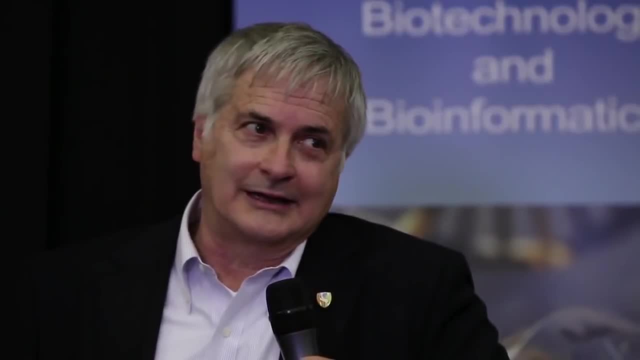 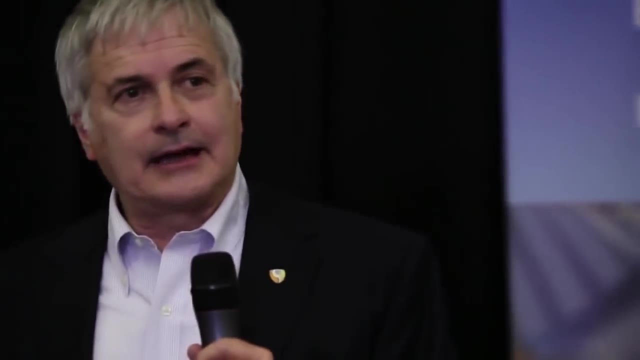 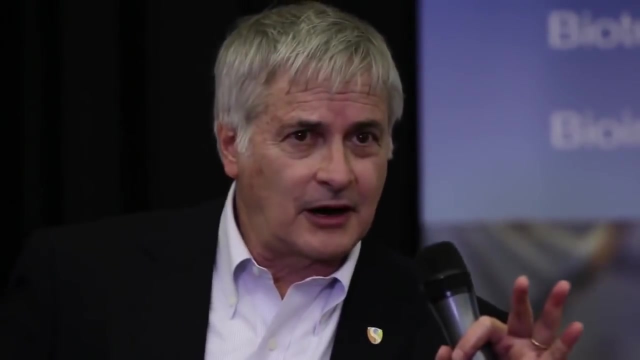 And that you know this was doing. the numbers is a one-line calculation And that was done by a couple of guys at MIT in 1959. And, to their surprise, what they did was they essentially said: if you took the biggest radar transmitter on the earth and then the biggest radar antenna receiver combination on the earth and you just aimed them at one another, how far could you separate them? 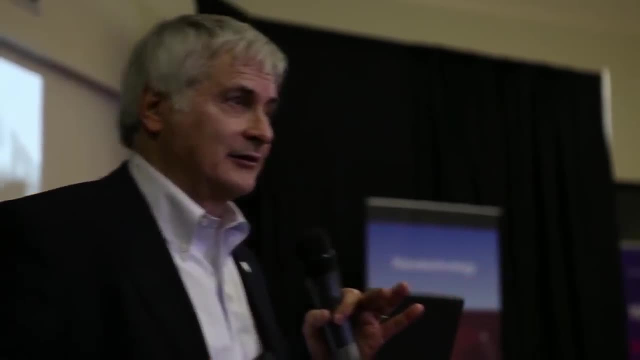 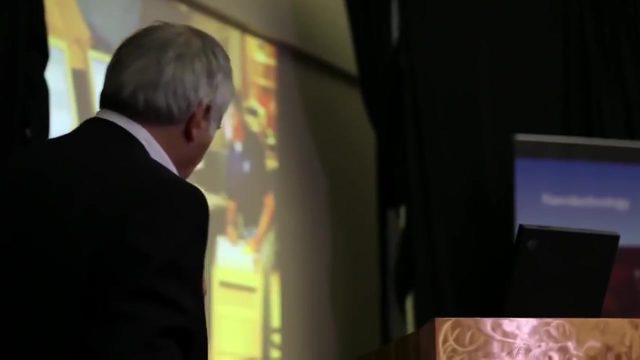 And still pick up the transmitter with the receiver. That was the calculation, And it turned out to be light years. That was the astounding thing. So this works on paper. Okay, Now the way you actually observe this is ten years ago now. 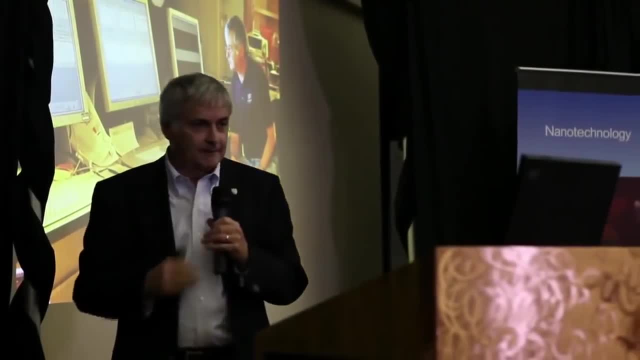 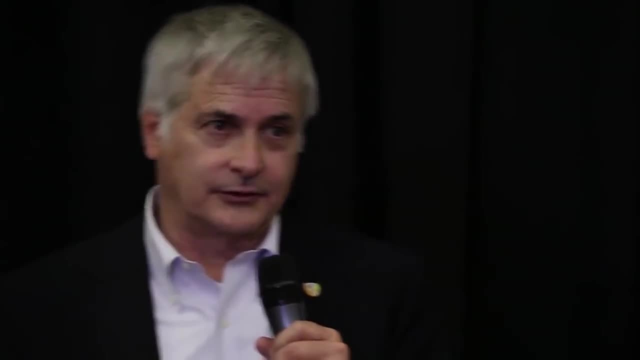 This is down at Arecibo in Puerto Rico. You have a couple of work stations that are doing the monitoring, because you have tens of millions of channels and so forth and so on, And also they don't require coffee breaks And they can find, they can integrate up signals and, you know, increase the signal to noise in various ways that your eye or your ear could not do. 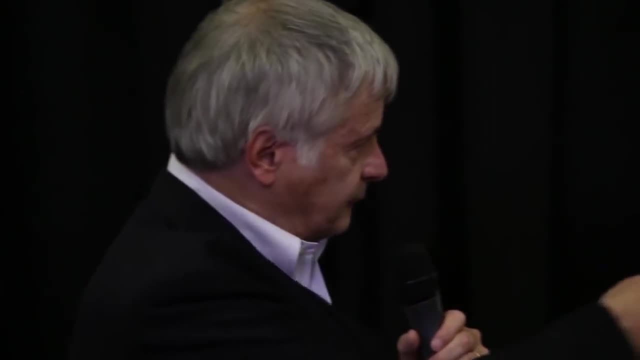 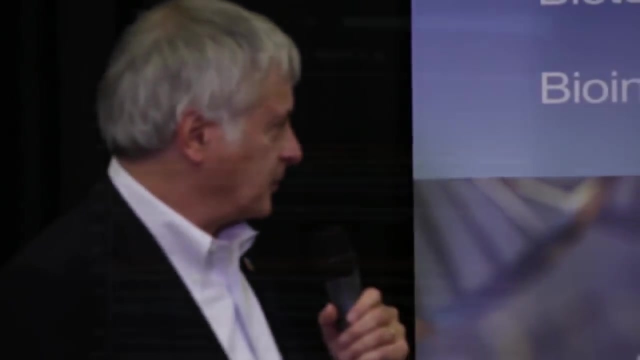 So obviously it's all done by computers And in fact you really wouldn't have to sit there once it's all automated- And in fact it is being automated now- You don't want to actually sit there. That's very boring. The kind of signal we look for are narrow band signals, If the aliens are deliberately trying to get in touch as opposed to just picking up their cell phones, which would be very broadband. if you just wanted to get in touch, you would put a lot of transmitter energy into a very narrow band. 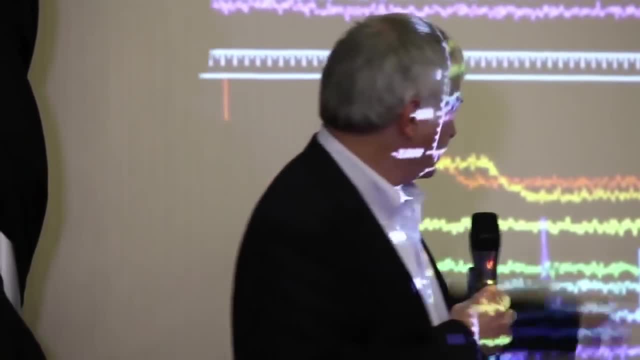 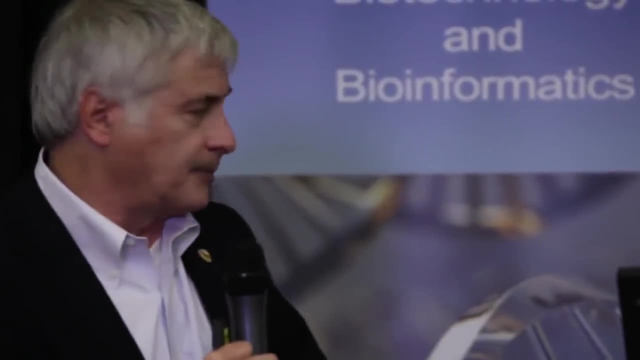 Because that makes the signal to noise at the receiving end the highest. So you look for things like this. Those are the kinds of signals, by the way, that nature does not make: quasars, pulsars and so forth. You don't have to worry about those. 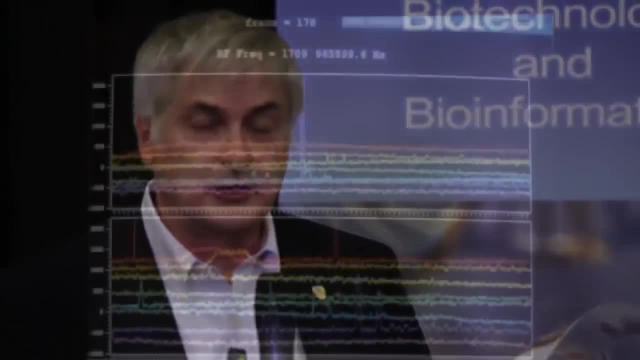 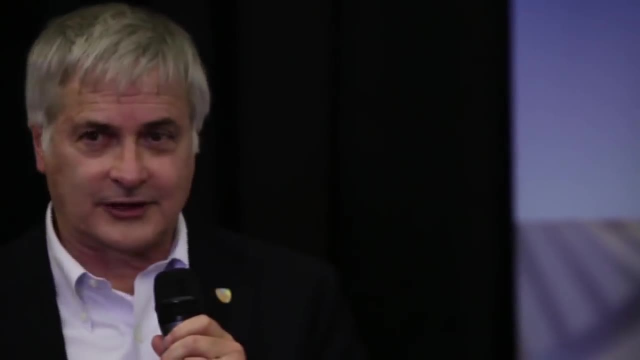 You never get such a narrow band signal, So you look for very narrow band signals, one hertz, even less. Now this looks good. This is right off the telescope down in Puerto Rico, But those are all you know: radar sets, telecommunications satellites and stuff like that. 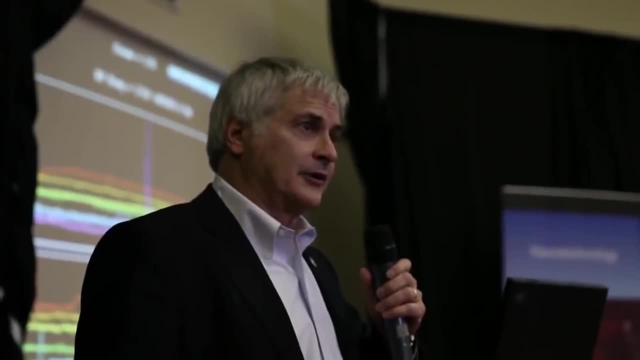 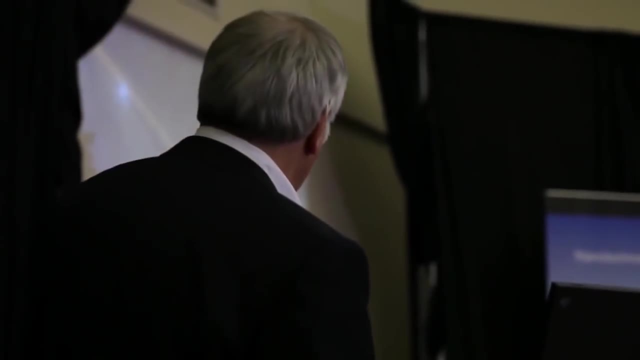 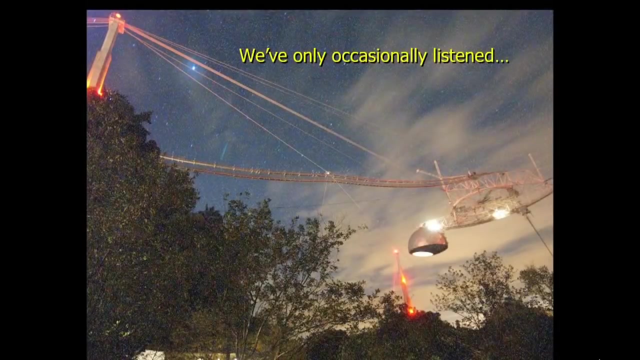 And you have to sort all that out. Where you really want to put this whole experiment is on the backside of the moon right, which is perpetually shielded from earth. But there's certain problems there with cost. Okay, Let me point out again that although this experiment is now a 50-year-old endeavor, it's very intermittent. 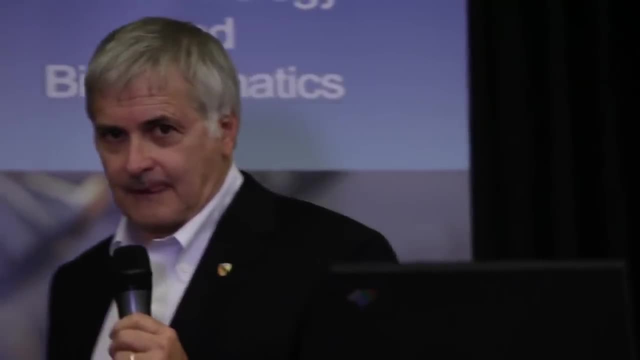 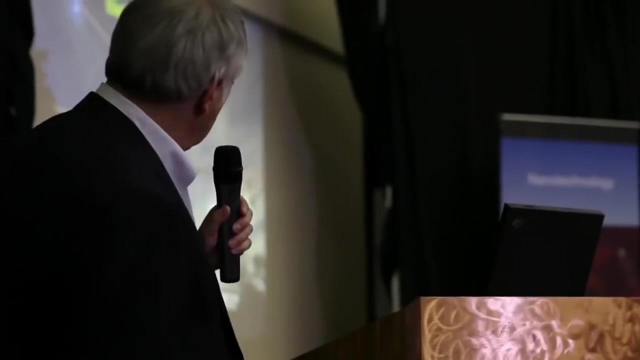 If you add up all the observing time done for SETI, in which we looked at particular targets in the sky, it only amounts to a few months worth of observing, And that's because we always had to use somebody else's antenna, like this one down in Puerto Rico, a thousand feet across. 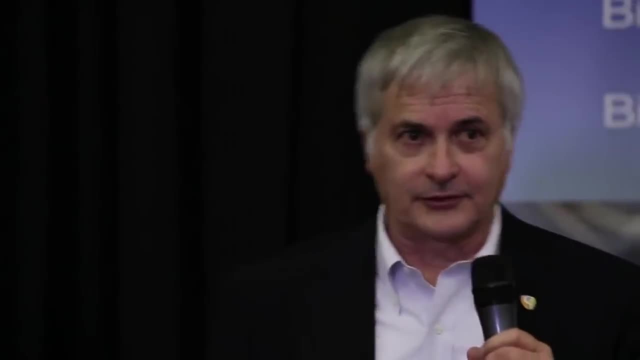 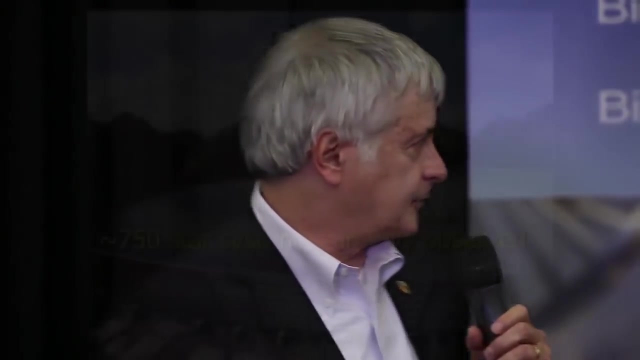 It's a great antenna, but it's being used mostly for studying pulsars and quasars- sorry, not quasars, pulsars and galaxies. So you only get a little bit of observing time. Well, we're trying to improve that. 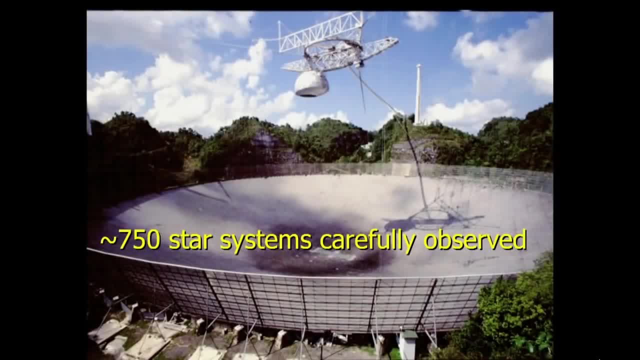 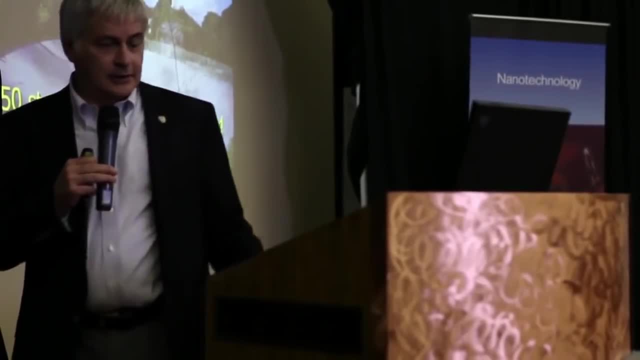 The bottom line of all this is actually that the number of star systems looked at carefully for signals is fewer than a thousand. It's a very small number. Paul Davies has a book out now called The Eerie Silence, But even he will admit that there really isn't an eerie silence. 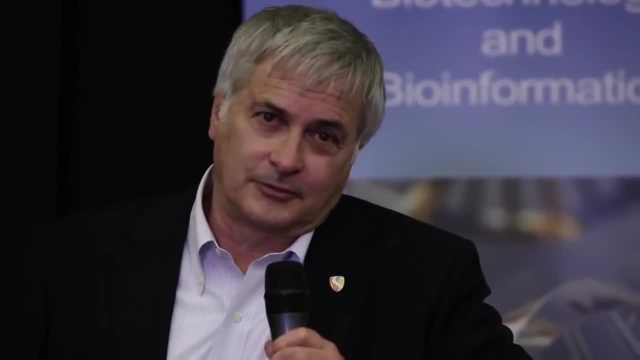 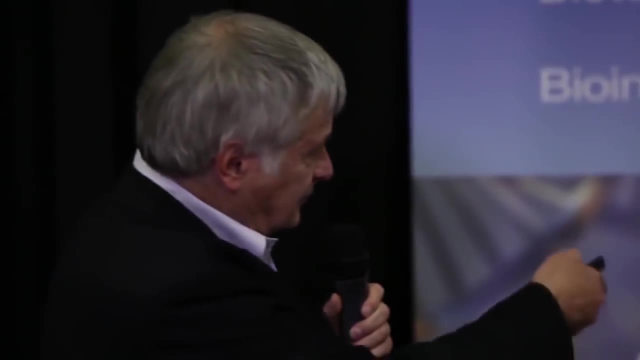 We've been trying to find ET and we've barely scratched the surface. in terms of the number of star systems that have been looked at carefully, It's not at all surprising We haven't found them so far, But this is kind of discouraging. 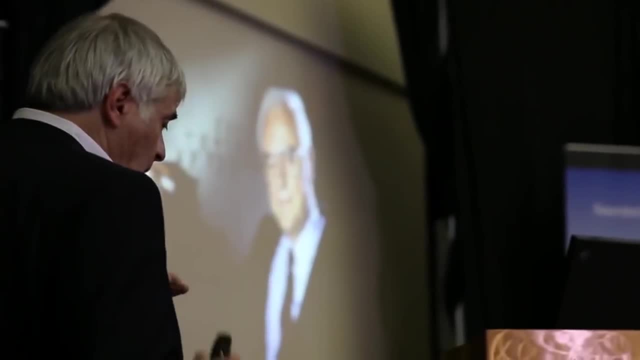 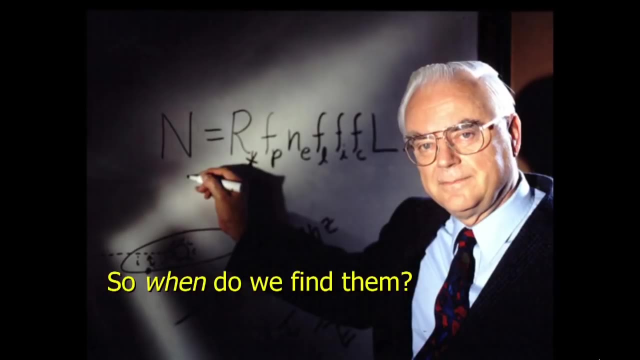 After 50 years, we still have fewer than a thousand stars, looked at carefully. Well, that's going to change. So this is Frank Drake. by the way, This is the guy who did the first SETI experiment. Frank just turned 80, last month, or two months ago, I guess. 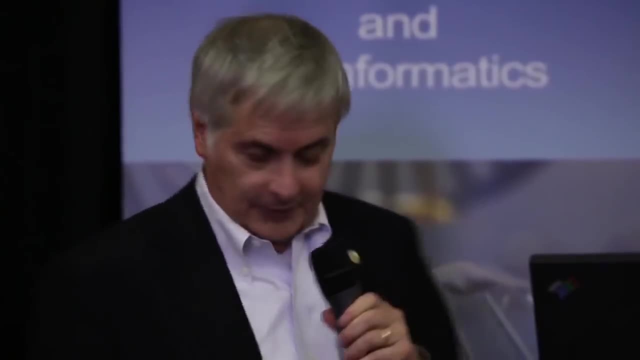 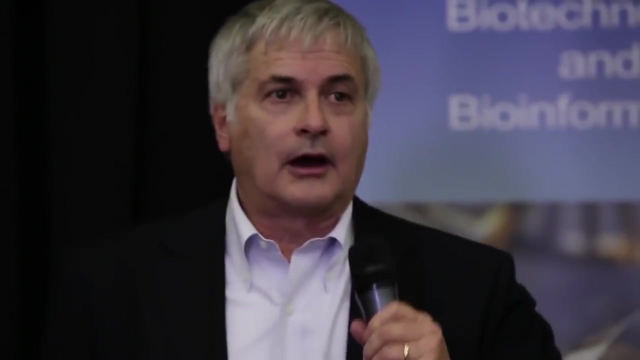 And he still comes into the office. He comes in and writes this equation on the board. We're not sure what it means, but there it is. And, as I said in the beginning, Frank and the rest of us are frequently asked: when are we going to find them? 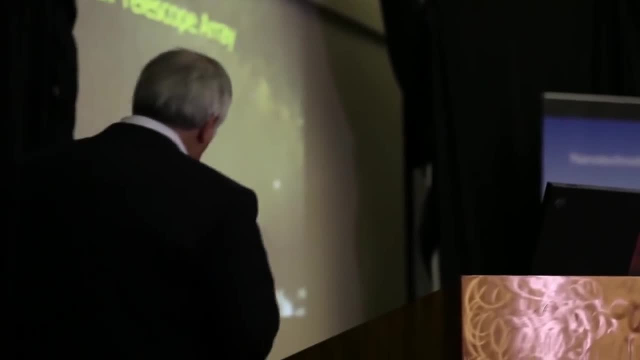 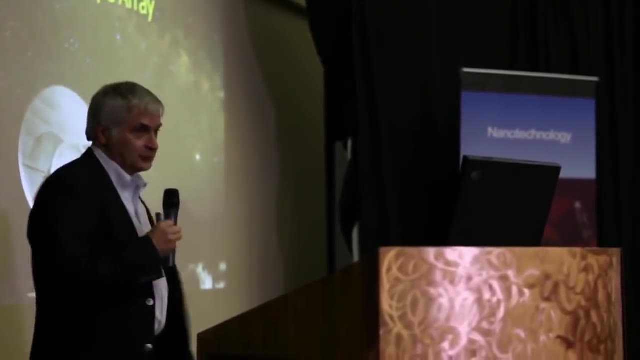 Now here comes the answer to that. To begin with, we were building this. We were building our own instrument. It's called the Allen Telescope Array. This is Paul Allen. He gave the money to get this started. Okay, so the first 42 antennas of an eventual 350 were financed by Paul Allen. 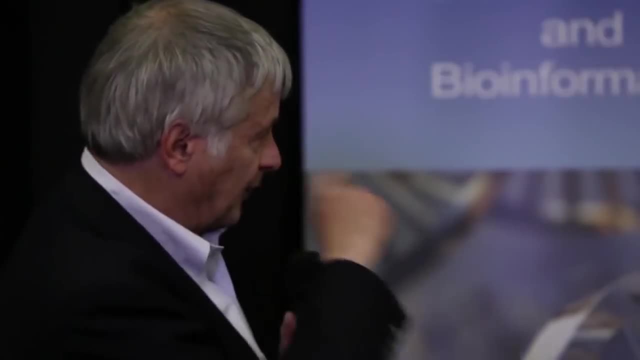 They're about 20 feet across. You can see me in this photo. There's Jupiter over on the right. They're about 20 feet across. This is about a five-hour drive from where you're sitting. If you have the time, you might drive up there and take a look at it. 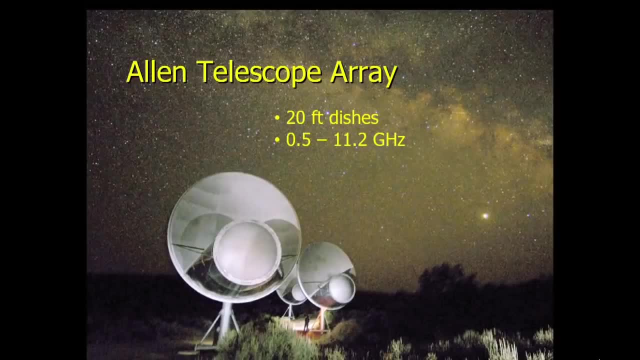 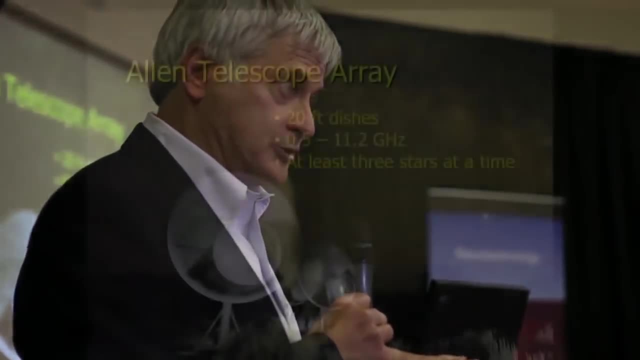 It's kind of a nifty place. It can cover a very wide range of frequency And because it's an array, you can actually make pixels on the surface, You can make pixels in the sky, wherever you want them, just computationally. 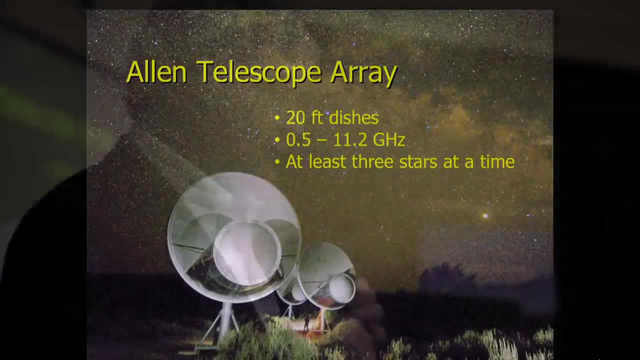 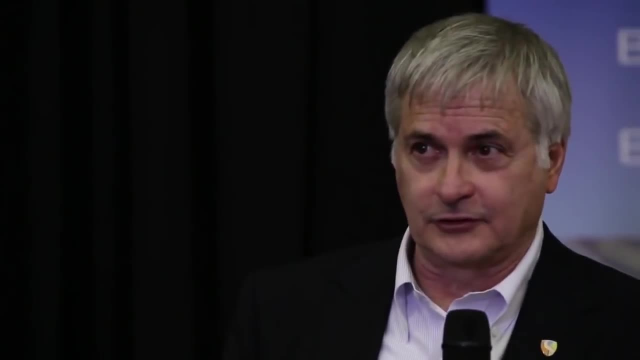 And that means you can look at more than one star at a time. That speeds up the search. The whole thing that's of interest here is not that this is more sensitive than previous searches- It's not, But it's faster. It's much, much faster. 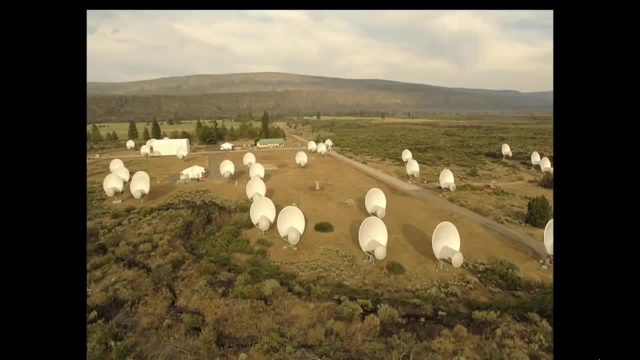 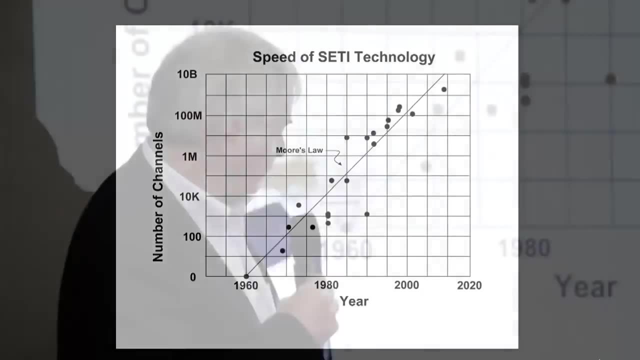 And not only is it faster, it will continue to get faster. This is what it looks like- all 42.. This is some sort of plot showing the speed of SETI searches. I just took some index of the speed of our searches. 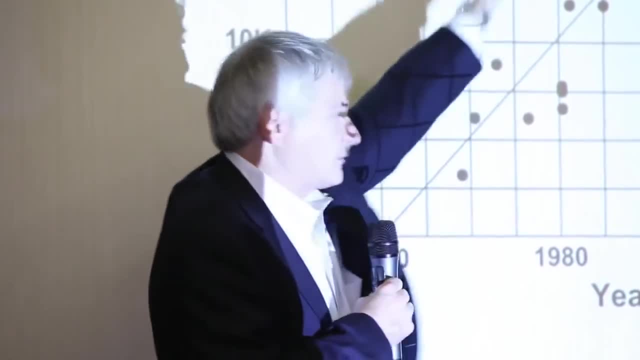 Ever since Frank Drake's first search in 1960. So these black dots show you know the speed And you can see it's going up. And those of you who are still conscious may notice that this is a semi-log plot. 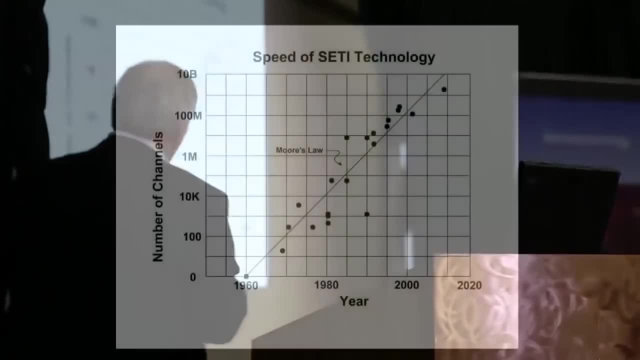 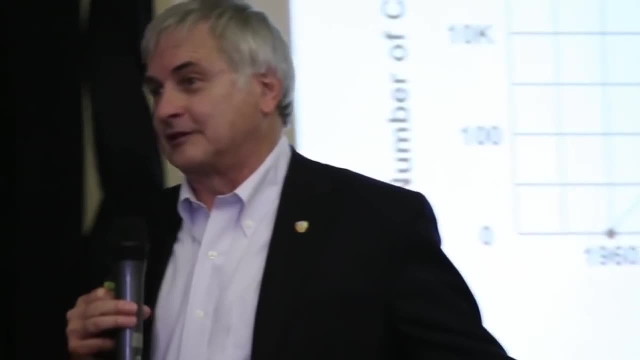 So it's going up exponentially And of course, what's fitted here- singularity- is Moore's Law, right? Well, it follows Moore's Law pretty well, because this is mostly digital electronics. So when people ask: when are you going to find ET? 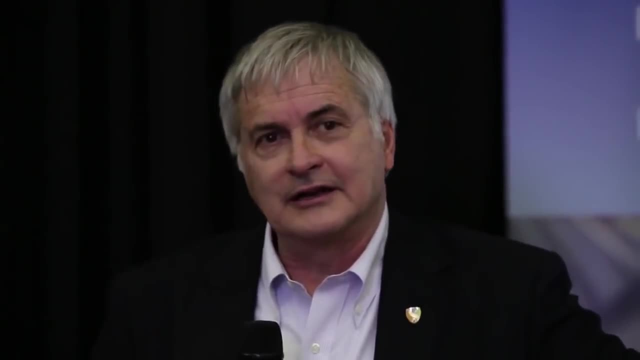 Well, look, you're looking for a needle in a haystack, And the question is: when are you going to hit a needle? It only depends on a couple of things: How big is the haystack? We know that We're looking in the galaxy, so we know how many star systems there are. 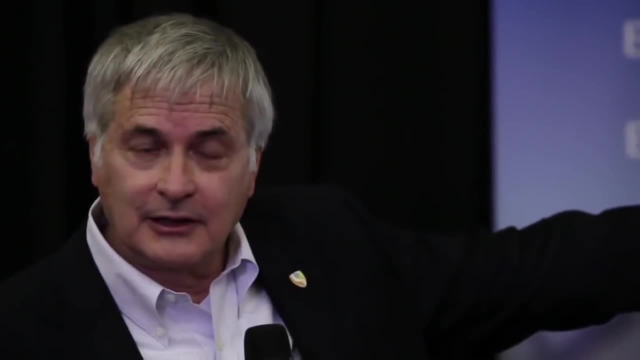 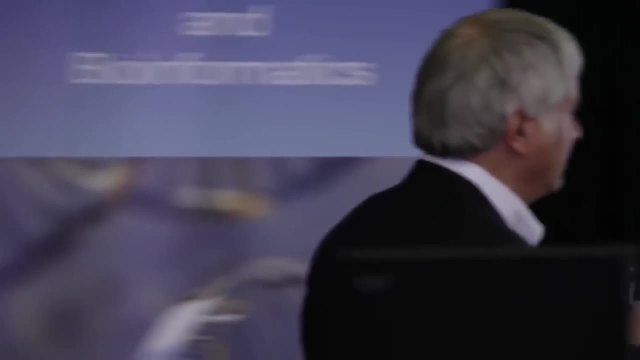 Second, how fast are you going through the hay? Well, that tells you. And third, how many needles are in there? Well, that we don't know, right, Okay? well, here are some guesses, as the number of needles n gives the needle number. 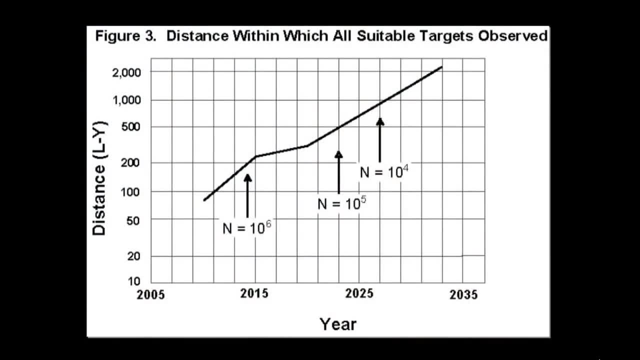 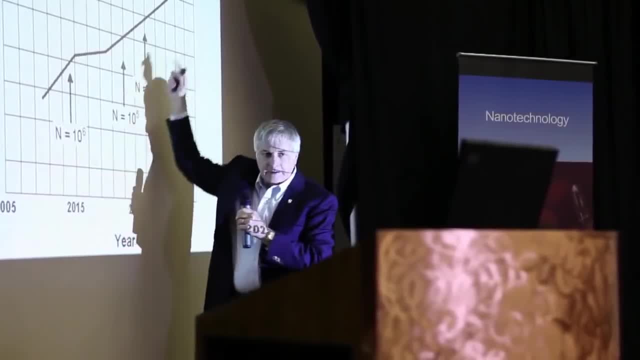 Okay, This line up here shows you how far out into the galaxy we would be able to search with this thing, assuming it was more or less completed in that year, And you can see 100 light years out, 200 light years out, and so forth. 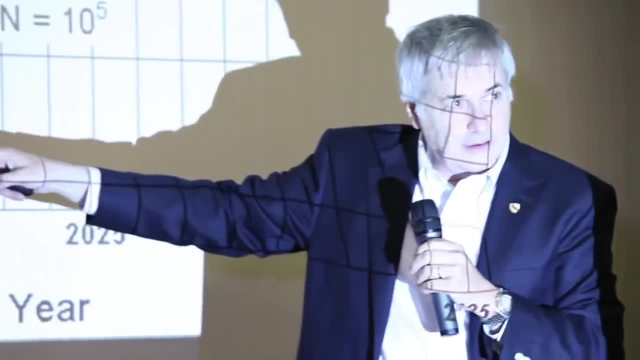 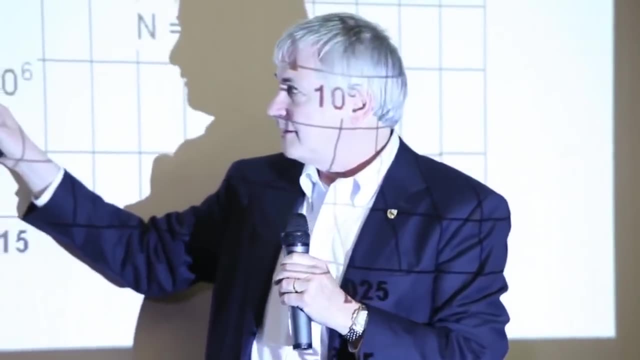 It just keeps going up, But the number of needles is unknown. Carl Sagan figured- I don't know- probably a million, not billions and billions, but a million broadcasting societies in the galaxy. If he's right, then you know, by 2015, we might hit one. 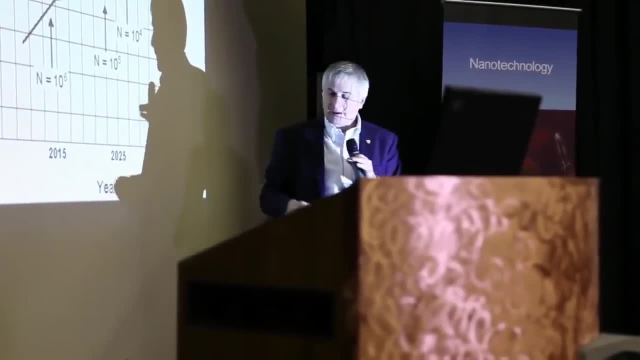 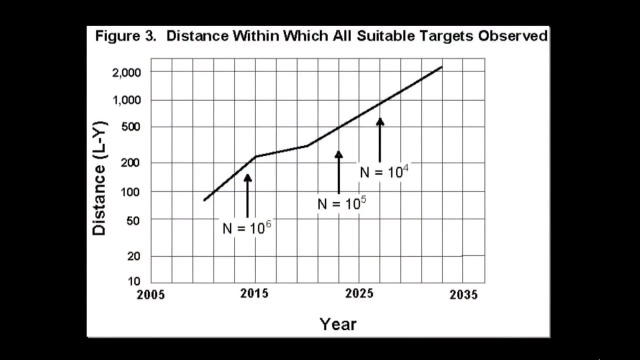 Isaac Asimov figured there were 670,000.. For some reason Asimov was able to compute this to two decimal places. I mean it was brighter than these other guys, But if he's right, then it takes a little longer: 20,, 20-something or other. 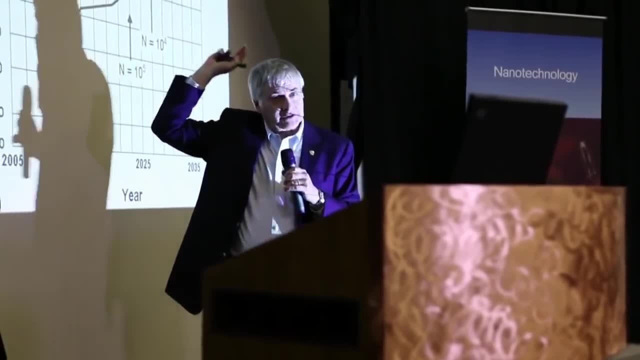 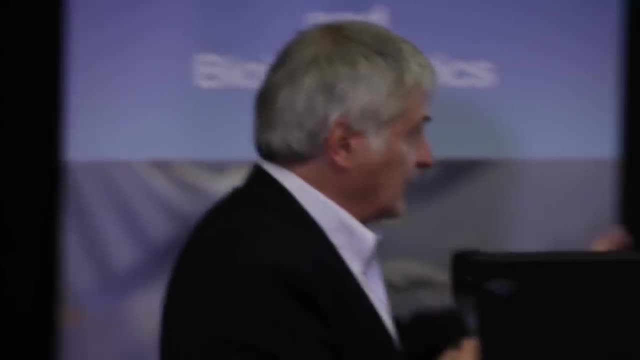 And Frank Drake himself figures 10,000.. Now these are called estimates, But in this case estimate is a euphemism for guess, because nobody really knows. But it is true that this range from 10,000 to a million is kind of the range estimated. 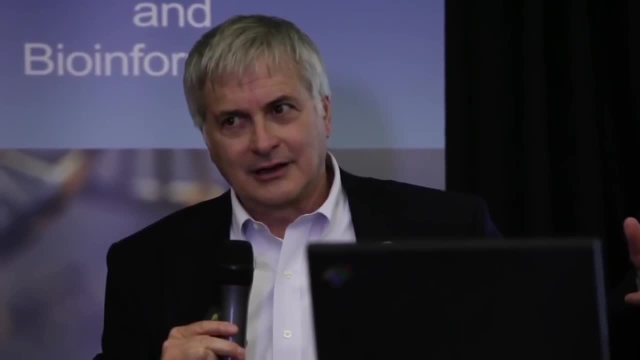 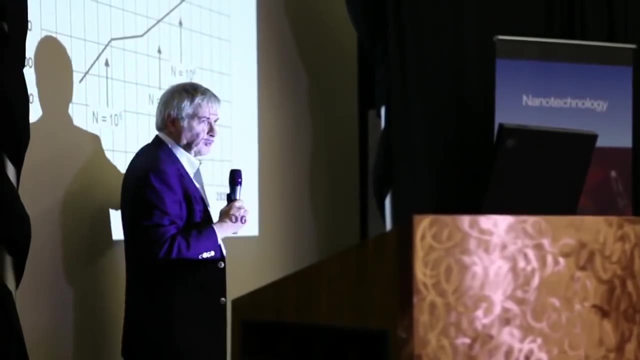 by the people who initiated this whole project, Right? So if this project is going to work- if it's going to work at all, it's going to work before you all become middle-aged. This isn't something that's going to take generations. 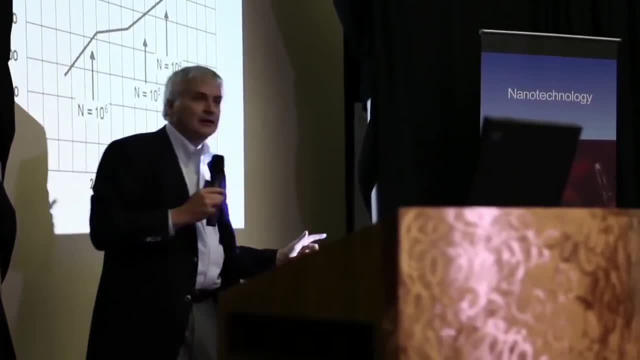 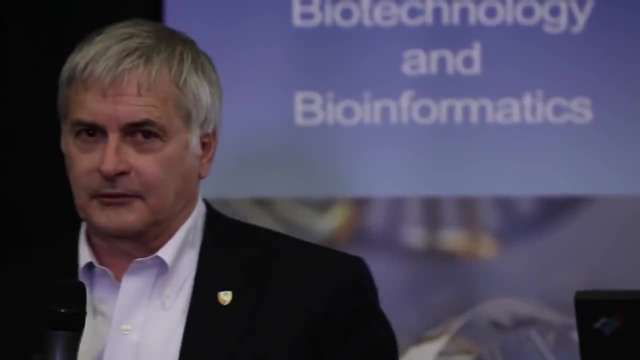 Either it's going to work in the next couple dozen years or there's something wrong, And it could be a lot of things wrong, Right? I mean, it could be that, you know, we need a lot more sensitivity, Or it could be that we're looking at the wrong part of the spectrum. 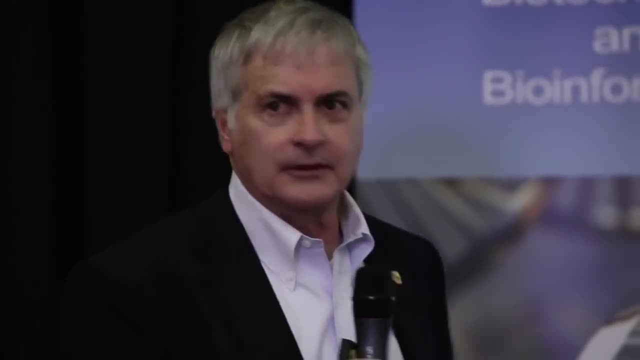 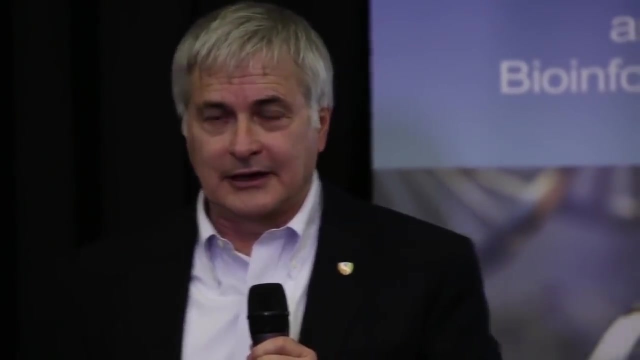 Or it could be that they aren't out there, Or it could be that they're not using radio, Or you know. you can make a whole laundry list of things. But if the assumptions that were made 50 years ago have any validity, have any merit, 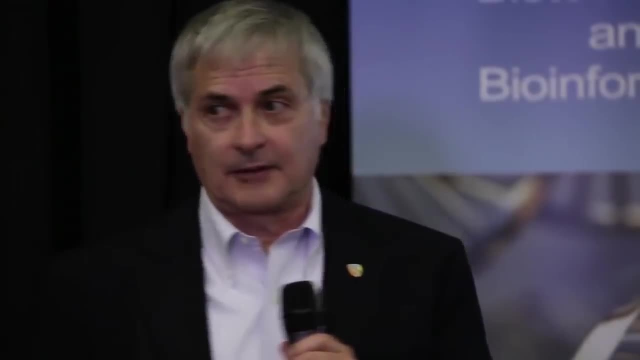 this is going to pay off in your lifetime. It's going to pay off in the next couple dozen years. Okay, So we'll find ET within 10,000.. We'll find ET within two dozen years, Assuming we're not missing important physics. 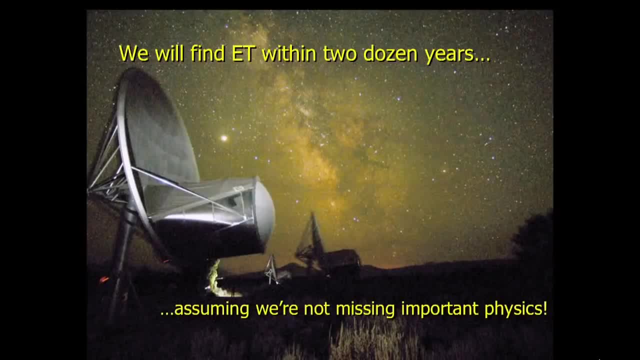 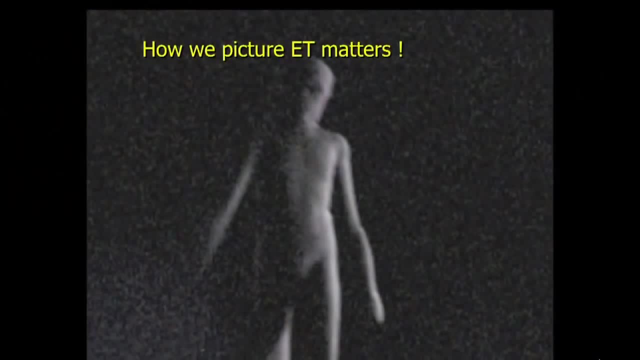 We might be missing important physics. I also said how we picture ET matters. Let me just get back to that, because I do think it's slightly relevant for what you guys do, And that's this: We've always assumed that ET was carbon-based. you know complex molecules. 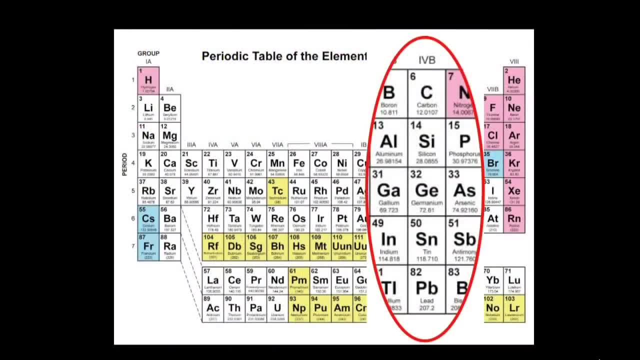 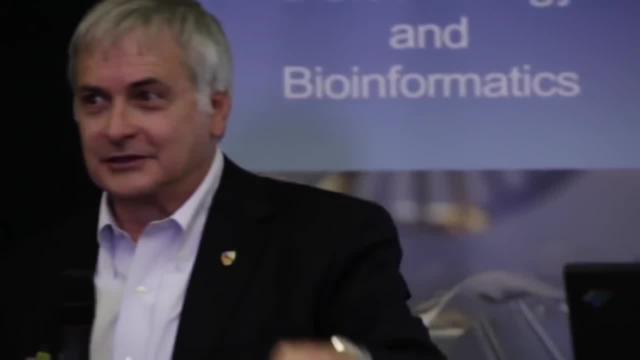 There's a periodic table. There's carbon up there. Carbon: you're made mostly of carbon compounds. Why is that? Is it because there's a lot of carbon out there in the dirt? Well, there is a lot of carbon out there in the dirt. 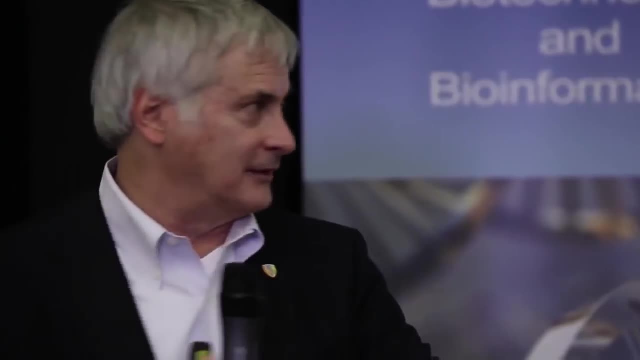 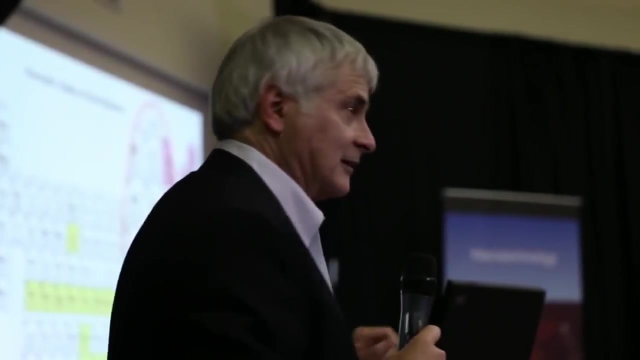 But there's more silicon out there in the dirt than carbon. You're not silicon-based. Could it be an accident? It's not an accident. Carbon has four covalent bonds. It's a small atom, smaller than silicon, So you know it hooks up. 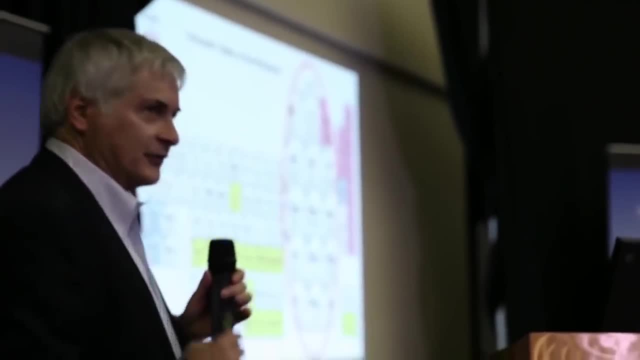 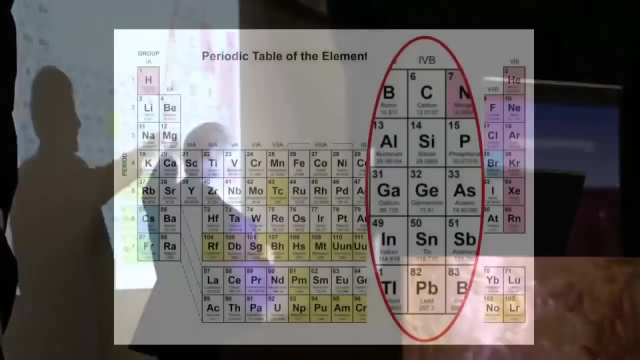 It makes interesting molecules right, And life is, after all, just interesting molecules. I don't know if you think of it that way when you wake up in the morning, but that's all. it is right. Now you can say: well, yeah, but what about silicon? 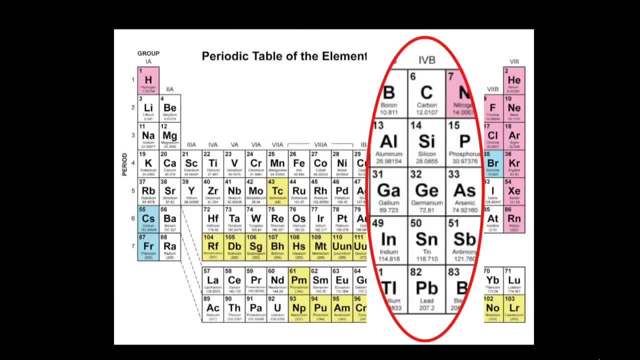 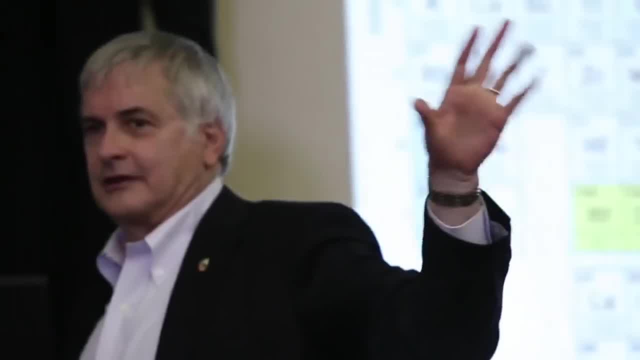 It has four covalent bonds too. Yeah, but it's a bigger atom, The bonds are weaker, and so forth. The atoms- sorry, the molecules- it makes are not quite as interesting. I mean, consider: carbon hooks up with two oxygen atoms and you get carbon dioxide. 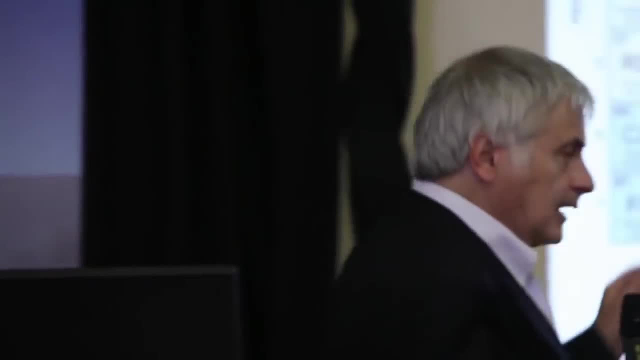 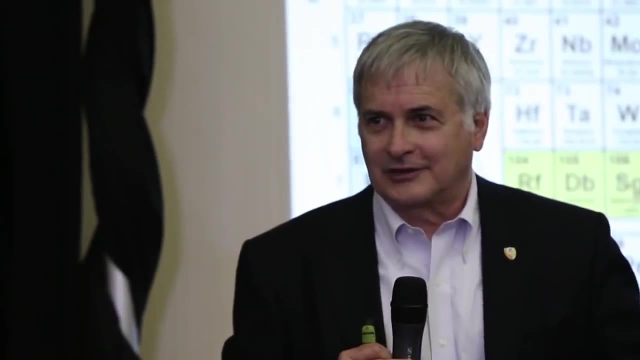 which is kind of useful, particularly if you want to, you know, heat up the earth. You take silicon and you connect it with two oxygen atoms and you get silicon dioxide, which is quartz, which isn't so interesting for biology, right. 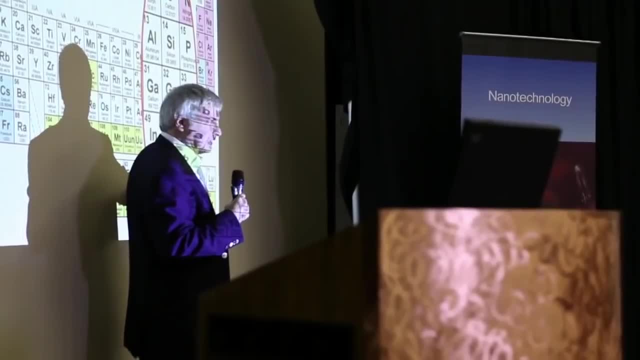 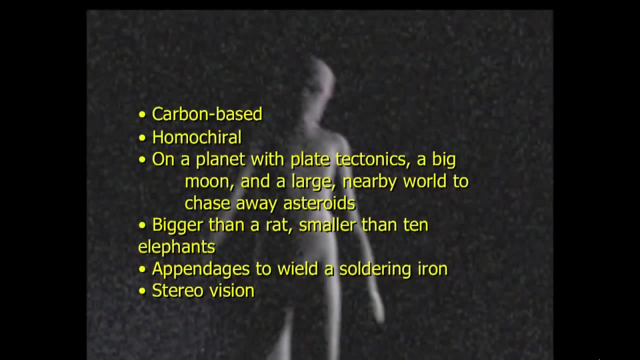 Germanium. even less interesting: Tin tin-based life, Wizard of Oz maybe, I don't know. Okay, so we always assume that the aliens will be and we'll have all these sort of properties that we have. I mean, we could go through them. 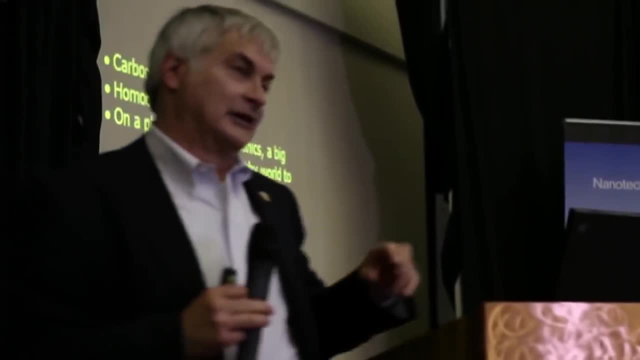 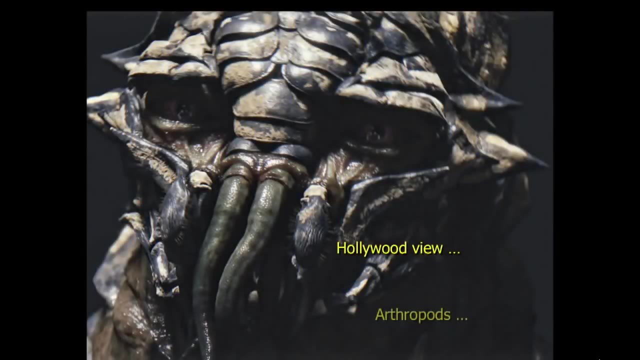 but these are all just simple engineering considerations. We assume the aliens, you know the little gray guys or something like that. Here's well Hollywood view of some aliens. This is District 9.. These aliens come to earth. They're just a social problem. 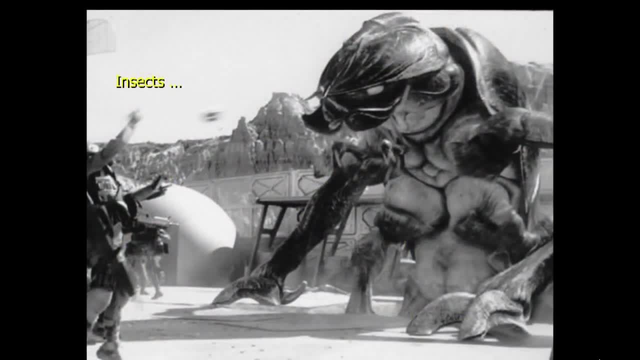 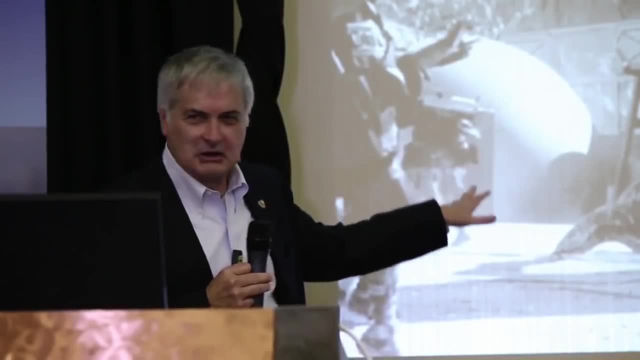 Arthropods And then the starship troopers. remember Paul Verhoeven's film. You know the aliens are bad here. And of course Hollywood knows that you don't like insects, right, Because you know they're annoying. 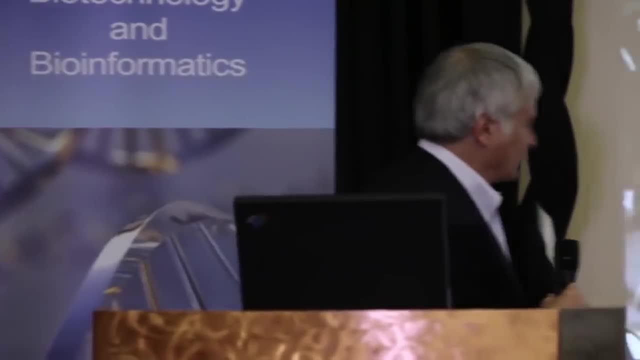 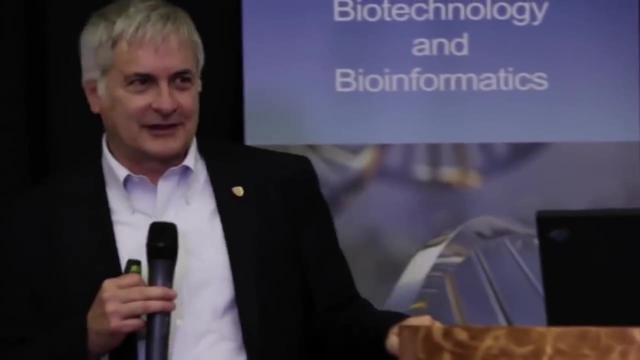 They compete with you for the food supply. They carry disease, Whatever. So he figures: if you don't like small insects, you really won't like big insects. The aliens are big insects. Of course you know scaling laws If you actually made an insect like this. 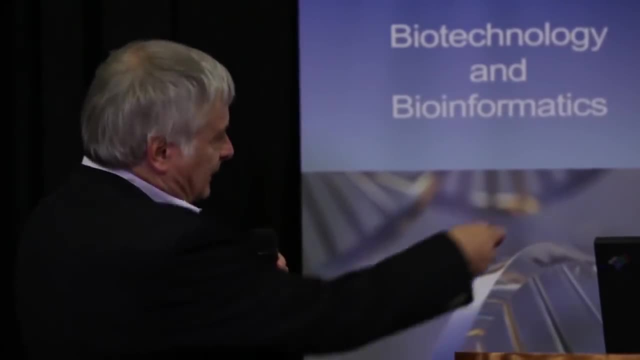 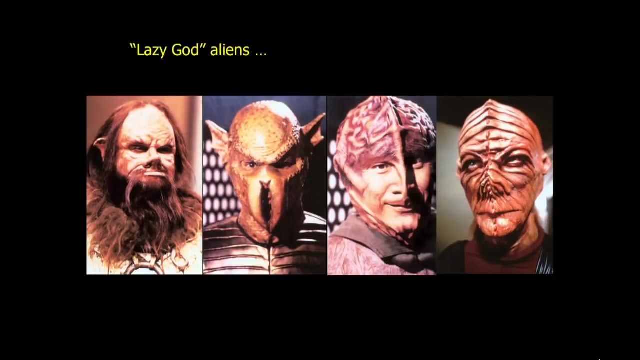 it would collapse under its own weight and you'd have to really awful clean up, But any case did this Hollywood's view. Oh then the I love these, The lazy god aliens. This is the only design that works. 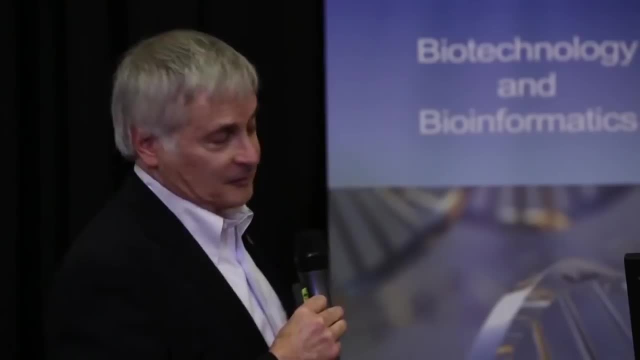 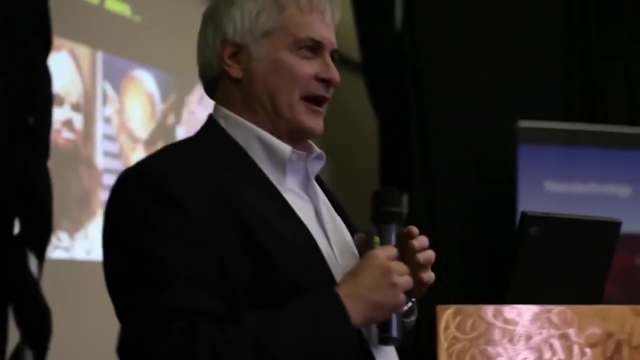 Any one of these guys could walk into a plastic surgeon in Palo Alto and the guy would probably say: I can fix that, So I'm sure they could. You know, a guy like this moves in next door, you know, and eventually you'll invite him over for dinner. 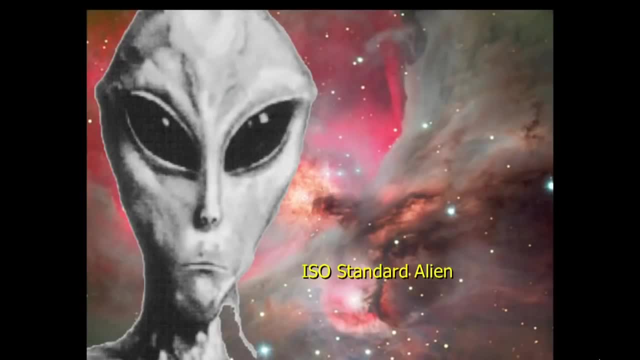 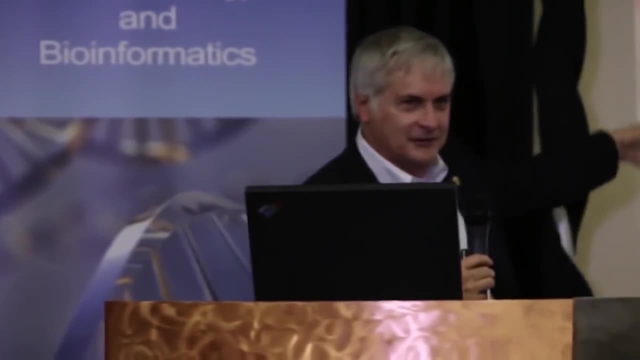 All right Now. these kind of this is your standard alien, And Lloyd Marino has pointed out that this is just a projection of what we think we're going to become right, This is where we're headed: We're losing our hair. 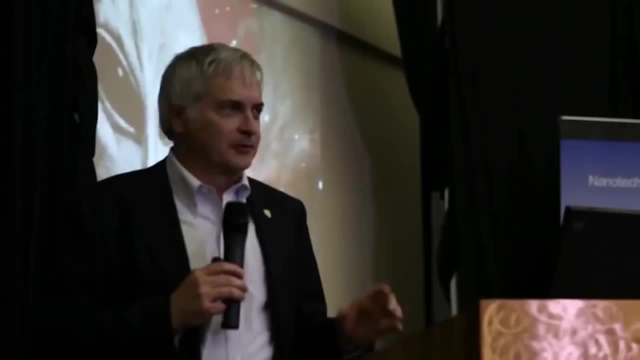 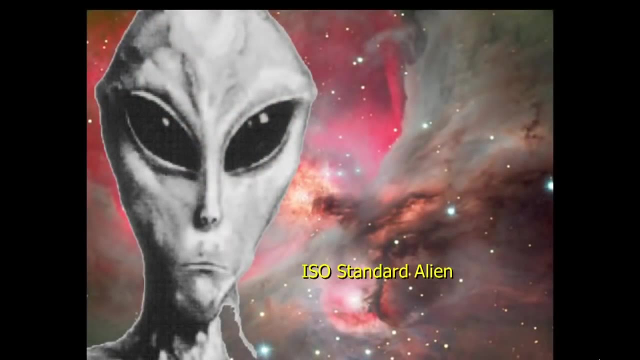 These guys have gone all the way on that. Don't have big noses or big mouths because they've lost their olfactory sense and their dentition And, in fact, by this point, the only real jobs are designing websites. so they have big eyes. 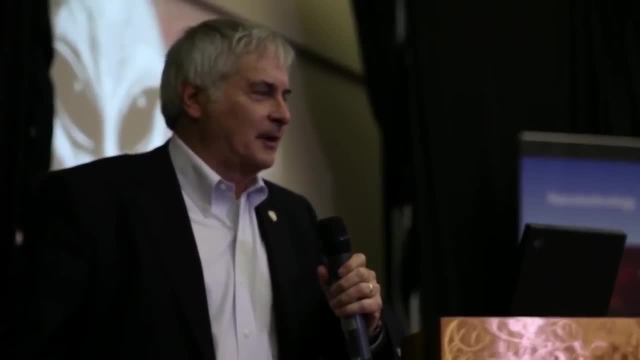 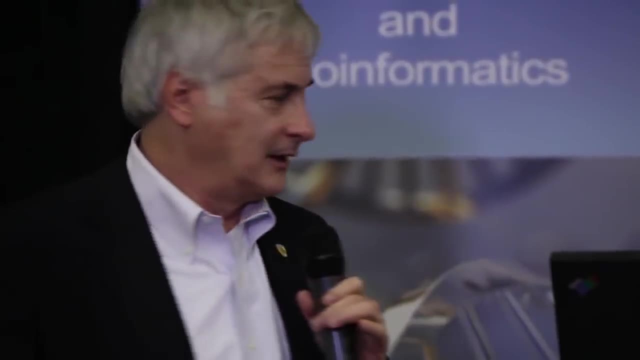 Okay, Well, this is interesting, but it says more about us than it probably says about the aliens. All we're interested in, as far as the aliens are concerned, is that they be intelligent- Intelligent enough to build a radio transmitter. Okay, 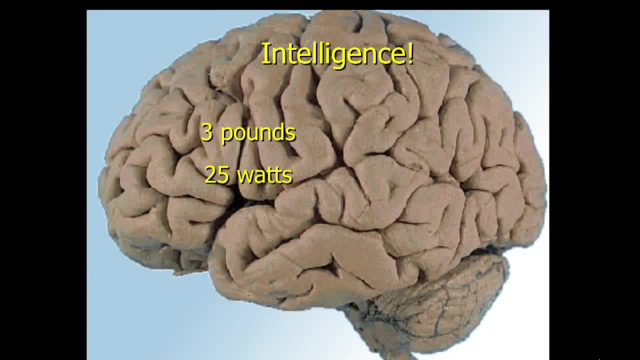 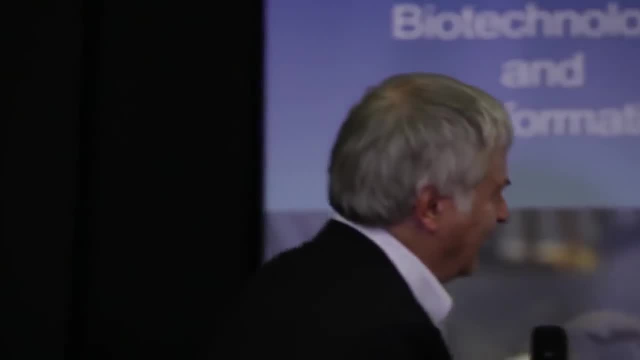 Now that's your intelligence. You've got the little three-pound brain which runs at about the power level of a fridge light. Okay, I told my brother this. You know, I always called you a dim bulb and it turns out you are because. 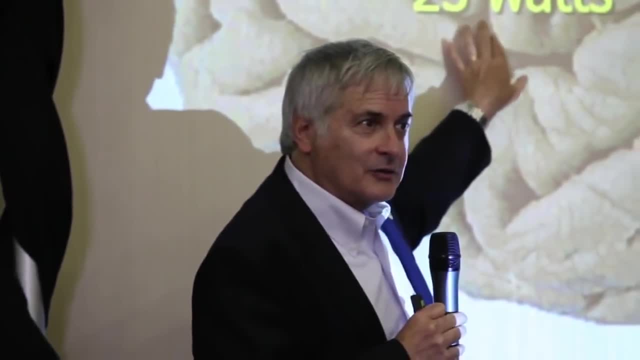 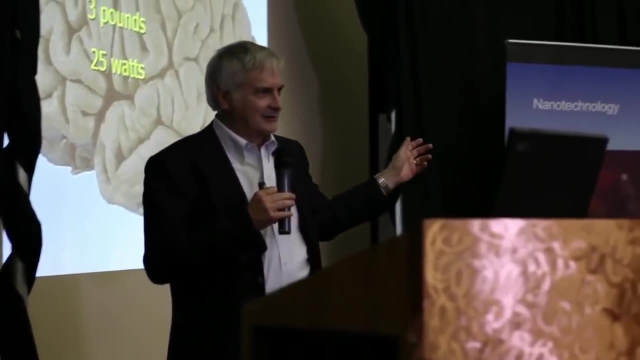 Now, 25 watts isn't a whole lot, but, on the other hand, 25 watts is about one-third of your entire body power consumption. Your body runs at 75 to 100 watts, All right, So what this means. 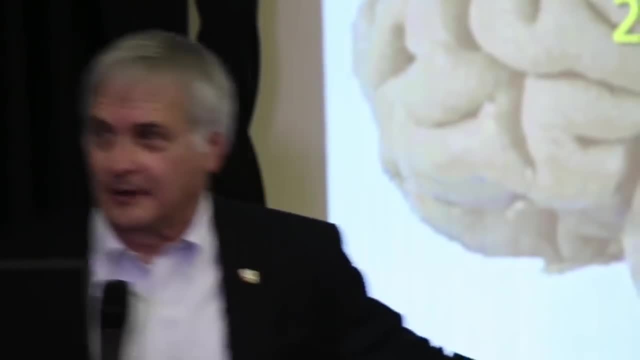 when you go to In-N-Out Burger, one-third of all the calories you eat go to keep your brain warm, despite the fact that, even if you're not thinking of anything- like most of the guys right, it just keeps your brain warm. 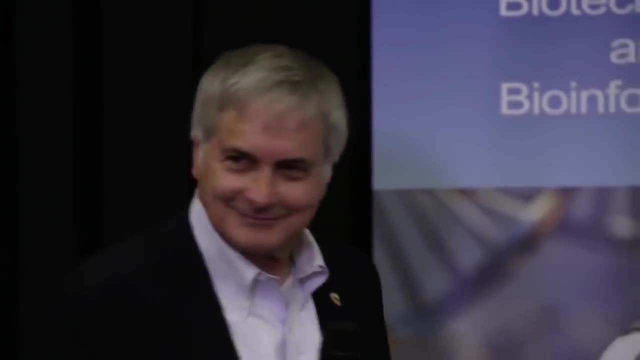 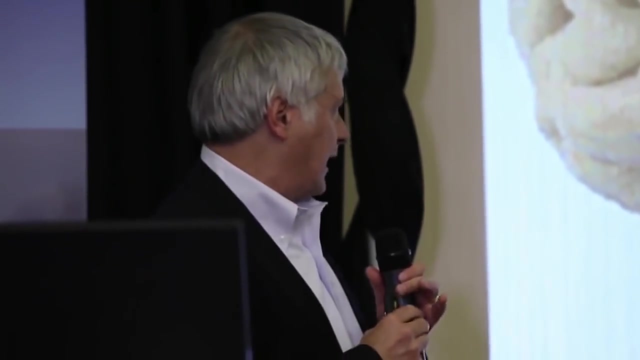 even though your brain is only 2% of your body weight. Very expensive to have a brain, It is Okay. So that's our intelligence. Now you might say, well, yeah, okay, Maybe aliens have the same sort of situation. 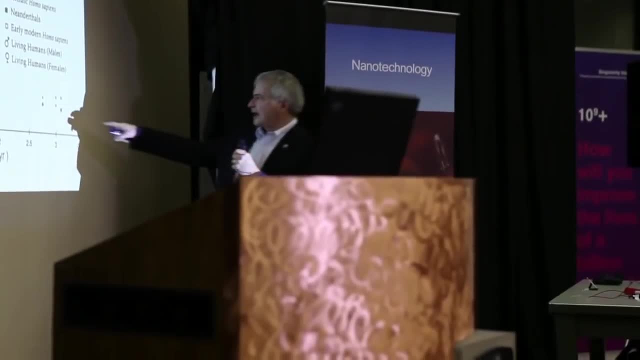 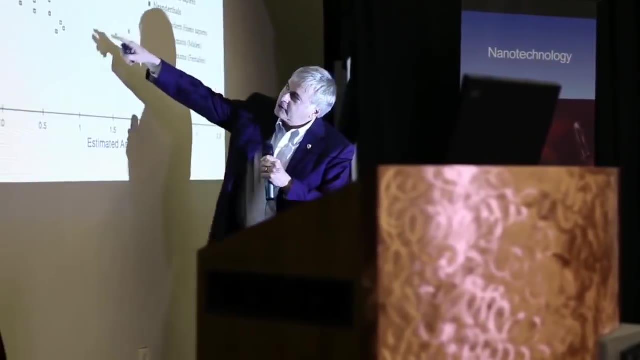 They've just gone to bigger brains, because that's what we're going to do. right? Here's a plot of our brain size versus time. So three million years ago our ancestors had half kilo one-pound brains. A million years ago, 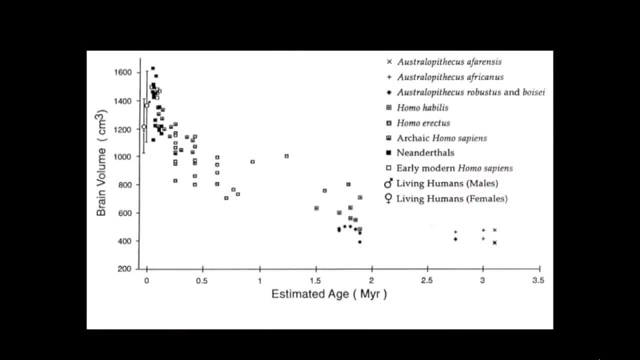 we had two-pound brains and now you have a three-pound brain. Now that last pound was important, because when you have a two-pound brain, you're a forest ape. When you have a three-pound brain, you get tenure at Stanford. 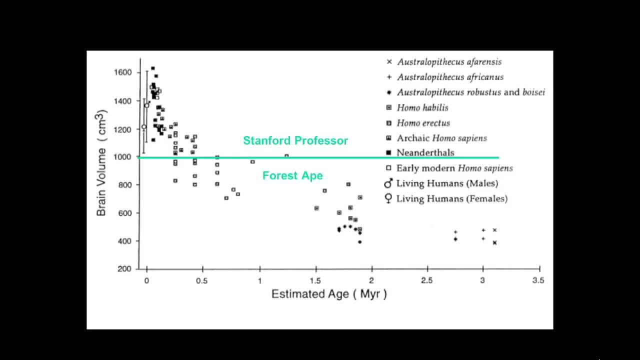 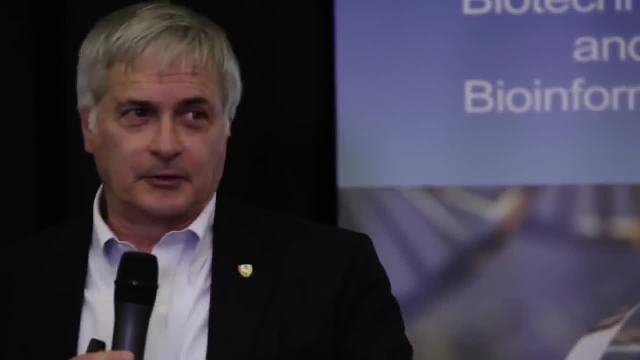 Okay, And the assumption here is that, well, maybe our brains will just continue to get bigger, Maybe, but you know a lot of objections to that. To begin with, the women will go on strike because they have trouble giving birth to babies. 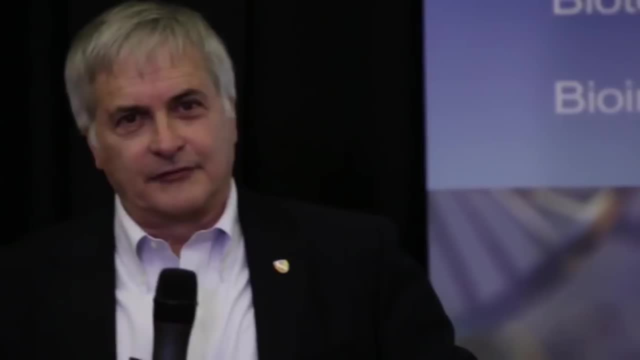 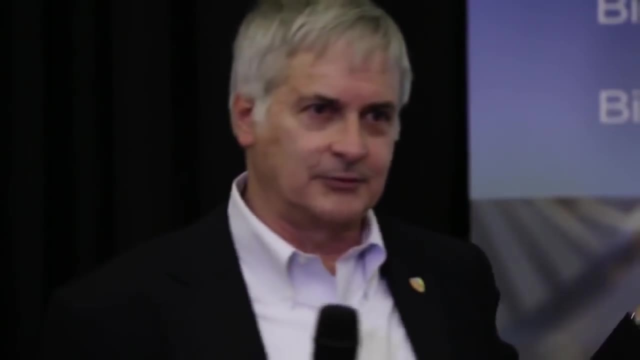 as big as their heads are. now You say you know you're going to have babies that are going to eventually have ten-pound brains. There are also mechanical difficulties with having a very big brain, because you know when you twist your head. 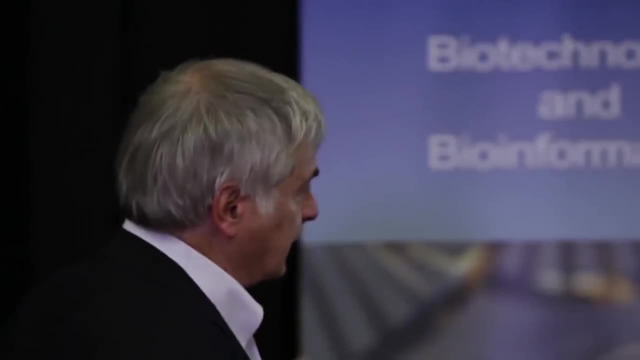 because you want to see what's in the rearview mirror, your head twists off and stuff like that. All these sorts of things suggest maybe that won't happen. In any case, it probably isn't going to happen because of this, This plot. 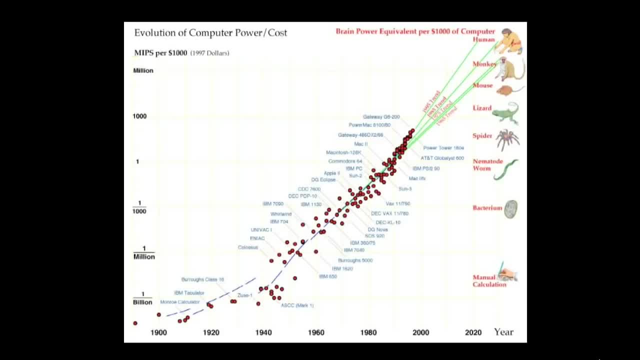 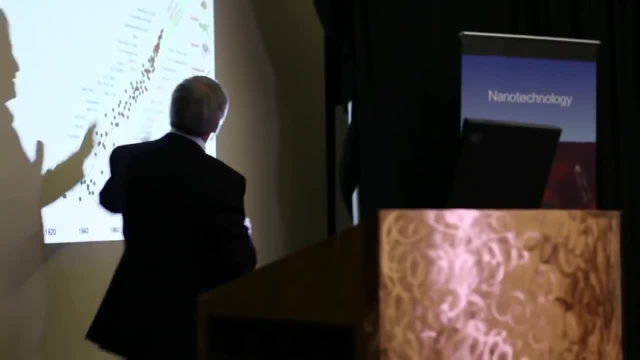 you know Hans Marovitch at Carnegie Mellon. all he did was plot the amount of compute power you can buy per thousand dollars ever since 1900. And of course it's going up exponentially, Headed for the singularity. 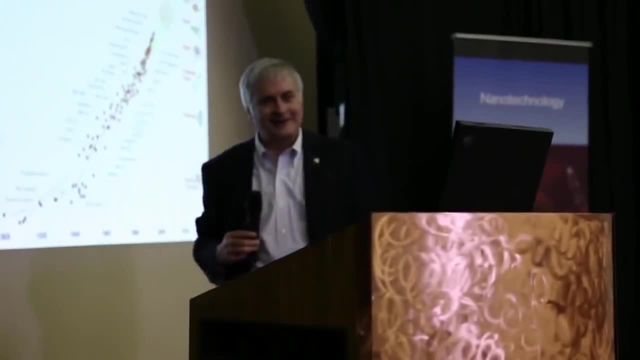 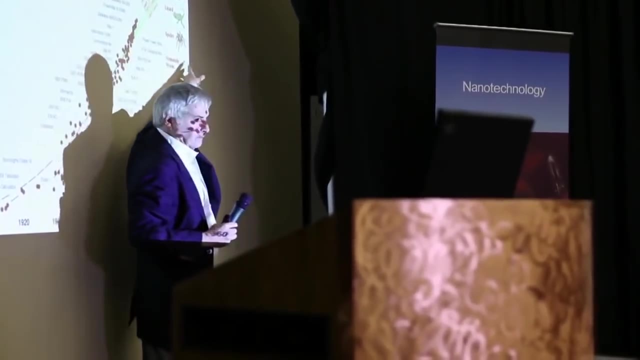 Erity, erity, erity. So so 19, right, I mean a lot of people dispute some of this stuff, but in 1997, for a thousand dollars you buy the compute power of a spider Right. 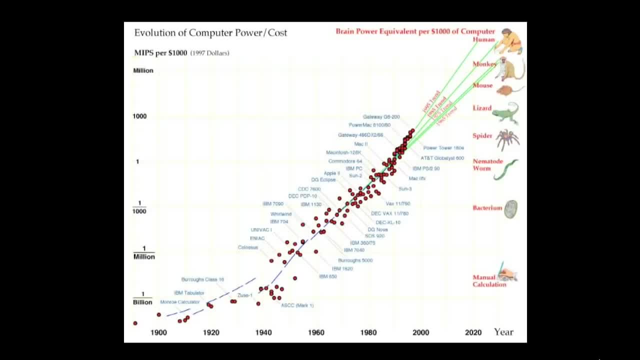 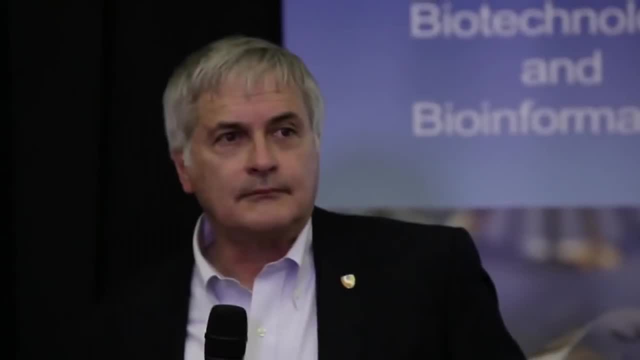 Today- I mean, there's no data here- but in 2010,. okay, if you're selling car insurance or something, And the point here is that by 2020, for a thousand bucks, you buy the compute power of you. 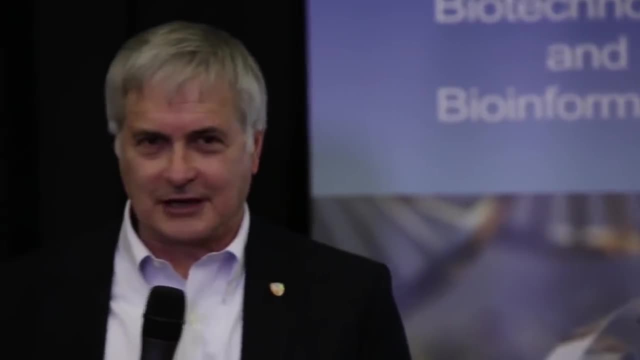 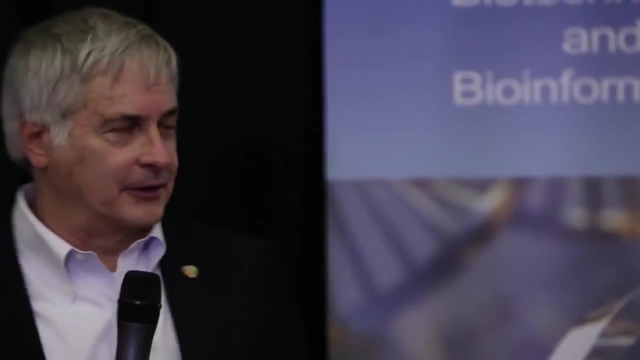 Right Now, of course, it's unclear whether that means you got artificial intelligence, because it takes more than just the hardware, But on the other hand, maybe the software will catch up. This is all your bailiwick, so I won't say much about this. 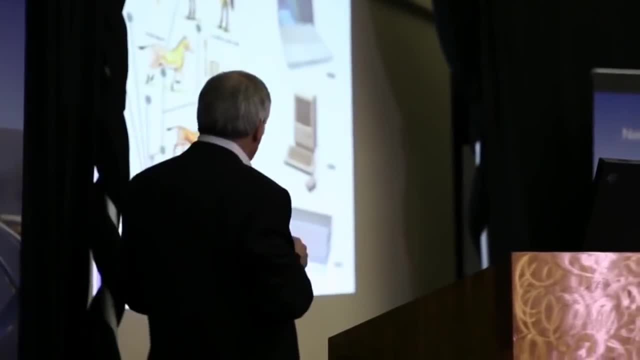 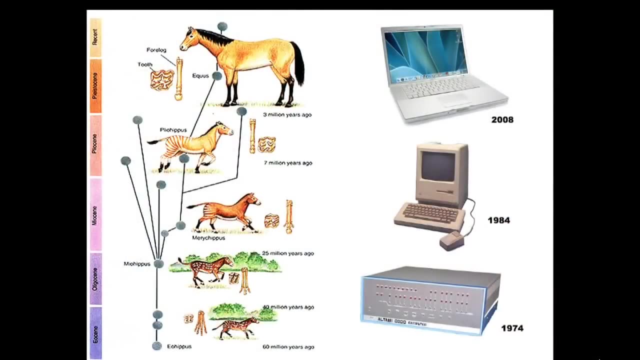 The point is there's a real time scale argument here And this is it, And I just made this little graphic showing the evolution of the horse. What is this? 60 million years ago, a horse was the size of a collie dog. 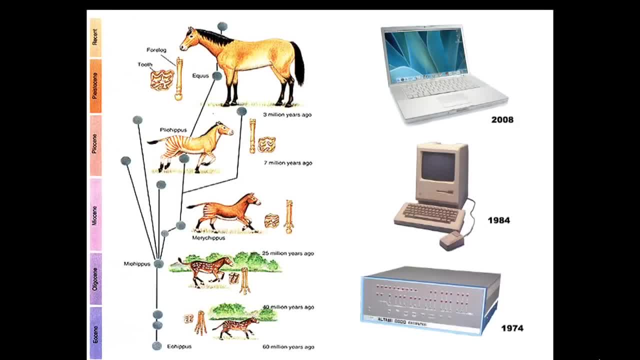 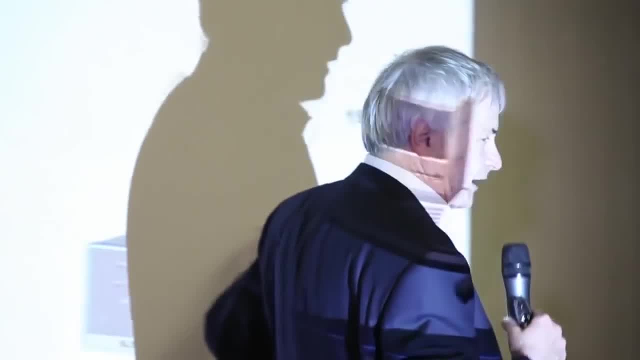 Today, most horses are the size of a horse. Now, that's what 60 million years of Darwin has done for him. You look on the right hand side. I had a 8-bit computer. you know, in 1977 I had to solder it. 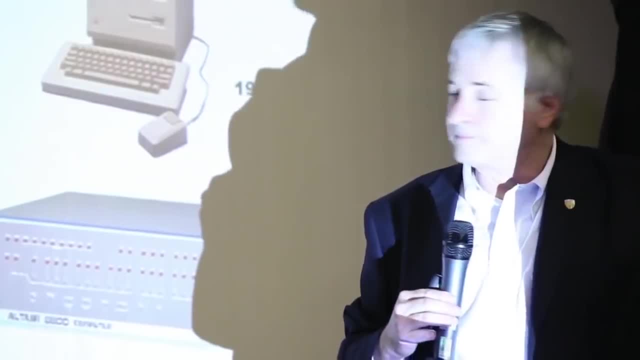 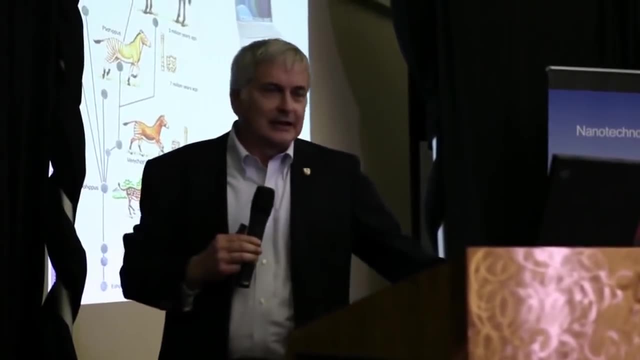 together myself. The computer I have at home today is about: given the bus width and the speed of the processor, I reckon it's 8,000 times faster than what I had in 1977. So in other words in 25,. 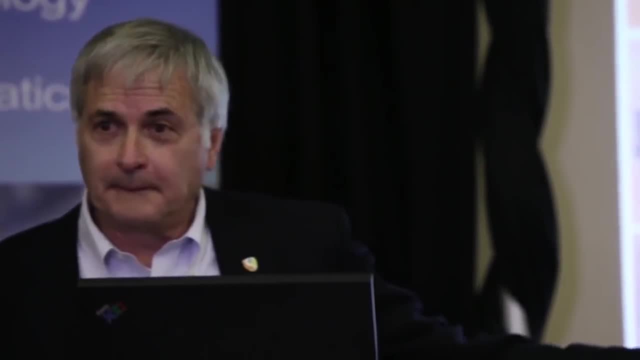 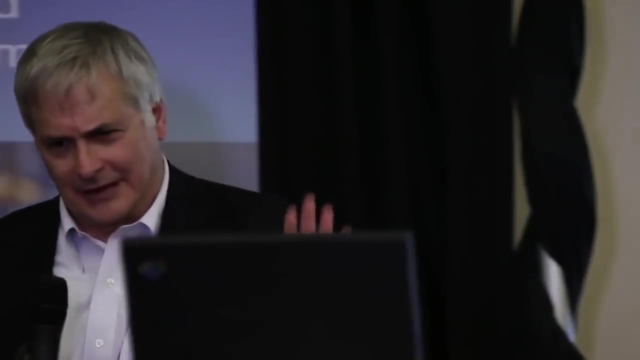 35 years we've had 10,000-fold improvement in computers In 60 million years. we took a horse from this to that. Right, I don't have to hammer you with this. The point is it's only been 100 years. 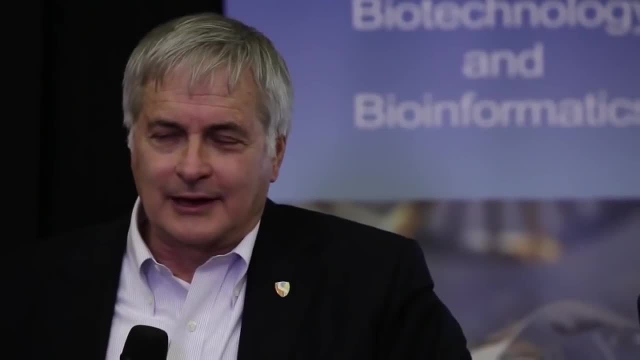 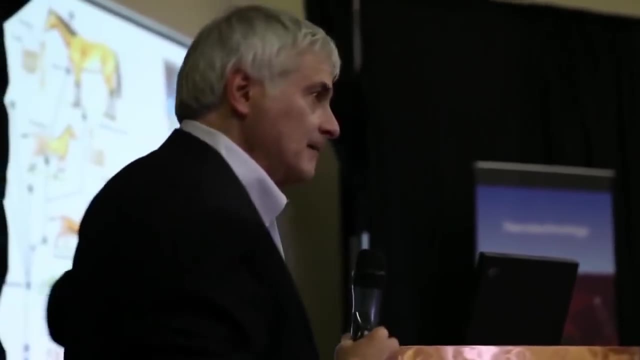 since we invented radio, Right? So imagine the aliens invent radio so they can go on the air and we can hear them. But 100 years after that, 200 years, whatever number you want to choose, as long as it's not unreasonable. 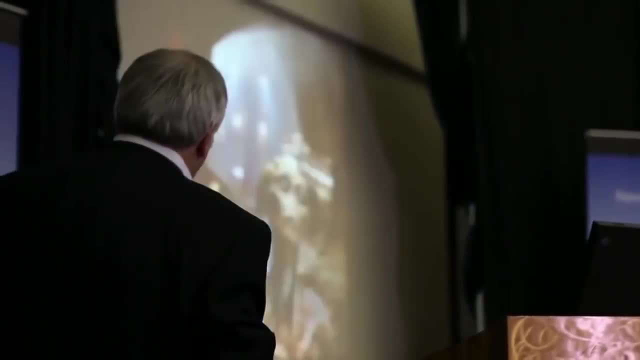 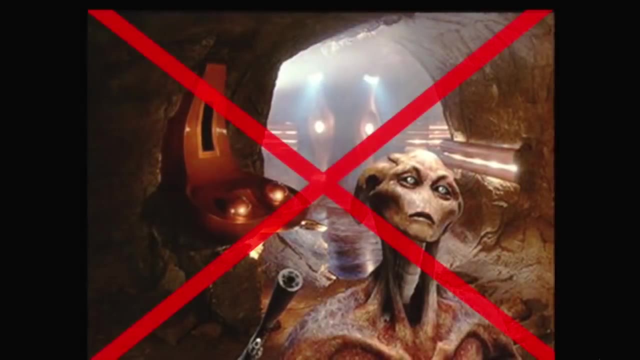 they invent their successors, Right. That's presumably what we're doing in this century. Okay, So the idea that you have aliens that are sort of soft and squishy guys like this just doesn't make any sense, because that's very unlikely. 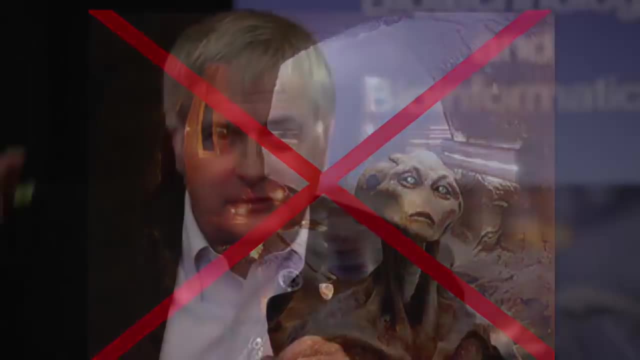 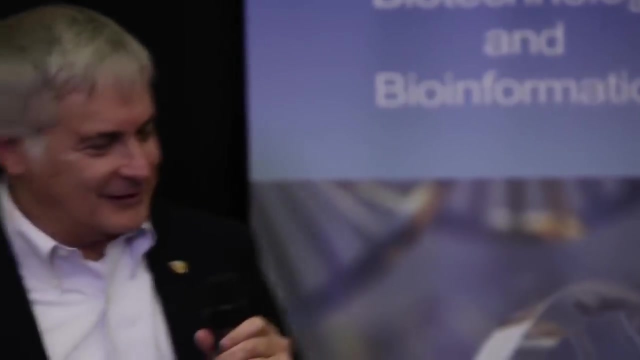 You just happen to catch them when they're in that short interval between inventing radio and inventing something that's a little bit better Right Now. I suggested this up at the University of Washington once and one of the undergrads said: but 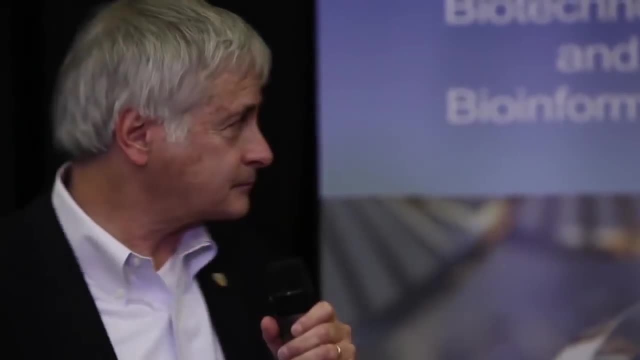 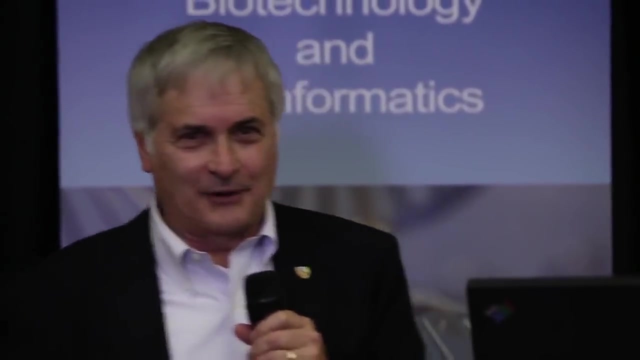 if you invent thinking machines, won't they kill us? And that's the natural optimism of youth, of course. But I, you know. I said, look, I've got goldfish at home and I don't wake up. I'm smarter than they are. 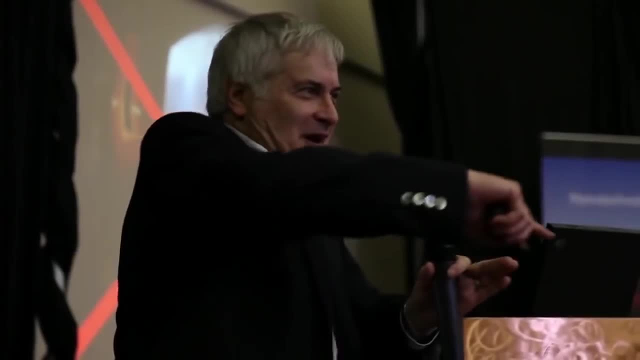 but I don't wake up in the morning and say I'm going to kill those guys. So I don't know, I don't need, I don't mean to say, what I'm going to do is when the computers get really smart. 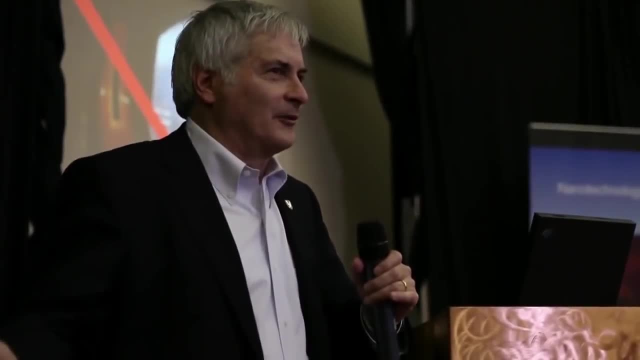 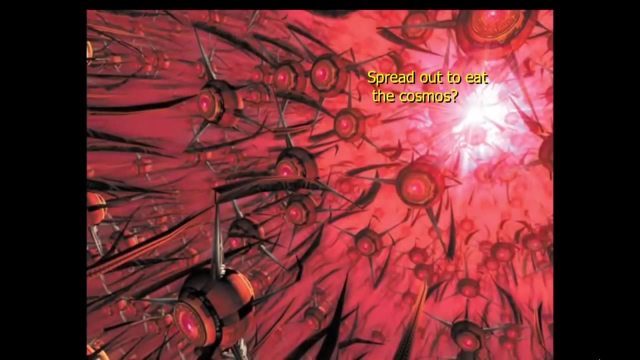 I just turn the keyboard around, you know, you type whatever. That's a whole issue that you all can deal with. My only point is that I don't think that the aliens are going to be little soft, squishy, gray guys. 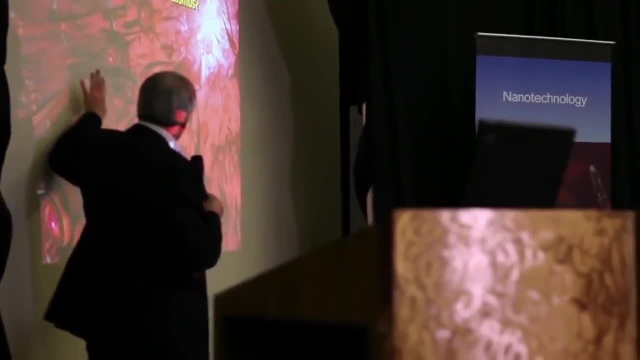 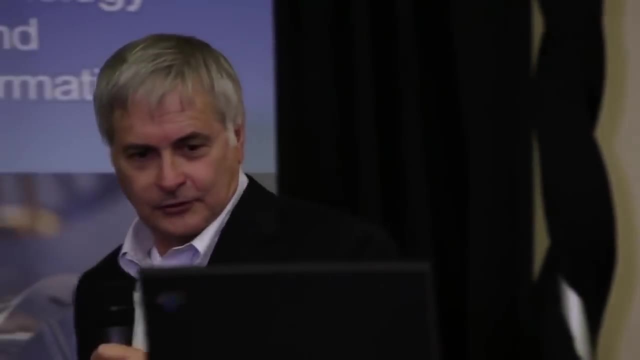 You're going to find some sort of machine intelligence Now. Kurzweil came to the set a couple of months ago. you've all heard from Ray, and Ray thinks they're all going to be, you know, nanobots. 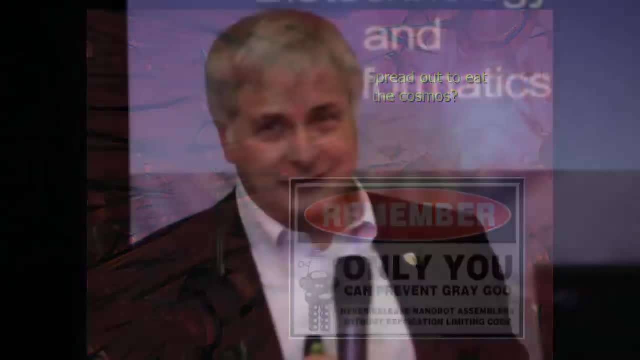 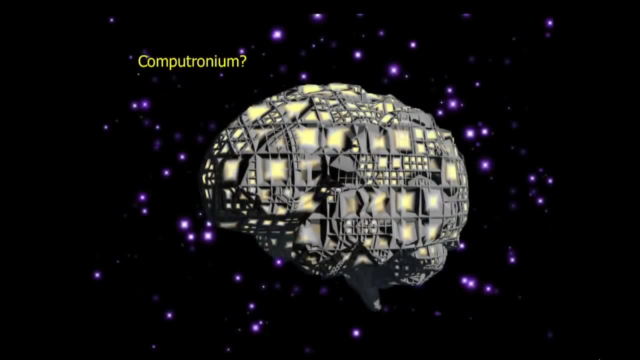 It'll be distributed intelligence, that sort of thing, out to eat the cosmos, right? And you know, maybe that makes sense, You tell me. It seems to me that that's a little less likely than putting as much of the flight time. 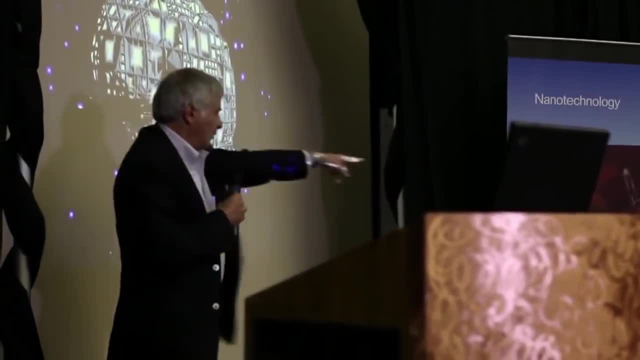 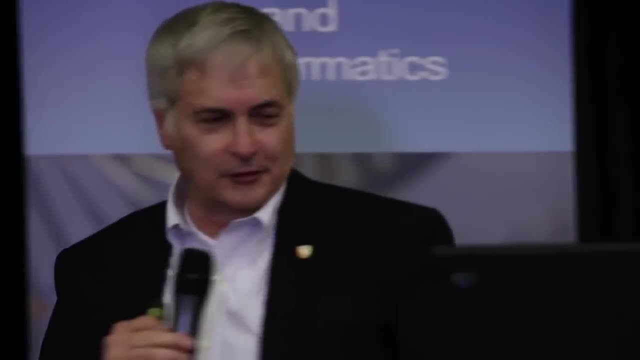 you know, between different parts of the intelligence. You don't want something way over there, when you know when you're trying to think fast. so maybe you just build it all out of computronium, which is from the next planet. 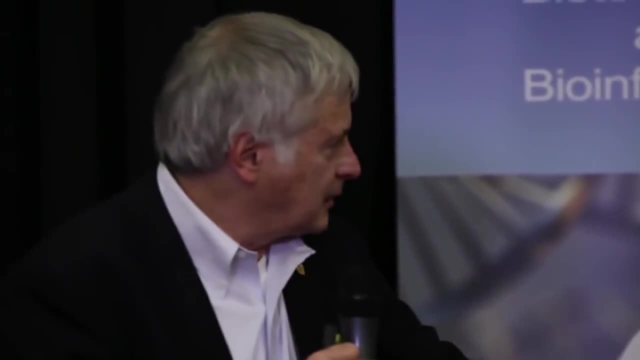 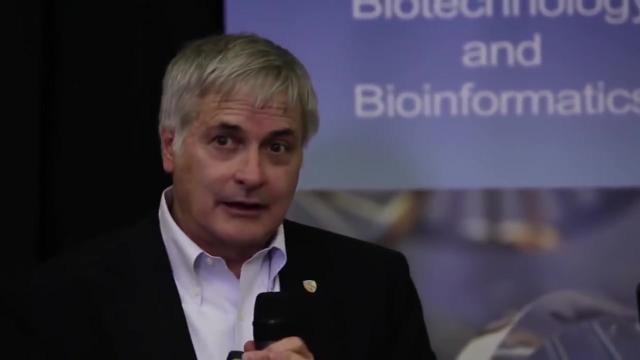 the next moon over from the Navi, I guess. Computronium, The maximally compact computational material, computronium- Ask Ray about it. Hey guys, I don't know, but I do know that, if this is true, this is. 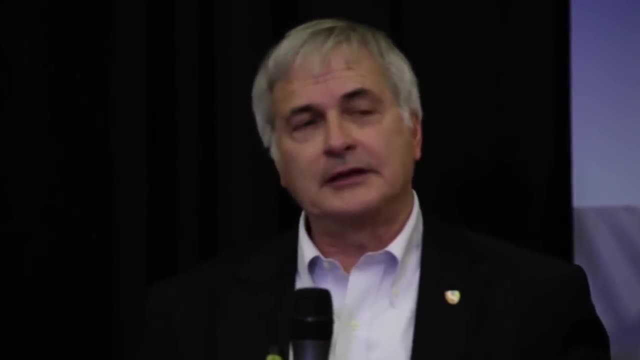 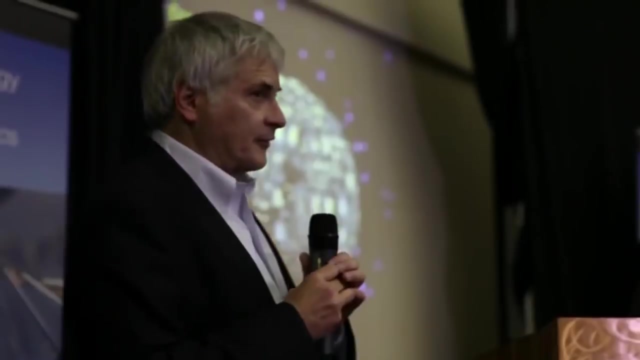 as I say, a very simple time scale argument. The idea that we should be looking for ET on, you know, Earth-like worlds, watery worlds, with thick atmospheres and conditions, sort of like here, may be very, very provincial. Where would synthetic 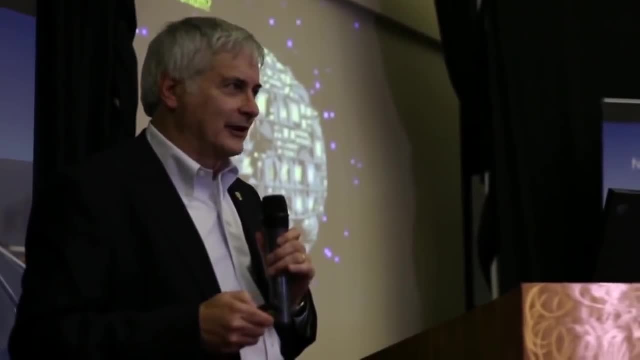 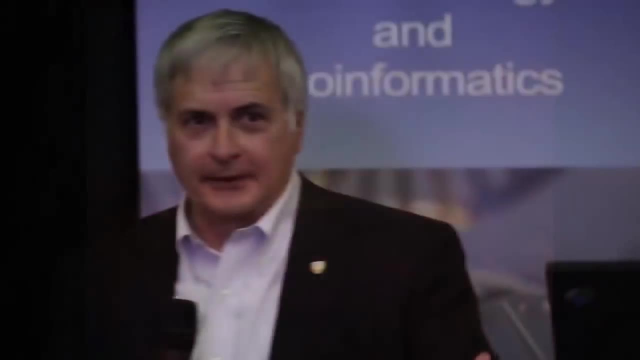 intelligence go, And I don't know the answer to that. If you know the answer to that, send me an email, because I'd like to know. The only thing I can think of is when you ask: what would they find important? Right? 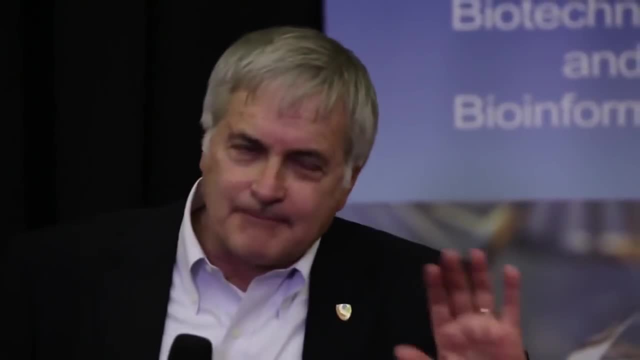 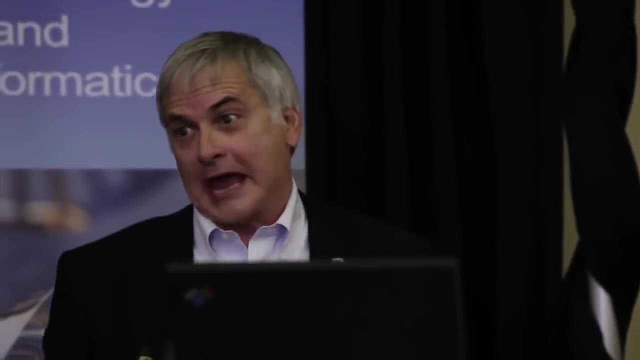 What do you find important in life? I know you're all thinking sex and money, but it's actually matter and energy, which you know matter and energy. if you want matter and energy, this part of the galaxy is okay, but it's not great. 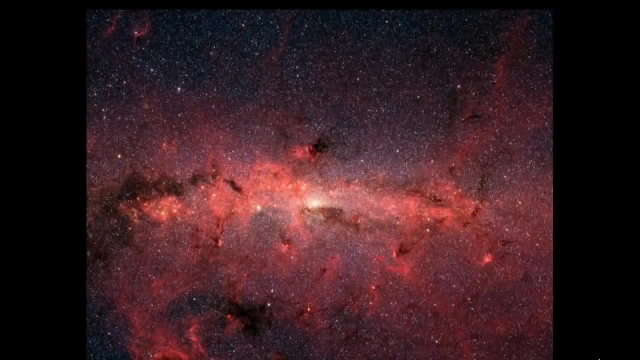 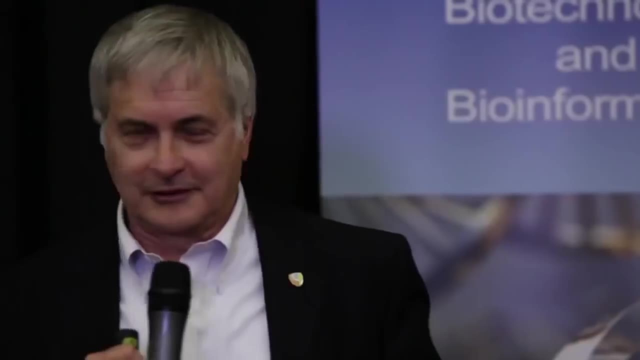 You probably would go to some place where there's a lot more action, like the center of the galaxy seen in this little infrared photo. Okay, And so maybe we really ought to spend a lot of time looking at the galactic center. It's kind of unfortunate. 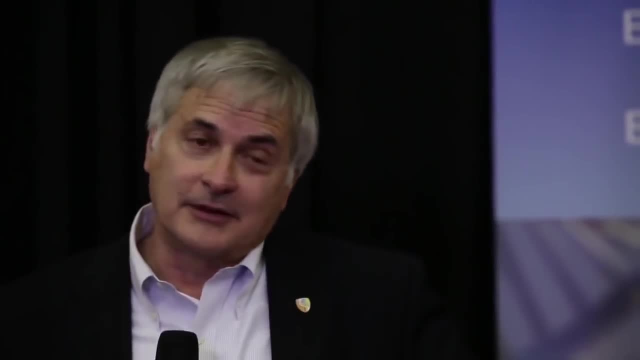 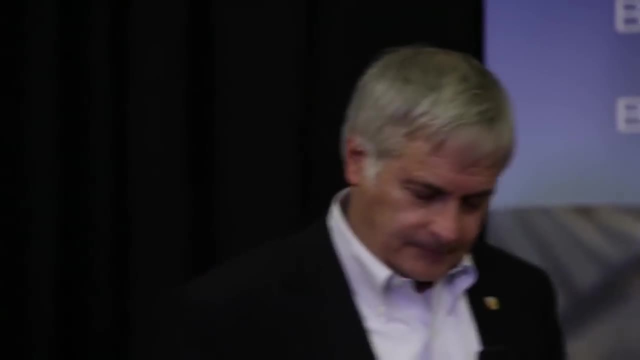 that it's in the southern hemisphere, but hey, Because that's maybe. I mean, there's been plenty of time for truly advanced machinery of any sort to get there, And maybe that's where the signals are coming from. Well, I think I'm going to. 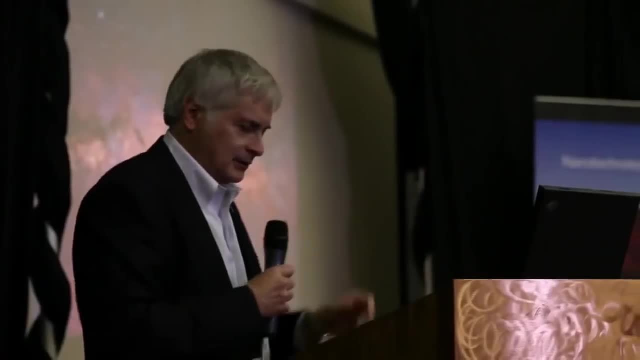 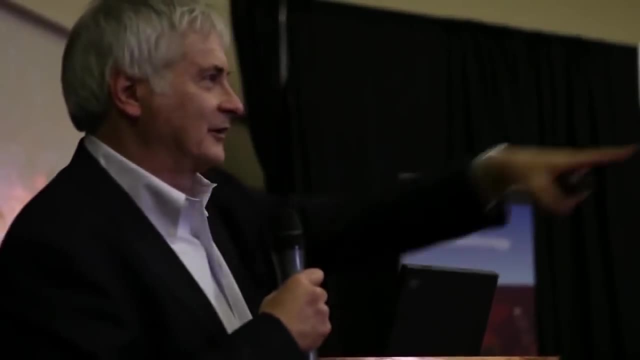 stop it there and ask those questions that you know I've deliberately avoided going into because I've spent too long on this. So is anybody conscious who wants to ask a question? Yeah, I just wanted to hear your opinion on the wow signal. 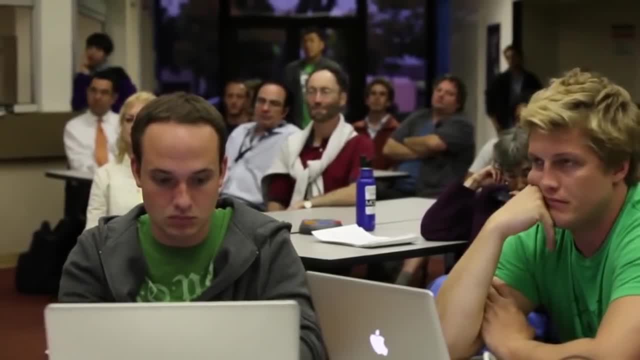 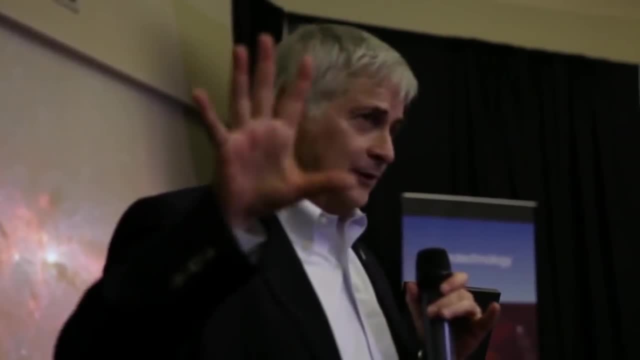 and also, do you agree with Stephen Hawking that we should not be trying to contact? Yeah, The wow signal. The wow signal was found in 1977 at Ohio State University. What happened is they had a big radio telescope there. that wasn't terribly. 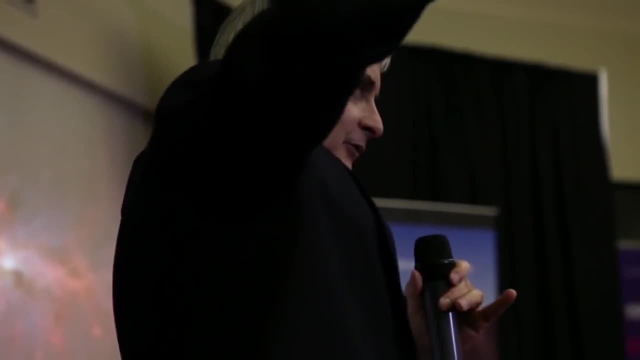 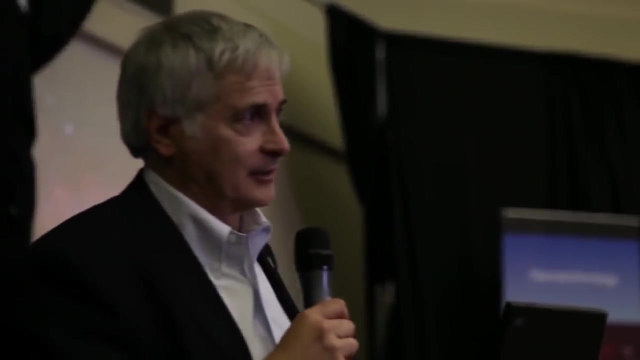 useful for radio astronomy. It was in Ohio, in Columbus, Ohio, and the Earth would rotate, as it turns out it does, And you know, it would just sort of sweep the sky past this, And every morning one of the astronomers would go into the shack. 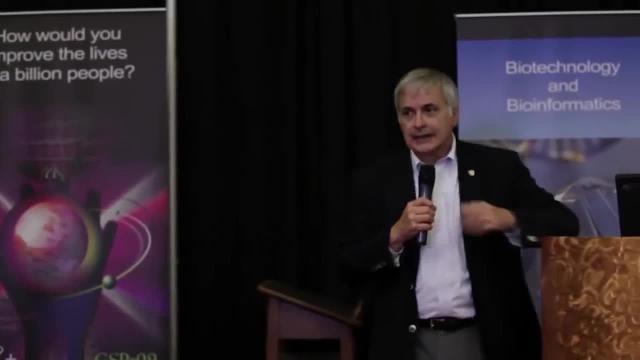 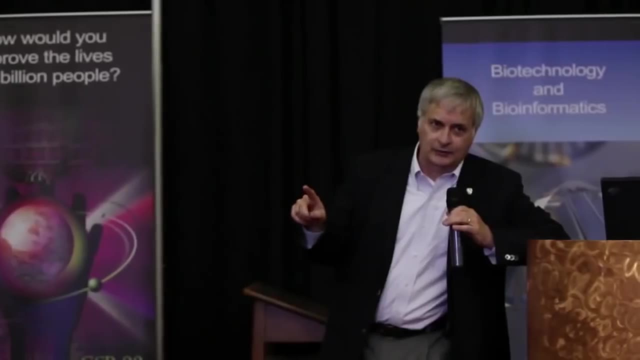 where they had the computers and would look at the printout. In those days, computers, computer output was printout And he was going through the printout one day and he finds a signal that looks very much like what you expect from an extraterrestrial source. 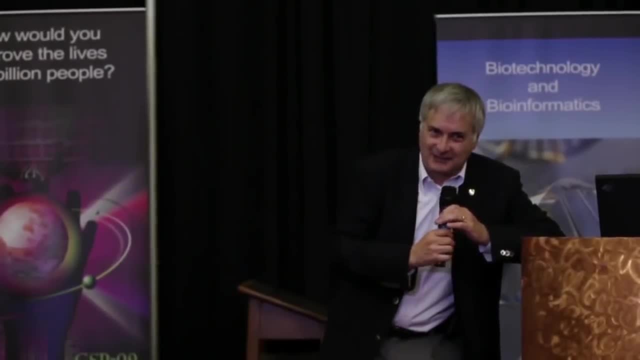 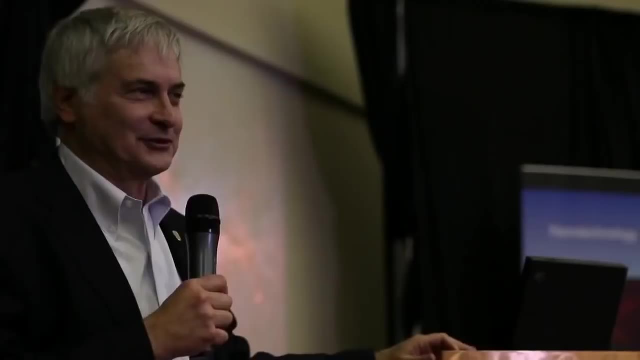 And he wrote wow next to it. That was brilliant. to have written wow next to it, because there had been thousands of such signals Right Calling it wow, was truly a bold stroke, a brilliant stroke, And it's become famous. It has all the characteristics. 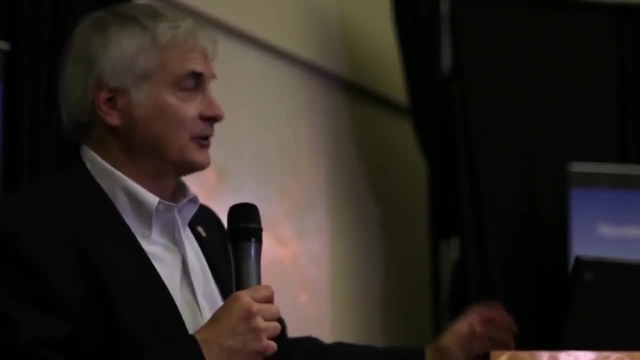 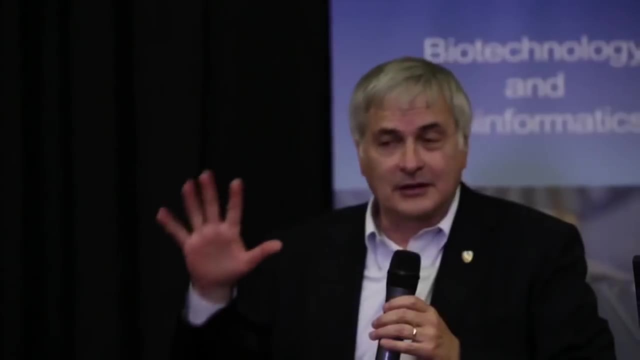 of a signal coming from beyond Earth, But I don't think it was ZTE, or in any case, it doesn't matter whether I think it was or don't, because that telescope had a second receiver on it which automatically looked at the same spot on the sky. 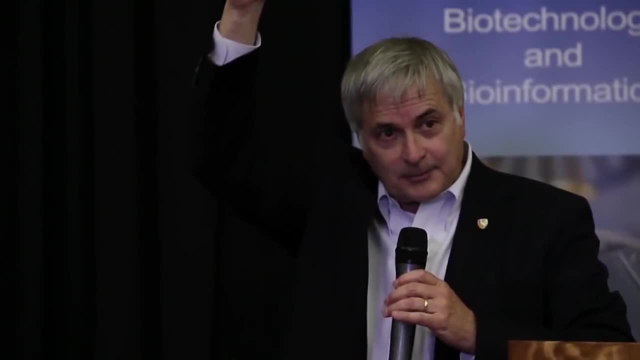 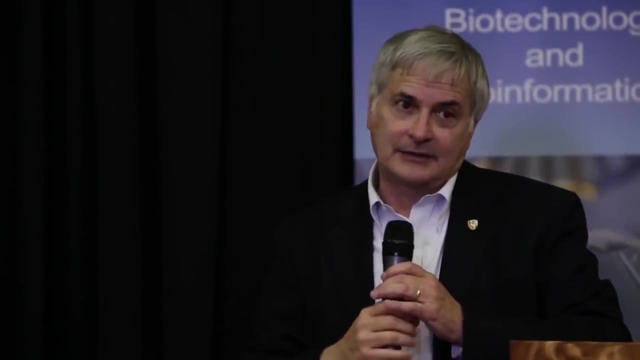 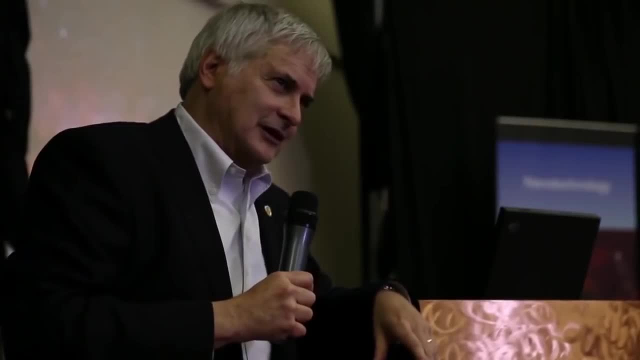 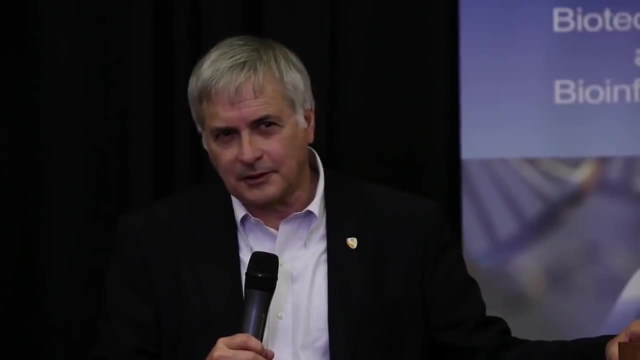 you can say, well, I don't know what it was, and maybe it was ZTE, and then he went on vacation. I mean, you know, could be, but that's not science. So that's so much of the wow signal, The other part. 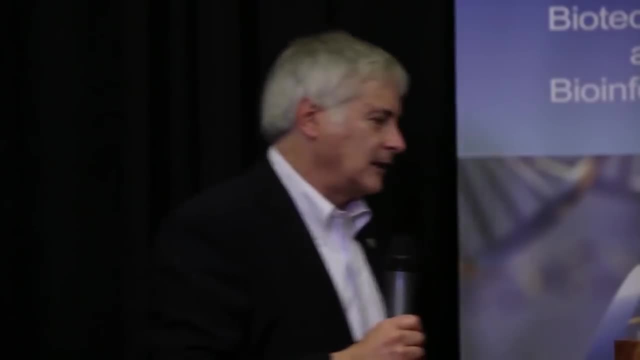 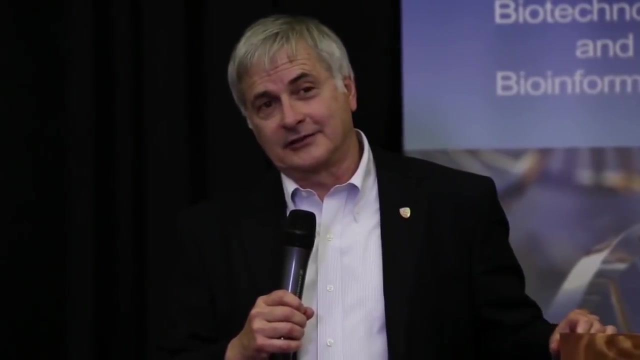 of your question was: Oh, Stephen Hawking, yeah, yeah, did you all hear this? It was like about a month ago when the Discovery Channel had this show about Stephen Hawking and they resuscitated a statement that he had made, maybe in one case. 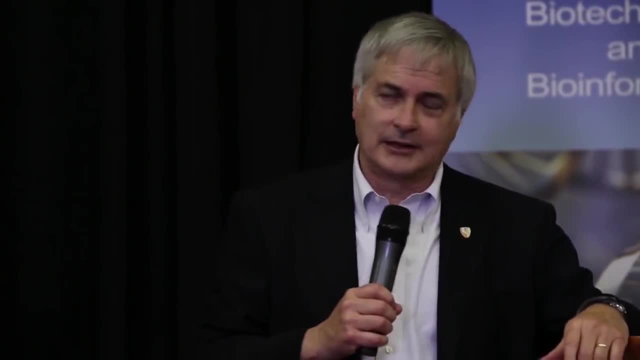 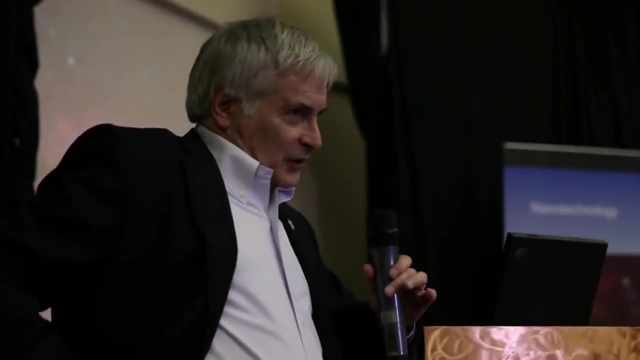 I think he may have made this statement. contact with ET might not be a good idea, because consider what happened to the North American natives when the Europeans first visited them. It didn't work out so well for them, and that's certainly something you can learn from our own. 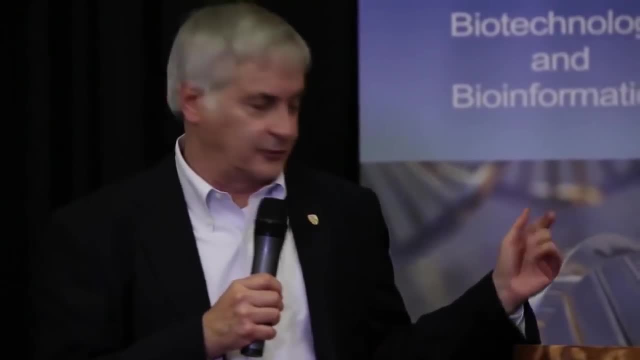 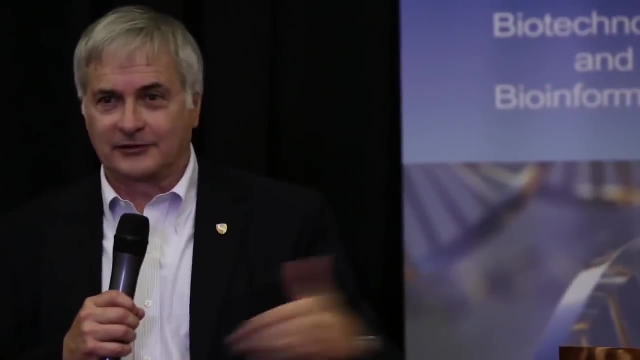 history. I mean, you look at even Captain Cook, who was under orders from the British Admiralty not to interfere with the societies he found in the South Pacific, but nonetheless he destroyed their culture simply by sailing into their lagoons with these ships that had really nifty things, like the wheel. 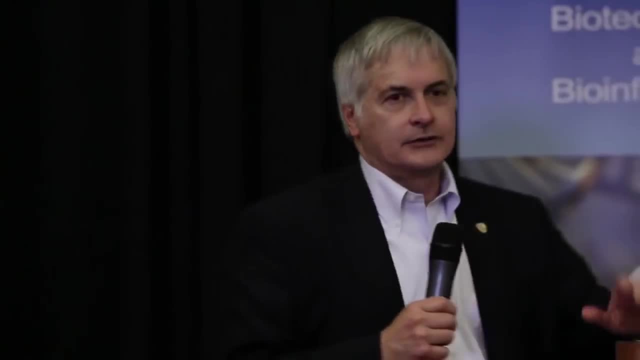 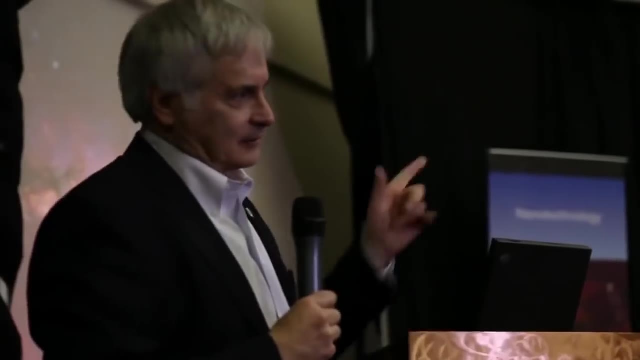 and metal and syphilitic sailors and all that kind of stuff. They figured whatever mojo these guys have is better than ours, and they immediately became converted and their own culture was subsumed into Western culture to a large extent. So that's all that. 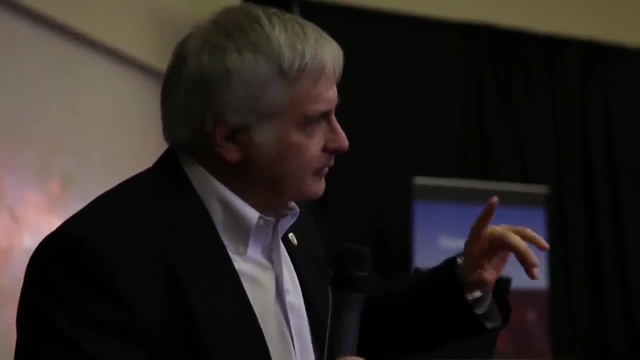 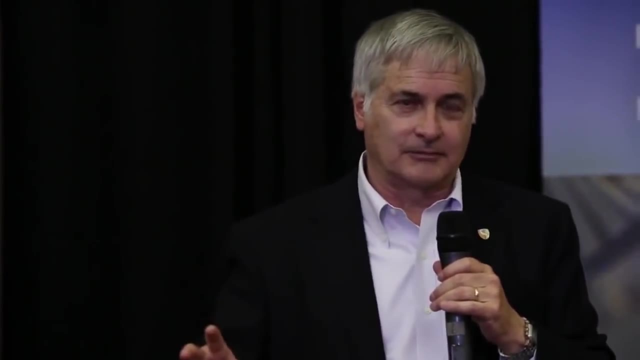 Hawking was saying: Look, beware. Well doing SETI, there's no danger there. You're just listening. You tune in your local radio DJ and he doesn't jump into the car and start molesting you because you tuned him in, but he doesn't know that. 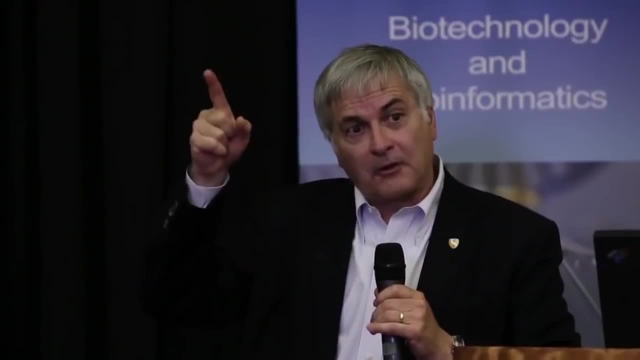 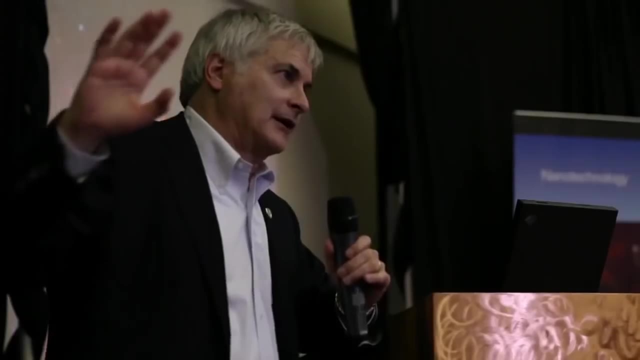 You don't know that. but what Hawking is saying is: but don't broadcast anything back, because that's like shouting in the jungle: You don't know what's out there. You know, maybe it's a very, very small probability that anything malevolent is out there. 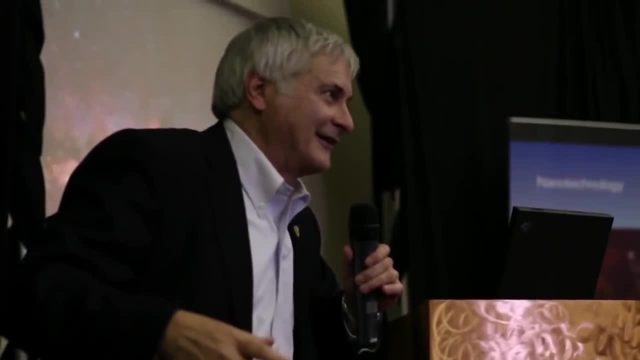 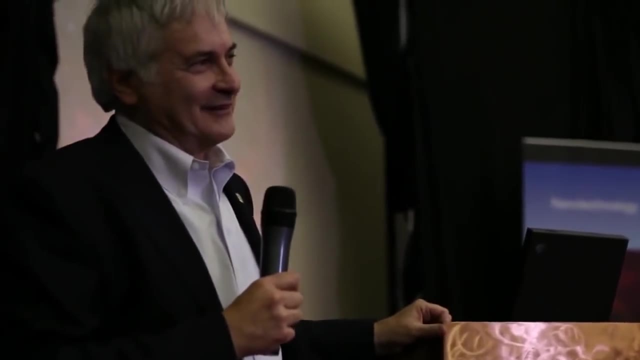 but, on the other hand, if you want to be the person responsible for destroying the earth right Now, I don't buy it. In fact, those of you who want to look it up, if you go to new scientists and type in my name, you'll find out. I wrote a little opinion piece on this about three weeks ago, and what I said about that to a 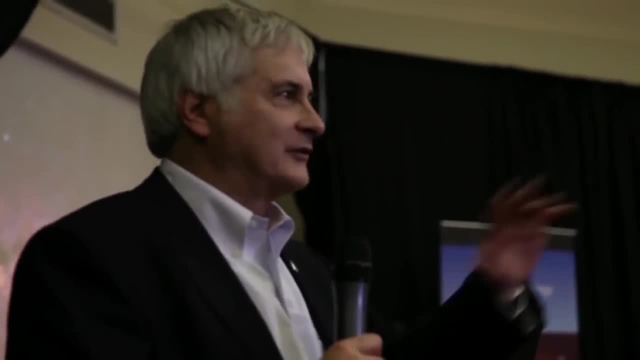 and what I said was this: look, you know you can worry about that. obviously we don't know what the aliens are capable of or what they're interested in doing or any of that stuff, and and maybe you don't want to risk the earth, I, I know it. 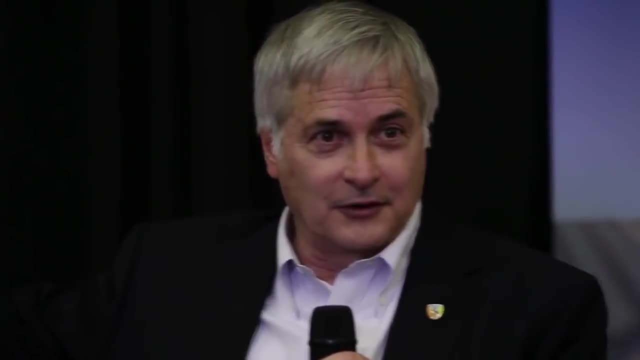 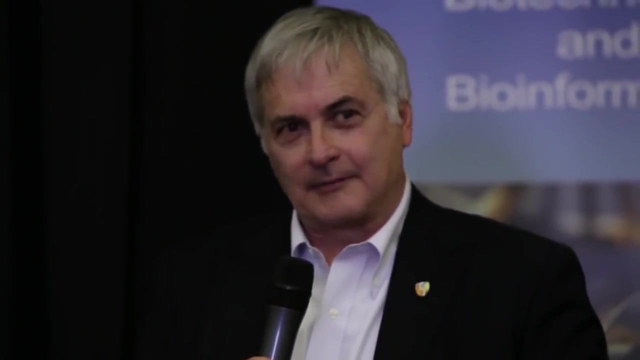 I didn't note it in there, but you know Carl Sagan sent a map of where the earth is out on the Pioneer and Voyager probes, right. so you know it's like a map of the stars home. you know, I'm sure nobody gave Carl Sagan permission to tell the. 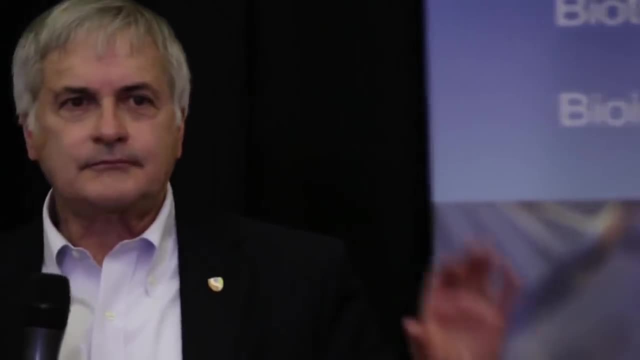 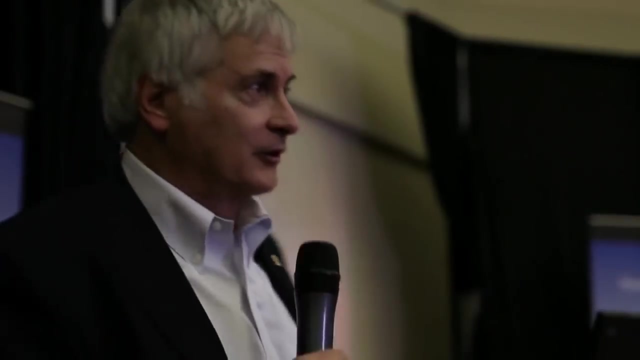 universe where you live. but he did. those things will never be found by aliens, it didn't matter, but a signal might be. and if you find a signal coming in, you might broadcast back: hi, we're the earthlings. you want to join our book club? we got. 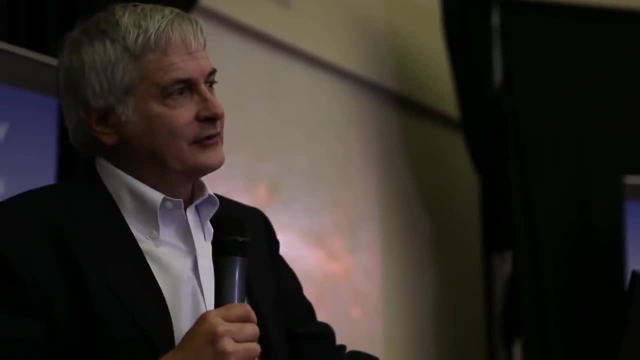 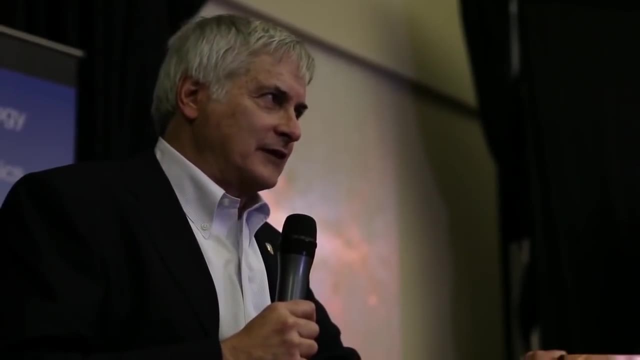 some used cars, what you know, you do all that and he's saying that maybe that's a bad idea. well, it may or may not be a bad idea, but the point was that we've been doing this for 70 years, right, we've been broadcasting in a space willy-nilly for. 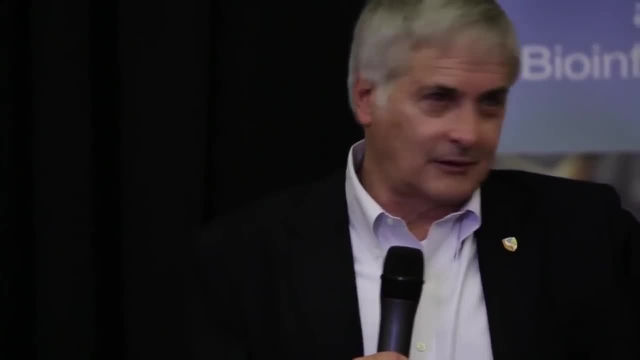 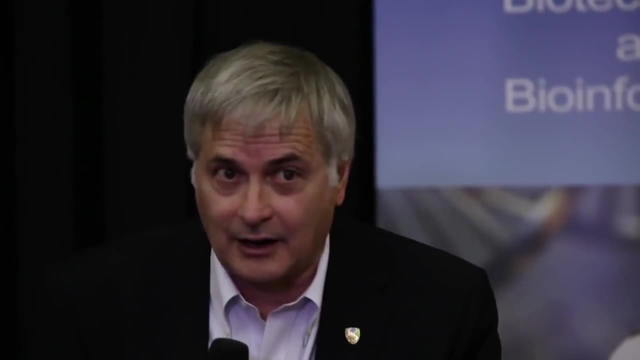 70 years, TV 24: 7, all. also the cities of Earth had these TV transmitters. you say yeah, yeah, but those signals are very weak by the time they get to the aliens. and that's true they are, but they're only we by. you know maybe three. 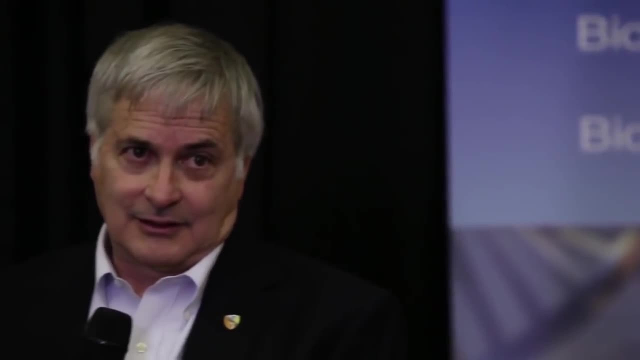 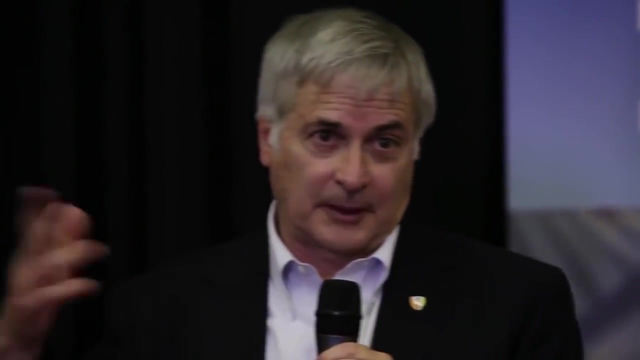 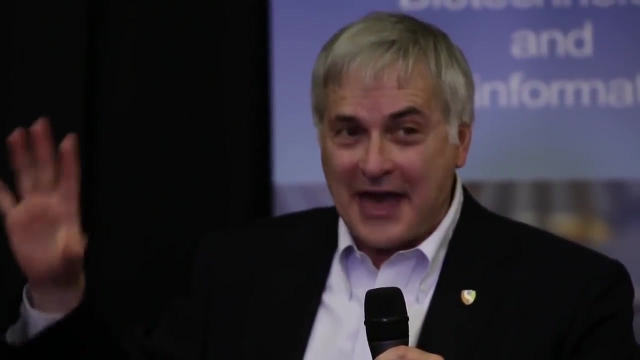 or four orders of magnitude below what we would be able to detect at those distances. so if you look at the growth in sensitivity of radio telescopes, you see that that increases by two orders of magnitude per century. if these aliens are capable of mounting an attack on Earth, they can easily pick up this stuff. 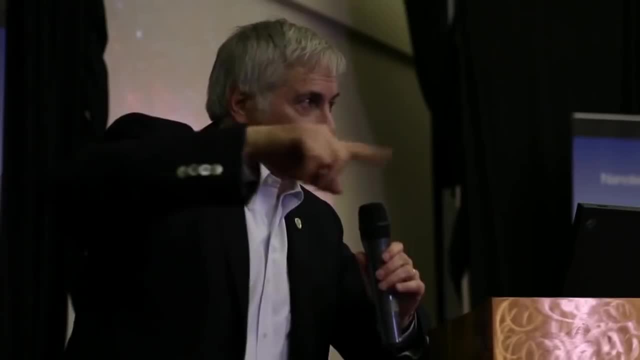 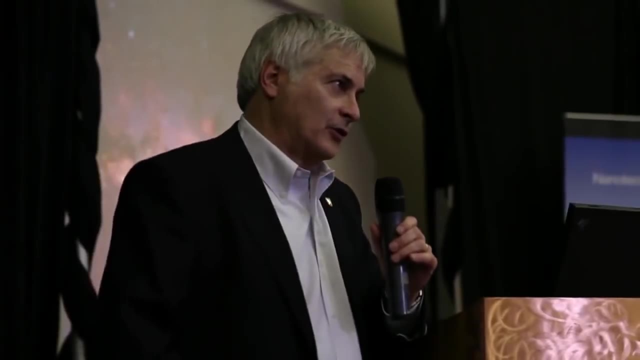 and in fact they've already gone just a couple hundred earth-sun distances away from their planet and they can use their own star as a gravitational lens, which gives them another 10 or 11 orders of magnitude of sensitivity. They can see our street lamps, frankly. 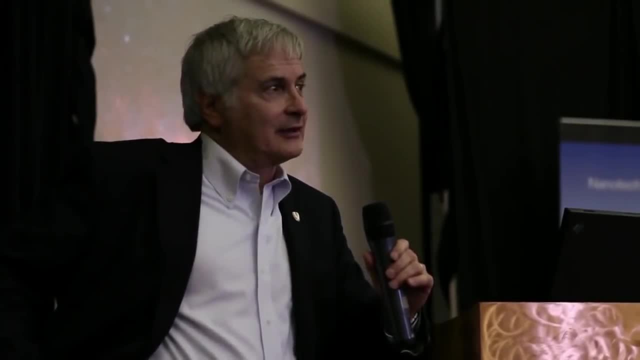 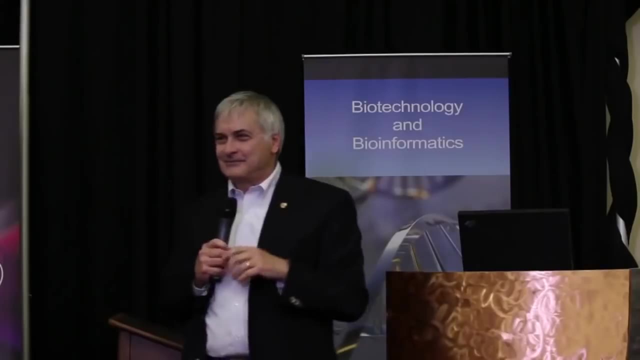 And so if you want to really be paranoid about this, that's fine, but it's too late. That horse has left the barn. Are you going to lose sleep about this? I don't Any other questions We want to get out of here. 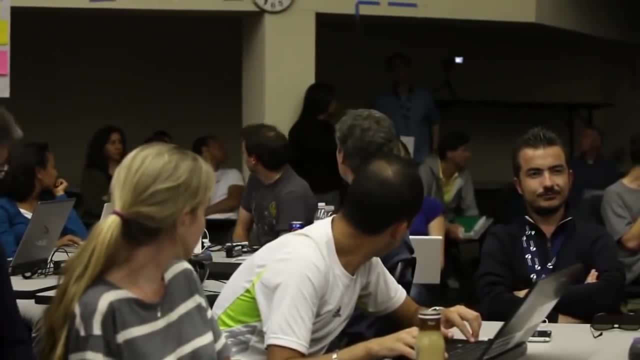 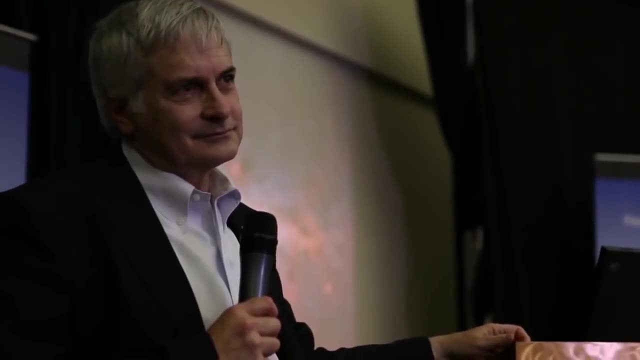 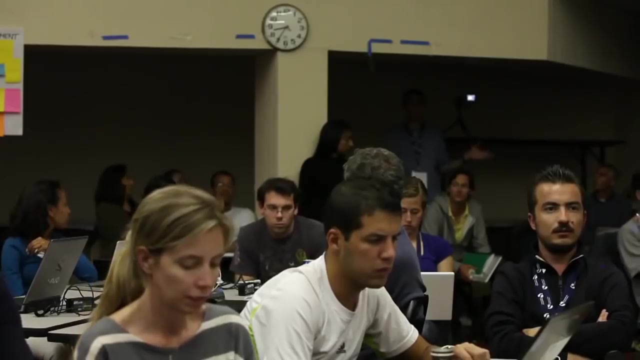 Yeah, Could it be possible that maybe we're looking for radio signals and maybe, because of our development cycle, that's not what the aliens are out there using, Because we're starting to learn that quantum computing, quantum entanglement, allows us to begin to start looking at how we can transmit information at a quantum level. 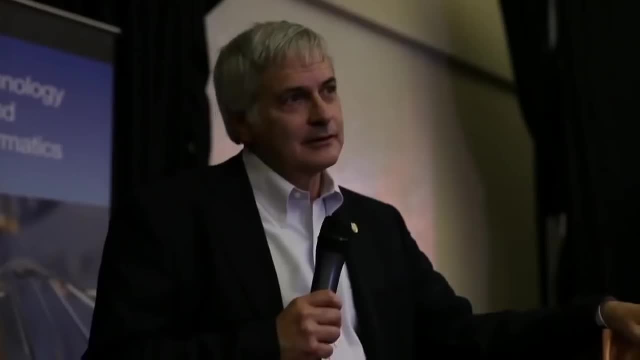 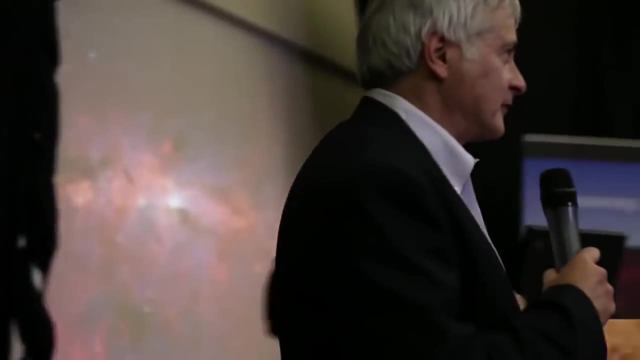 So maybe we're just kind of, you know, not advanced enough. Yeah, Well, that's certainly possible. Everybody heard the question. Anybody here mind asking whether you heard the question? Yeah, I get e-mails about that essentially every day. 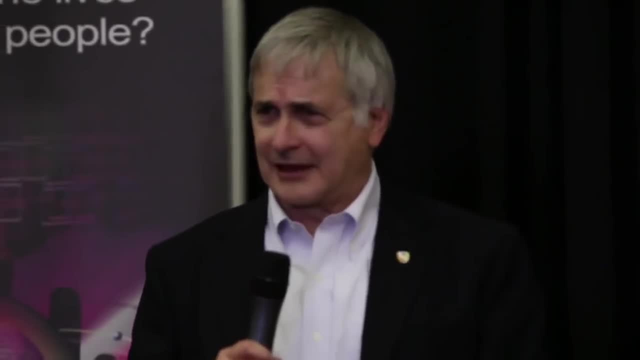 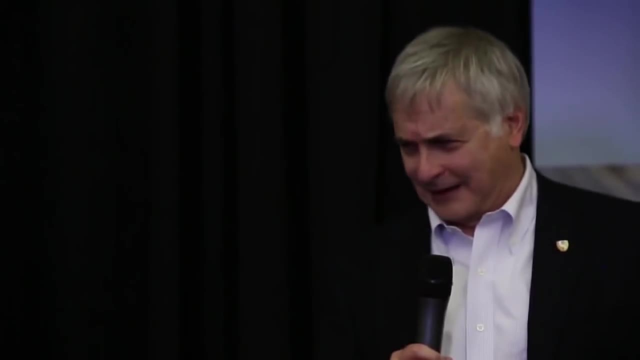 They say radio, Radio signals. We also look for flashing light, Electromagnetic radiation, How yesterday, how 20th century. That may be, That may be, But that you know. it's kind of like telling Chris Columbus: hey, man, forget these wooden ships. 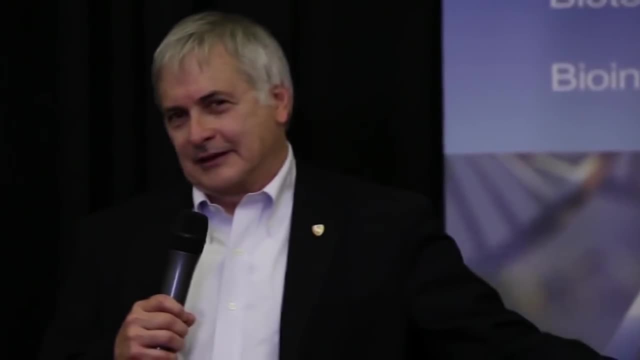 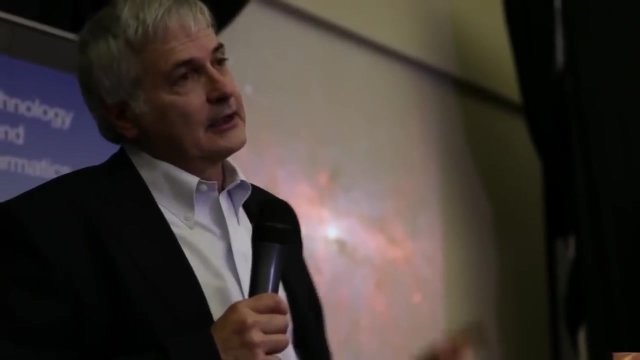 You know, just wait a couple hundred years, You'll be able to cross the Atlantic in six hours eating peanuts off your lap. you know That doesn't help him, And it turns out the wooden ships were good enough. The point is this: 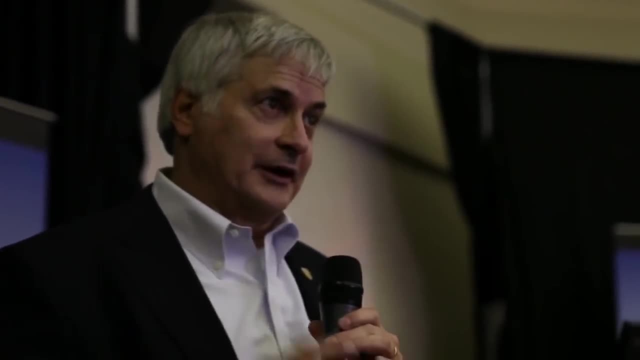 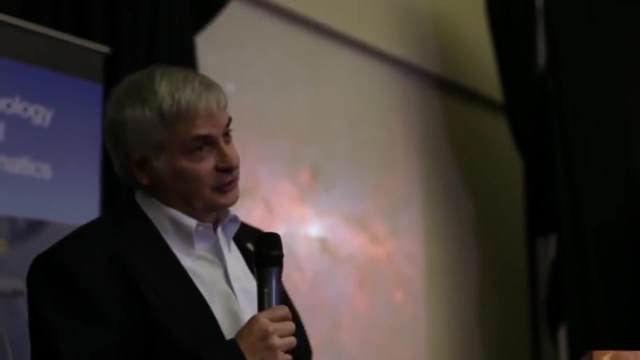 We don't know. There may be physics that allow some sort of communication mode that really trumps the sorts of things we've thought of, In which case this may be barking up the wrong arboreal fixture, I mean. maybe that's true. 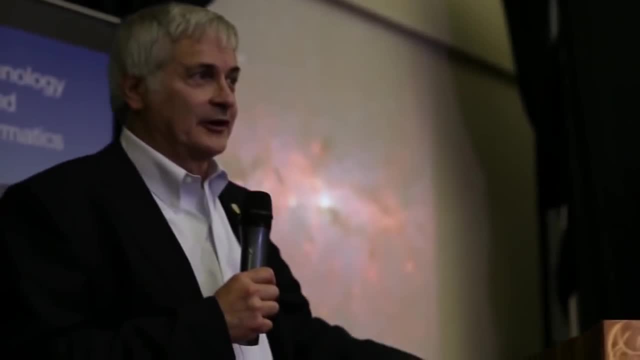 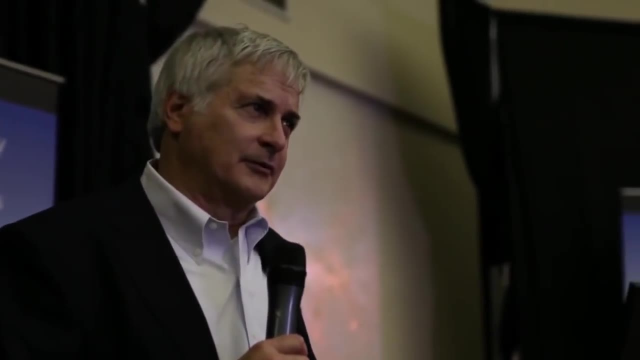 But is that an argument to say, well, we just won't do this, We'll sit on our hands and wait for other physics? That doesn't sound like such a good argument to me. And as far as quantum entanglement is concerned, there's something called Bell's theorem. 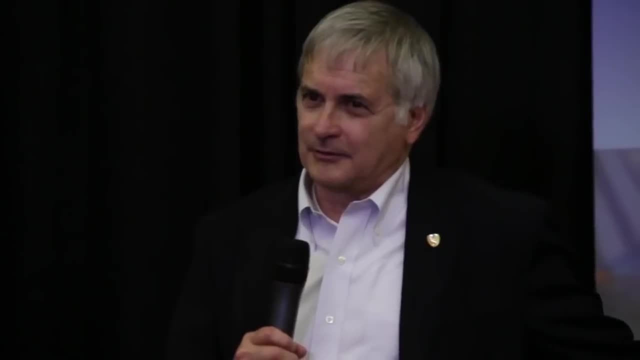 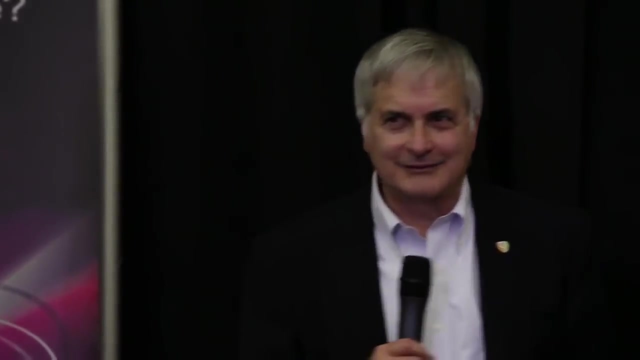 You may want to look it up. It's not clear that you know quantum entanglement will allow you to actually communicate faster than the speed of light. Quantum entanglement works, but in terms of sending information it may not beat the speed of light. 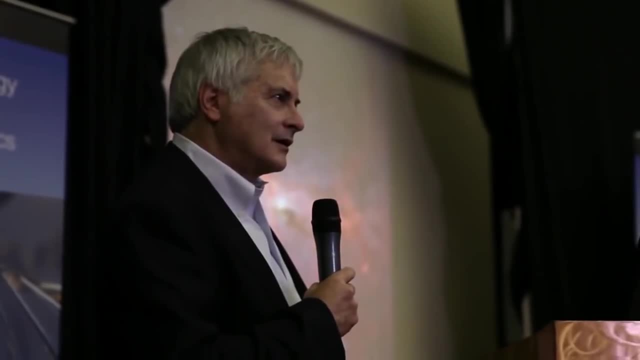 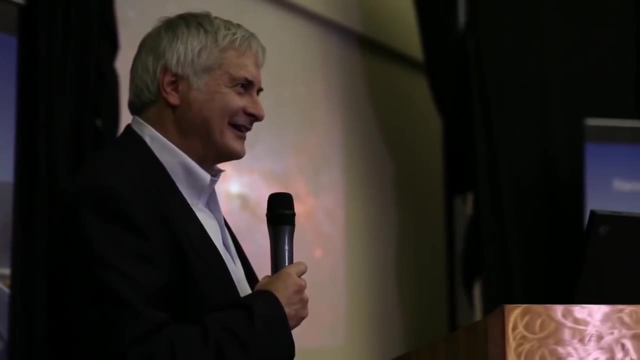 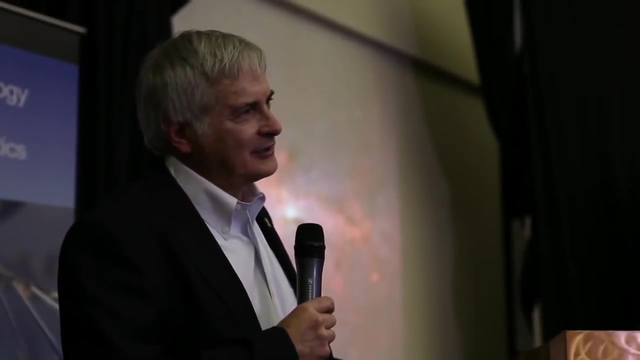 Yeah, Okay, Yeah. What would be the name of that first digital signal processor, the custom one you had built? Were you involved with that? Is that what you're asking? Which custom digital signal You mean? the one that we used in the early 1990s? 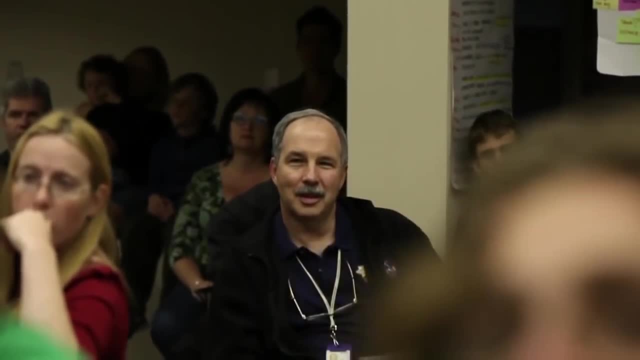 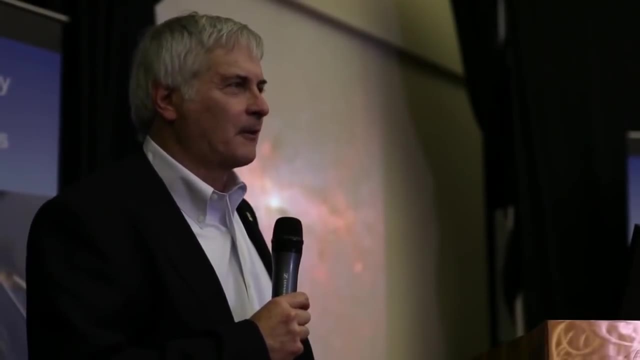 The original Project Phoenix custom one. Oh, it's still being used. We use it for the Island Telescope Array. We're trying to replace it. Yeah, It's still. most of it is still being used. It is, If you're a part of the engineering team. 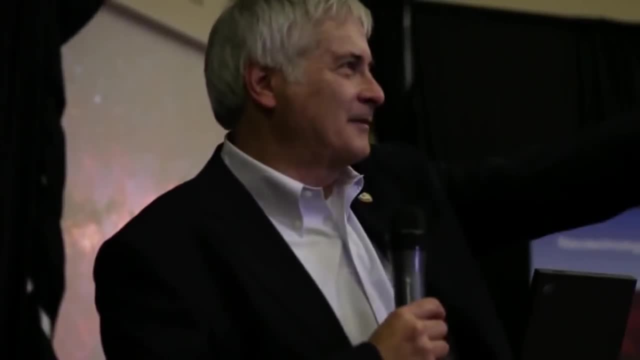 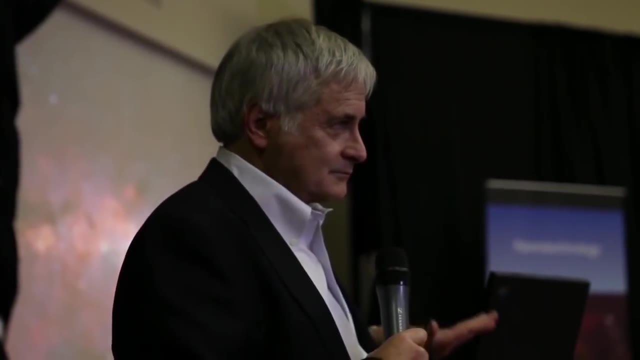 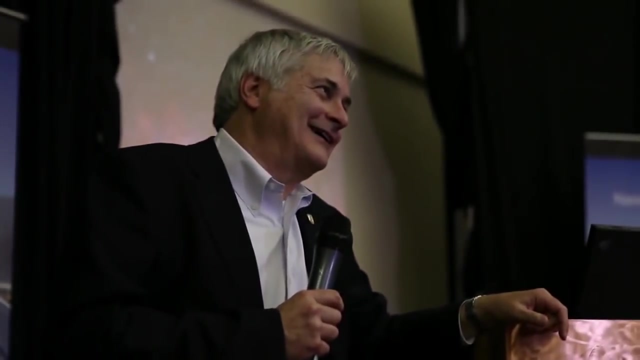 my, I'd take my hat off to you if I had a hat, The guy behind you. What about like topology and like the geometry of the universe as a medium of faster than speed of light travel? Well, Like a mathematical approach, Because I mean, obviously nothing goes faster than C, that we know. Yeah, Well, you're suggesting: why don't we just warp space and then we reduce the distance between us and them, and then we get the signal faster, Which is true if you have, you know, a black hole at your disposal for warping space adequately to do that. 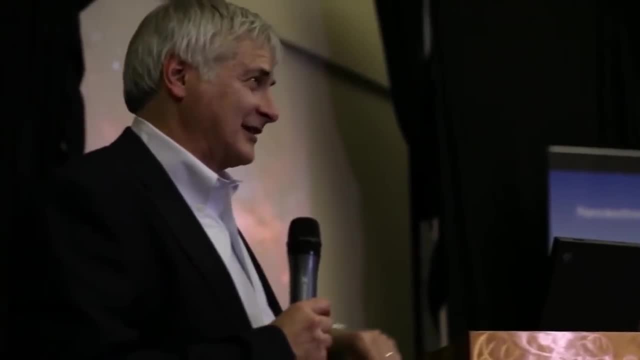 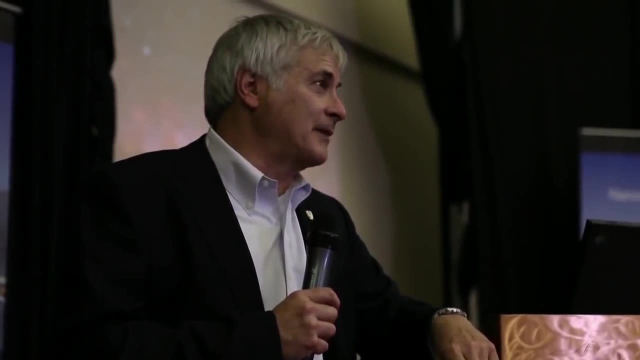 I mean, yeah, well, we don't, maybe they do. I mean that sounds like some science fiction film by Ray Bradbury or a story right, Yeah, Yeah, well, who knows, They may do that. I mean, that's sort of like asking: what about faster than light travel? 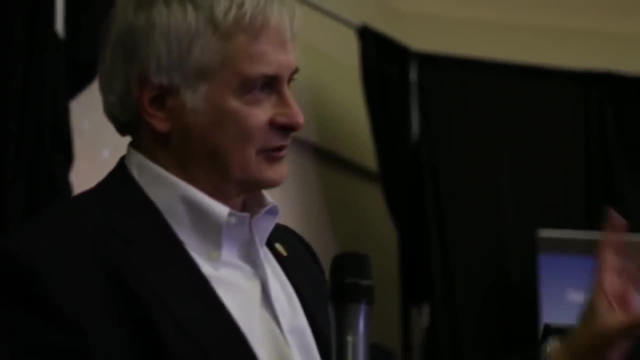 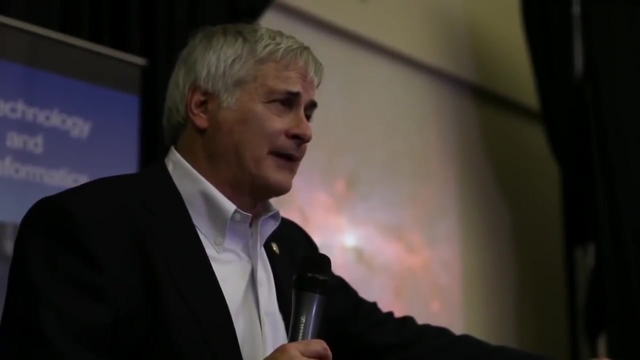 You know the way to implement. that is to warp space. You don't really go faster than light, but you just shorten the distance by creating wormholes- Wormholes, as you know, wormholes work on blackboards. It's unclear whether they would work in practice. 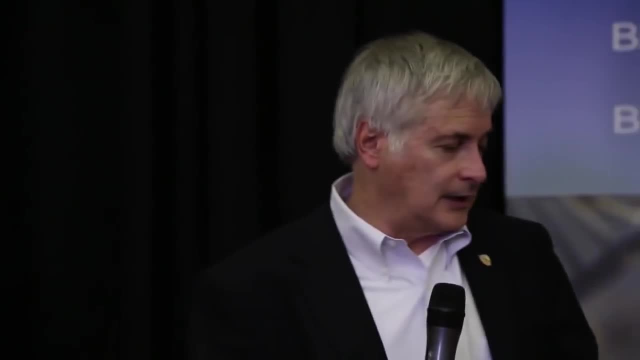 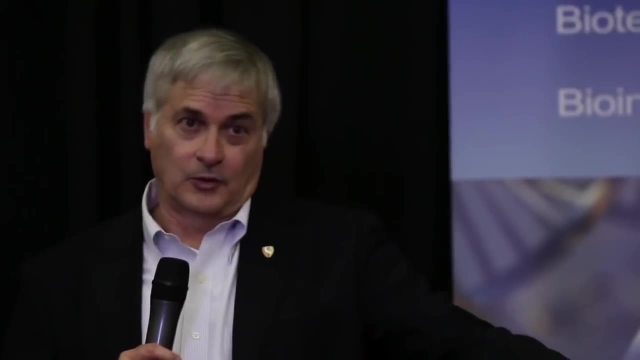 I asked a cosmologist about this when I was living in the United States- I was living in Europe, actually about that- And I said: do you think you could ever in fact use wormholes for travel from one spot in the universe to another or one era to another in traveling time? 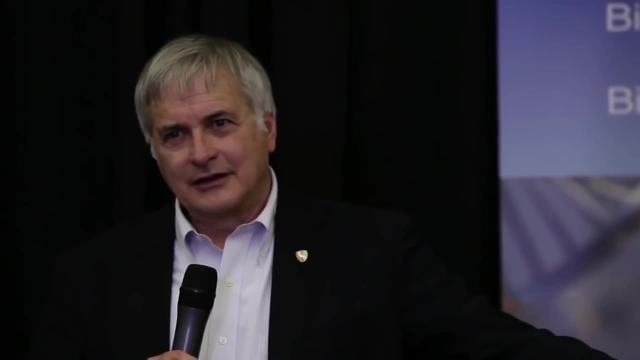 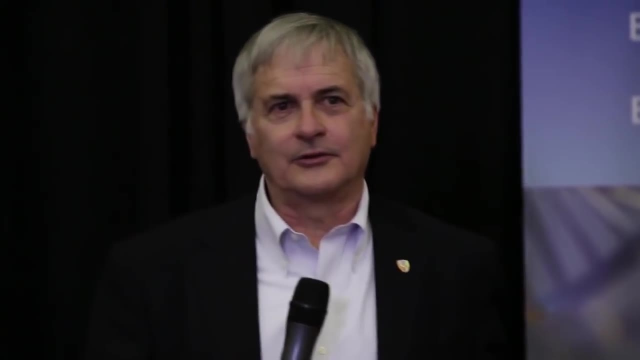 And he said he doubted it. He said because if that were the case, then an alien could pop up in the seat next to you and he didn't think that was a nice thing to do. So his take on it was that it wasn't likely to prove practical or possible. 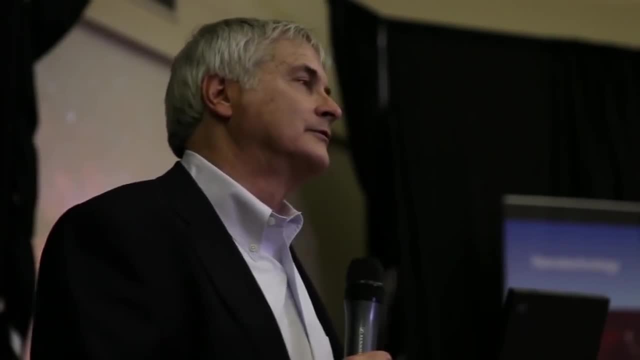 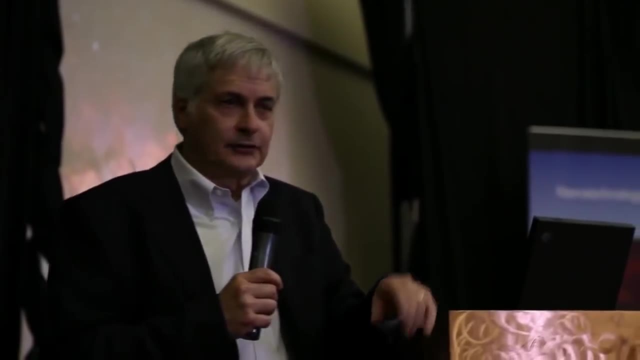 Practical is a different word possible, But I don't think anybody knows If you can work it out Between now and next Tuesday, you know how would we decode the signal. First off, let me point out to you that in our radio searches- it's not true in the optical, but in the radio searches- we integrate for minutes at a time. 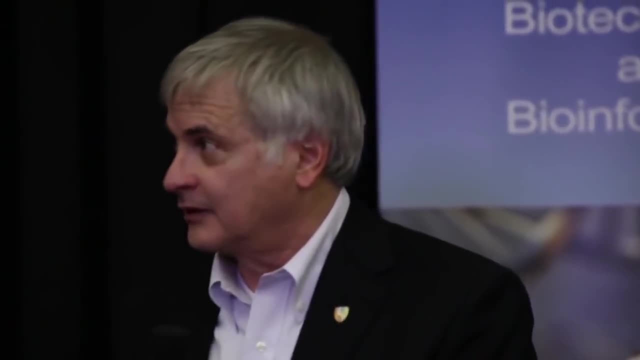 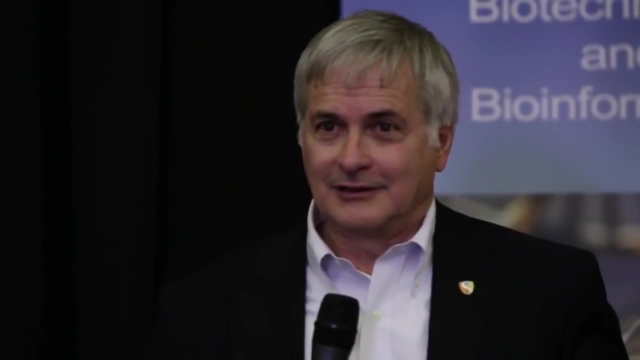 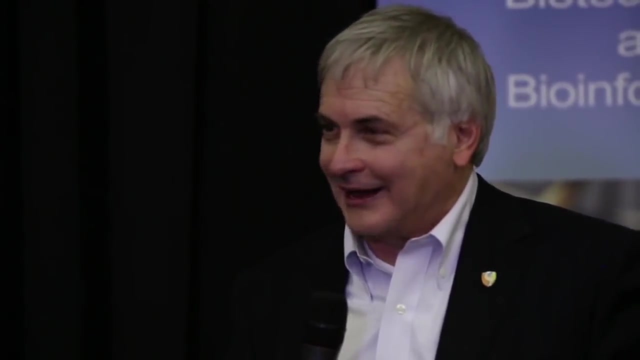 In other words, we average the incoming cosmic static for a few minutes. That builds up the sensitivity so you can find a much weaker signal, But obviously it throws away the information. If you took a TV signal which has like a five megahertz bandwidth, you take a TV signal and you average it for two minutes. well, the picture and sound are pretty much gone away. 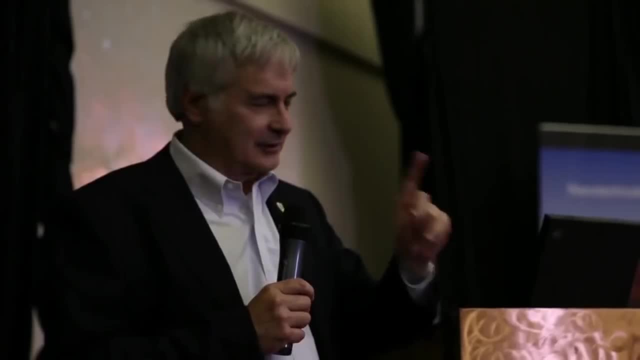 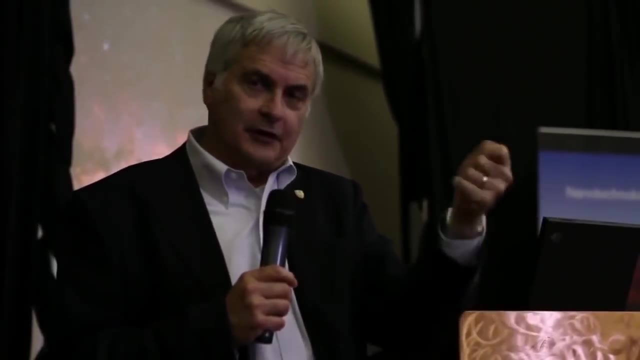 All that's left is the fact that you know that there's a transmitter right, There's a carrier. Okay, So we do the same. And if you found that, you say, okay, well, let's just change the hardware a little bit so we can see variations that are occurring at a microsecond level or a nanosecond level. 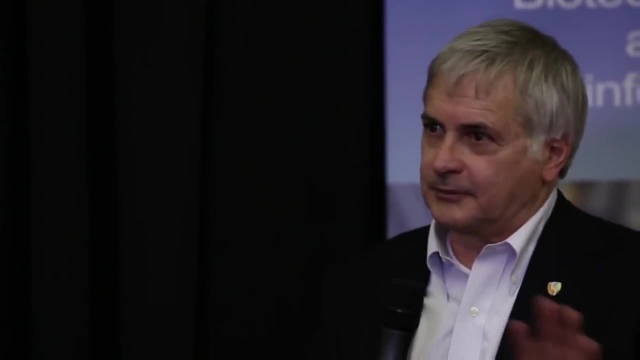 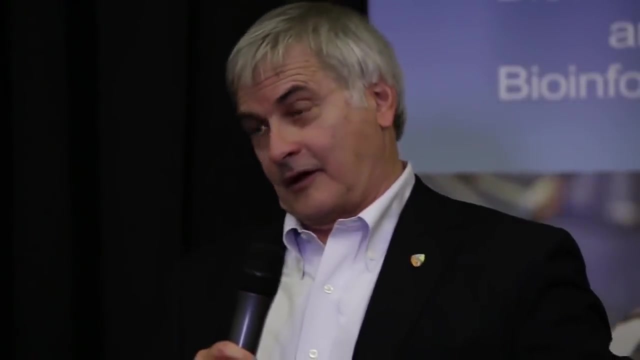 But now you don't have the sensitivity. In order to do that, you'd have to build an instrument that, in the case of a TV signal, would be four orders of magnitude bigger, So that's a very much bigger antenna, But, on the other hand, all of this, which is privately funded, completely dependent on people like you. 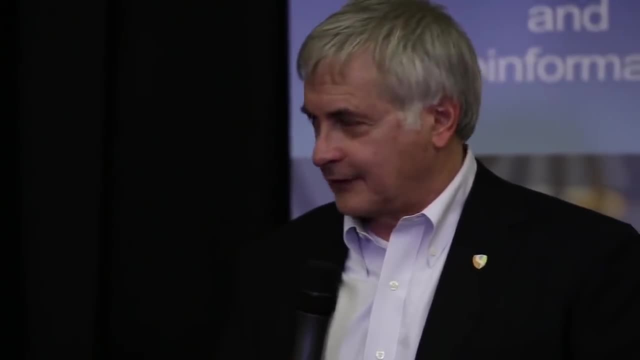 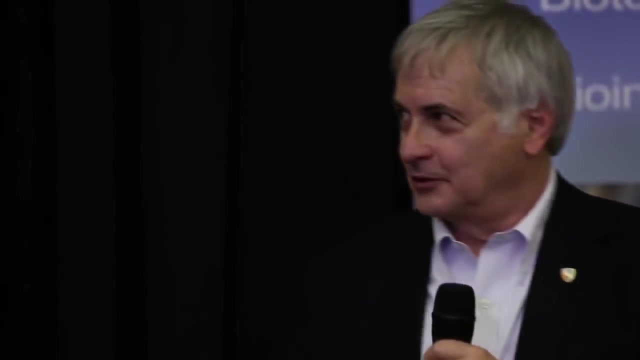 Right To fund it. I think you would get the money to build that. Yeah, yeah, very quickly, Okay, So let's assume that happens. And then they get all these bits coming down, And so the question is, what do you do with them? 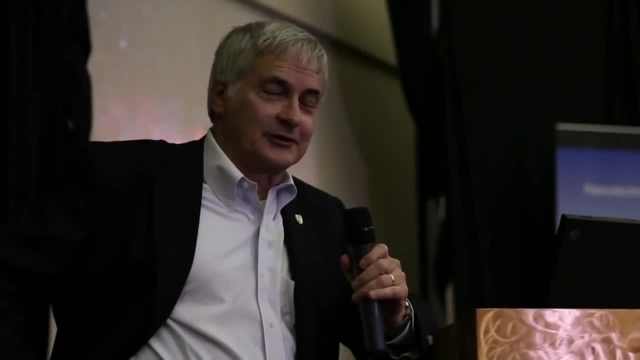 I think. I mean, there are two approaches. You could just, you know, turn them over to some experts. It sounds like the Dead Sea Scrolls, But we still don't know what the Dead Sea Scrolls said. so you know. 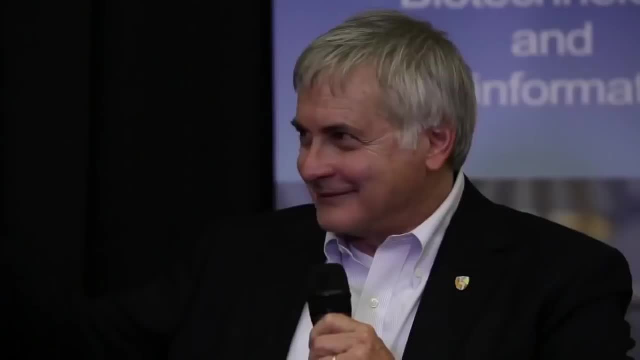 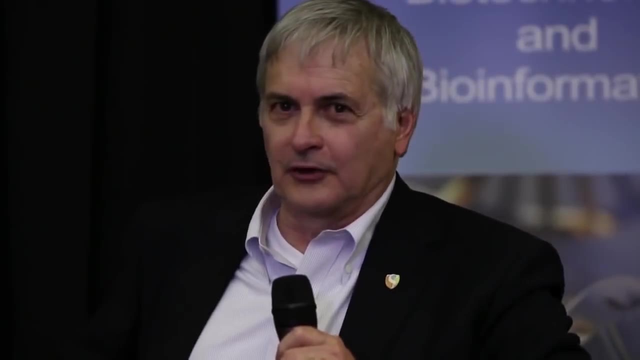 Or you could just put them out on the web. Everybody download them to your hard drive and work on it, And I'm not sure that you'd ever figure it out. I mean, who knows? I mean, would Neanderthals ever figure out a digital television signal? 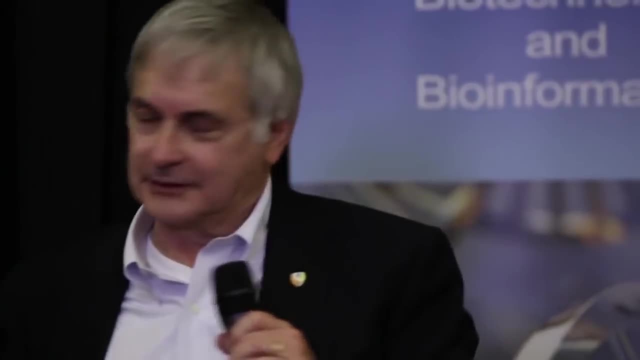 Probably not, Even if you gave it to them. you know, it's not that they were stupid, But they'd probably not figure it out. And somebody suggested to me: yeah, after 200 years of trying, people would start worshipping these bits. 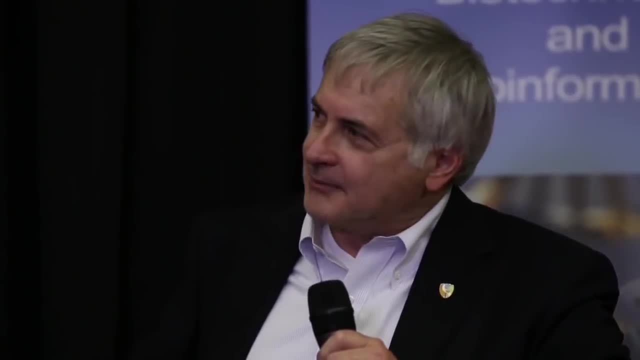 I don't know if that happened or not. I mean, if they're trying to make it easy for you to figure it out, then maybe you would see pictures and things like that, and you know a dictionary Who knows what they'd do. 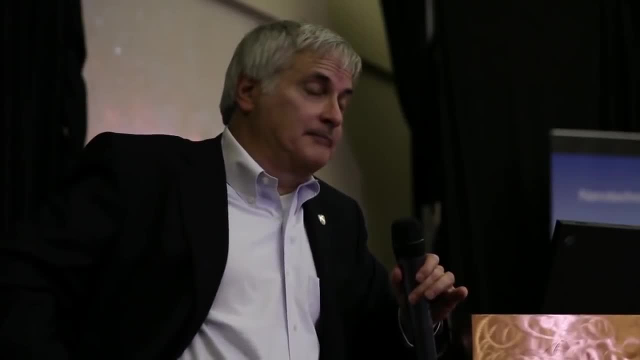 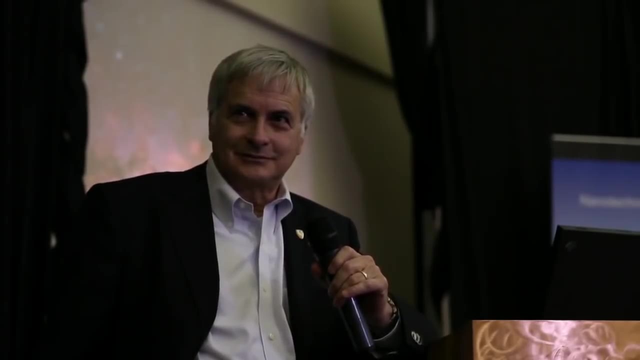 But I think you, in my opinion, the best thing you do is just put it all out there, Let everybody try, Yeah, but there's no sort of systematic way of looking at this. I mean to put it that way: everybody tries a little bit. 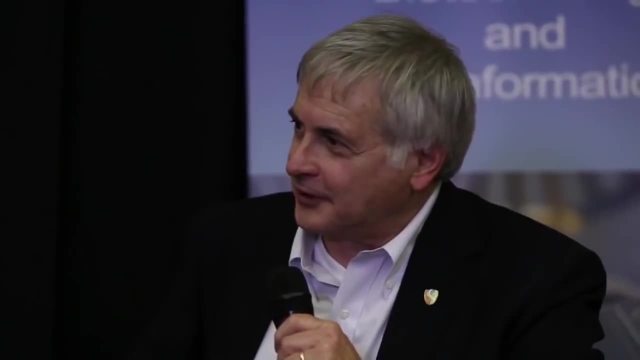 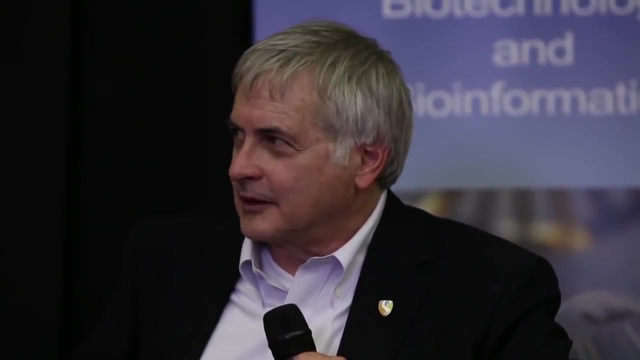 Well, letting everybody try means that you also let the experts try, insofar as they're experts, I mean the people who are good at pattern recognition, the people who are good at decoding things. you know they'd be amongst those people that got hold of it. 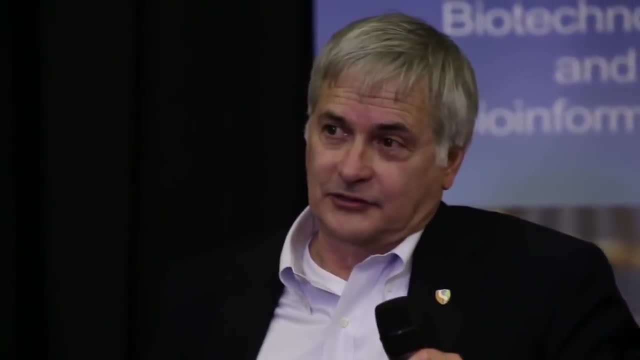 I mean, think about it. The hieroglyphics were decoded very quickly by Champollion in you know four or five years Now. mind you, he was expert in it. He also had the Rosetta Stone and all this stuff. 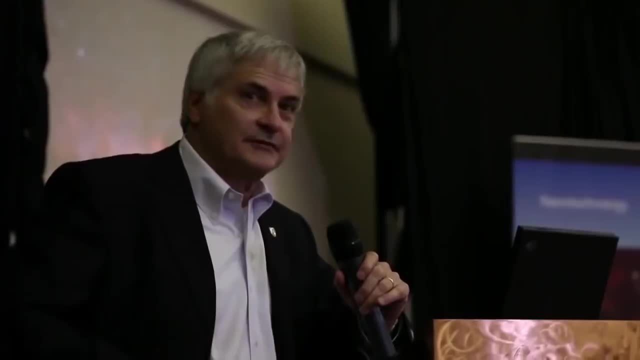 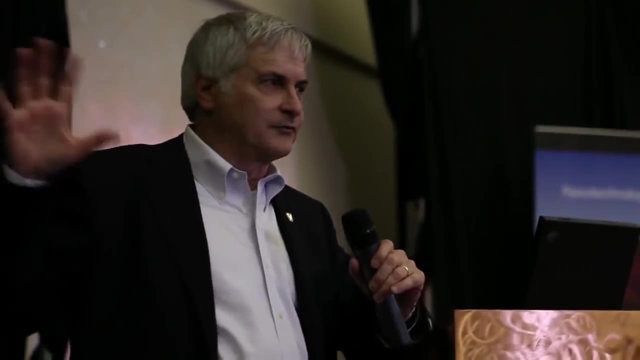 They figured it out anyhow, even without the Rosetta Stone, because there was so much of it. There was enormous redundancy, There was a lot of material right. There's some codexes from, you know, middle America that have never been figured out. 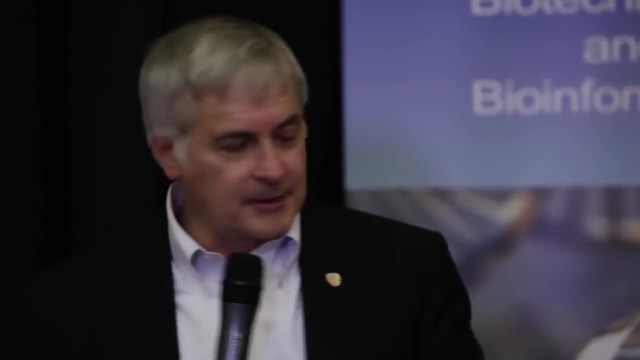 because there isn't much material right, So it would help to have a lot. I mean, people ask: what should we broadcast to the aliens? you know, And I even wrote a paper on that. I mean, you know, a lot of my colleagues say, well, we ought to use mathematics. 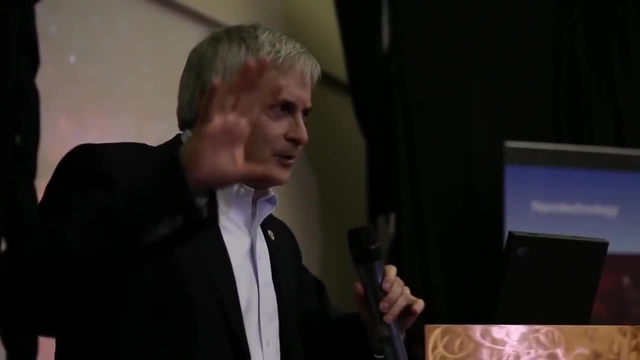 or we ought to send them our best music, or we ought to send them, you know, our noblest achievements. The heck with all that. I wrote the paper and I said: send them the Google servers, Just send them everything. 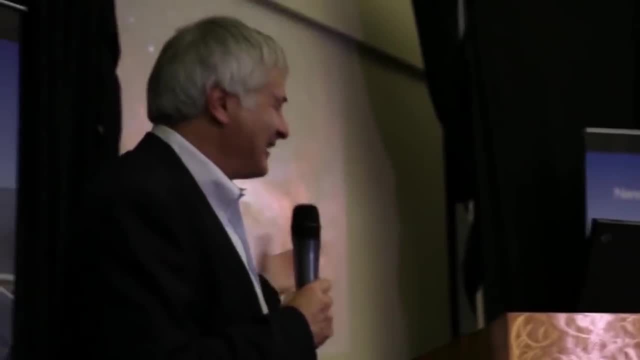 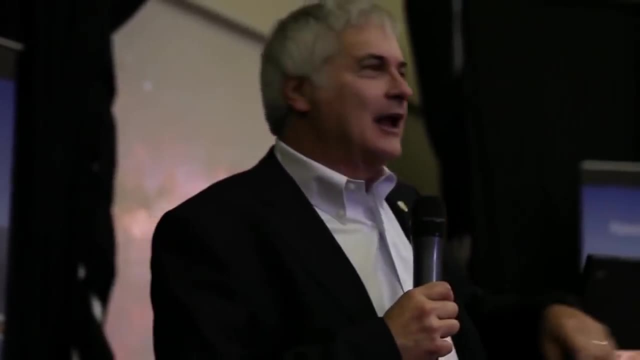 You know, somebody said: but there's a lot of porn on that, You know I said well, so what? You think that the aliens would be offended by human porn? God nude humans zork. What do you think? 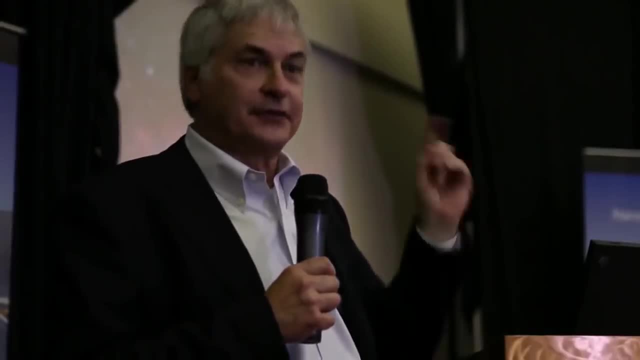 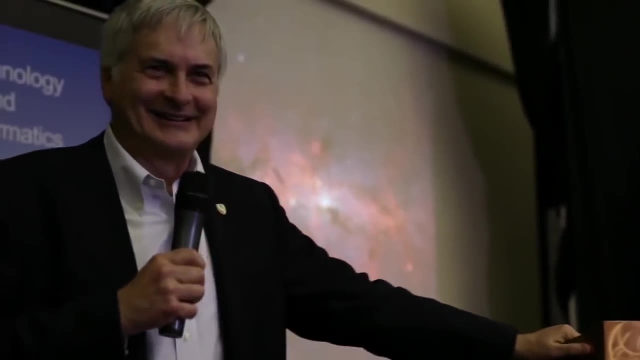 But send it because it's so redundant. There's so much redundant information that they'll figure a lot of it out. That was my suggestion, But nobody knows. This is a problem down the road. You look familiar. Yeah, I saw your cousin once. yeah, 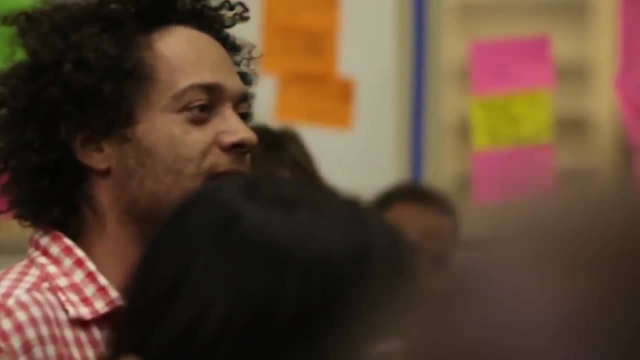 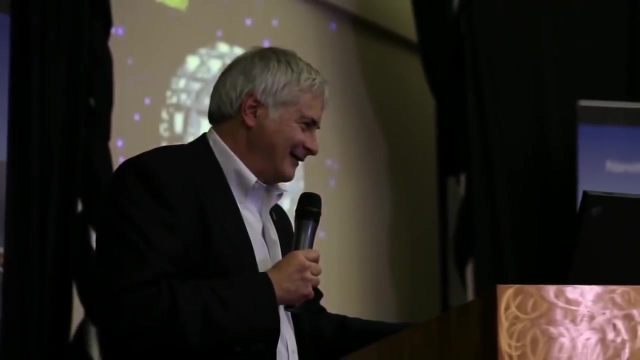 If a signal is sent to the internet. if and when a signal is discovered, what is? or is there a protocol for notifying the general population of the planet that, hey, we've got some buddies, or not buddies? Okay, All right. 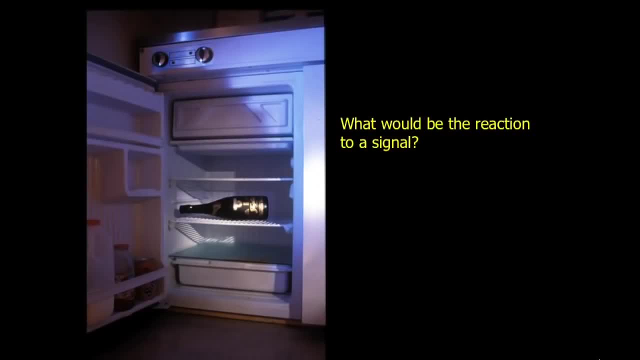 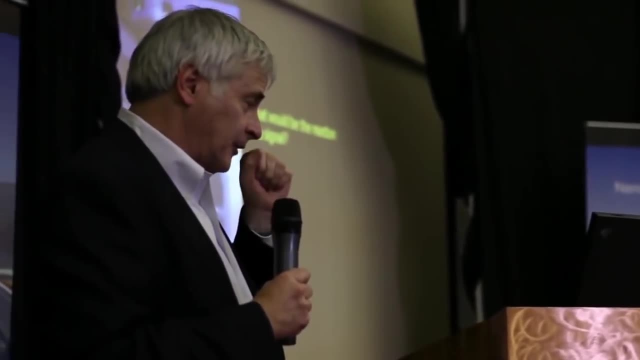 You forced me to show these last slides. There is a bottle of champagne at the observatories. We always keep it there. It's really there. I made this photo, Sorry, in Arecibo in Puerto Rico, But this is the island telescope right too. 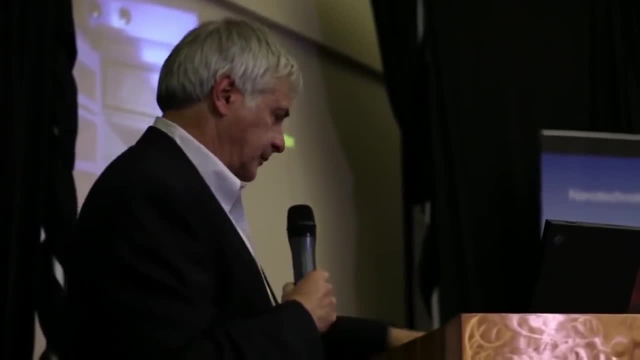 Excuse me, Every time I go to the observatory it's a different bottle of champagne. But actually when you actually get a signal, nobody thinks of it. I mean, everybody thinks of it. Everybody thinks it would be a big cover-up and all that. 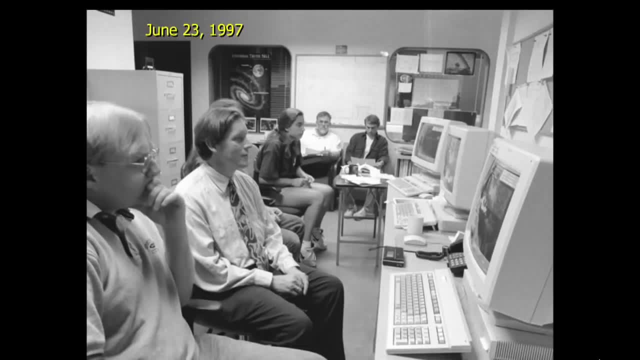 This is a photo I made at the Asseti Observatory- sorry, the Asseti Institute- back in 1997 in June. This was made at 3.30 in the morning And we were following a signal that looked like it was the real deal. 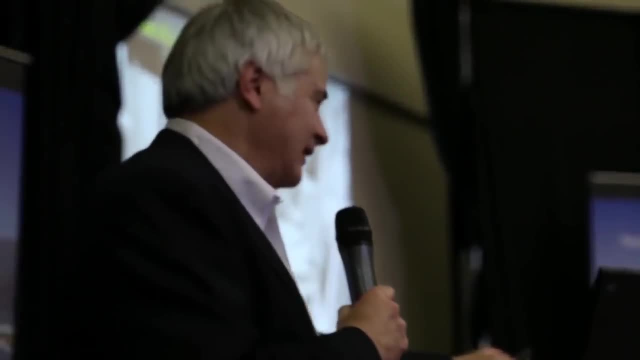 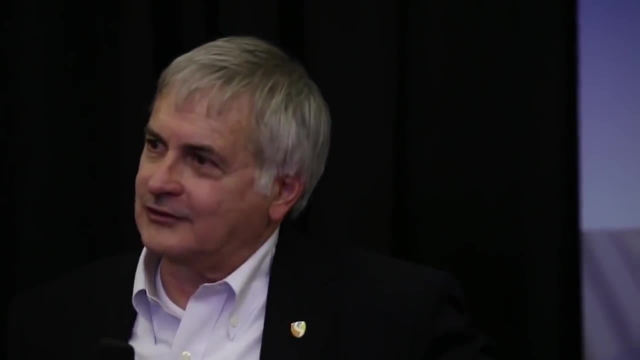 If any of you still have an interest, by the way, in this subject despite this talk, I have a book called Confessions of an Alien Hunter And I begin with this signal because it was sort of interesting. It showed what happens if we actually get a signal. 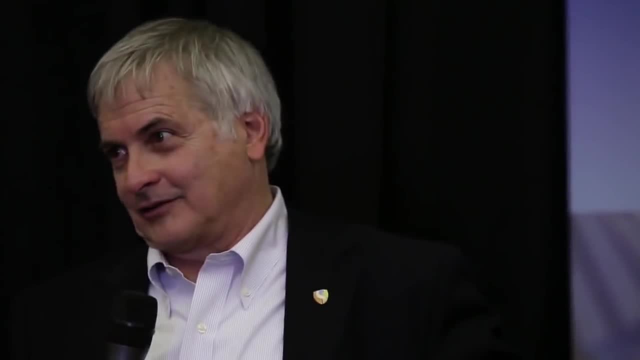 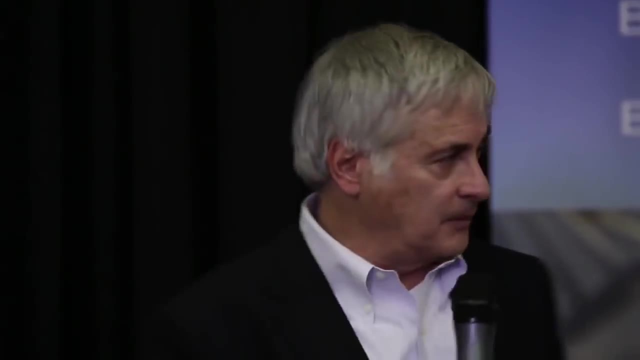 Because we thought it might be the real deal for about 16 hours. Turned out it was the Soho Solar Research Satellite. The signal was bouncing around the steelwork of the antenna- just the right way to mimic ET. But there we are at 3.30 in the morning and nobody's going out to In-N-Out Burger. 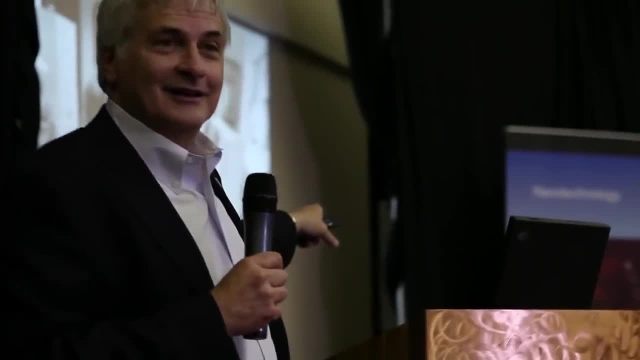 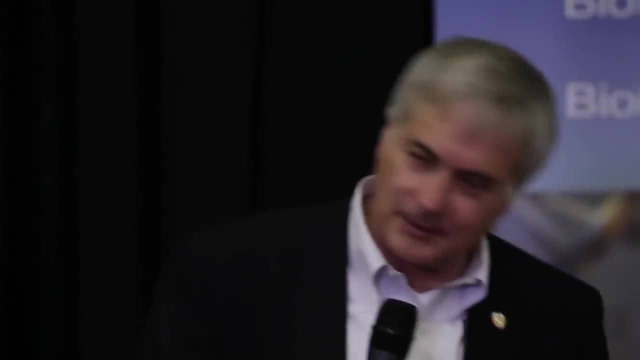 and nobody's going home to go to sleep. We're just sitting there, glued to these monitors, right At 9.30, the star had set. We had to wait 12 hours before we could see it again, And I was sort of half asleep at my desk and the phone rings. 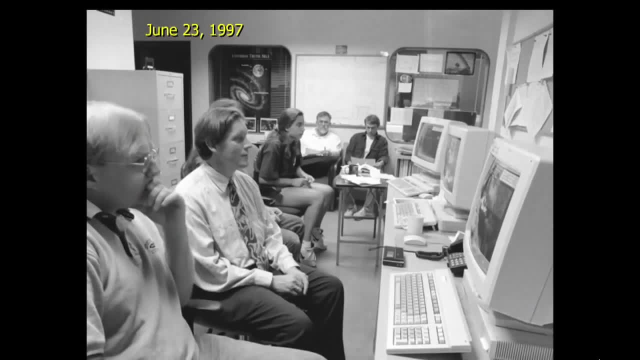 And it's the New York Times right, They already knew about it. There's no secrecy, There's no policy of secrecy. So what would actually happen is that the media would be all over it and, of course, the more responsible. 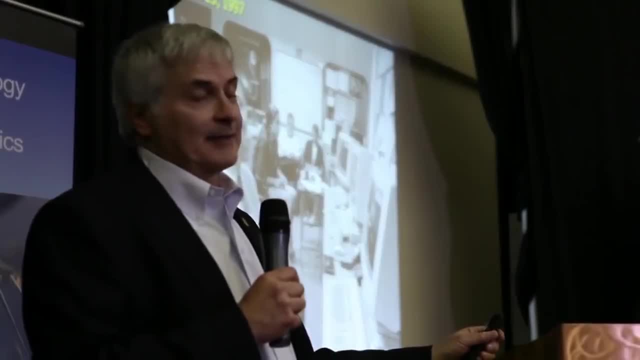 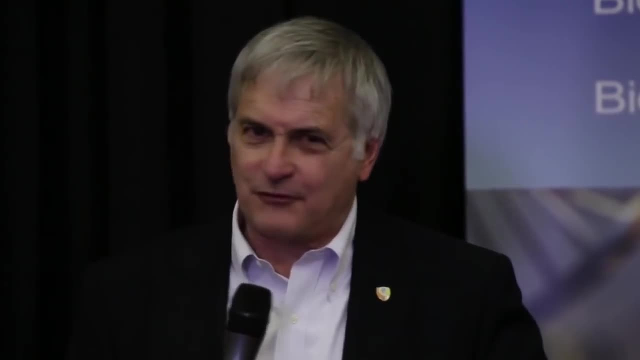 The more responsible media will wait until you've confirmed the signal is truly being extraterrestrial And that might take you a week. But the Weekly World News, the checkout line press, they're not going to wait, So you'll read about it first at Safeway or at Lucky. 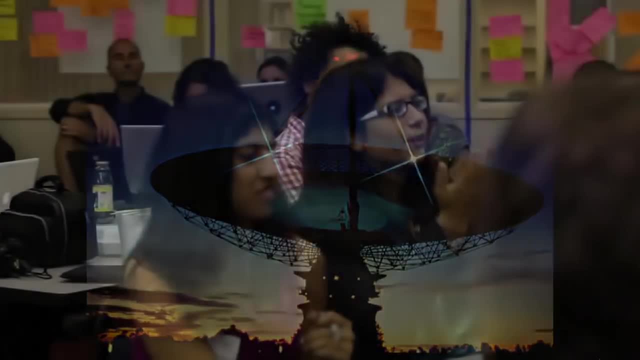 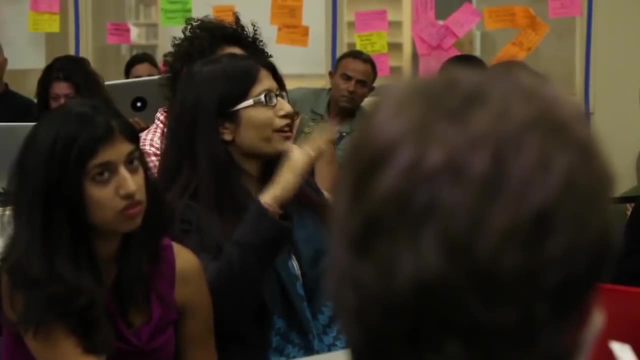 That's for sure. Yes, you So actually asking the reverse of Conor's question. what if? I mean this is assuming that whatever signal was intercepted was intercepted by SETI? What if there was some crazy UFO person who actually did intercept the signal? 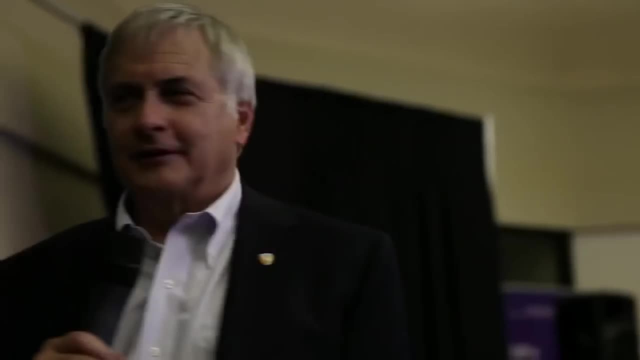 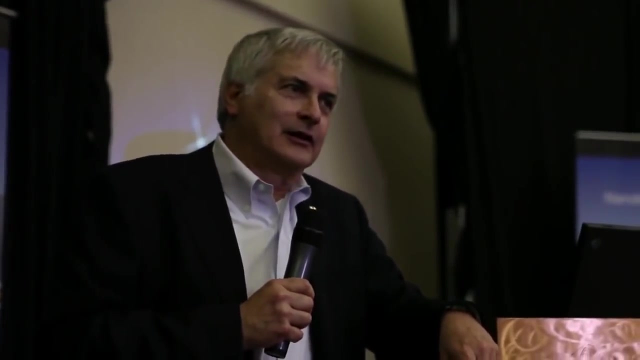 How would they even know? I appreciate your implication that the people at SETI are not crazy and wacky. Yeah, yeah, well, we've seen that happen. actually, What if it's somebody out there, just the great unwashed right, that find the signal? 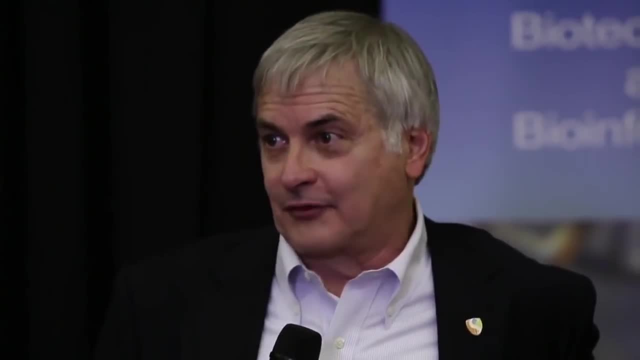 That could very well happen, And very often there's a lot of precedent in science for discoveries being made by people who weren't looking for what it is that was discovered, right, I mean, you know, penicillin, whatever x-rays. 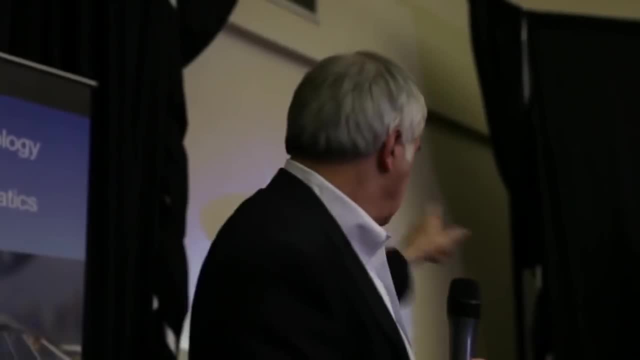 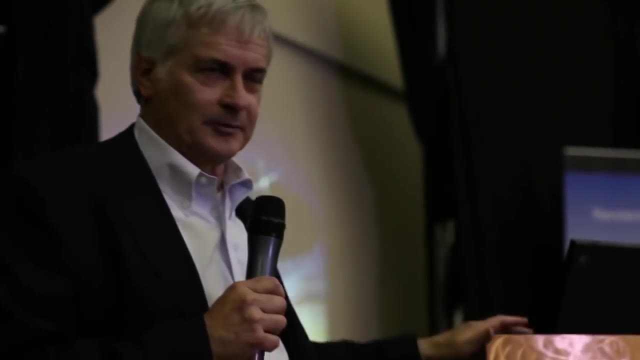 The that could happen. There was a in. I think it was 1999 or 2000.. There was an Internet Claim, a claim on the Internet, some guy's website by an amateur astronomer in the UK. 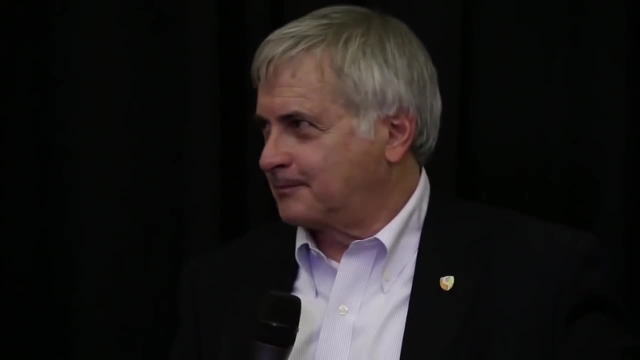 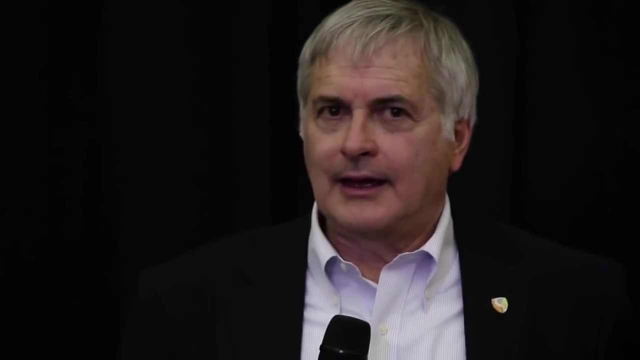 who said that he had secretly used his employer's dish to look at the star EQ Pegasi and had found a signal And he was publishing this. And you know I was driving home from- well, I wasn't, I had given some talk down in Monterey. 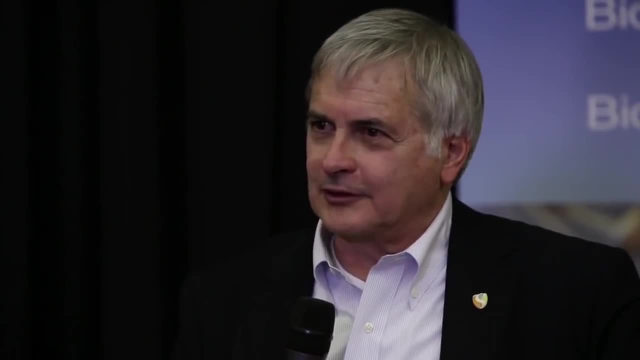 or something. I was driving up 101 the night that this story broke And I was listening to Art Bell- I don't know if you know- coast-to-coast AM this late afternoon And he was saying I wish Seth would call me about this. 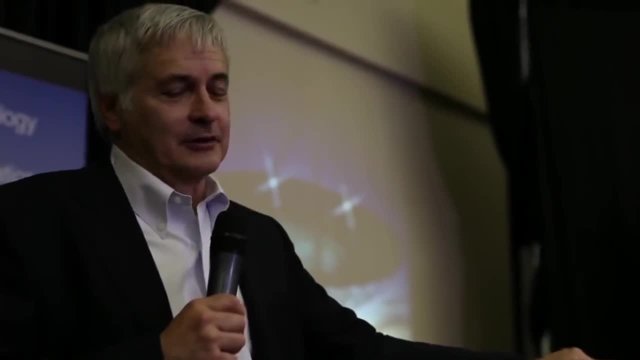 And I nearly drove off 101.. And I got home My wife said Art Bell's been calling you And I said I figured that And I went on And I said: look, it looks like a hoax to me. 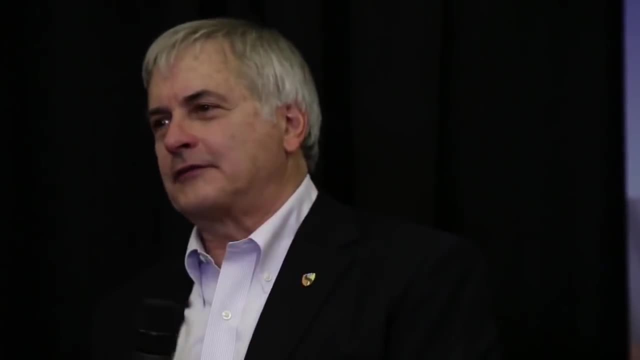 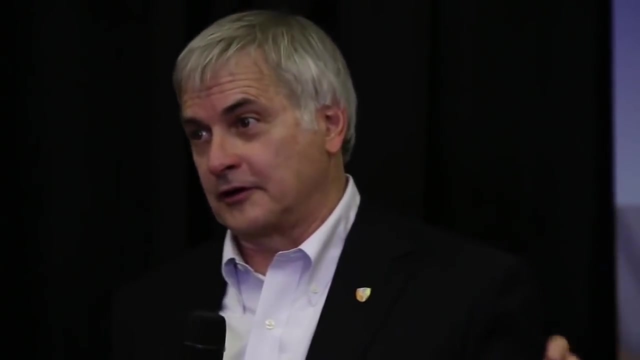 Well, for a week there were all sorts of efforts to figure out whether this was a hoax or not a hoax, And it even led some people in Australia to actually use radio telescope time to go verify this thing. It was a complete hoax. 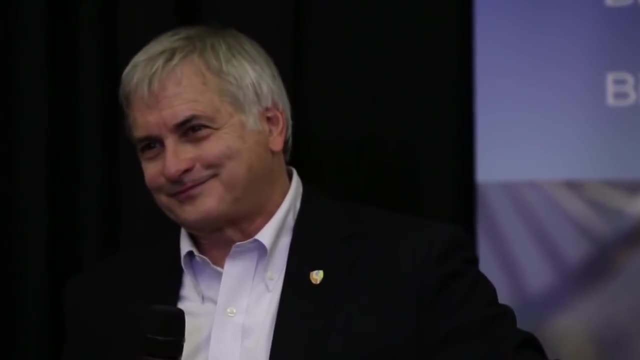 It was obvious that it was a hoax. To me it was obvious. But you know, So you know, You could see it. You could say: but what if that had been real? That's really your question. What happens then?